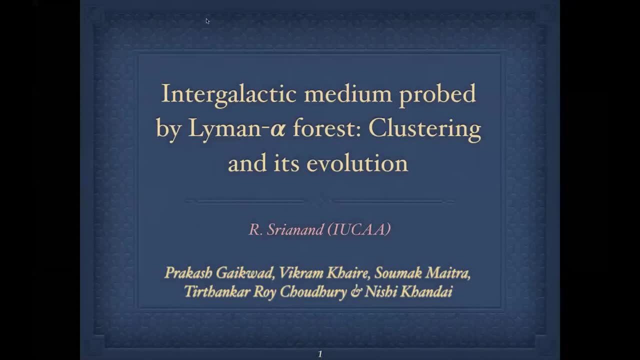 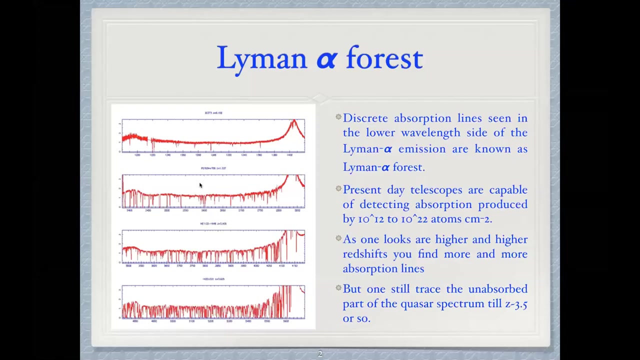 Sreyanand. He will talk about intergalactic medium probed by Lyman-alpha forest, clustering and its evolution. So, Anand, I will give you a warning after 20 minutes. So that will be a five minute warning And then there will be five minutes for questions. You can start now. 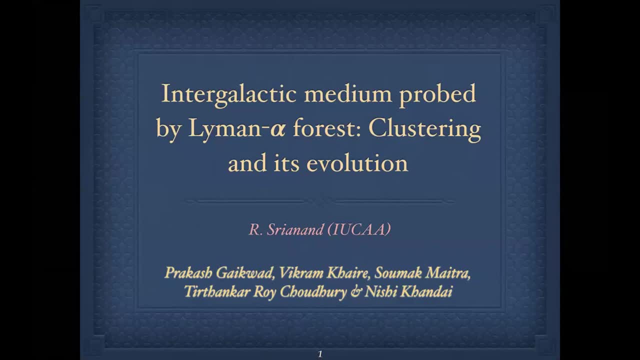 So thank you, Raghunathan. Can you hear me? Yes, I can hear you. Okay, good afternoon. I will be talking about Lyman-alpha forest seen in the spectra of quasars, and how one can use it to extract. 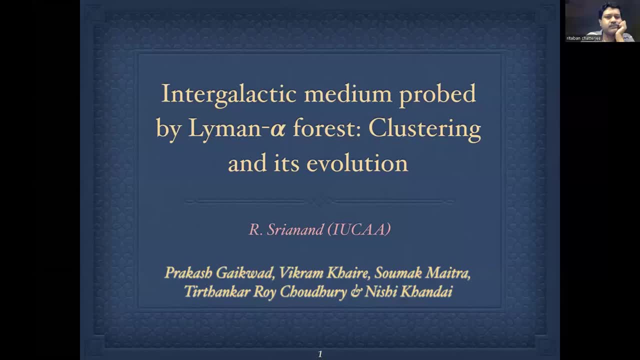 various information related to our cosmology or galaxy formation and evolution of the universe itself. This is the kind of program we have been carrying out for now nearly seven, eight years, And this resulted in three PhD works whose names are given here: Prakash Daikwad, Vikram Kaire and 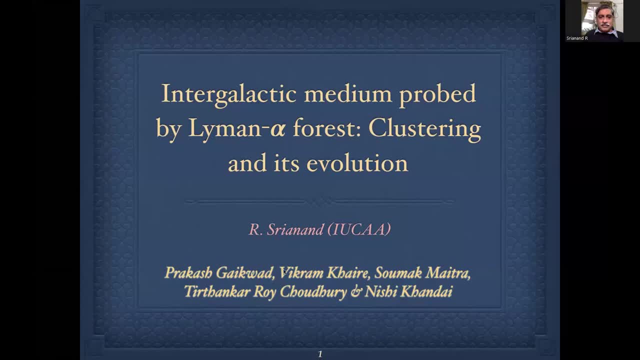 Somak, Maitra And basically these in collaboration with Tithankar Raichaudhri and Nishi Kandai. The basic idea: here I will just go through the basic idea behind using Lyman-alpha forest And, without going into the details, I will present various results and 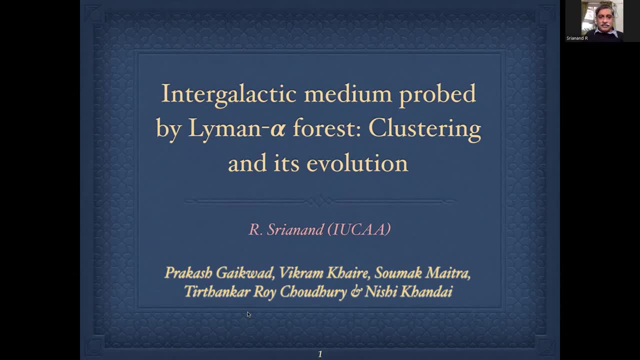 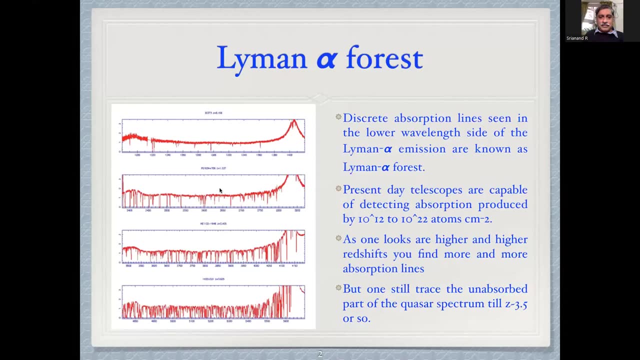 what are the implications. If any one of you wanted more detail, we can do it after the talk. Basically, if you look at Lyman-alpha, if you look at a distant quasar and if you take the spectrum, you will notice that there will be Lyman-alpha emission. And if you go to the wavelengths, 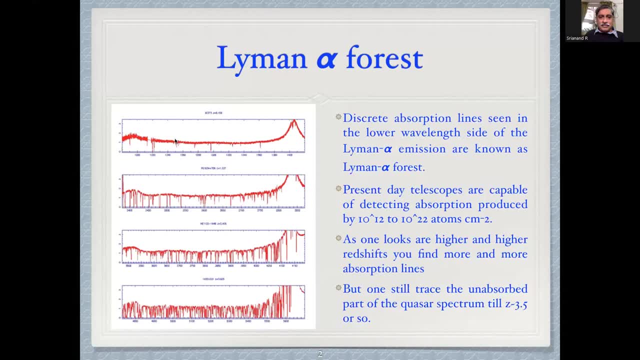 which are lower side of Lyman-alpha emission. you will start seeing large number of absorption lines And these are thought to be produced by the neutral hydrogen gas which is in the intergalactic space between us and the quasar. Okay, this is traditionally found in front of 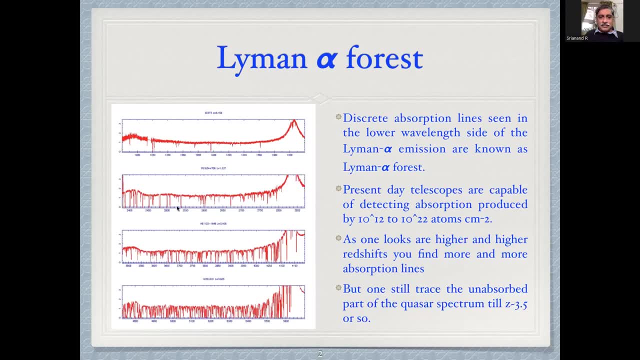 quasar. but you have to be aware that any object you observe which is at a distant universe will have an imprint of material which is present between us and the quasar, material which is present between us and that object, and in particular the all pervasive what? 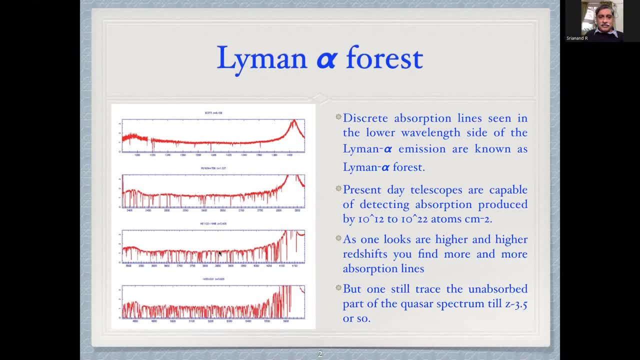 you call intergalactic medium. it is seen in the form of absorption and I have shown different spectra, quasars, at different redshifts. higher the redshift that means farther the object is from us, you find that the absorption strength is much, much stronger. basically, the summary is that discrete 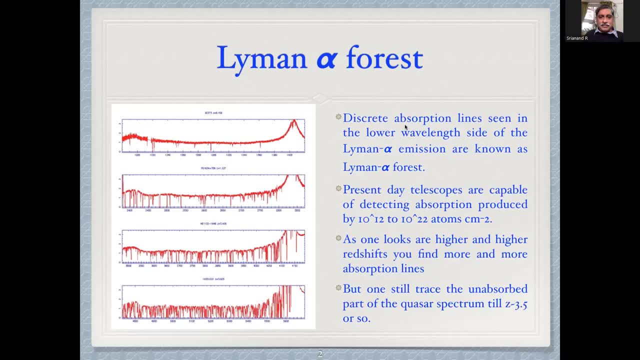 absorption lines you see in the spectrum of quasars. we call it as Lyman alpha forest because they look like a forest and it is mostly produced by neutral hydrogen gas which is present in between us typically. what kind of numbers one is talking about? if you look at the weakest absorption? 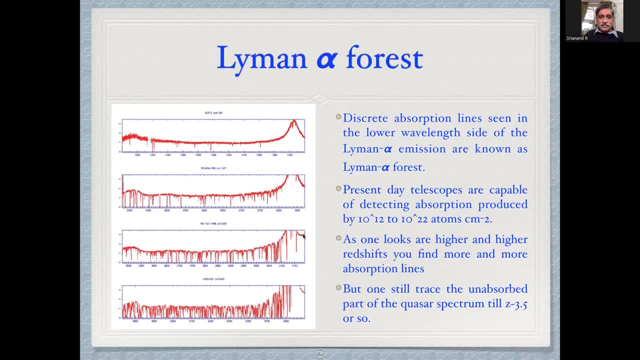 line one can detect in any spectrum, that will correspond to a column density of 10, to the minus 10, to the plus 12 centimeter minus 2, whereas the strongest absorption one can detect who are so called damp Lyman alpha. one can count up to 10 to the 22 atoms or hydrogen atoms per centimeter square. 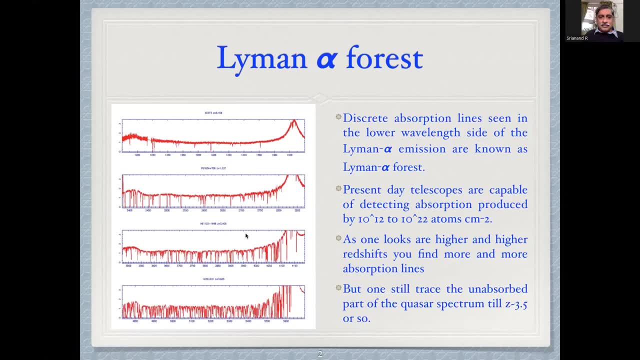 so it is one of the most powerful absorption lines that we have seen in the spectrum of quasars, one of the extremely powerful tools where the dynamic range of detecting gas column densities is 10 orders of magnitude. It is amazing. I think it is one of the things which we don't realize. 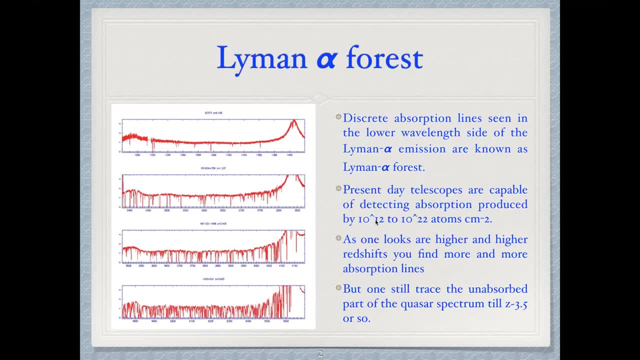 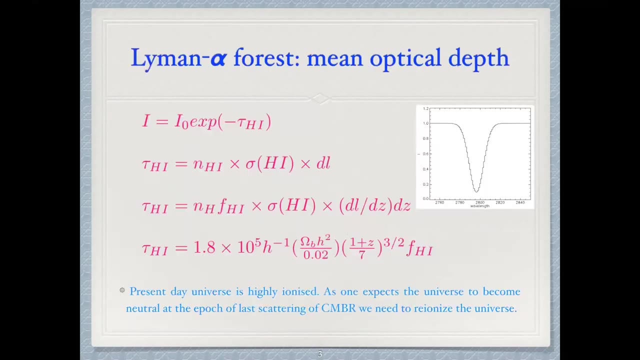 If you look at these kind of clouds, what is contributing to this kind of column density? you are talking about several orders of magnitude lower densities compared to the best vacuum you can think of in the laboratories. So what do we do? Let's do a very simple thing. 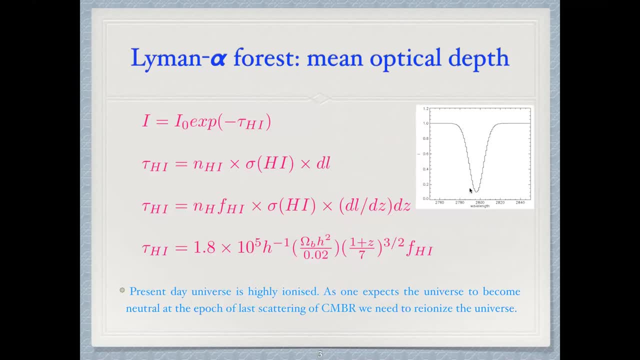 which we understood from our graduate school. If you find any absorption line, you can define some intensity at any wavelength lambda And usually you know that in the case you will write down as IE is unabsorbed intensity multiplied by some optical depth exponential of. 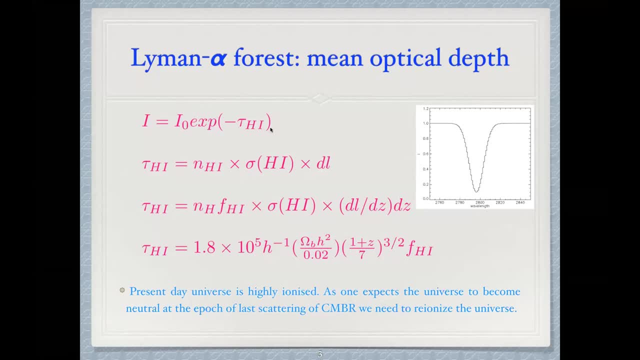 minus tau. It is very simple radiative transport equation. But what is tau? The optical depth is nothing but the density multiplied by the cross-section and the length over which you are integrating. right. This is the kind of thickness of the gas slab along your line of. 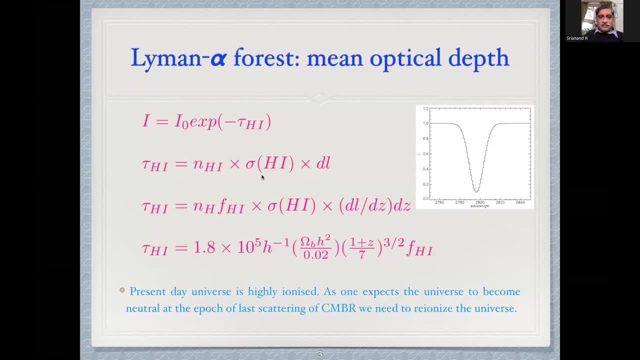 side Density, and this is basically the absorption cross-section. So what you can do is that you can think of neutral hydrogen density as total hydrogen density multiplied by some fraction of that hydrogen which remains neutral, multiplied by this. Here, what you can do is that, like a 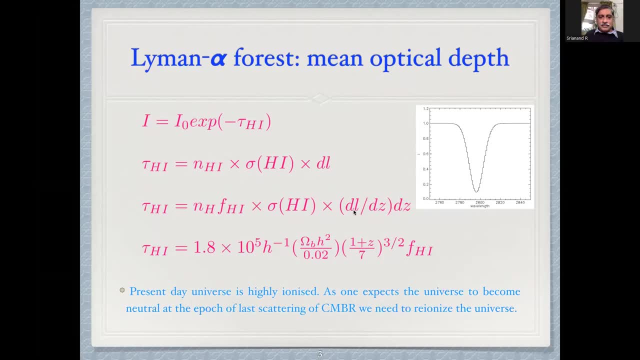 mathematician, you can multiply and divide by dz. dl by dz is coming from cosmology. It will tell you that if you give a path length of l along your line of side, what does it correspond to? the redshift difference in your observations? whatever, right. 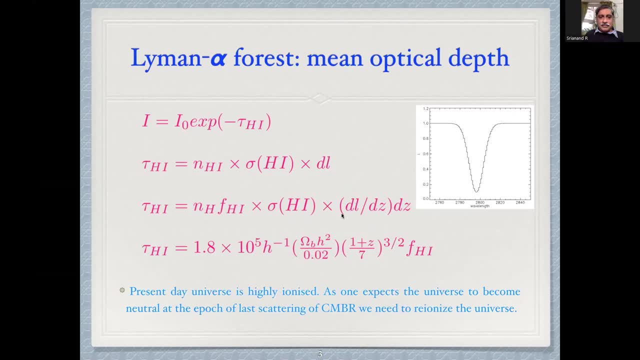 So if you plug in various numbers and take this dl by dz from your favourable cosmology- in this particular case I have taken lambda cdm- you can write down tau h1.. What is the optical depth of hydrogen you'd expect if you take all the baryons produced in the universe? 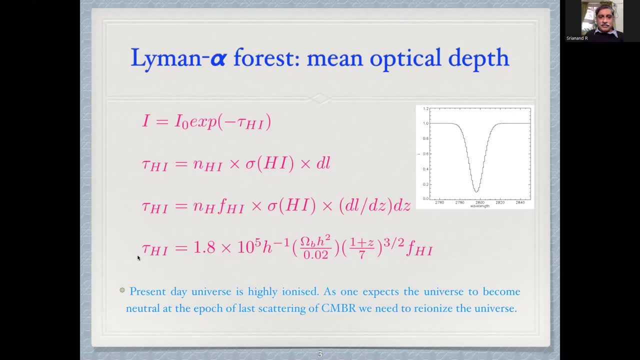 and uniformly distribute them between galaxies, and what you will get. This is the optical depth you'll get. It's amazing. For any typical optical depth, you're getting a value which is like 1.8 into 10 to the 5. if all the hydrogen atom remains neutral. This is the number of baryons focused. 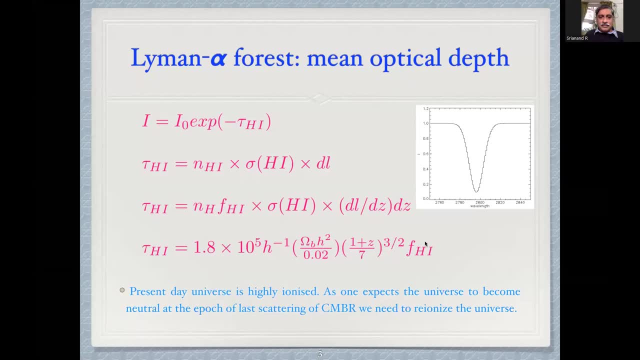 Now, how would you go back to this? Can you if change the size of the baryon? If, starting with this baryon, Can you counting by Baryon? Can you now select the height of the height of the remains neutral. This is one of the strongest probe of how neutral the intergalactic medium. 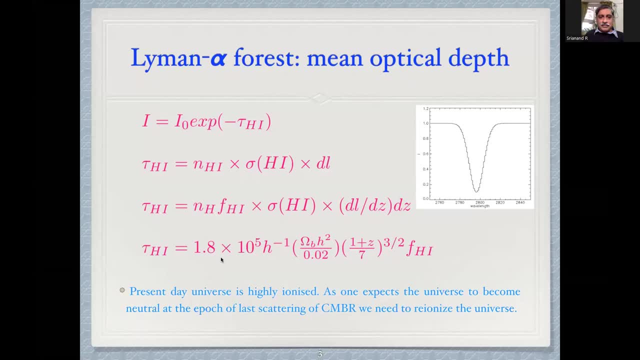 is, And you see that if you do not do anything, the optical depth is very high. This goes by the name Gunn-Peterson optical depth. What it implies is that whenever you look at a very high redshift object, you should not see any emission below its Lyman-alpha emission. 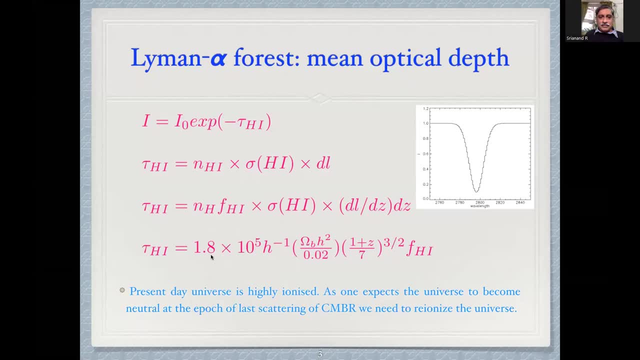 line, Because below that, if universe is neutral, you would not have seen any light coming, because e to the minus 10 to the 5 will be very small number, right, So nothing will come to you. So this is the basic idea, which tells you that the fact that we have seen absorption 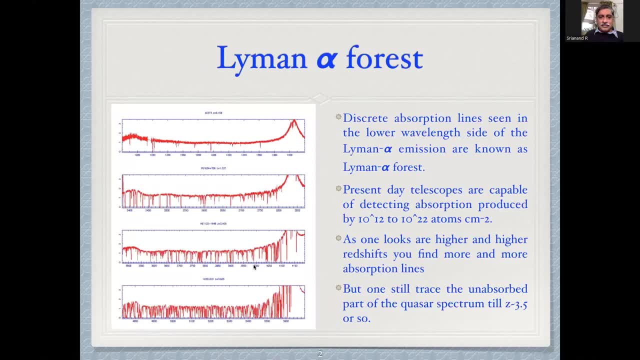 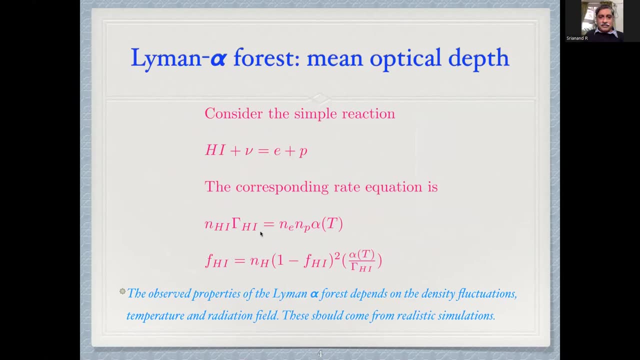 lines very much in this spectrum means that the universe is highly ionized. So this is what we started with. If you say that universe is ionized, you can also do one more trick. Then you will realize what drives what fraction of hydrogen will remain neutral. You can do. 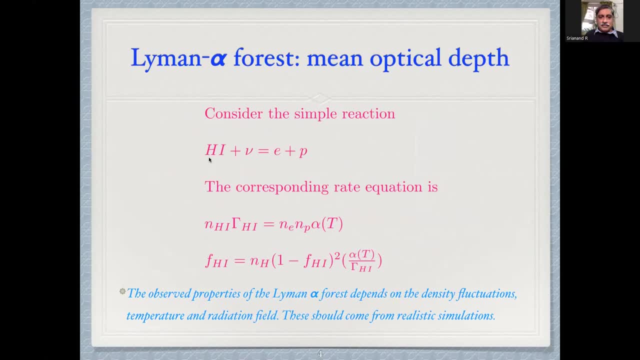 a simple photoionization equilibrium calculation. You take hydrogen. You have number density. You have photons interacting with hydrogen, It produces electrons and protons. You can write down a rate equation. This is the neutral rate equation. This is the rate equation. This is the rate equation. 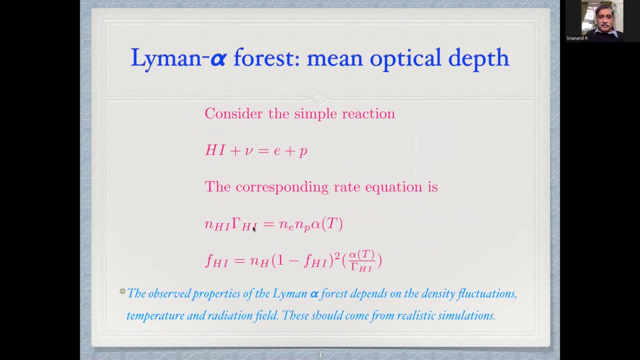 This is the neutral hydrogen density multiplied by the rate at which you are ionizing is equal to the rate at which you are recombining. So this is kind of ionization equilibrium. Now you do the same trick. You write down FH1 into NH And this will be 1 minus F times. 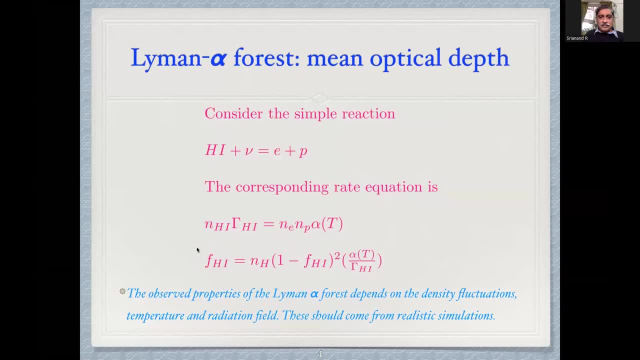 NH, So you can actually calculate. It's a very simple equation. you can think of FH1, what fraction of hydrogen which will remain neutral, And if you say that this is a small number, you can neglect: 1 minus FH1 squared, Then you see that fraction of hydrogen which 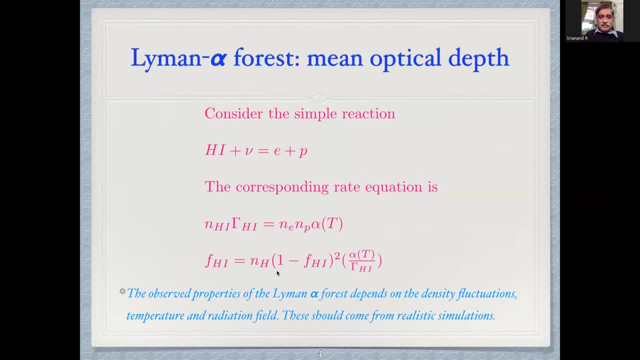 remains neutral, will be decided by what is the density of the region, what is the recombination coefficient which depends on the temperature. So density, temperature and the rate at which you are ionizing. So, basically, if you find an absorption line system and you can, in principle, probe these, 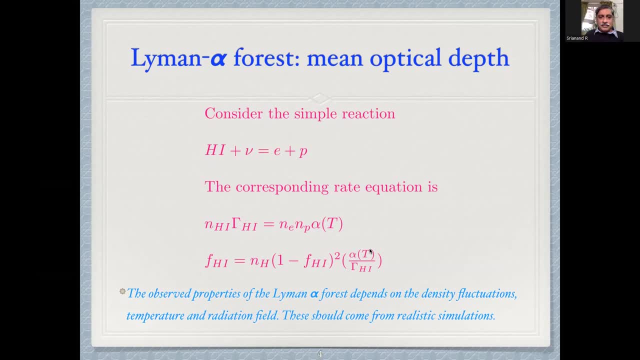 three quantities: density, whatever recombination coefficient, or temperature, or you can say photoionization rate. So this is what we are going to do, What we have done, what we have done, what I'm going to show here, is that we are going to use simulations, Basically. 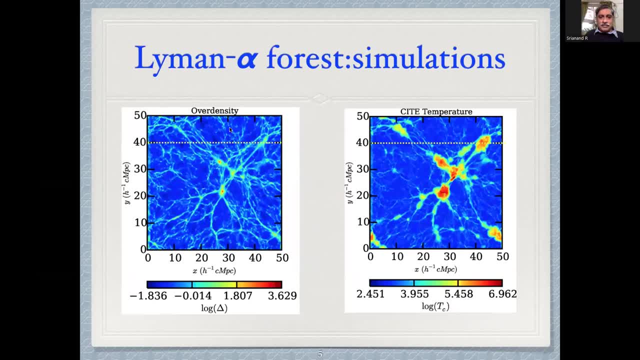 these are hydrodynamical simulations. We have a snapshot And you know that in typical cosmology, gas is not uniformly distributed. It is clamped in different regions And if you shoot a sightline through this, you can actually find out at each location what is the density of gas which. 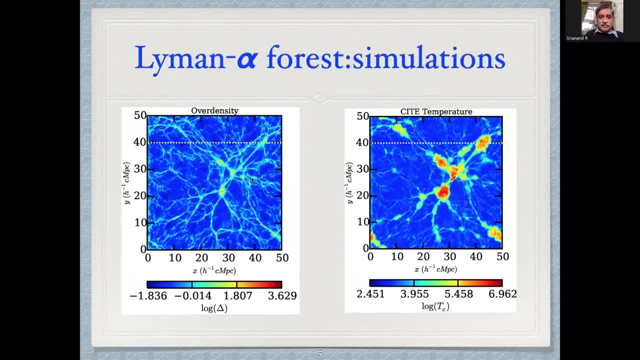 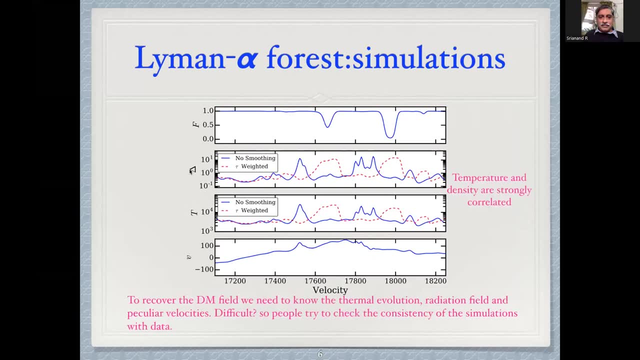 is present. Of course, this simulation will also give you what kind of temperature each gas particle is having, So you can actually construct something like a radial profile. This is what is done here. This is the density contrast, in the sense that density normalized to the local density. 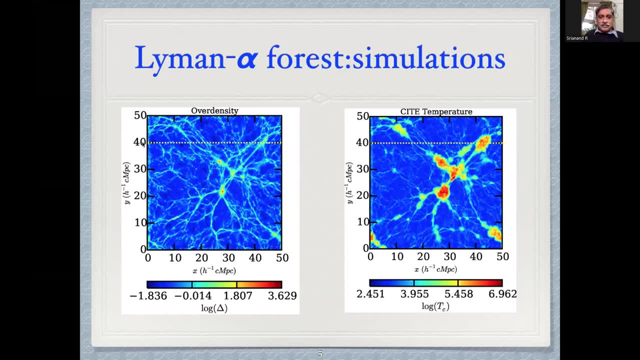 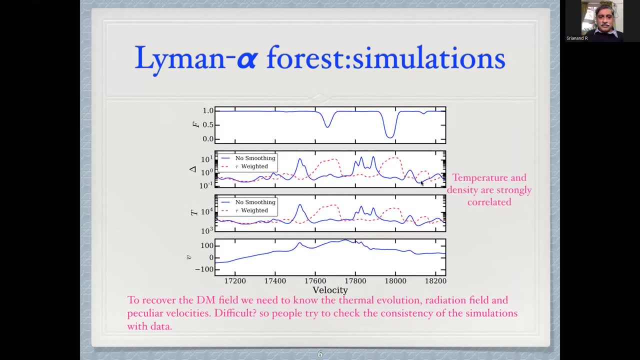 And you can see that this is kind of a line of sight which is exactly like this. You are going from here to here. What you will see is that density is going up and down with respect to some kind of mean value. This is the kind of temperature in these regions. 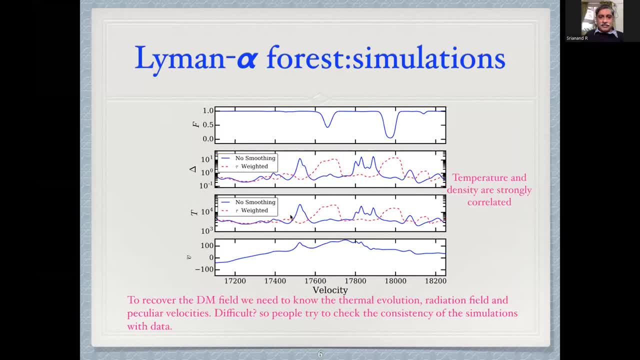 And you can see. one thing which is relevant from this simulation is that wherever there is high density, you also see high temperature. This is what is the thing which people call it as equation of state. And you can also see that these gas particles are not in rest because they are moving, because 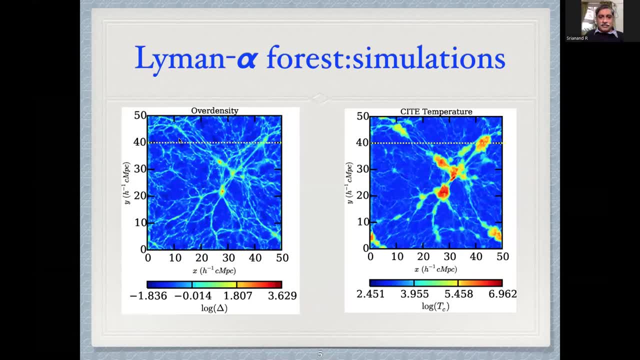 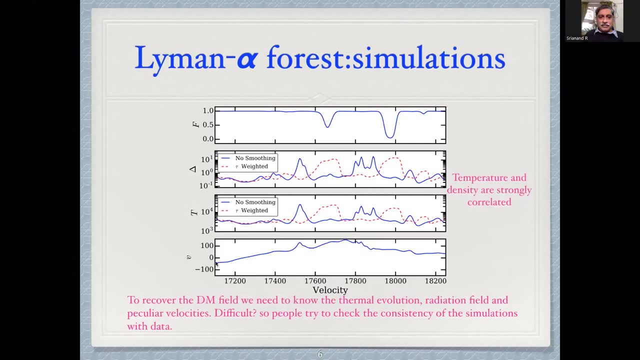 of the influence of gravity and expanding universe. There are two quantities which governs the motion of this particle. So you can also find out what is the velocity of the particle on top of this Hubble flow. You can just look at what kind of velocities they have In that. 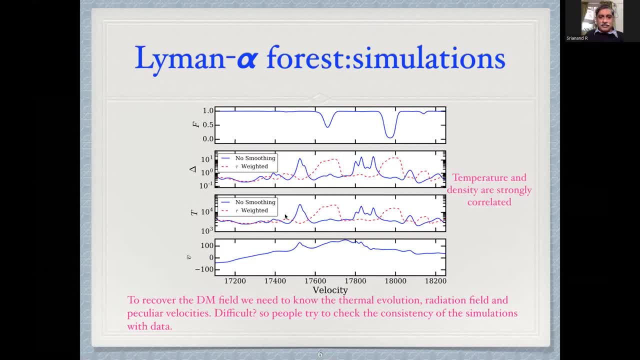 case you can take. what you have to do is that you take this particle. What is the temperature? You can calculate. what is the amount of neutral gas this particle will have and produce the absorption at this place. Then you look at what is the velocity. If the velocity is very high, you can calculate. 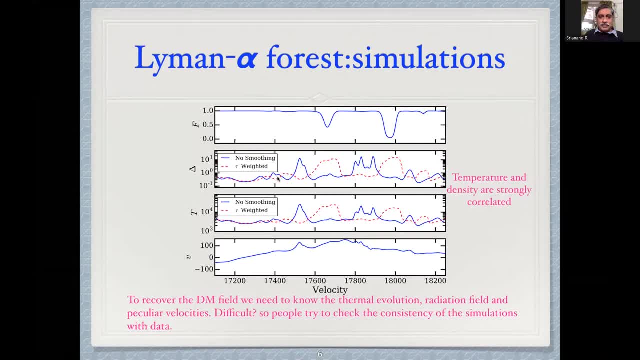 what is the amount of neutral gas this particle will have, And then you look at what is the plus or minus. you move the particle in the wavelength space because the Doppler shift and you will get the profile. this is what is done here. what is done here is that this is: 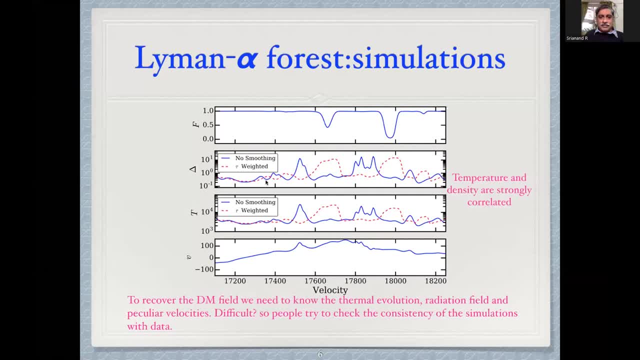 the absorption profile. you have to see if your line of sight is passing through a density field like this, a temperature field like this and velocity field like this. so what is interesting here is that, even though you find strong absorption, you would think that there is a strong 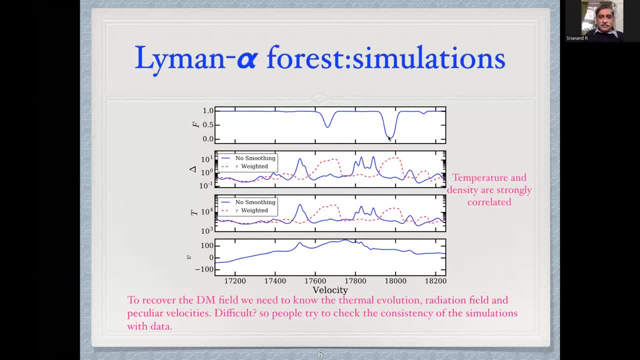 cloud which is sitting there, but in real space. if you convert that into a real space location, you will find that there is very low, not very high, density region is present there. so it's clear that the absorption you see is related to the density field, modulated by the local velocity. 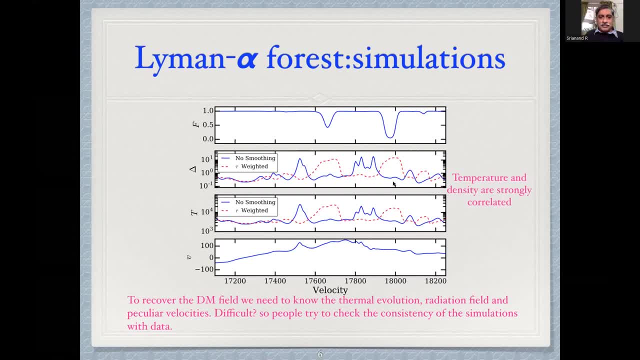 field. so it is a very difficult problem to do. the way one one addresses is that you do realistic simulation and produce the data exactly like the way you do in observations and do various statistics with the data. I'm not going to go into these details, but I can do it in the in the 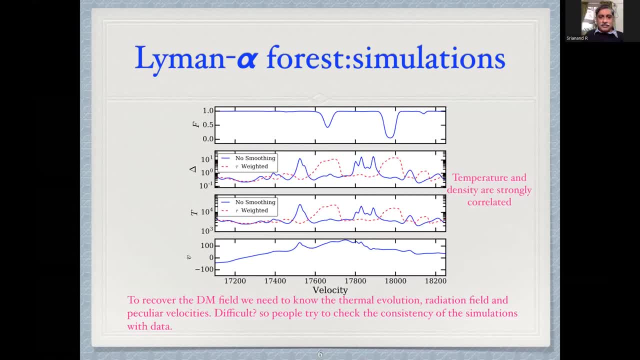 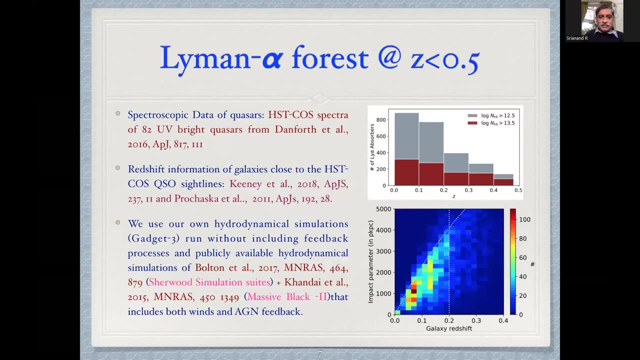 discussion session, then what you can do is that you can compare the model which reproduces all the observed properties and derive the parameters of the model as the possible parameters from the real universe itself. so this is what one does. I start with the lower redshift. I will focus on two issues here. one is that low redshift, which is 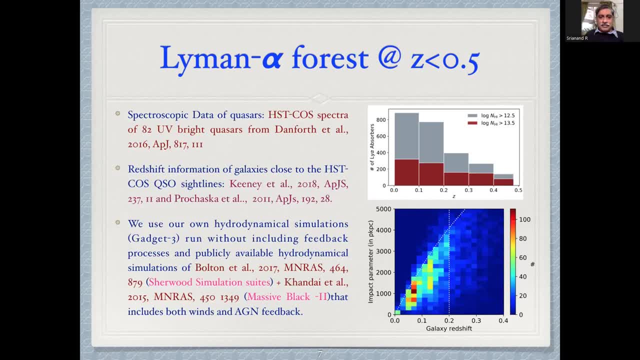 we mainly focus on redshift below 0.5, where the Lyman alpha line is actually in the uv. so you have to use Hubble space telescope and we have used archival data from Hubble space telescope which has been compiled by Dunforth et al and also you. 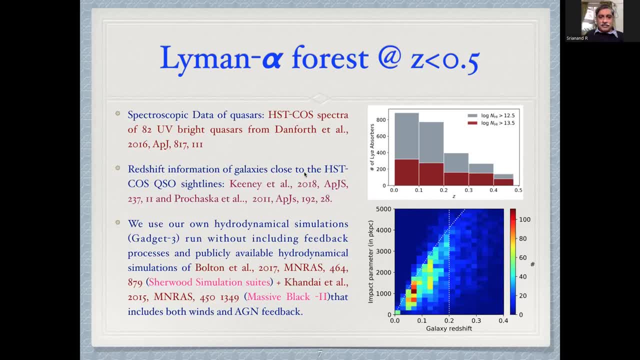 can see that in low redshift you along each quasar you can also locate where the galaxies are in the foreground. so you can map the distribution cosmic web in front of the quasar sight line and you will be able to measure whatever quantities you study in gas. 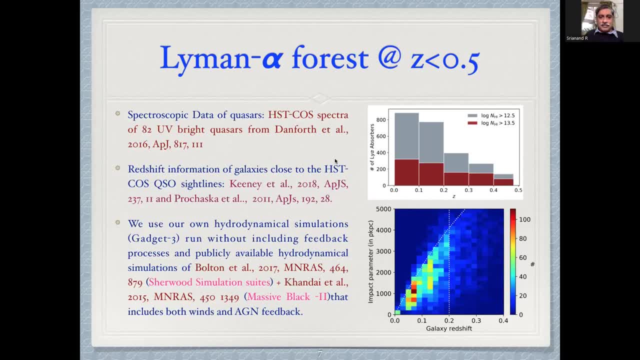 in absorption with respect to the galaxy density field itself. so this is the distribution of, basically, absorption regions which you are probing in the redshift space. here is the idea of what kind of galaxies which you are studying. basically, impact parameter means how far you can go. these galaxies are distributed with respect to the quasar sight line at different redshifts. okay, 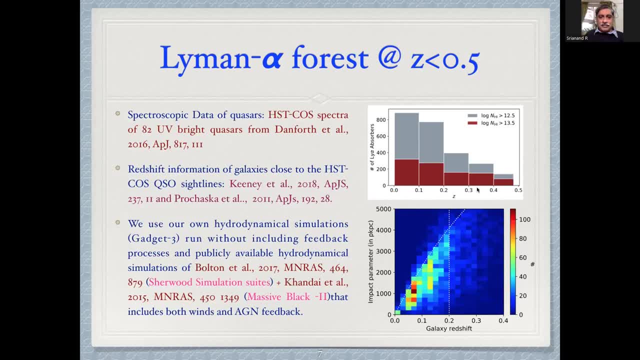 this is basically giving you the completeness of this. so what are the things we try to do? so at this redshift we run several simulations and we also borrow existing simulations in the literature and then try to construct the observable quantities and try to compare with them and try to find the best fit value. so there are three quantities which we study for the 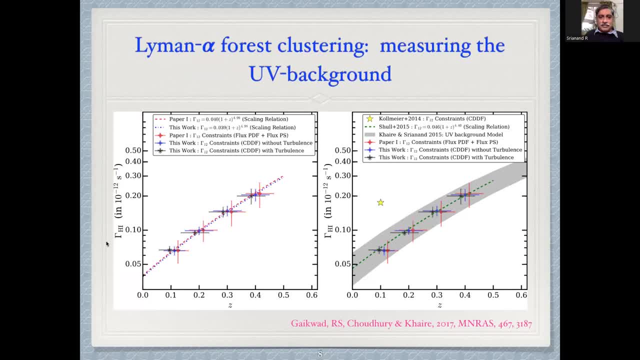 best fit. the first one I will focus on is what is known as the photoinitiation rate. so we try to measure the rate at which you can. you can ionize the hydrogen atom as a function of redshift and it is possible to do this and this is our measurement. it is done by krakash at a couple. 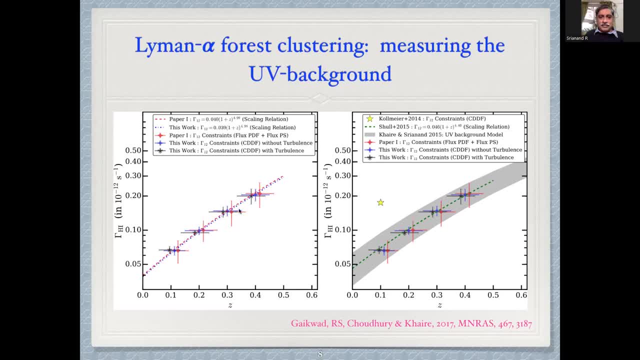 of years back and you can fit it with the evolution which goes as one plus z to the power five, roughly right. so it's clear that you, first of all, you can measure rate gamma h1 and you can also ask what is the rate at which the radiation field is evolving as a function of redshift, I think. 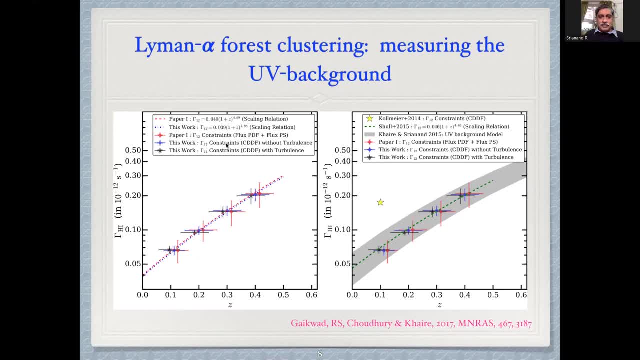 this is one of the the first measurements where one one quantifies this evolution in with higher precision. actually, what we can also do is that you can do a theory. you know that how many quasars are there, you know how many galaxies are there and you know how the gas are distributed in the universe. 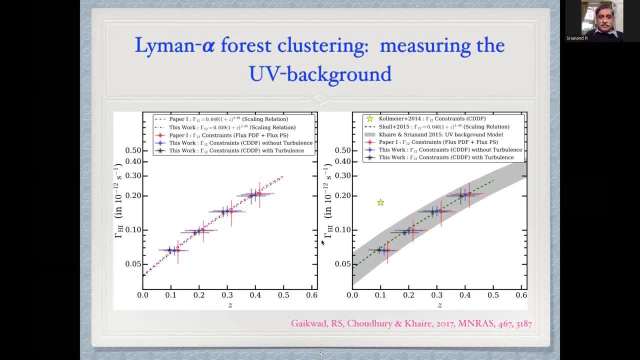 you can actually calculate what is expected from a standard cosmological model, lambda, cdm plus quasar distributions and galaxy distribution. this is the phd work done by Vikram Kaire and you can see that we predicted this in 2015.. this matches exactly on top of whatever one measures from the observations in 2017.. 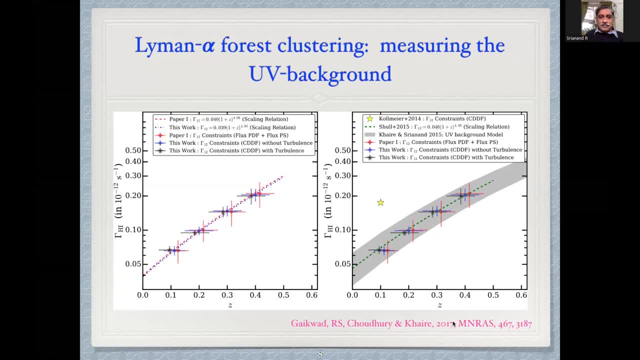 these measurements, as well as this model, has an important implication because before this work, there was a work done by Colmay et al in 2014. they measured this value somewhere here, which was factor six, more than what you can, what you can think for. so so they end up. 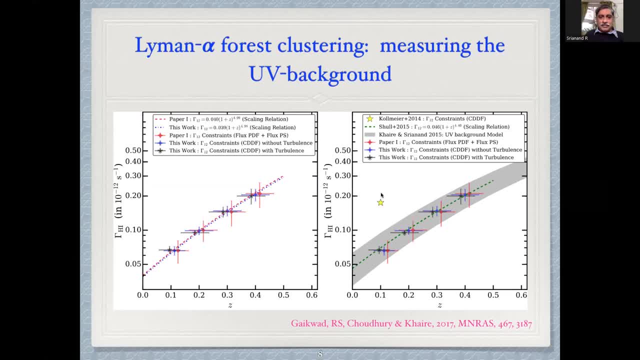 calling it as photon under protection crisis and they said that there is a big crisis in cosmology. I think we solve the crisis in cosmology because of two reasons. this work: when they did the background radiation on calculated they missed a considerable amount of quasars which are present, at least factor two to three, and we also see that to. 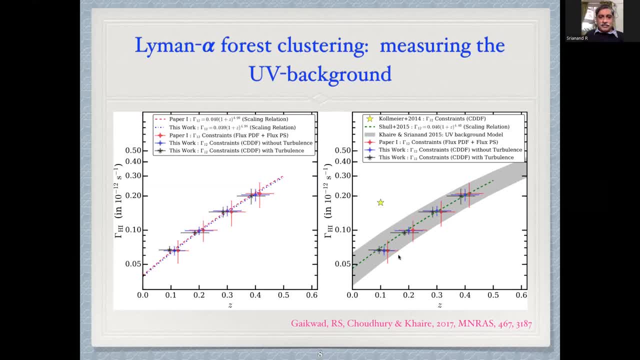 measure these from real observations, one has to do much more. constrained models spanning wide range of parameter space, which were which we were able to do with the precautions during precaution thesis with it. okay. so this is the first result. this is that measurement of uv radiation field and solution. 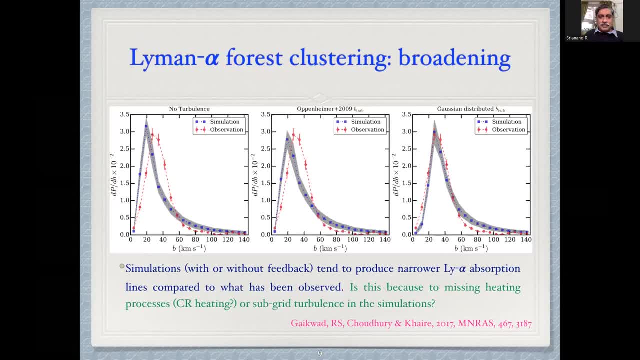 that is what we call as photon under production crisis. while doing this thing, we realized one of the problems with the simulations. even though we are confident about these measurements, the simulations have their own shortcomings. it is not that simulations produce everything properly. so these are the observed distribution of what is the width of these absorption lines produced. 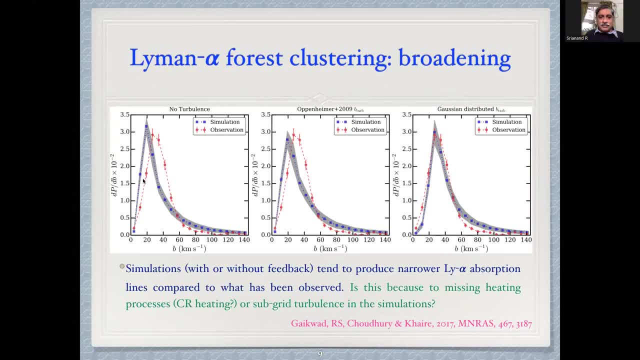 in the, in the real universe. so red points says what you measure in the real universe and the blue curves show what one gets in the simulation. so we find that the simulation tend to be more defined by the absorption lines, which are which are actually weaker, or we can say that we 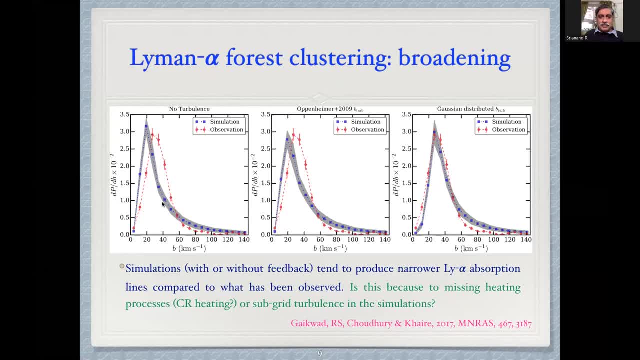 are narrower. so how to make the absorption line broader? you know that one of the things one can think of is to do Doppler broadening. you can say that you can heat the gas bit more so that the motion, random motions, will be increased and it is possible that, uh, uh, the you, you may have to. 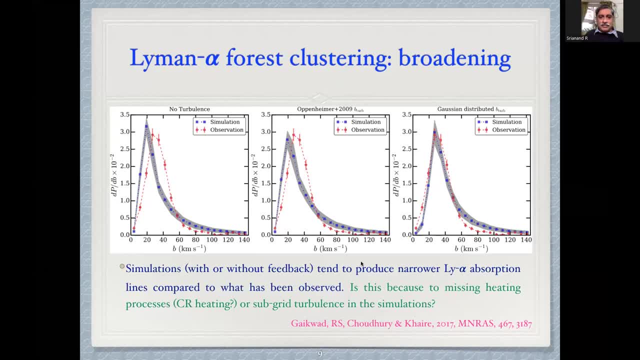 introduce we? we found out that whatever physical process one can think of which can be introduced by radiation field, heat the gas we can think of heating by cosmic rays or any other non-standard heating which could help. or we can say that our simulations are done in cosmological sitting with the 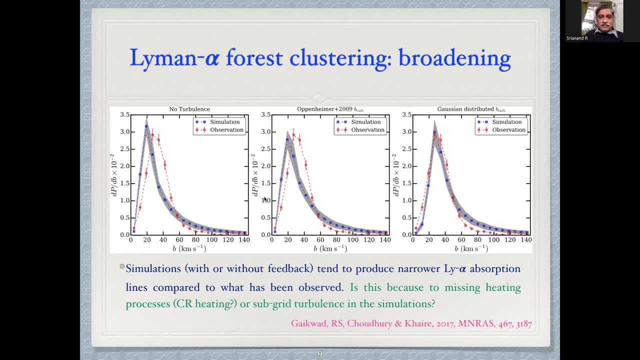 minimum dynamical range, so you may be missing some amount of microphysics. at the small scale, for example, our pixels will be about 50 kiloparsecs, because we are talking about several tens of megaparsecs, so it is quite possible that you are missing this turbulence. so we are unable. 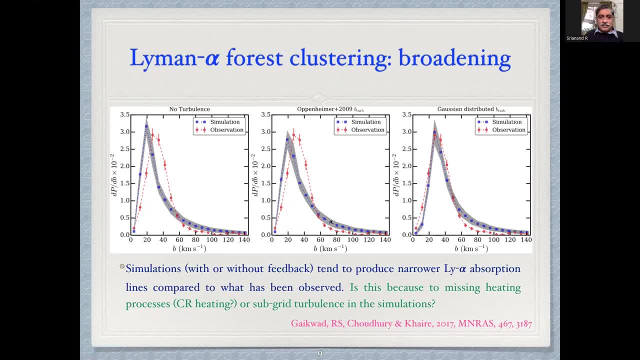 to address that at that time with the existing simulations. so now there are attempts being made to understand whether turbulence or this cosmic ray heating can be incorporated by different people in the field, not only us. so this is the issue. i want to brought out the third thing, which 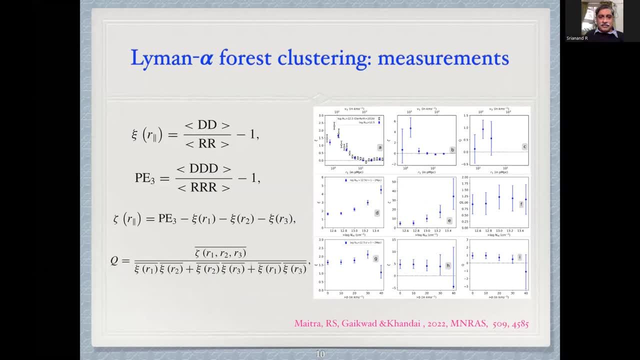 we did is that we asked the question like whether limon alpha forest is uniformly distributed or not. you see absorption lines. you can ask the question: if i go and find an absorption line, what is the probability that i will find one more absorption line within the separation of r? this is what we are doing here. you can count pairs of uh absorbers and you can. 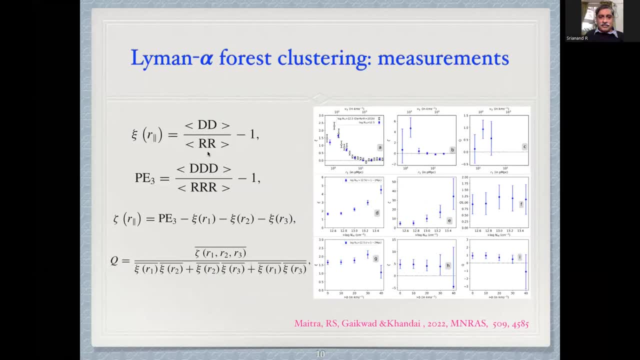 ask how many pairs are found with the separation r and how many you expect if the clouds are randomly distributed. and this is what is gone by this. this defines what is known as two point correlation function. similarly, you can define three point correlation function and reduce three point. 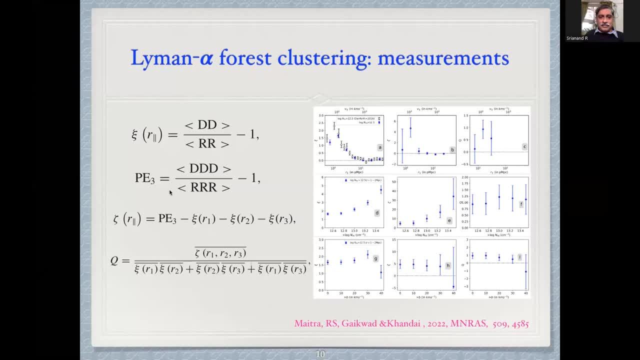 correlation function. so these definitions are extremely standard and one can actually do in. in our case, since we are doing one dimensional, we calculate these quantities along the line of sight. so let's target, uh, let's focus on this curve. what is plotted here is that the two point correlation 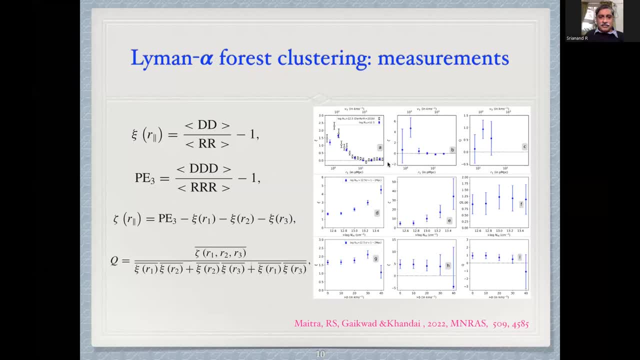 function as a function of separations, and we find that the limon alpha forest, which was in the when i was doing phd, people used to say that there was no clustering. definition of limon alpha forest is that absorption without clustering, without metals, but this has been now proven to be not the correct. 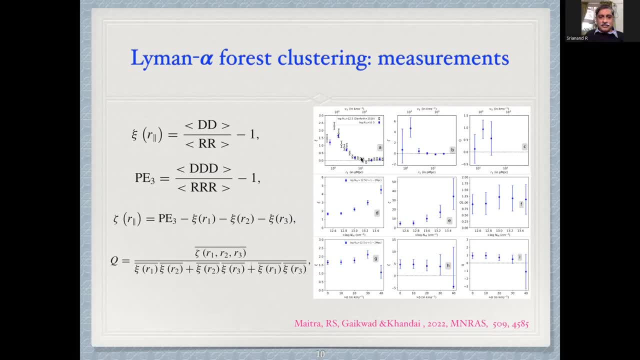 statement. so you can clearly see that we detect the two point correlation up to 10 megaparsecs rather than a mid-term scale, and we can also now define three point correlation. the idea is that if you sit in one, one particular location, you ask that what is the probability that you will find? 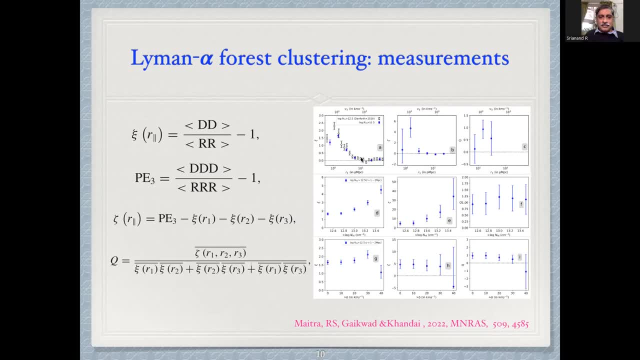 two absorber, one in the right, right direction at a separation r1, another in the left direction with a separation r2, and this you can. you can again do it like uh. basically you can, you can calculate what is the number triplets observed, a number of triplets predicted from uh, from the 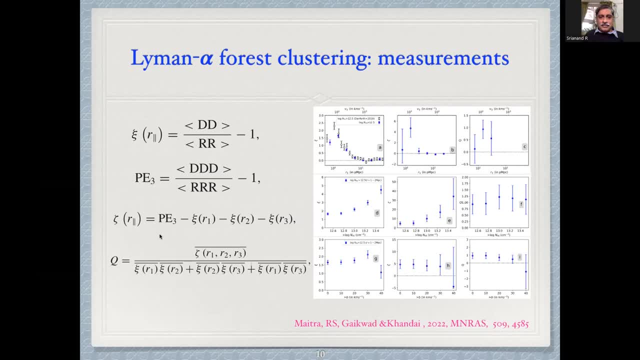 random distribution, then the actual three-point correlation function, when we determine the three-point correlation function, will be defined like: this is known as a probability excess for finding a triplet. then you have to make the correction for the fact that there could be doublet, which will be sort of: 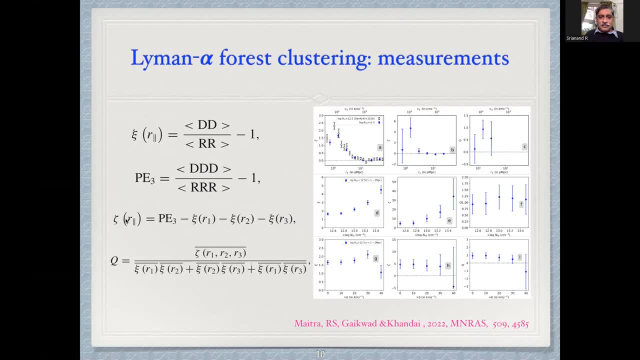 contaminating this triplet correlation. so we can- actually- this is the kind of thing given by p wills- so we follow the same thing which which has been used in the case of galaxies, we fall it for- follow the same thing for clouds. then one can define the dimensionless three-point correlation. 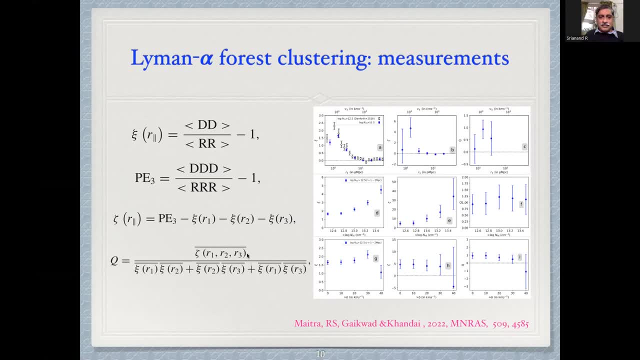 function as the, as a cyclic combination of the, the three-point correlation divided by the cyclic combination of two-point correlation. these are all standard definitions. what i wanted to tell you is that we actually measure the three-point correlation at the scale of about one megaparcel. 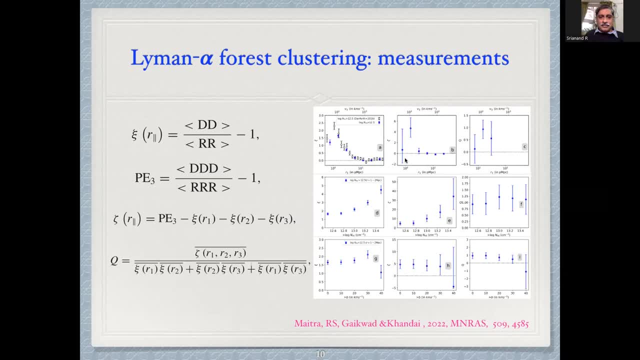 and this is the first ever measurement of three-point correlation of the liminal forest uh reported in the literature, i think. i think the first ever means that is first right. the second thing is that we can, we are, we can also obtain the value of q. again, first measurement. 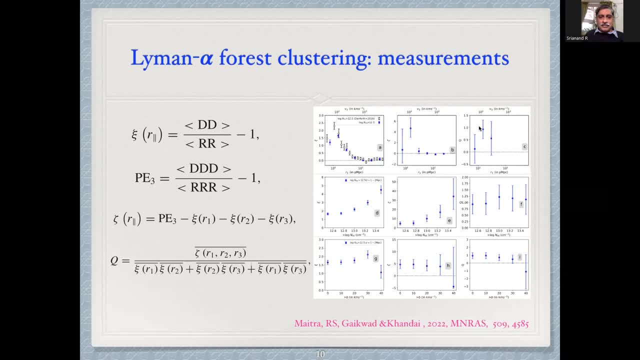 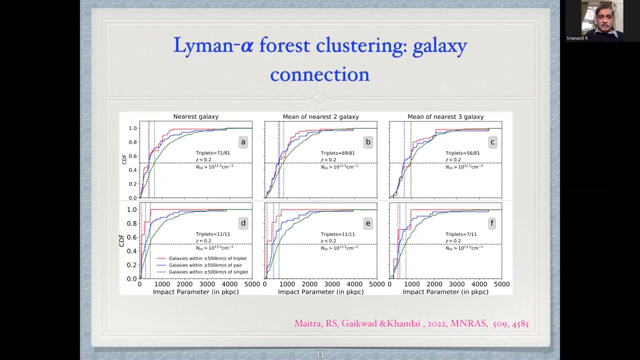 q measurements are slightly, uh, less statistically significant because q has also been used in the analysis of the three-point correlation function, so the three-point correlation function is well defined in this work. there are two main results we obtain, which i will highlight. one is that, uh, the, the the three-point correlation, the regions which we are finding. 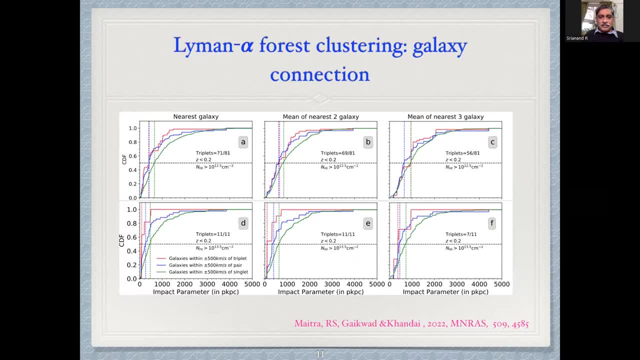 three-point correlations are tightly correlated with the galaxy distribution. we can see it in the following way: what? what is the histogram shown here? is that we can actually look at a liminal for forest. you group them into following, you say, the single absorption line, without any neighbor. 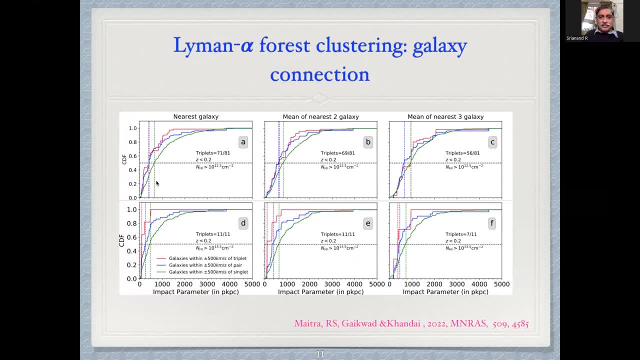 you can say doublets and triplets, right. you can look at the distribution of and then you look at where the galaxies are. since we know the galaxy distribution. what is the distribution of nearest galaxy with respect to triplet, with respect to doublet and with respect to a single absorption? 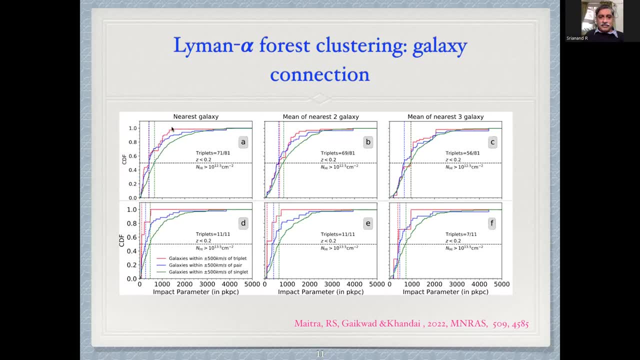 and the red is for the triplets, and you can see that the median value of red curve in all these curves are closer to zero compared to the green curve, which is coming from the isolated absorption absorption systems. this clearly demonstrates that when you are looking at the multiple 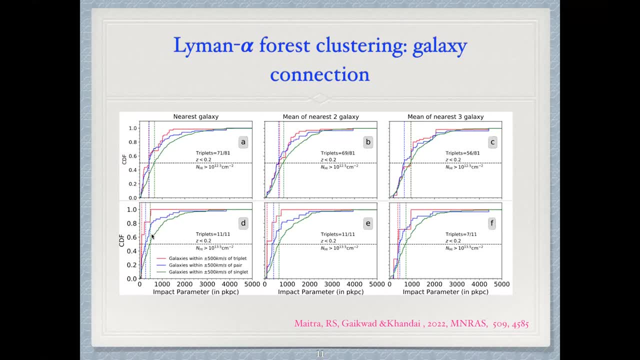 absorbers triplets what we are actually predicting. the three-point correlation is coming from the region which is tracing the filamentary structures in the liminal forest. again, this is this. i would say that it took a lot of effort, but this is the first confirmation of connecting what one see in 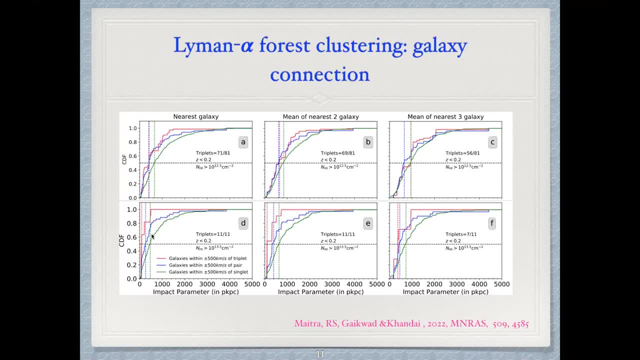 one-dimensional clustering into, into whatever you see in the three-dimensional structures. in the case of galaxy, it is possible for low redshift because we are dealing with uh, with uh hst spectrum, which gives you uv absorption lines, and we are dealing with deep uh galaxy surveys. okay, so this? 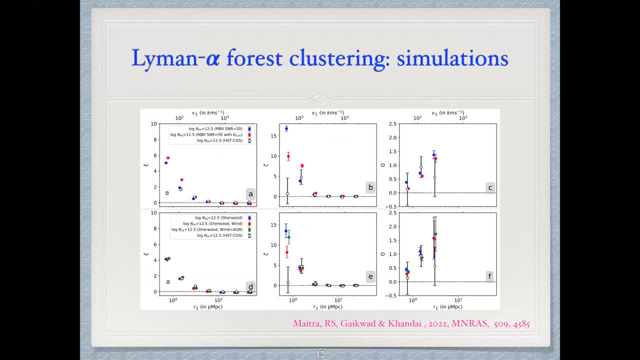 is for the lower shift and uh. so we can ask the question: can one make this clustering uh consistent in simulations as well? so this is the plot, where the open squares are for uh, for observations, and the red and blue ones are two simulations which we used. one thing which is evident is that both three and two point correlation, if you are at a larger 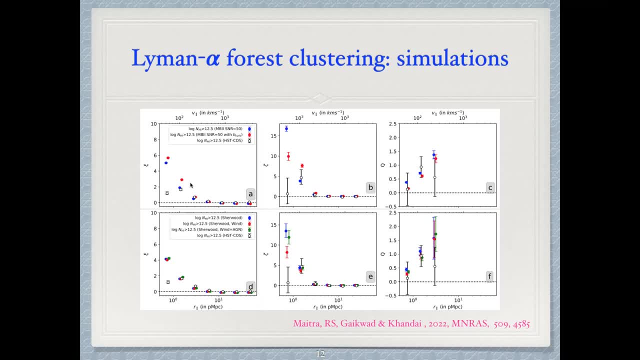 scale. if you are beyond one megaparsec, you will find that all all points coincide here as well as here. when you are at a smaller scale, we find that observations produce larger clustering compare. sorry, simulations produce larger clustering compared to observations. i think, if you remember, i was mentioning that there is a typical tendency in our simulation to produce absorption. 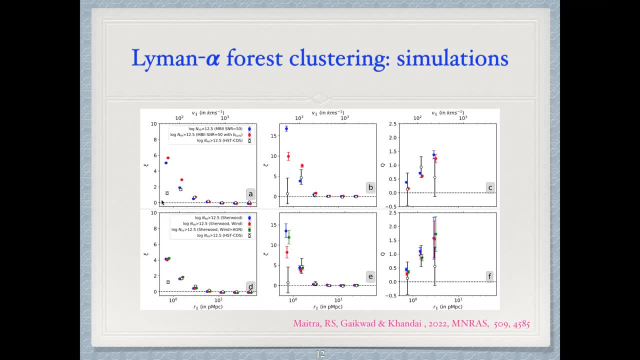 lines which are narrower. when there are two absorption lines which are narrower, it is easy for us to distinguish between them as a separate entity so that we can calculate the clustering them. if the absorption become broader, our ability to resolve two absorption becomes difficult because they become merging with each other. so you have five more minutes. yeah, i'm okay with that. yeah, 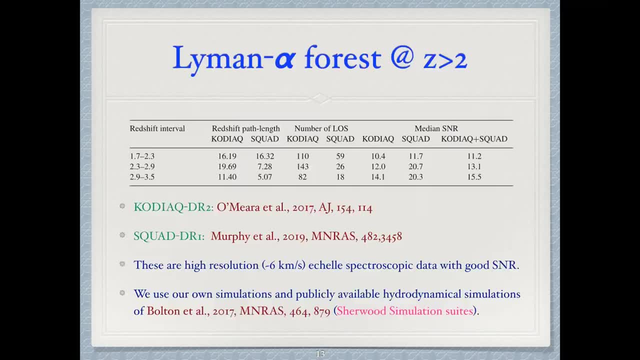 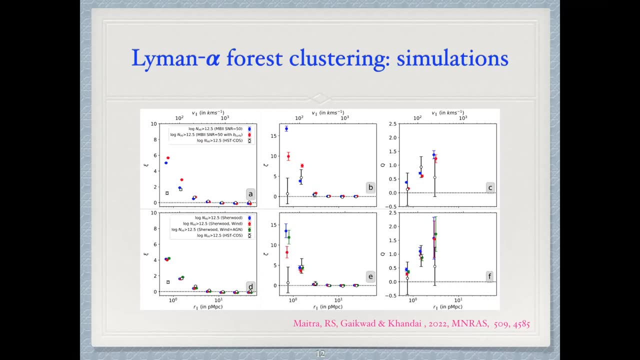 thanks, so so basically, this is another problem we we have to solve. so, in summary, in lower edge shift, what we have found is that we are first measurement. we reported for two point and three point correlation function connection to galaxies. there are issues with in the simulations when we 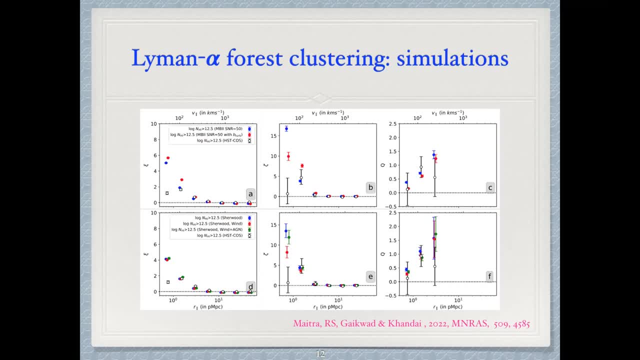 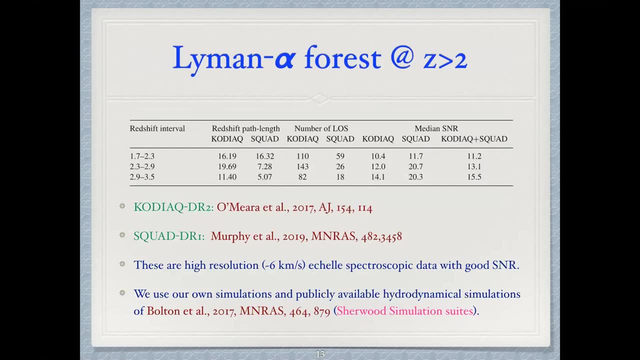 are dealing with small scale in terms of width of the lines as well as clustering properties. now we move uh to the higher redshift because in between you cannot do this. basically the observational problem: because of the our atmosphere we are, we are unable to measure the uv spectra from. 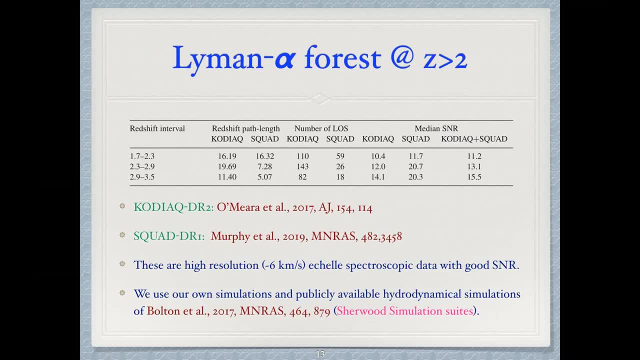 ground, but when it, when the redshift is about two, we will be able to do this exercise more correctly. so i will uh. this slide gives you what kind of data we are using, what kind of uh simulation one is using. this is the biggest sample of data compiled for high redshift quasars, as well as this: 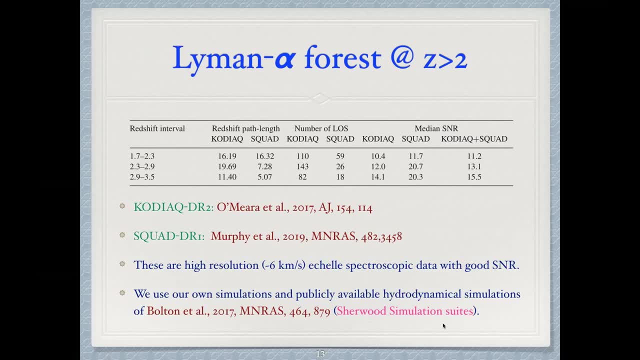 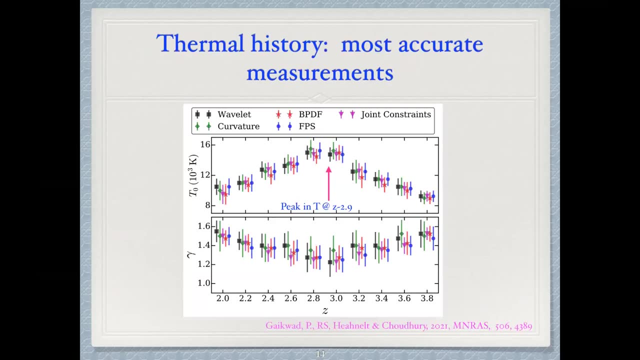 is the number of simulations from the literature, as well as our own for this work. so now let me go back to the same thing. the first thing we start with is the is the measurement of temperature of the intergalactic medium, because lower redshift temperature is not very useful. i didn't mention 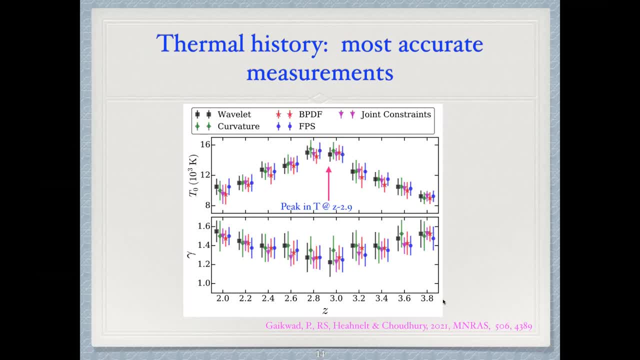 it in in great detail. in high ratio we can measure temperature. this is the measurement of temperature as the function of redshift and first thing we notice is that there is a peak around ratio 2.7. it is confirmed at a very high, significant level and this peak is expected if the universe is going. 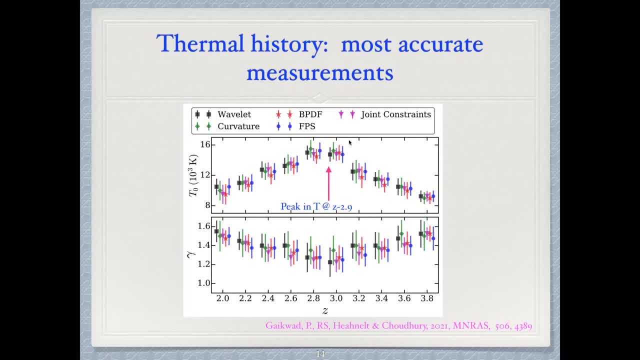 through helium to the initiation. so this one can think of as a proof of yet another proof of helium to re-initiation occurring around ratio 2.9. but not only proof. we can constrain it much better. i'll go into the details. so people measure gamma h1 like we have done in low redshift and for gamma. 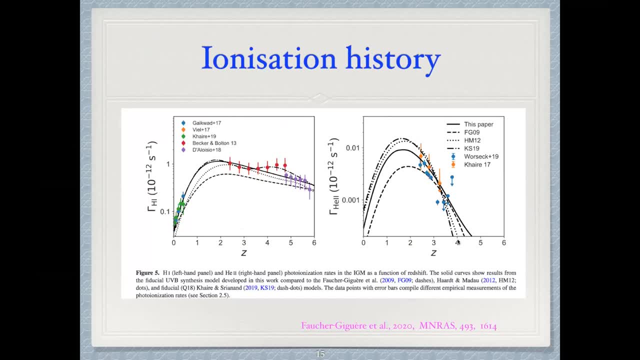 helium to a higher redshift, and several models are proposed, including ours, which goes through these points, so that we have a consistent model of background radiation which will give you hydrogen as well as helium. if you have done only this much of work, but when you now look at what is needed- and in fact you want to do this- we have to tweak a bit. 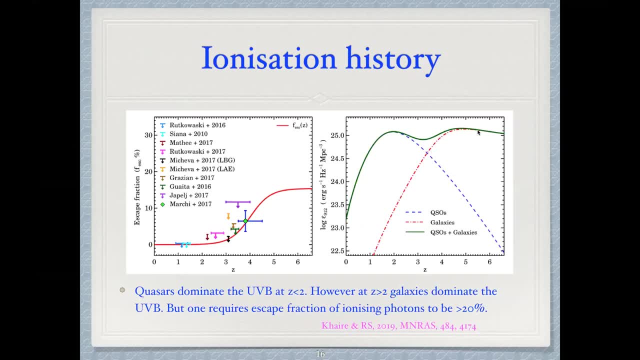 we have to say the following: you have to say that at high redshift usually the radiation field is dominated by galaxies and low redshift radiation is dominated by quasar, with a condition saying that suddenly, at high redshift the galaxy should have large escape fraction of uv ionizing photon. 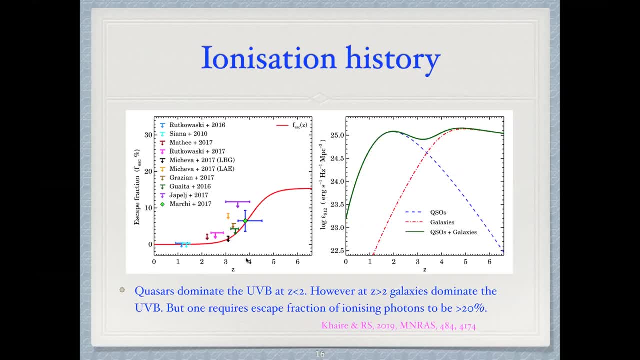 we know that in low redshift, most of the uv photons don't escape galaxies. this is another challenges, one phase, and this is basically being highlighted by several people in the in the literature. okay, so now let's come back to this. you have this measurement of temperature and you 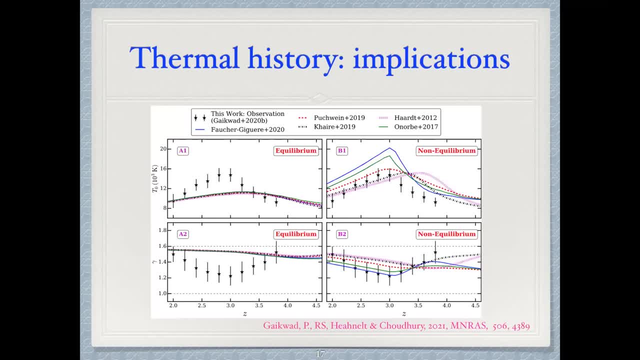 have this radiation field. you think you have already constrained very well. and what do you make? so you put this thing and find out what is the predictions. and these are the predictions. if you don't do anything, you follow the standard procedure. uh, everybody adopts in the simulation. 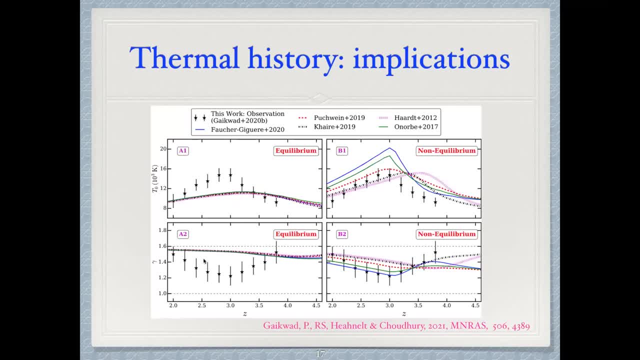 so you find that basically the temperature profiles are not as predicted by the models. observations produce much sharper rise in the temperatures. however one can. one can make them by saying that, okay, absorb in the simulation, assume equilibrium, ionization and heating. you actually evolve the temperature and then see what happens. then you see that actually the 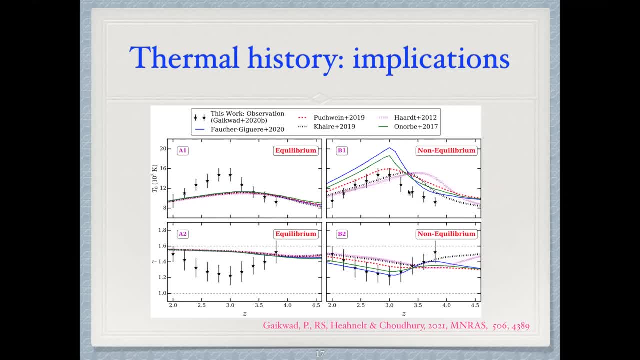 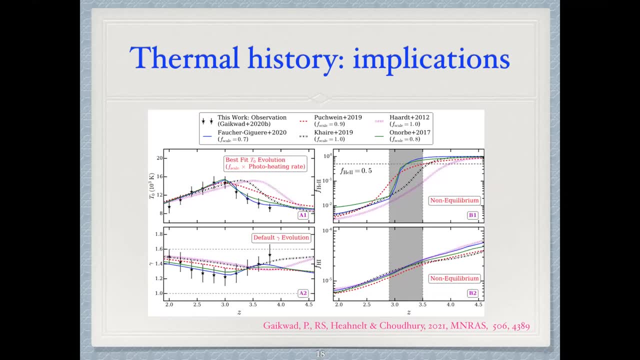 range in temperature is increased, but still these curves are not sitting on top of the observational data. so we are. we can pick one more thing saying that: okay, you are making some mistake in the. in the calculations you say that your efficiency of heating the igm as from the standard textbook. 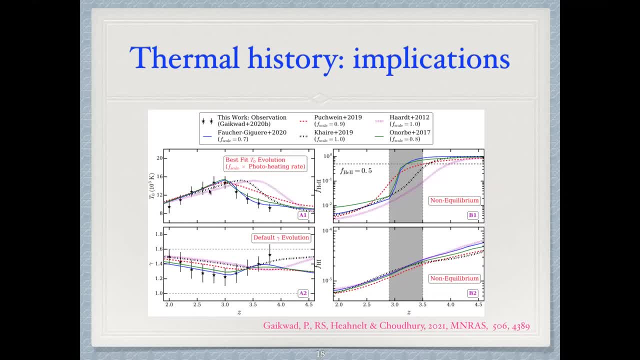 is not valid, you reduce it by a factor, scale factor. then you are able to fix it. so couple of points. we measure the temperature. it challenges the existing standard models of uh evolution. in the simulations we have to introduce two quantities. one is the non-equilibrium evolution of 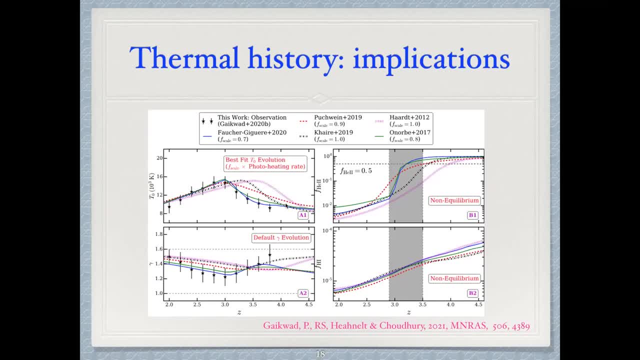 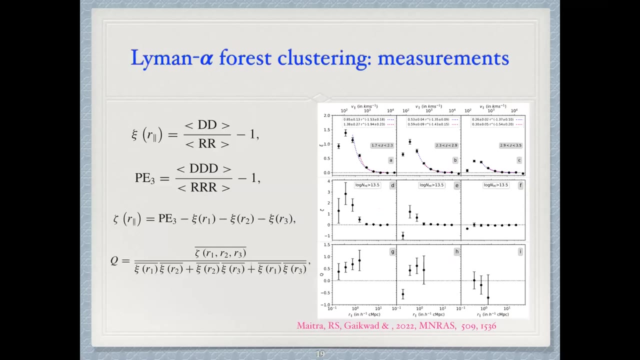 the heating and radiation ionizing field. in addition to that, you have to also say that when you are doing heating, you are not efficiently heating. somehow you have to manipulate the heating efficiency. so this is very important result and it puts interesting constraints on the helium population. helium uh area initiation. i have a couple of slides. 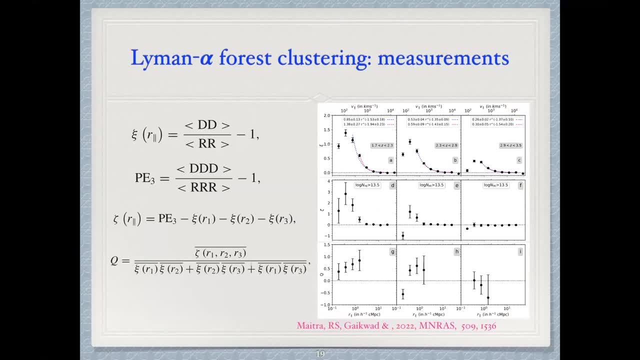 where i want to want to say that the same thing which we did in the low redshift clustering, we also managed to measure the high redshift clustering. i must say that this is again, once again, very important contribution to the field. nobody else has done this before. i have to reiterate. 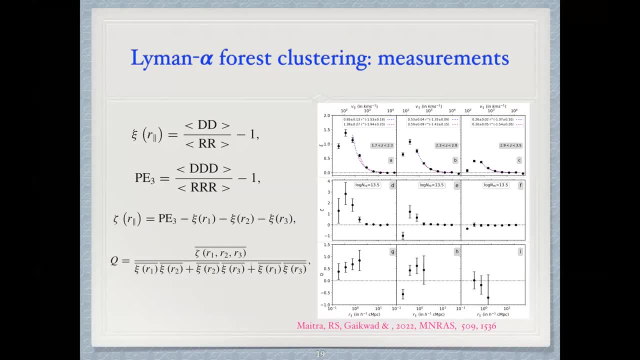 because these are phd works. so it took two, three years to do it, but it was very important. contribution done by somak mitra. so here is the two-point correlation measured at different redship. with your eye, you can clearly see that there is a strong evolution in the clustering of two-point. 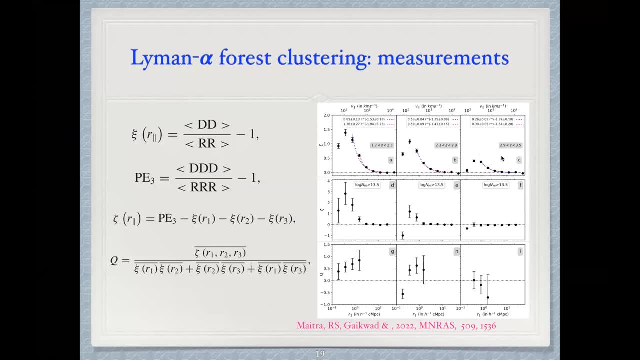 correlation function. as you go to higher and higher redshift, the clustering goes down. this is the three-point correlation function and again, this is the first measurement of three-point correlation function at these redships. again you see that this is decreasing as a function of redshift and this 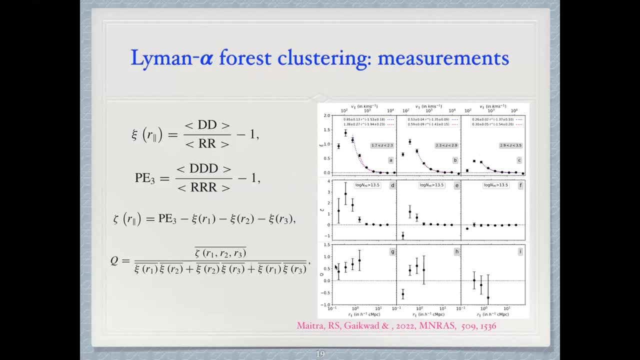 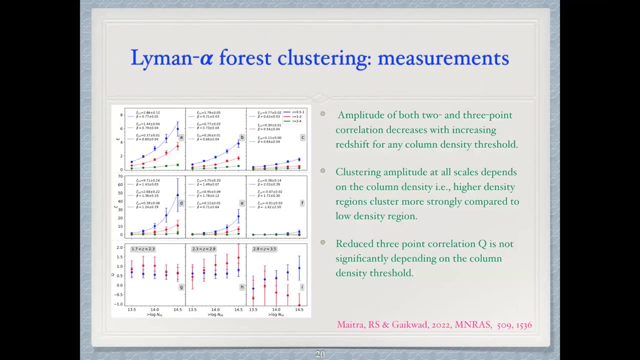 is the measurement of q, and its q of 0.6 is amazingly consistent at all redship. we have to understand: why do you get q of 0.6? okay? so now you can ask the question like: uh, what kind of things one can think of? it seems that if you can now higher it, should you have much more data. we 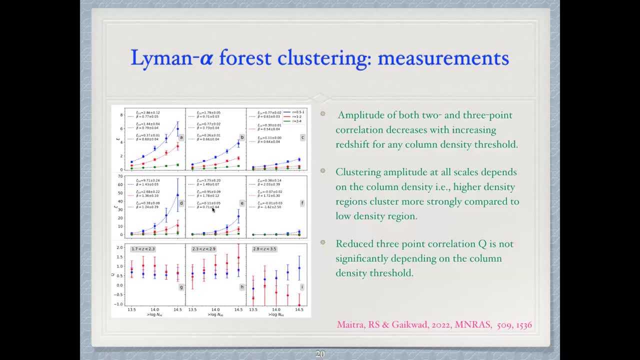 can split them into lots of things, right. so this is the part like yellow and white, we can structure a few of these very well-done measurements down from the clustering of two-point correlation, and you can see this one shows that the amount of radiation has increased, and so it takes about. 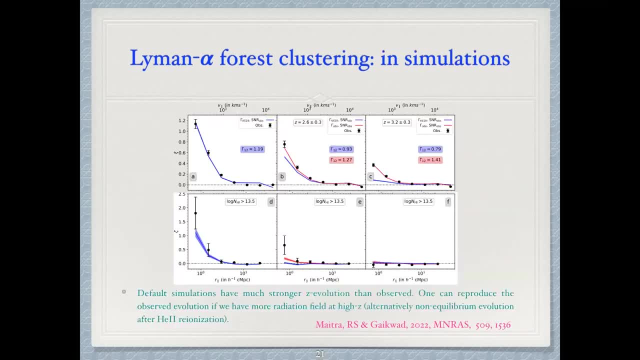 seven hours to get the overall resolution back to the normal right and we can see that, that this is the x-ray which we can use to calculate the extent of the reverberation of this surface right. so we can stop at x-ray and this is the area where the red circle that we are starting. 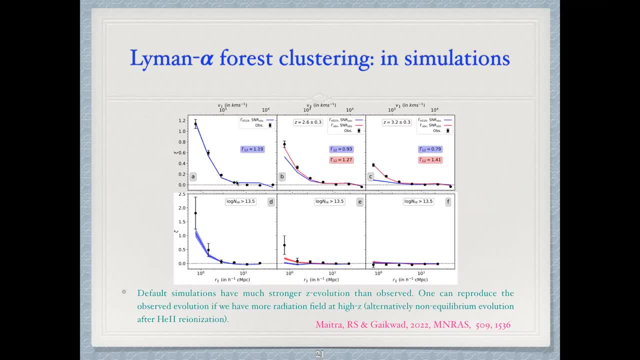 to see the effects of redshift, and here you can see the strain of the redshift and we can start to see the result at x-ray two. when you go to higher redshift, the clusterings are completely under predicted by these models. So if you really wanted to fit these blue curves, if you really want to fit these black, 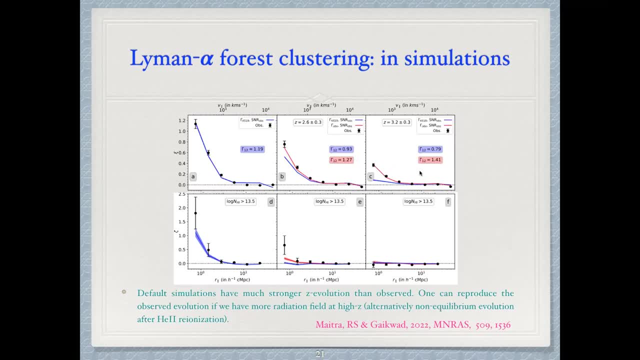 points. what we have to do is that we have to enhance the radiation field, one of the methods. Time is up, It is done last. I am have only one slide left here, Okay, So so basically, then, this curve- actually, I can put this curve on top of this. data points. 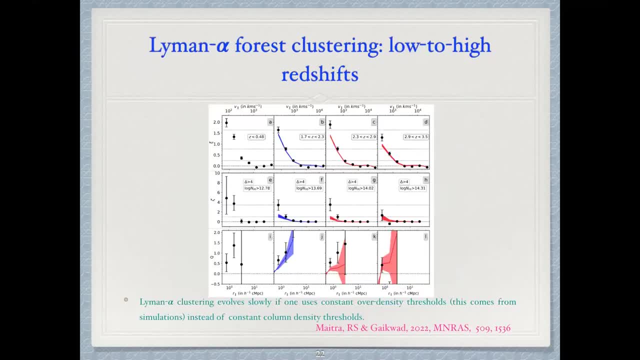 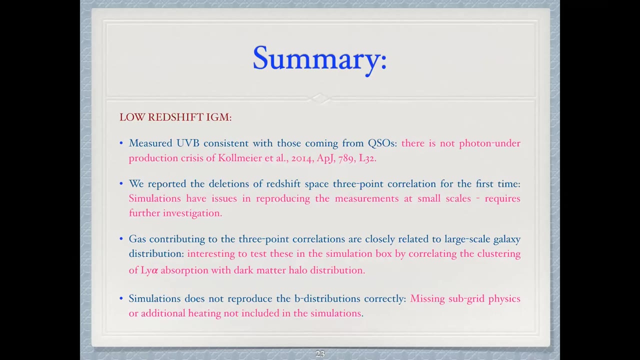 by changing the radiation field. So the bottom line I wanted to okay, the same thing is explained here. I will go to the conclusions summary, because this is exactly the same curve. we put it together from lower redshift. So I just summarized in two slides: lower redshift, IGM. what do you, what do we understood from? 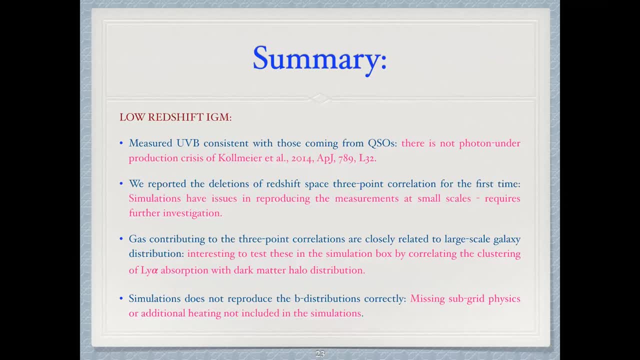 this exercise. The measured UV background is consistent with quasar. there is no photon under production crisis. A reported detection of three-point correlation. we report the three-point correlation function for the first times. Simulation has some issues at small scale which has to be sorted out. 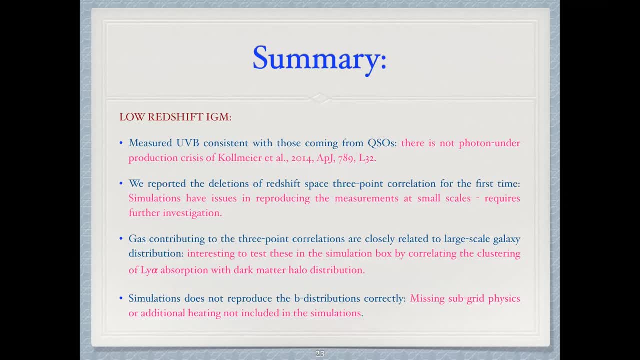 Gas contribution to the gas contributing to three-point correlation are coming from large scale Galaxy distributions, so they can be very good probe of how filamentary structure evolve as a function of redshift. This is one thing we are we are yet to embark on. 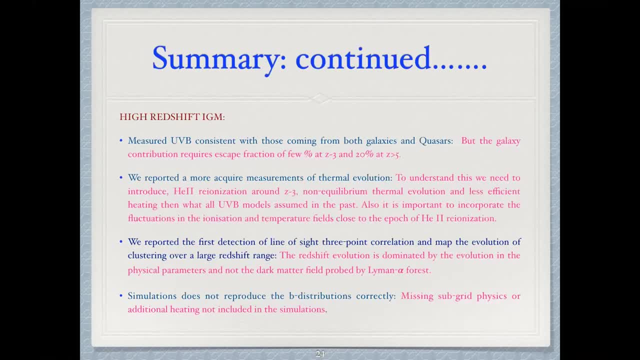 Simulation. do not produce B distribution as well as small-scale clustering When you go to higher redshift. this is my last slide. we measure UVB consistent with those coming from both quasars and galaxies. But you have to see there are some tweaks we have to do, as I explained later on. 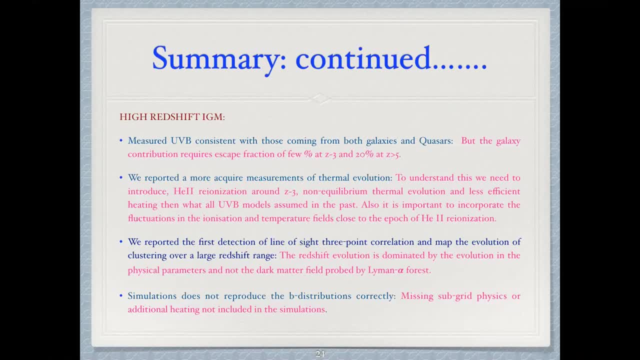 First time we have a very accurate measurement of thermal evolution of the IGM, which contains the rapid evolution of helium II, reionization at redshift III, which requires non-equilibrium as well as some puking in the efficiency, and we report first detection of line upside three-point: 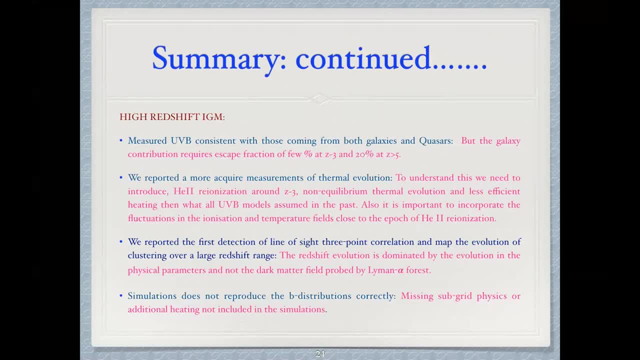 and two-point correlation functions and we are already saying that we may have constraints further, stronger constraints on the radiation field coming from these clustering measurements. So, okay, I think last part I don't want to go into. I think that's. that's not correct, Okay. 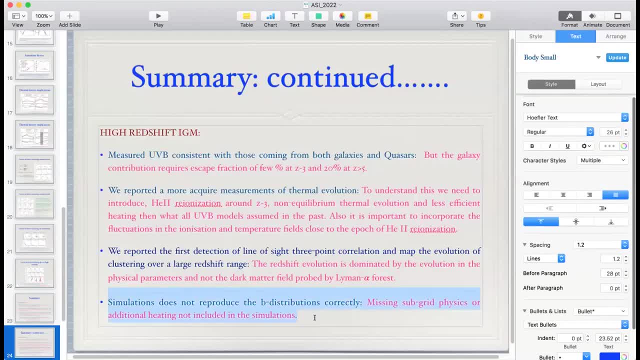 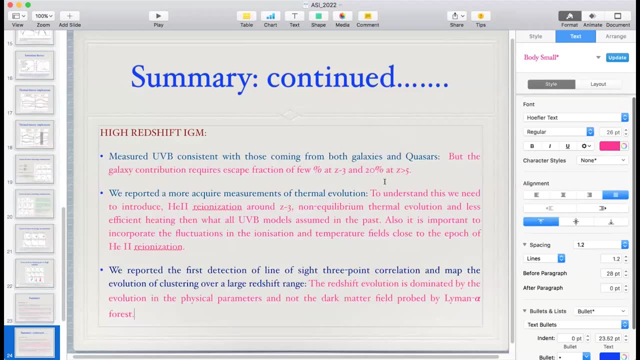 Let me stop, Okay, thank you. So I think we have time for a couple of questions. So is there any question in the chat box? I don't see any question. is there any question offline? Okay, Okay, I do see questions now. 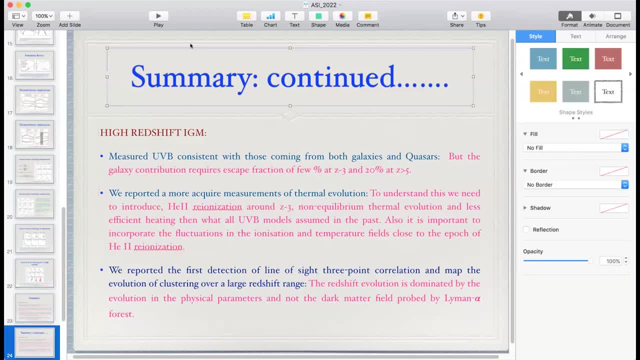 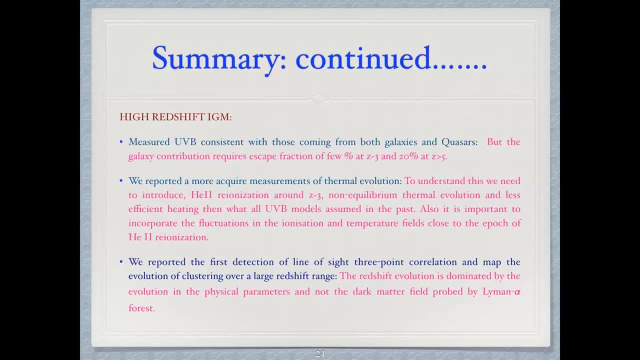 So should you turn a chatter? G has a question. Yes, please unmute yourself and ask: Can you unmute? Yes, I could unmute now, Okay. Okay, And I'm just a clarification. If you go to clustering, there's a couple of slides. 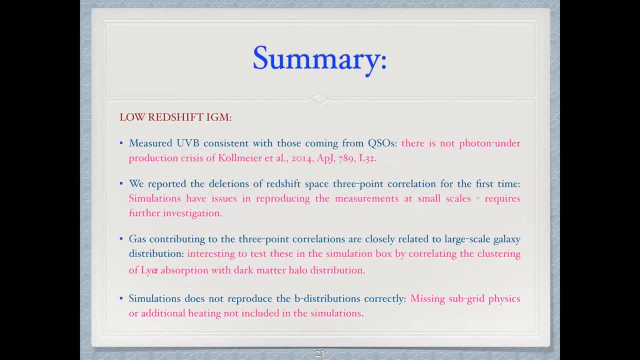 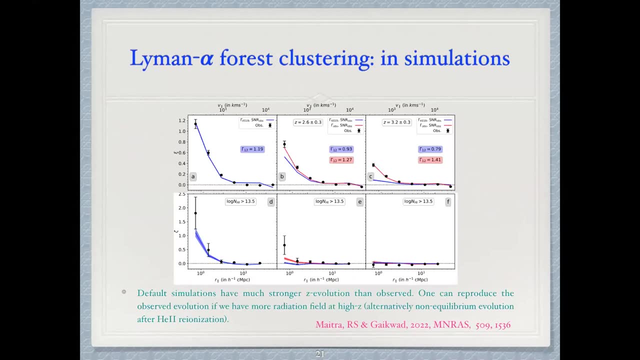 So can you hear me? Yeah, Okay, So if you go, So I have one, I'm not hearing you- Can you hear me now? Yes, yes, No, no, no, no. Sorry about that. 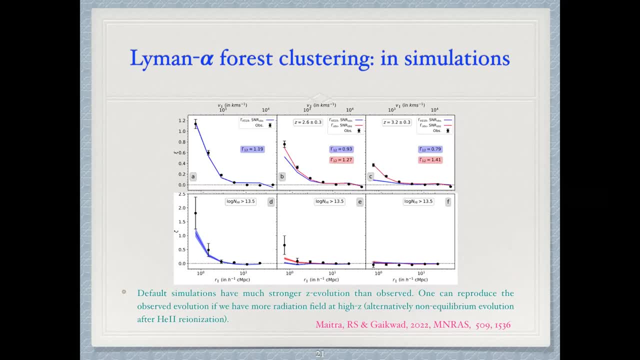 Yeah, So was there something where you showed clustering as a function of redshift, or was it? Yeah, this is a clustering as a function of redshift, Redshift, right, Yeah, This going redshift is redshift is given here. 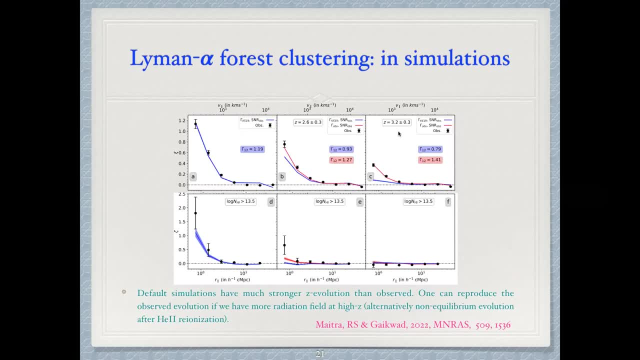 This is for 2,, 2.6 and 3.2.. Yes, Okay. So the question is that this is for which samples? This is for high redshift quasar spectra with special spectroscopy from ground, And like what is the sample size? 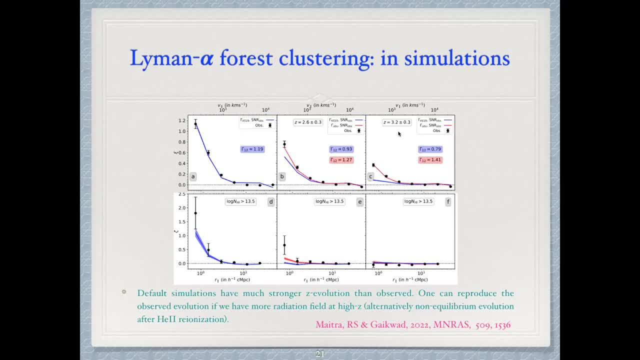 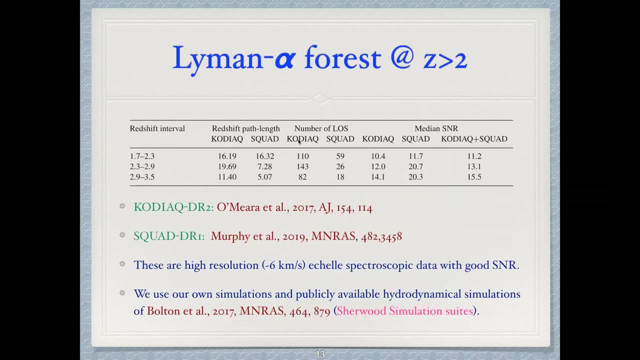 We have about. okay, I have given the details here where the number of quasars used is very high, but we have sampled them. This is the number of quasars you can see, Okay, So no, I was wondering that. 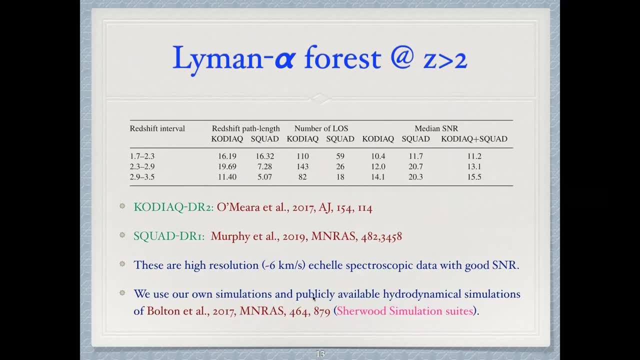 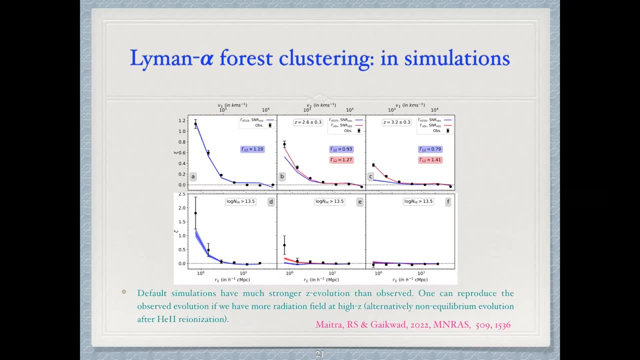 So if you, If you go to the plot Anant- yeah, I was just, maybe I was missing the spatial scale. I was thinking like what is it? H inverse- Sorry, I couldn't read it- T megaparsecs. 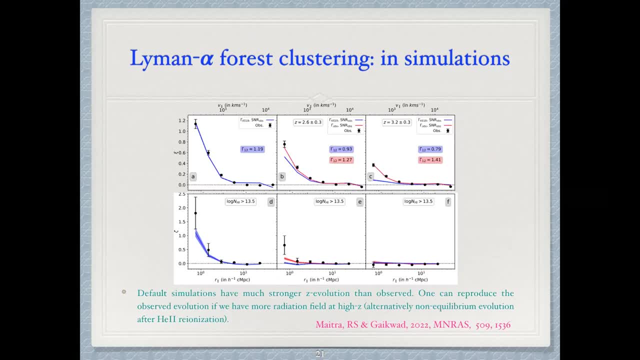 Is that It is like 7, 8 megaparsecs for 2 point correlation? Okay, Oh, 7,, 8 megaparsecs, 2 megaparsecs. Yeah, I was wondering that How to. 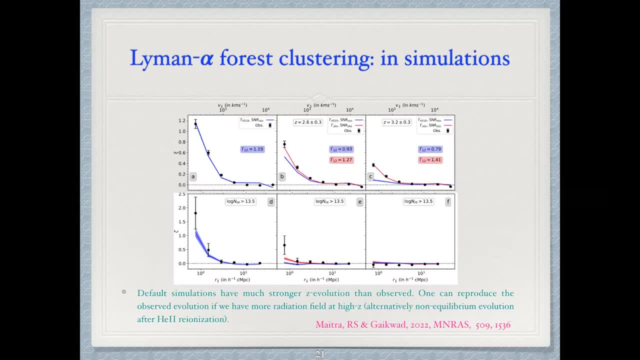 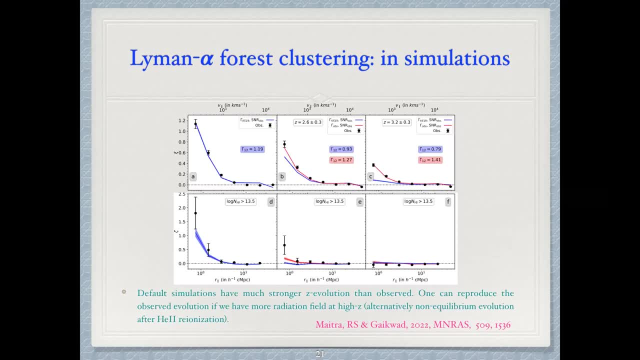 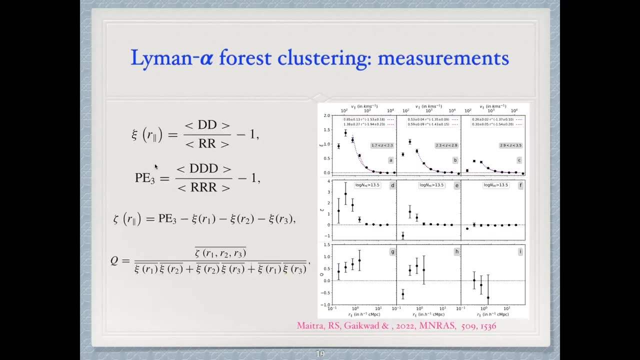 How to, Because the error bars look like quite small. So I was wondering that how I did. Can you just quickly explain maybe? like how was this measurement made that what they're in? You do this two point correlation like this right? 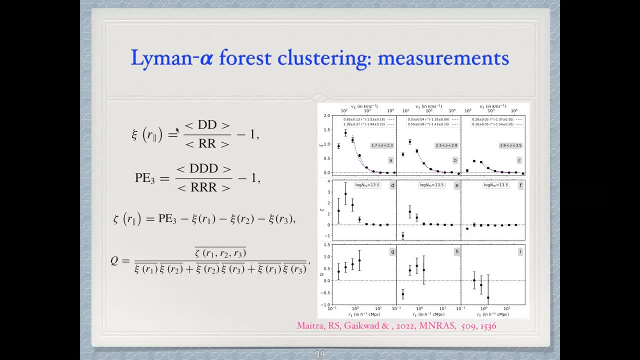 Yes, So basically, you sit in, you go to any cloud and you calculate how many clouds are there with different pairs, pair velocities, pair separations. That is dd, Yeah, And you, we know the total number of cloud along the line of sight. 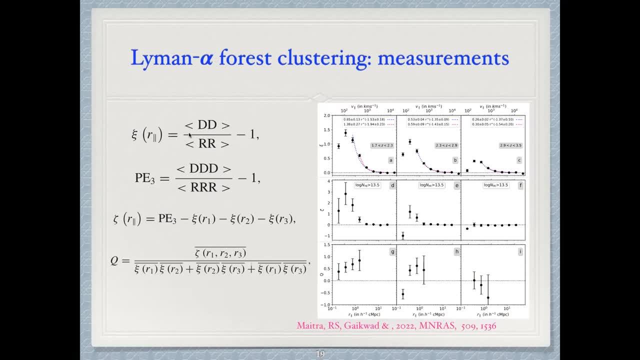 power, take the same number and randomly populate along the line of sight and do this exercise for random. so you know that how many data pairs are there, how many random pairs are there? that's right, and you calculate this and you can do the error in different, different ways. right, you can either do: 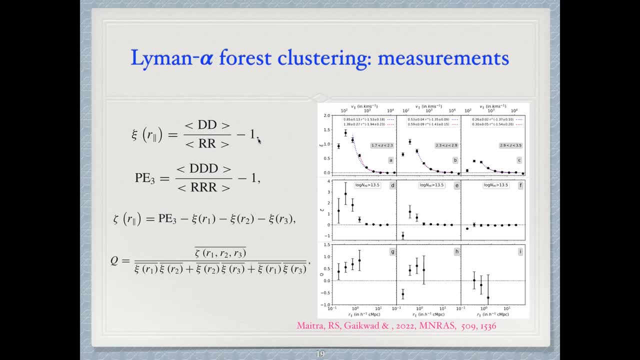 that's what i was asking: that what? what are these variables? either you can have error coming from the bootstrapping exercise because you in then the data thing. instead of using uh, say we have about 200 sight lines, we can bootstrap within them and calculate uh. what is the kind of error? 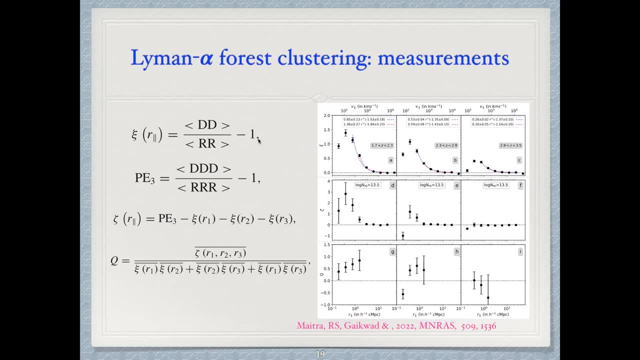 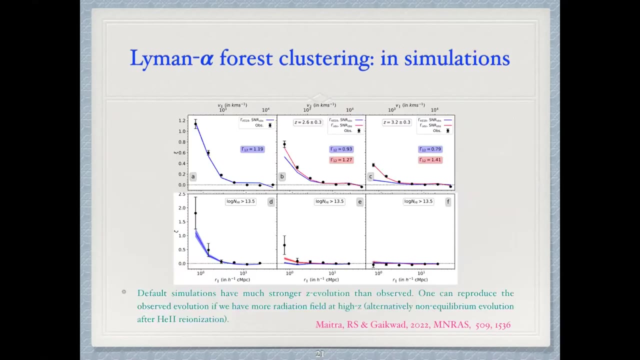 one gets from there right, or you can simply do root and error, which we don't do. we try to do the bootstrap, okay, okay, thank you, thank you. so, yeah, i was trying to ask that because, okay, thanks. so, uh, nirupam commented that basically, there are a large number of clouds along the line of sight. 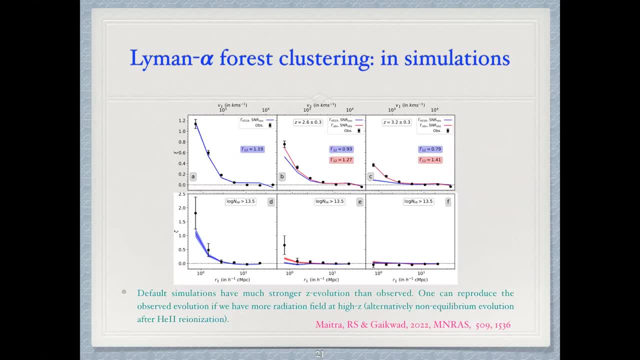 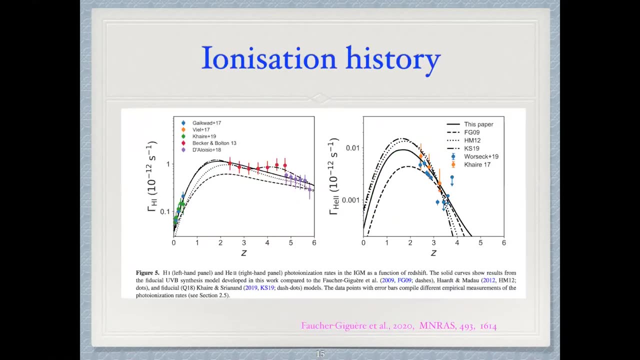 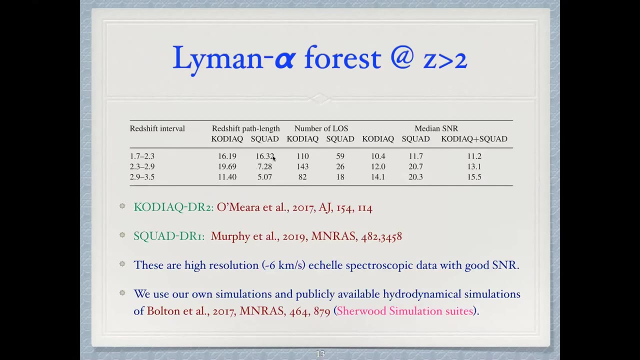 even if qso number is not that high. is that how the error bars are small, effectively? yeah, yeah, i think that is why, uh, what is important is, uh, this is the table. what is important is the path length and, uh, this is what one is talking about, right, so each quasar sight line, you cover quite a bit of redshift range and a lot of 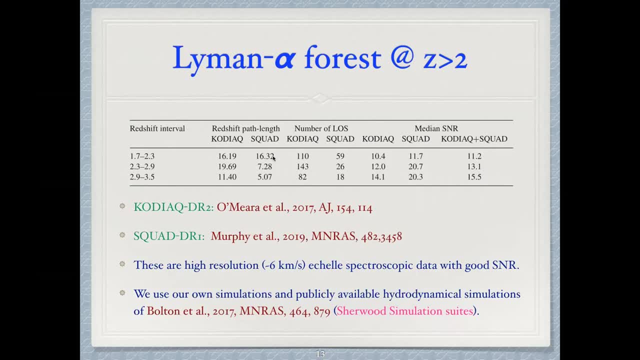 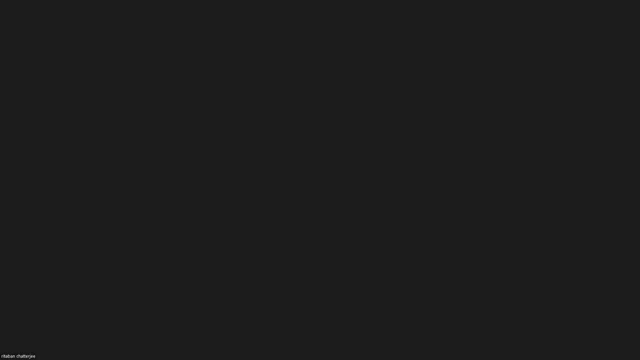 absorption is present. that is the idea, correct? okay, so is there any other question? i saw raising hand, but not anymore, so so if there is no other question, then we'll move on. okay, thank you, shayanan, for for this wonderful talk. um, so let's move on to the next talk now. 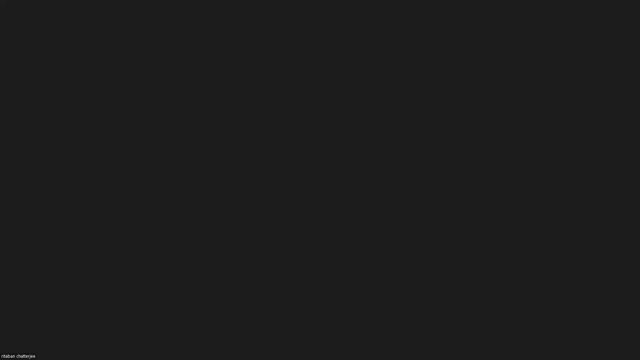 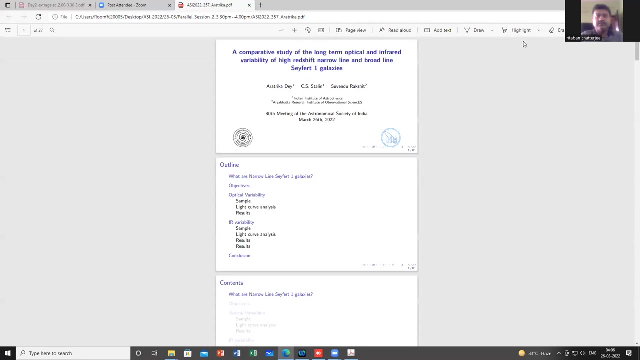 which is by arathrika day. uh, the title of the talk is a comparative study of the long-term optical and ir variability of high-rate shift. narrow line and broad line separate one galaxies. you have 12 minutes for the talk and three minutes for questions, and i'll give you a two minute. 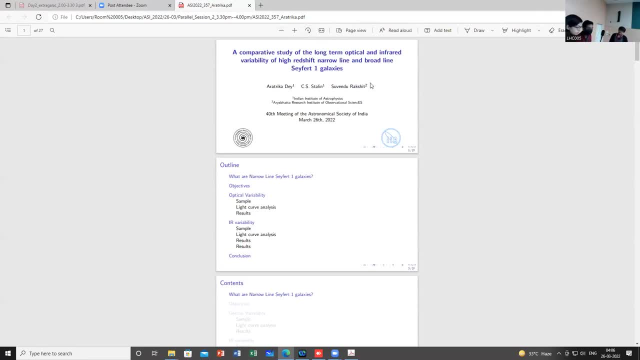 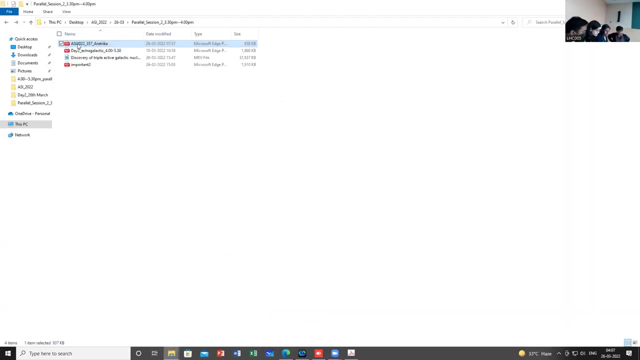 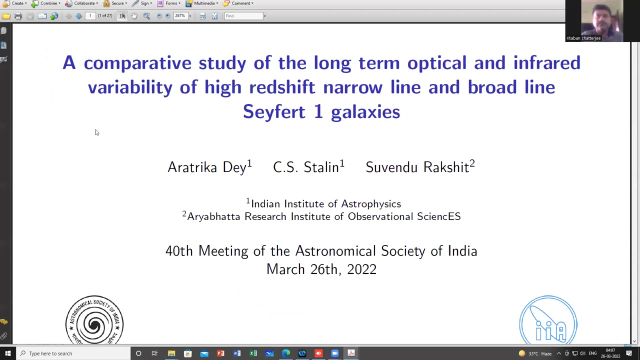 warning at the end of 10 minutes. okay, okay, can you make it in screen please? yes, could you please make it full screen? so is there a view option? i don't need to know you can, you can. yeah, it's okay, you can manage the rest, i suppose. 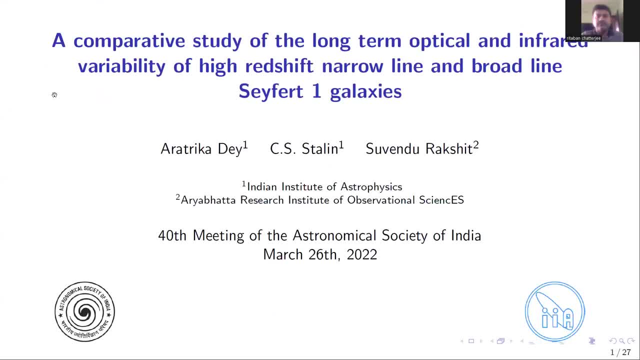 okay, so you can start. it's okay, you can manage the rest, i suppose. uh, hello everyone, both near and far. so, uh, i'm a jrf at indian institute of astrophysics, working under the supervision of professor cs stallion. today i'll be presenting my 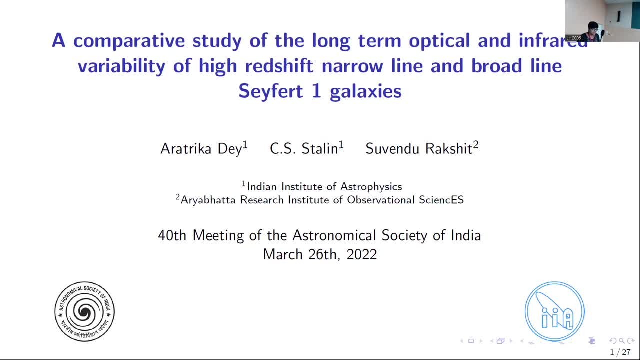 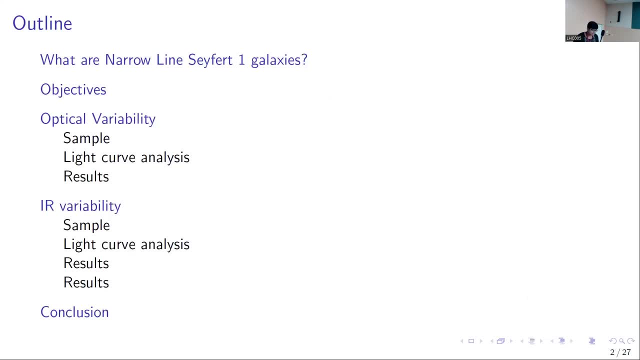 ongoing. ongoing work titled a comparative study of the long-term optical and dire variability of high redshift narrowline and broadline c41 galaxies. now the question that i'm going to start: yeah, hello. so i'm going to start with the question that what are narrowline c41 galaxies? 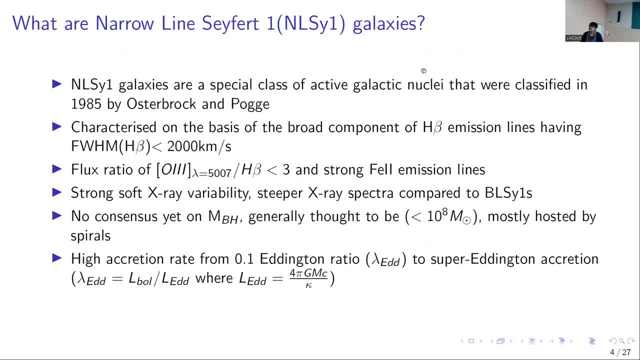 so narrowline c41 galaxies are a special class and active electric nuclei that were classified in 1985 by australian. they were discovered earlier but this classification came about in 1985.. now these are characterized on the basis of their optical spectrum on the. 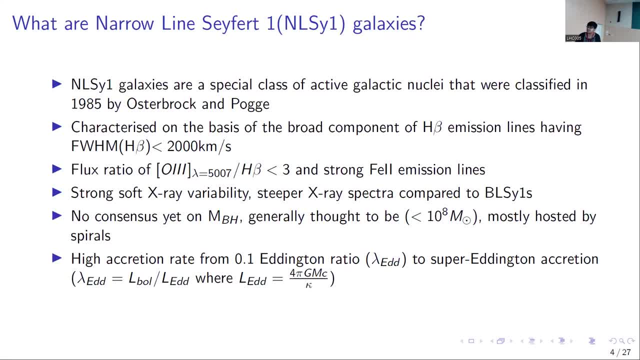 basis of the broad component of the hgb television lines, having a full width at half maximum of less than 2000 kilometer per second. they show weak o3 emission and strong fe2 emission lines. they are also found to show strong soft x-ray variability and steeper xr spectra, as 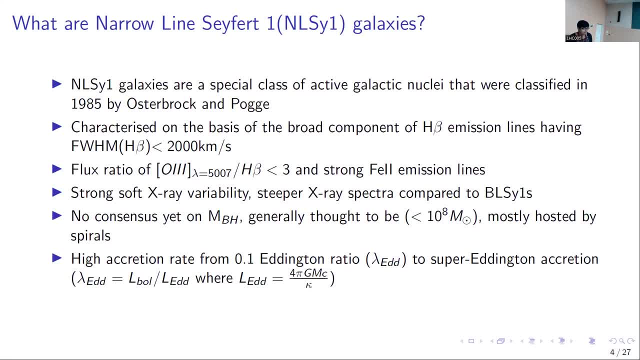 compared to their broad line counter parts. now we have not have we haven't yet reached the consensus uh on the on the nature of their black hole masses, but it is generally thought that the black hole masses range from 10 to the 6 to 20 to the rate solar masses and these are mostly found. to be hosted by spirals. so they are generally thought that the black hole masses range from 10 to the 6 to 10.8 solar masses and these are mostly found to be hosted by spirals, and these are mostly found to be hosted by spirals. 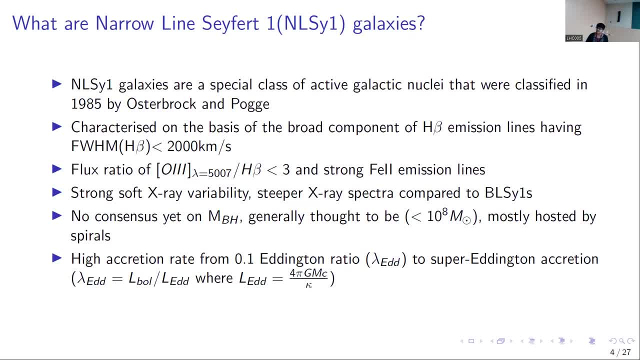 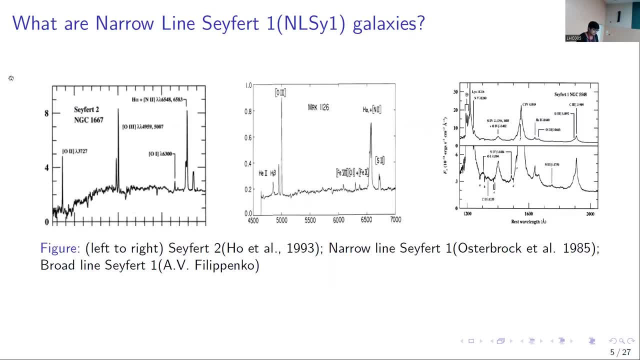 Narrow line. Seifert 1s also exhibit a high accretion rate, ranging from 0.1 Eddington ratio to super Eddington accretion as well. Okay, Here I have shown three pictures. At the extreme left this is the optical spectrum of a Seifert 2 galaxy. 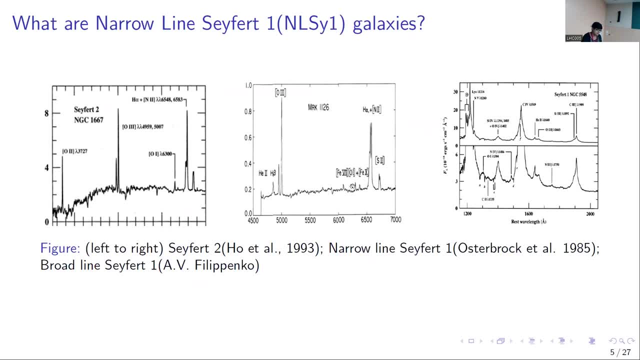 And, as you can see, there are no broad bases in these emission lines. This is a typical spectrum of a narrow line, Seifert 1 galaxy, And here the FWHM of the H-meter lines actually is less than 2000 km per second, but it is. 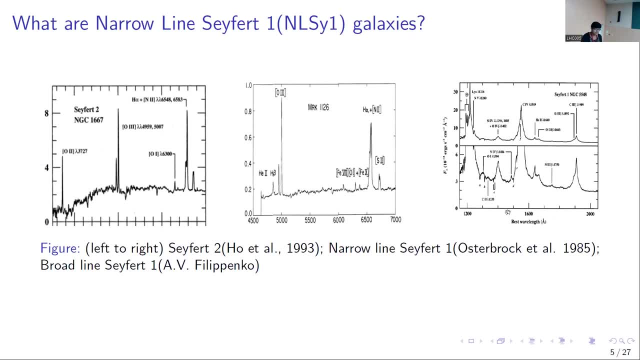 greater than the value that can be seen in Seifert 2 galaxies And coming to the broad line Seifert 1s, it actually exceeds the FWHM, exceeds the 2000 km per second. Now coming to the nature of the narrow line Seifert 1 galaxies, what we know so far is: 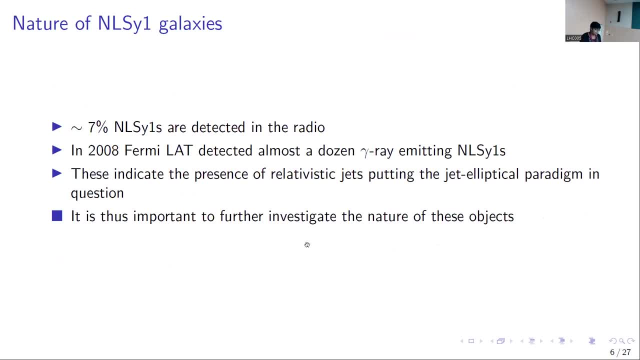 that almost 7 percent of them have been detected in the radio wave Around 2008,. it was found that many of them- a few of them- also exit, exit the radio wave and also emit in the thermal events. So these actually indicate the presence of relativistic jets in these objects, which 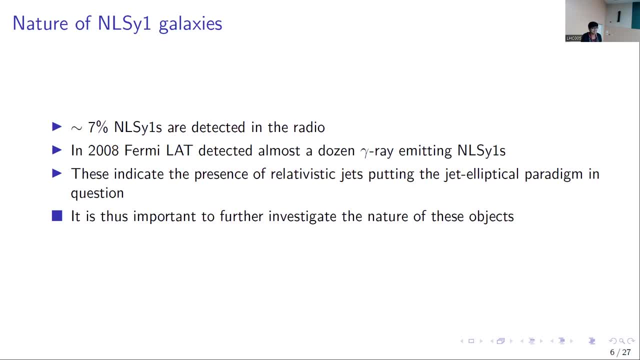 actually puts the jet at the elliptical paradigm in question. That is, jets can only be launched by elliptical galaxies. That sort of is questioned after the after these discoveries. Hence, it is important for us to further investigate the nature of these objects. 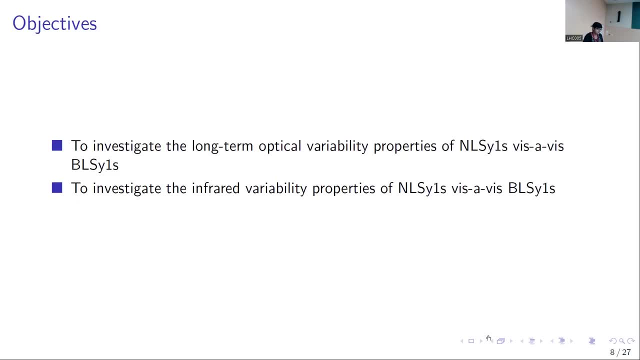 Now, having said the background, I'll come to my work. So, in order to understand what actually? what actually causes this? what actually causes this? This is the differences between these classes of galaxies, both narrow line, Seifert 1 and. 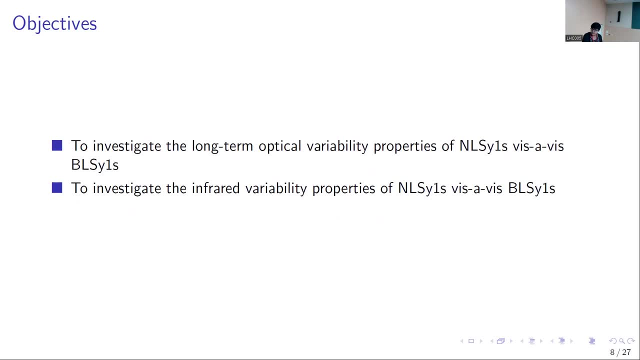 broad line Seifert 1.. One possible mode of one possible method of investigation would be to actually investigate their variability properties. So, keeping keeping that in mind, I have tried to investigate the long term optical variability properties of narrow line Seifert 1s in comparison with broad line Seifert 1s, as well as the 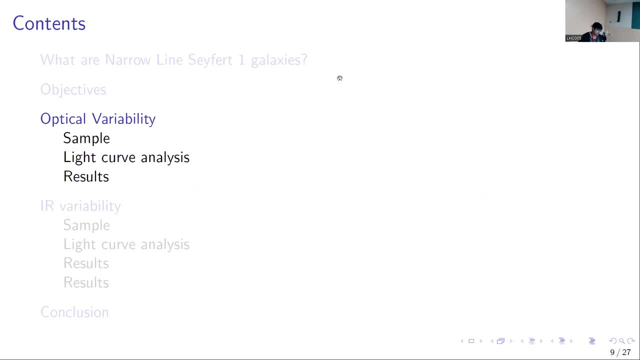 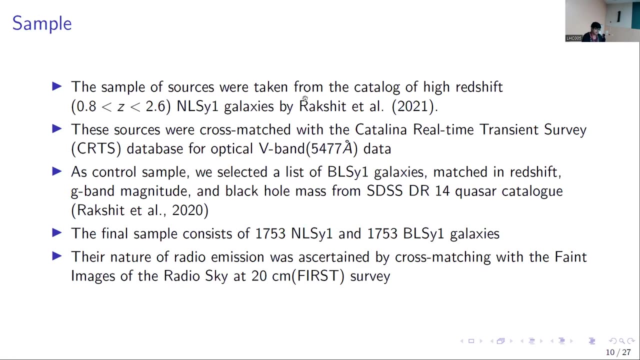 infrared variability properties. Now coming to the optical variability, This is the only investigation of part of my work, So the sample of sources were taken from the catalog of high redshift narrow line Seifert 1s, with the redshift range ranging from 0.8 to 2.6, 0.8 to 2.6.. 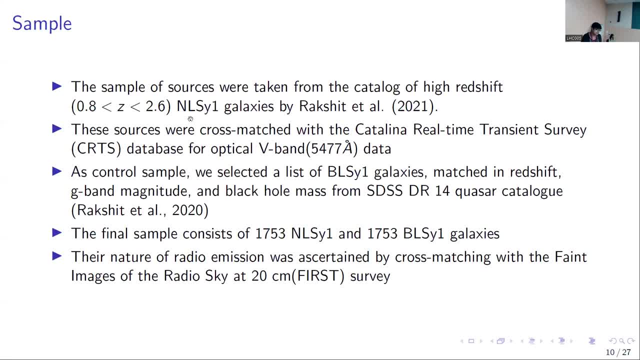 Now these sources were cross matched with the CRTS database in order to find their optical V-band data. Now, as control sample, I have selected a list of broad line Seifert 1 galaxies that are matched with the narrow line Seifert 1 galaxies in terms of redshift G-band magnitude. 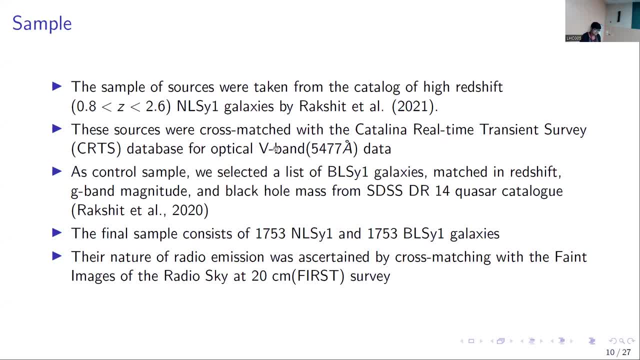 and black hole mass, And those data were taken from the SDSS-DR14 closure catalog. Now a final sample consists of 1,752 narrow line Seifert 1s and a control sample of the same number of broad line counterparts. 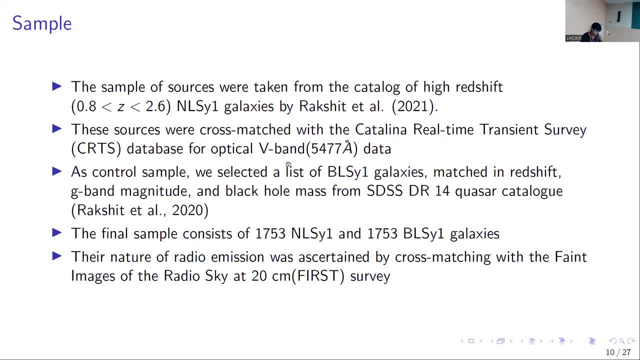 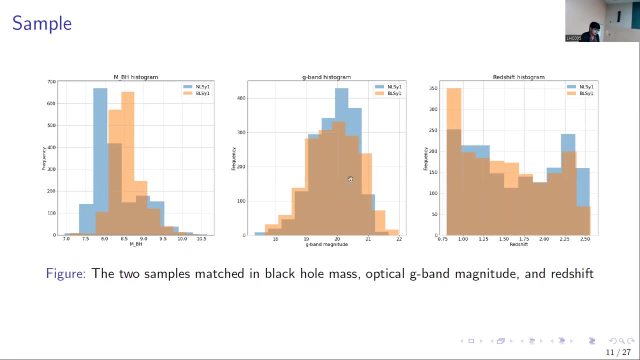 Now for all of these sources. I have again cross matched them with the first database in order to find out whether they emit in the 1.4 gigahertz range. Now let's go to the next slide. These are the histograms of my samples of narrow line Seifert 1 and broad line Seifert. 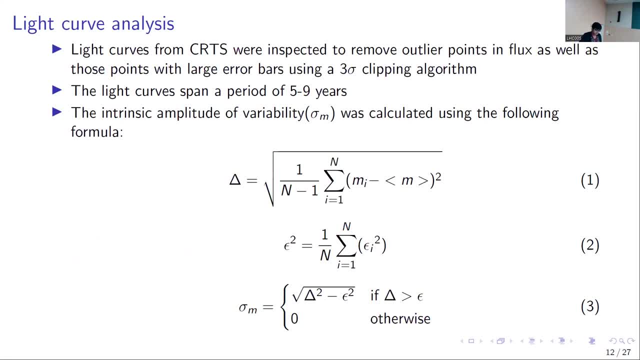 1s. Now, coming to the light-term analysis, the data from CRTS were inspected in order to remove the points with like the outlier points in flux, as well as points with large error bars. I used a three-sigma clipping algorithm. 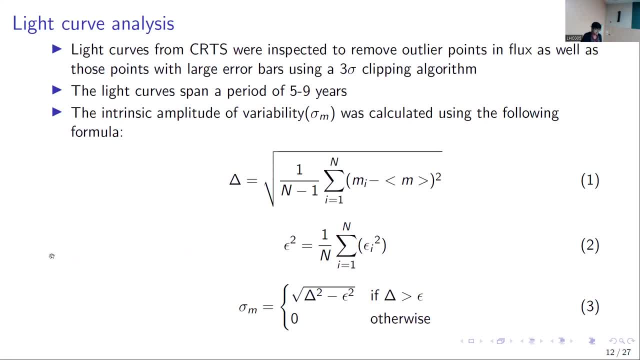 The CRTS data spans a period of five to nine years And, in order to calculate the intrinsic value of the data, I used a three-sigma clipping algorithm. The CRTS data spans a period of five to nine years And, in order to calculate the intrinsic value of the data, I used a three-sigma clipping. 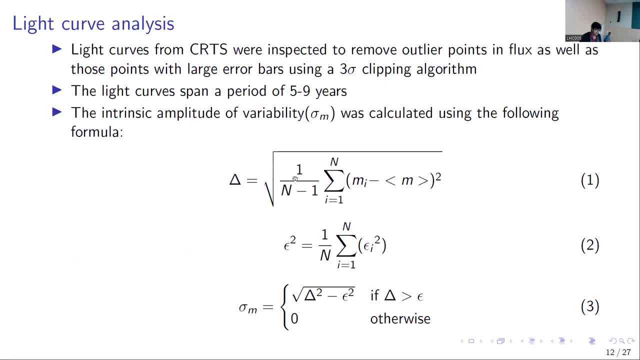 algorithm And in order to calculate the intrinsic value of the data, I used a three-sigma clipping algorithm. And in order to calculate the intrinsic value of the data, I used a three-sigma clipping algorithm. And in order to calculate the intrinsic value of the data, I used a three-sigma clipping. 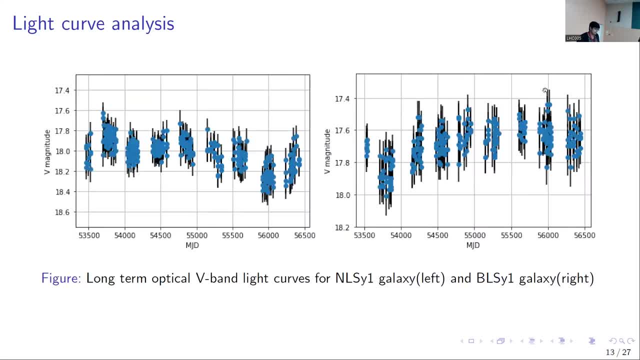 algorithm. Here you can see the amplitude of variability. I used this formula where sigma m is what I am looking for. Here are two sample light curves from the analysis that I have done. In the left there is a sample curve for a narrow line, Seifert 1 galaxy, and this is: 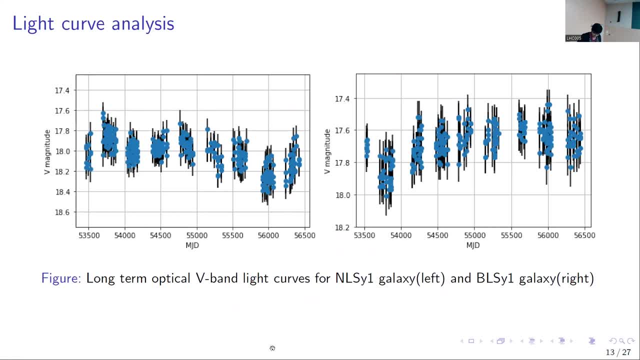 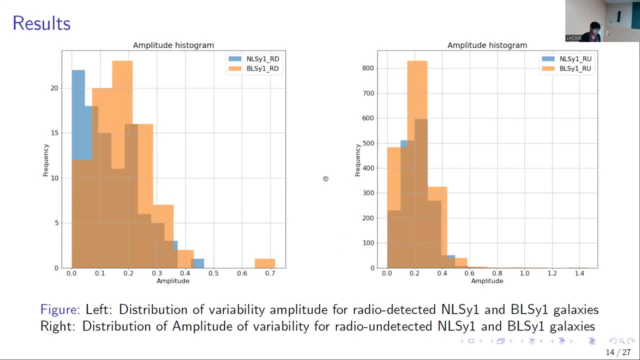 a broad line Seifert 1 galaxy. Now, coming to the results. what I have done is I have compared this sigma m with various physical indexes and I have distributed this graph to zero point zero with various physical properties of the sources. what i have shown here is on the on the left. 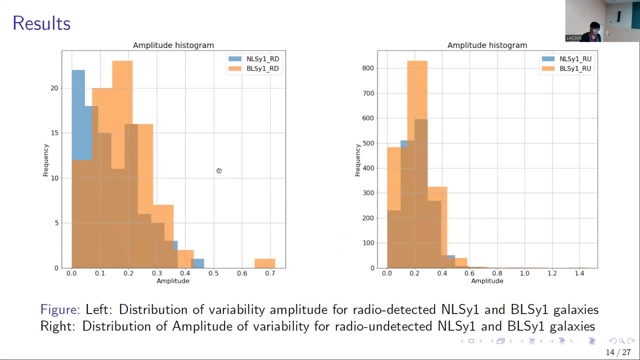 is, uh, basically the distribution of variability amplitude for only the radio detected: narrowline c41 and broadline c41 galaxies. now a clear shift is shown here. i'll. i'll elaborate the results in a later slide, and this one here is basically the distribution for the radio undetected ones. 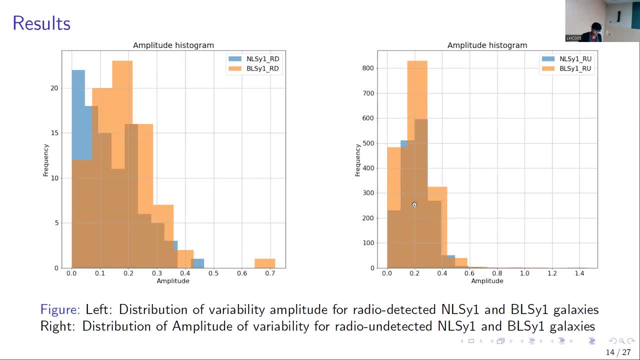 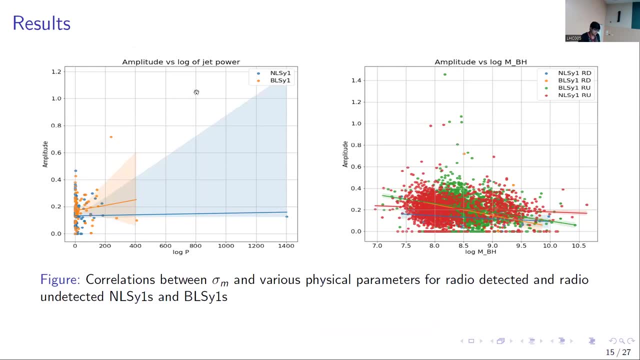 um, yeah, okay, now this is amplitude versus log of jet power. i have to. i have tried to find out the correlations between sigma and this uh uh, jet uh, jet power parameter and also the black hole mass. the results again come in a later slide. now, moving on to the second part of my work, which is the 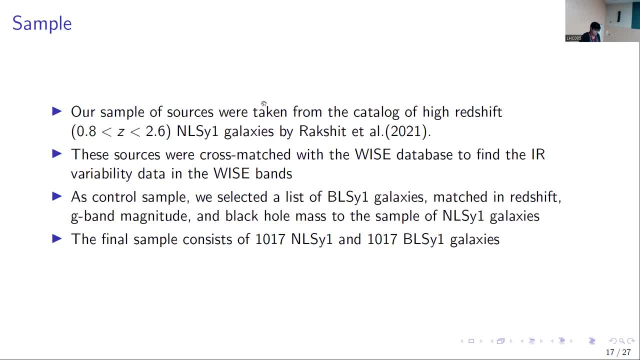 infrared variability. here again, my sample of sources were taken from the, from that same catalog, and these were crossmates with the wise database in order to find the, the data in uh in the wise bands uh, as control sample i selected this list of broad line c41 galaxies, again matched in red shift. given magnitude and 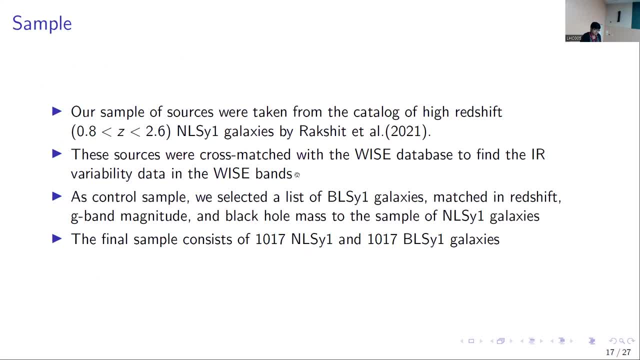 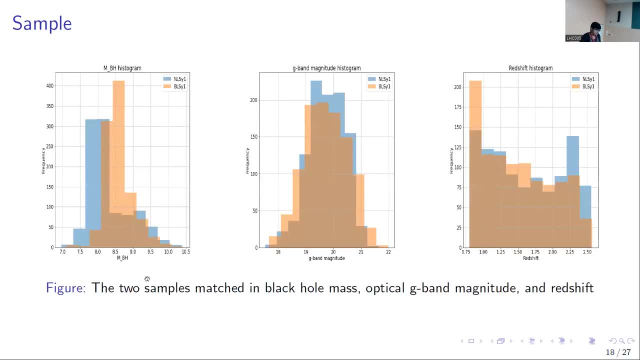 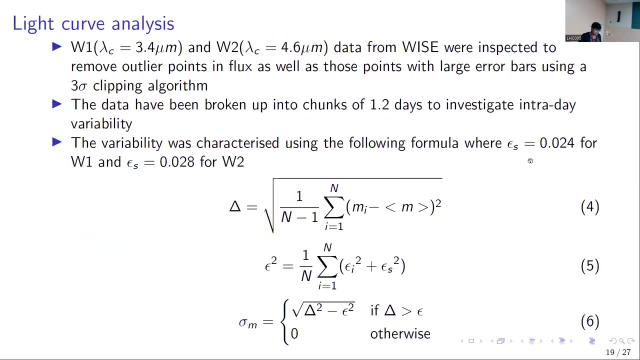 black hole mass. now, uh, my final sample consists of 1017 narrowline uh seaford ones and their broad line countered ones. uh, this is again with the distribution of my samples in black hole mass, given magnitude and red shift. uh, coming to this part of the lifetime analysis, so i've analyzed the data in two bands, w1 and w2. 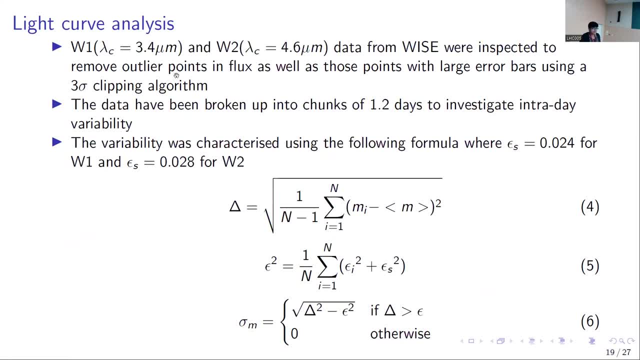 uh, again, i have removed the outlier points and flux, as well as points with large error bars. uh, i have also tried to investigate a short-term variability by breaking up the data into chunks of 1.2 pieces. uh, this is the formula that i have used in order to characterize, uh, the aptitude of 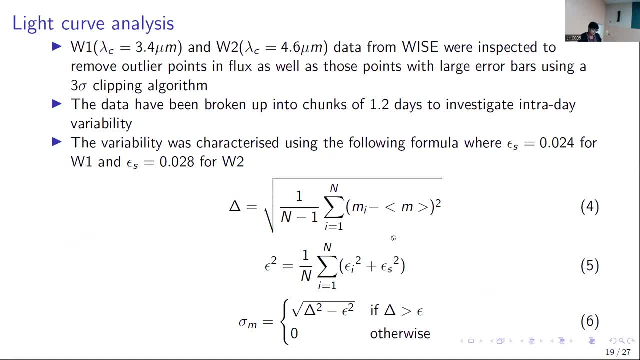 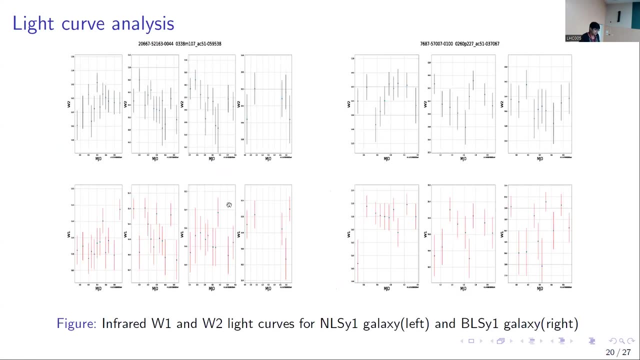 value in order to calculate the amplitude of variability. the only difference is that i have a systematic error term coming in which has been calculated to be 0.024 and 0.028 values for w1 and w2 bands respectively. this i have taken from the literature um. these are two sample light curves for 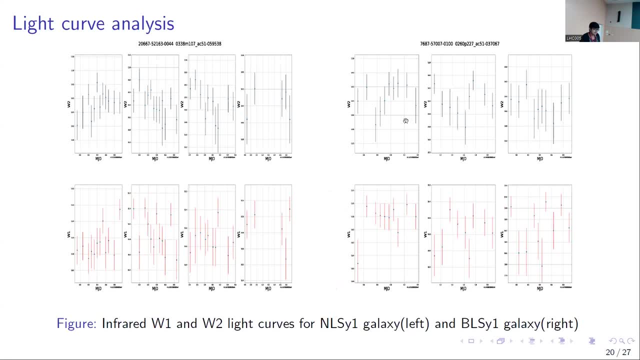 the left one is for a narrowline seaford one and the right one is for a broadline seaford one. the bottom panel shows the w1 data and the top panel shows the w2 data. uh, these boxes basically, uh corroborate the the 1.2 day chunk. 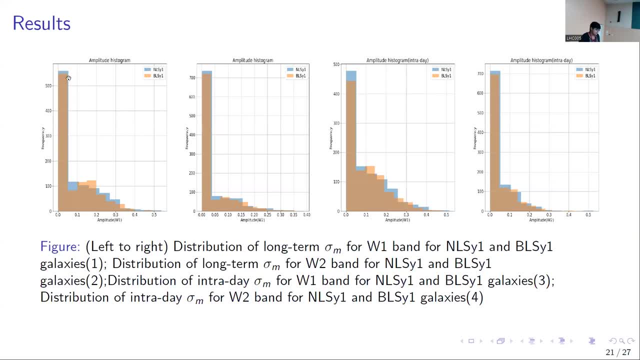 okay, so these coming to the results, uh, this, uh, at the extreme left, this is basically the distribution of long-term uh amplitude variability for w1 back, and this is the same for the w2 band, for narrowline c41 and broadline c41 as well. and uh, this, this is. these are the same quantities for the. 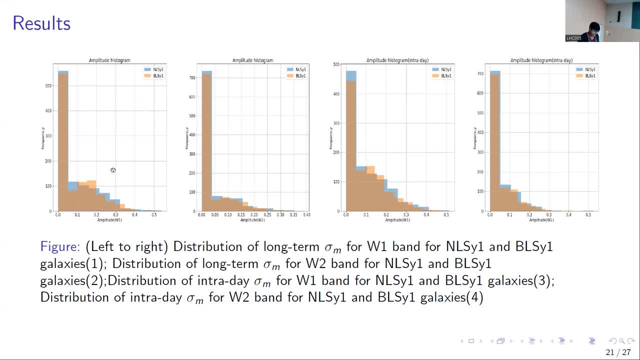 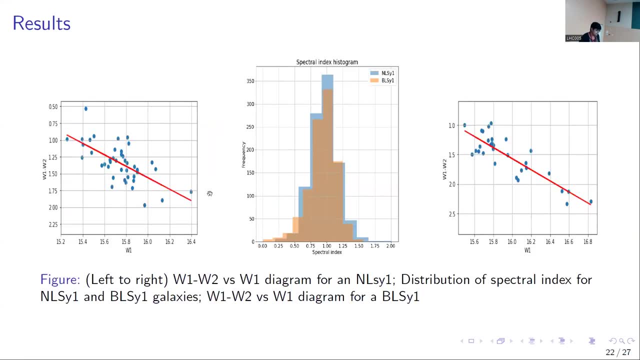 short term period. now, as we, as you can be seen here, these are quite, quite similar. here, what i have done is i have plotted this w1 minus w2 versus w1 diagram for a for the same narrowline, c41. that goes with the light curve that i showed earlier, and this is for a broadline. 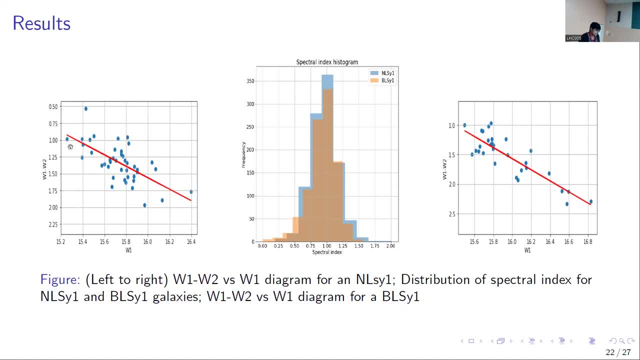 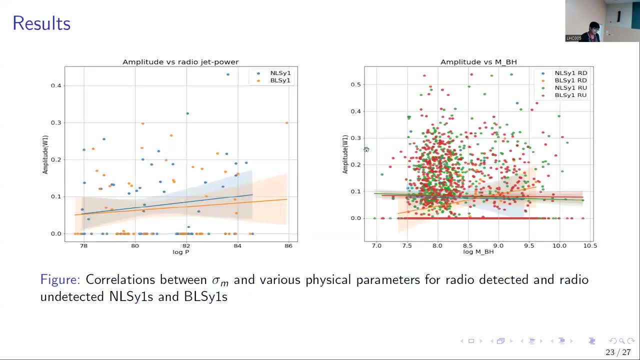 seaford one, and this is the histogram for the for the slope of this, uh, these lines that i have plotted for, the narrowline seaford one and broadline seaford one ones, uh, uh, similar to the previous work, i have tried to find out the correlations between the 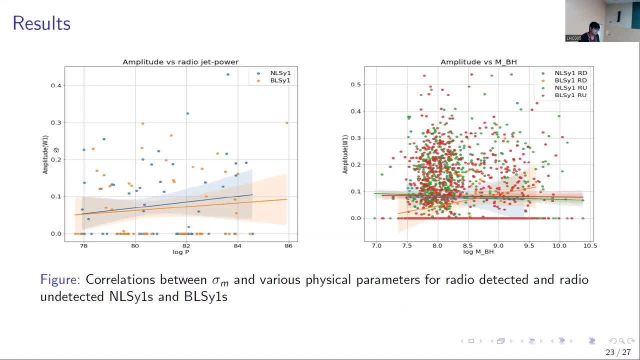 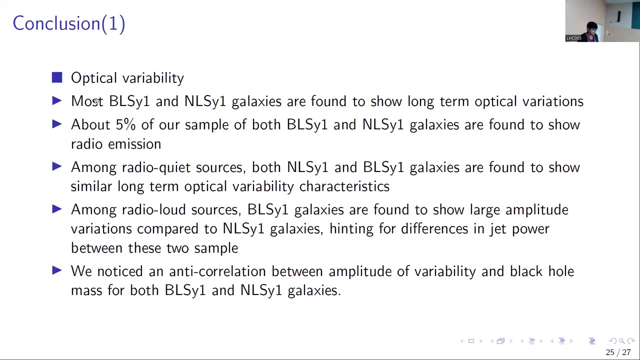 the amplitude of variability and the physical parameters like radio jet power and the black hole mass for for radio detected as well as radio undetected, narrowline, seafood ones and broad lines. uh, now coming to the conclusions. so, uh, as i showed earlier, uh, i'll say about the optical 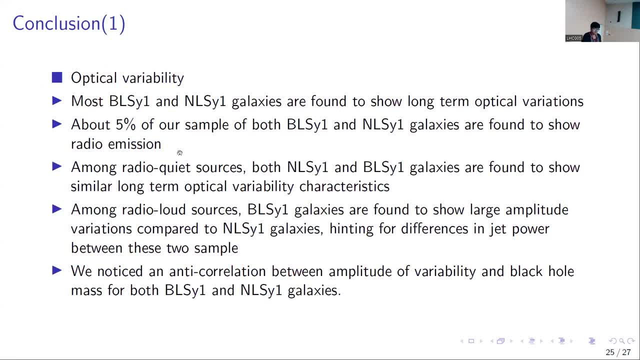 variability results first. so most broad lines, if i don't analyze, if i don't, galaxies are found to show long-term optical variations. we also found that, uh, about five percent of our sample actually were emitting in the radio. i mean it was available in the first server. uh, now for the radio, i think. 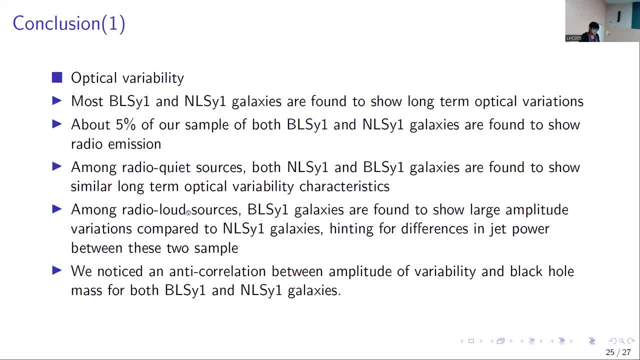 it is actually radio undetected. for the radio undetected sources: uh, it was found that both narrowline seafood and broadline seafood one showed, uh, similar long-term optical variability characteristics. but that did not hold true for the radio loud sources, basically radio detected sources. uh, it was found that the broadline seafood one 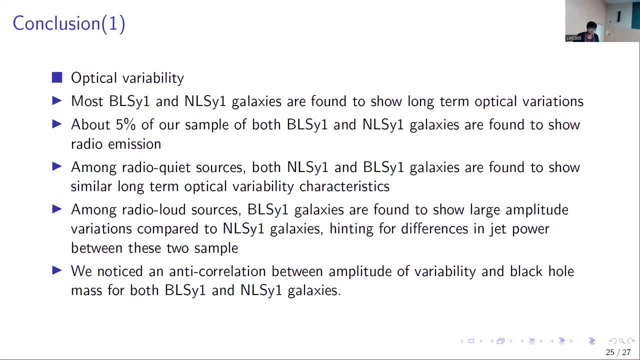 galaxies are showing higher amplitude of variability as compared to, as compared to the narrowline counterparts, which is which might have been due to the differences in jet power between these two samples. and it was also found that the jet power of the radio undetected sources is actually higher in the broad line, zero to one sample. and the curious thing that we noticed is 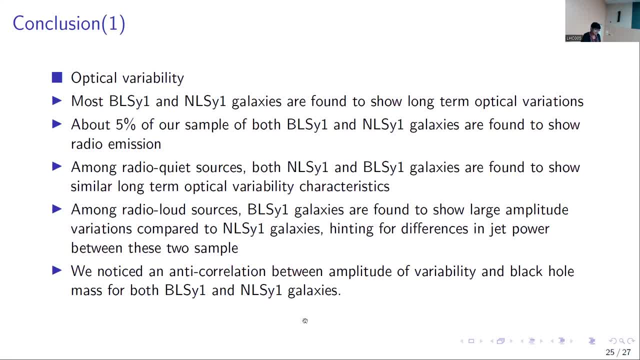 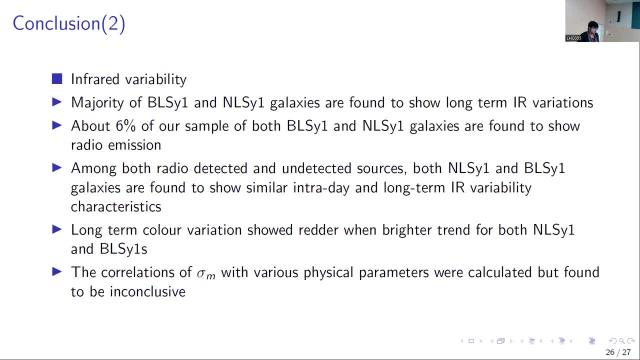 an anti-correlation between the amplitude of variability and black hole mass for both these classes of galaxies in the optical variability part of my work, of course. now coming to the ir part, it was found that, uh, not most, but majority of the of these two classes of galaxies. 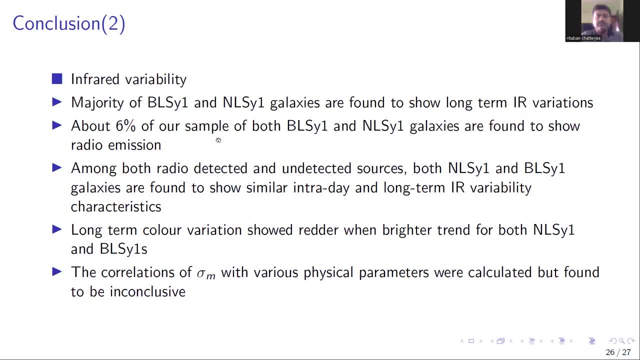 should long-term infrared variations. you have two more minutes, yeah, okay, uh, there is a question. what is the probability that the radio and the uh- almost six percent of our sample for both these classes- were found to be detected in the radio? for both radio detected and undetected sources, it was found that there were similar internet as well as long-term 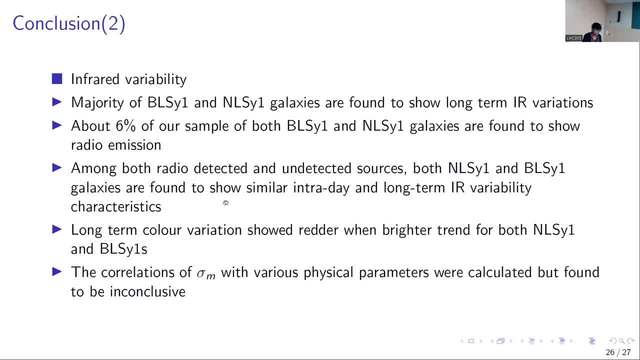 higher variability characteristics for both these classes of galaxies- uh, that i showed in one of the one of the previous slides, the histograms- uh. it was also found that long-term color variation actually showed the trend that they were red and even brighter. I mean, that was something that we saw. 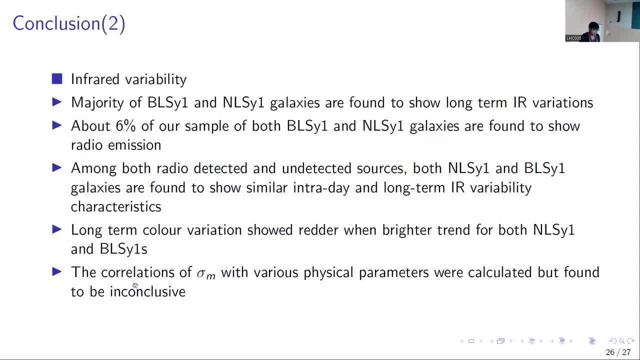 for all of our sources. actually The correlations that I've tried to draw with various physical parameters like radio flux at 1.4 gigahertz, corresponding radio jet power, black hole mass, all of that, those are calculated but those are basically found to be in. 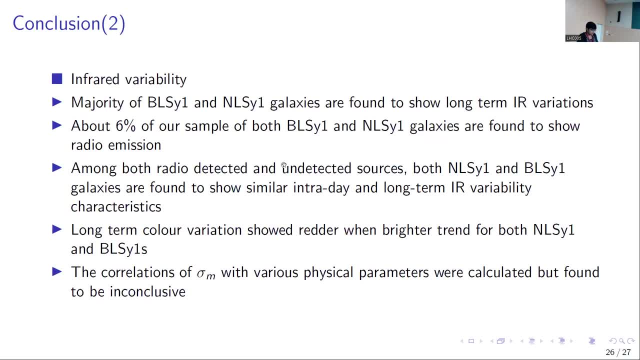 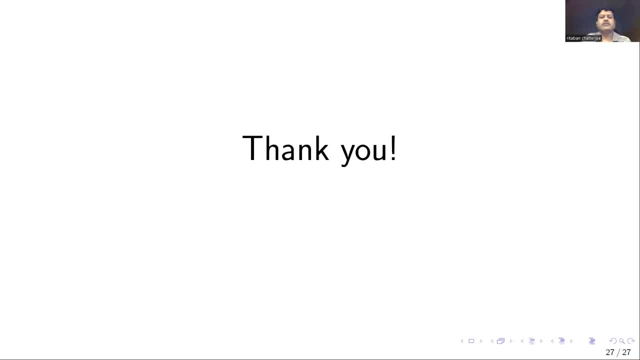 Nothing could be inferred out of that. So yeah, that's all, thank you. Thank you, Arathrika. So is there a question? Yeah, I think there is. So I don't see any raised hand in Zoom. Is there a question? 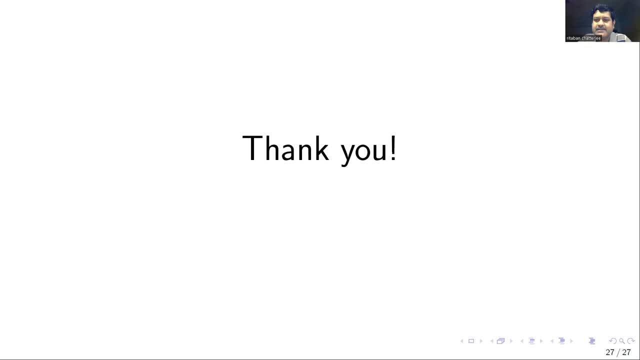 In the audience. there is In the audience, there is okay. So then can you please repeat the question when you hear it: Yeah, yeah, of course, So, yeah, plot. So you plotted jet power versus amplitude. I want to know how you have defined amplitude. 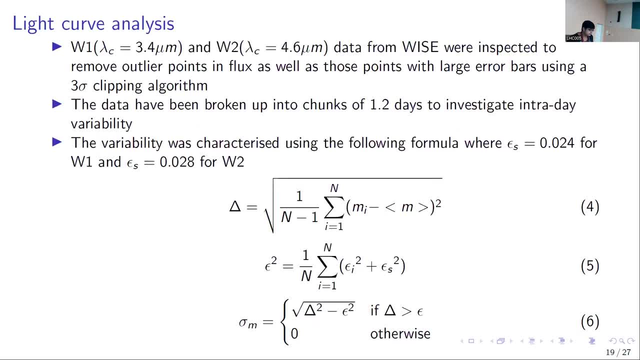 Okay, yeah, I'll go to the slide, maybe. So are you talking about the optical part or the radial part? You plotted one. it was an amplitude versus jet power in log, So that's something I've done in both the cases. 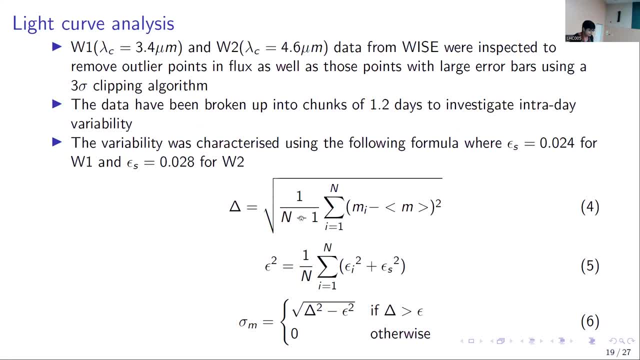 So any one of them? how do you define them? Yeah, this is how I have defined this amplitude of variability. So this is basically the variations on top of the error. This is like variability in the light curve. That is how you define amplitude. 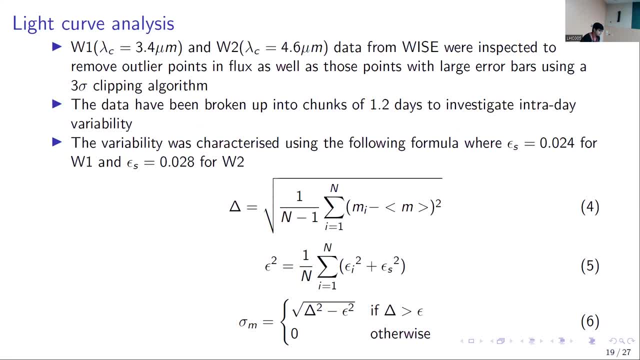 Yeah, yeah, yeah, It is variability of amplitude. Yeah, oh, okay, yeah, got it thanks. Oh sorry, you did not repeat the question. No, that's okay, we could hear it. Okay. So is there any other question in the audience? 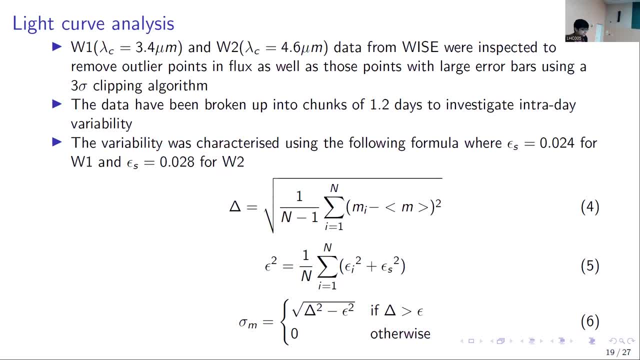 Because there is two raised hands in the zoom. There is another question. Okay, please go ahead. So my curiosity is that you have tried several parameters for both, that of galaxies, but uh, not, uh, yet you don't have any concrete separators right from the parameters. 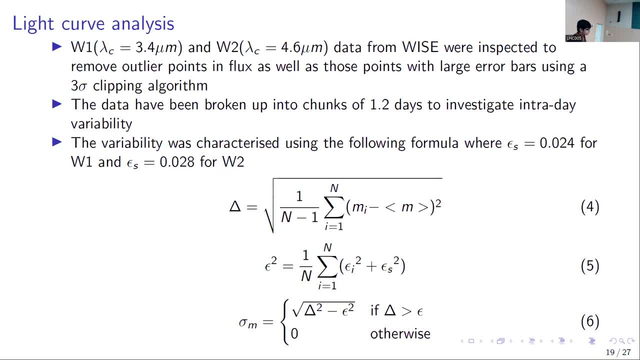 for the internet? i don't have. yeah so, but my point is like: uh, what, what all are your expectations? why you wanted to uh put these parameters? yeah so, narrow length support one and broad length support one. we know, like observation, that these are two separate classes of galaxies, but what? 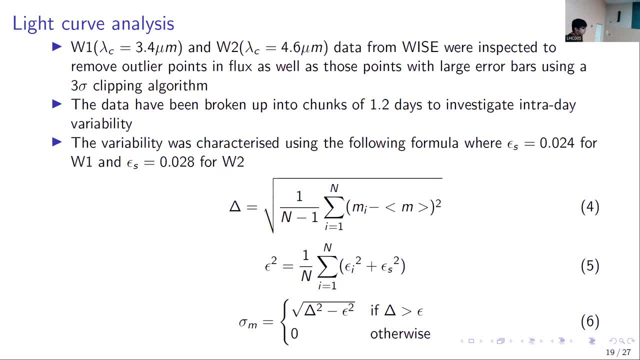 drives this difference? that's, uh still not clear to us. so, uh, the physical parameters like luminosity, black hole, mass accretion rate, these are found to be found to be quite uh like correlated with variability properties. so that's why, that's why i've investigated the variability properties and 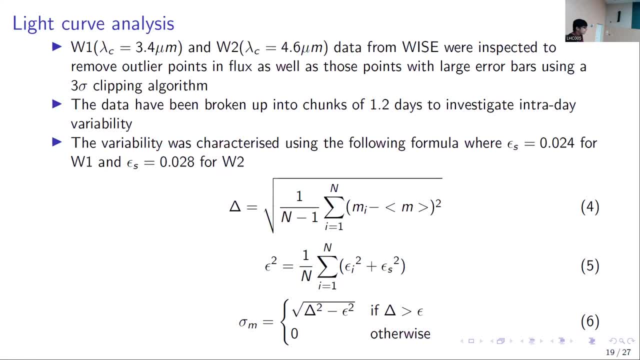 their correlation with this physical parameters in order to find out that, if some, some, some light can be thrown upon the, i mean what actually drives their difference, the difference that we see in the spectrum. so that's the idea. so does it say that, um, there is no differences in terms of no, that haven't concluded. 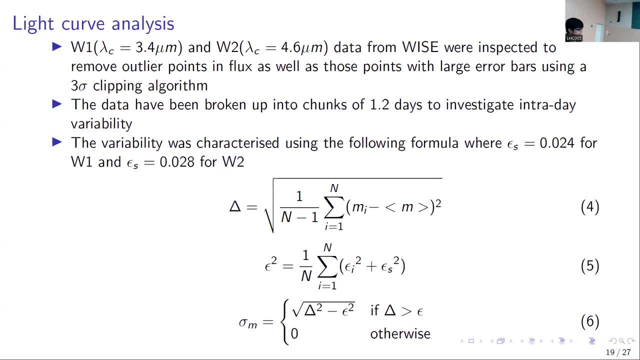 yet. so in the optical part of my work, i have seen some differences. uh, for example, there is a quite a clear difference in the jet power, but in the iron there is no conclusions. no conclusions have been reached yet. so so should we move to the next question now? so priyanka rani has a question. 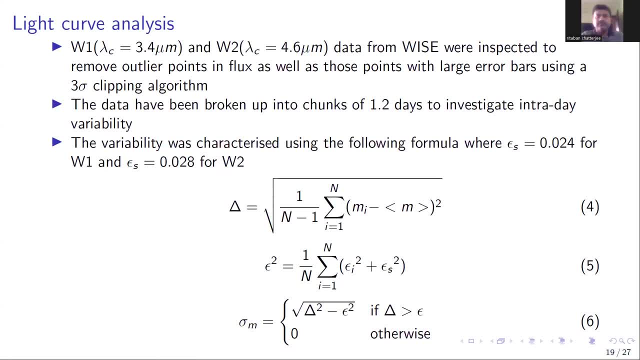 excuse me, sir, sorry, there's another question. okay, so then should we, uh, maybe the audience question. they can talk to the speaker after the session and we we should choose one of the zoom questions or whatever you prefer. okay, okay, yeah, yeah, one zoom question, maybe. okay, sure, so priyanka rani has a question. priyanka, could you unmute? 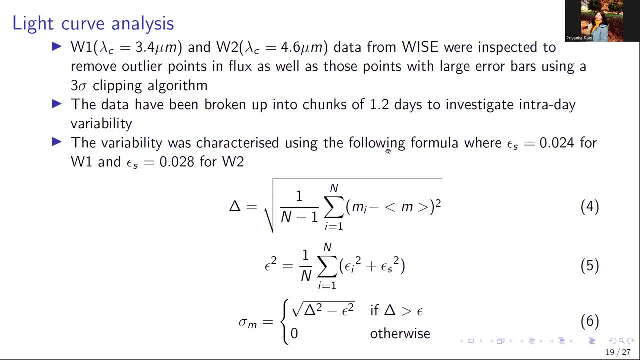 yeah, hi, can you hear me? yeah, yes, yeah. so i have one question, that how did you obtain this uh radio jet power and black hole masses for your sample? and another question is like: do you know, like, how many sources in your sample are known to have jets? because no, no, it's okay. 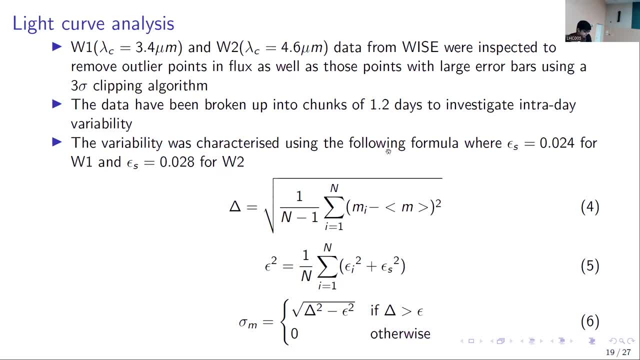 that. the second thing: i don't know how many sources have been known to have just that, i don't know yet. uh, but for the first first part, radio jet- i have calculated uh using this um uh data from first. so that has been redshift corrected and i have used a formula that i 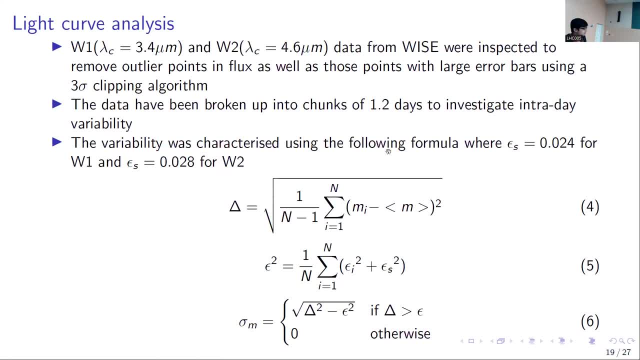 haven't put here. uh, how to um? so, basically i have calculated the luminosity distance, i know the red shift from the sdss- they are put in catalog- and i know the first flux in the flux density in the 1.4 gigahertz center. that's central. uh, that, that, that thing i know. so these things i have put. 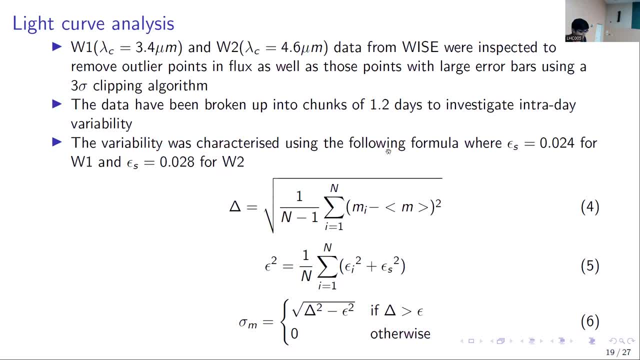 together to find out the radio density power. uh, i don't know how to, okay, so, um, so, should we move on to the next? uh, so, alanda. so, very quickly, you have a question? oh, another thing, bianca, uh, uh, so, none. i the sources that i've used that none of them have. 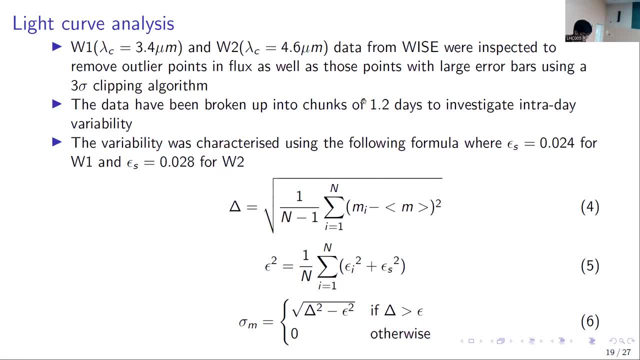 this, uh, have been detected in the camera. that much intended. hello, can you hear me? yes, hi, um, you know i may be interested in. um, i'm interested in spiral host, large radio galaxies. spiral host, large radio galaxies i'm interested in. okay, so you have said that six percent of your sources are detected in first radio data. yeah, yeah, and. 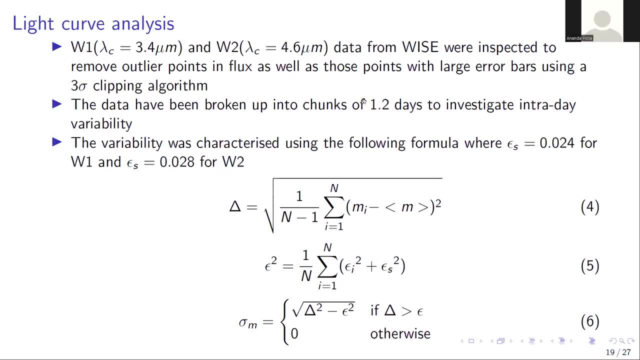 most of these such sources are in spiral. oh, that you have. uh, so okay, so the this is actually part of my future work, so it was known so far that mostly narrowline seaford ones, as well as broadline seaford ones, are hosted in spiral galaxies. but after this, 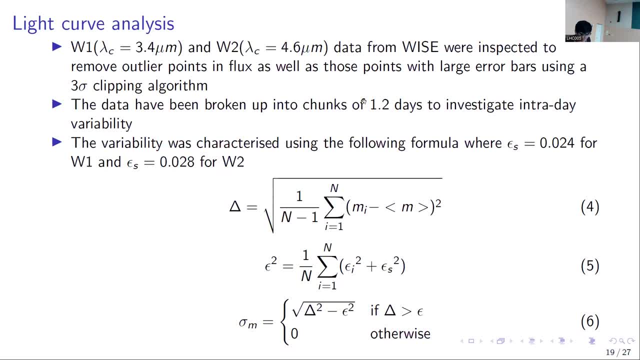 discovery of jets that has been. there has been questions about it like, uh, whether spiral galaxies can also produce jets or narrowline seaford ones can also be hosted in ellipticals. so this is part of my future. like to find out what sort of the nature of the host galaxies of narrowline seaford. 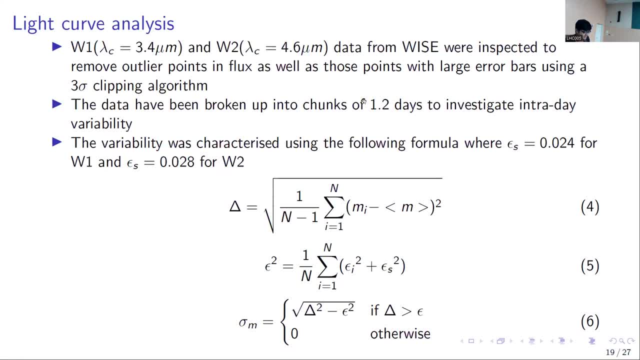 ones. so here i haven't said that all of these galaxies are radio, are spiral galaxies, because we don't know yet. they're too far, simply right too far. yeah, my mine is a high rate ship sample, so it might be difficult to actually resolve uh, that much so uh, i i don't know whether the, whether it's exactly because they're. 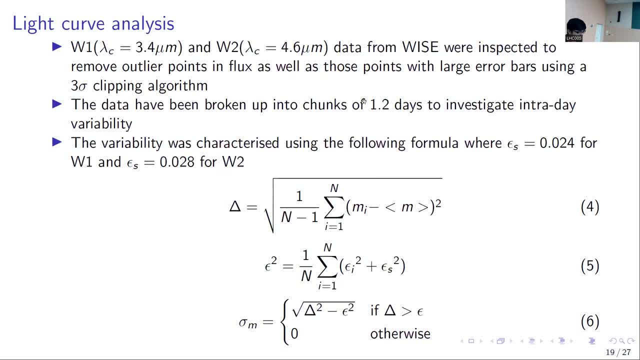 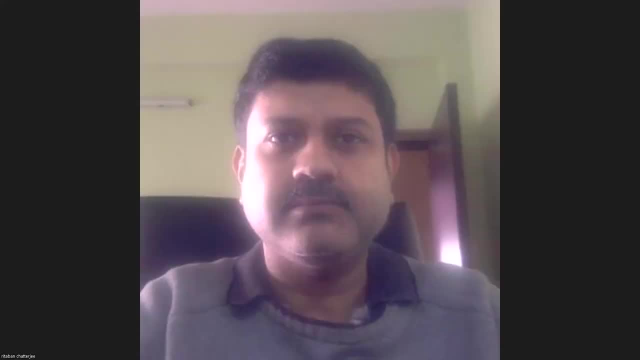 too far, but i think that is a possibility that, since these are high rate ship sources, it might be difficult, okay, so, uh, we have to stop now. please, uh, uh. if there are other questions, please, uh, talk to the speaker after the session and we'll move on to the next talk now, which is by jyoti jadav. uh, it's on discovery of. 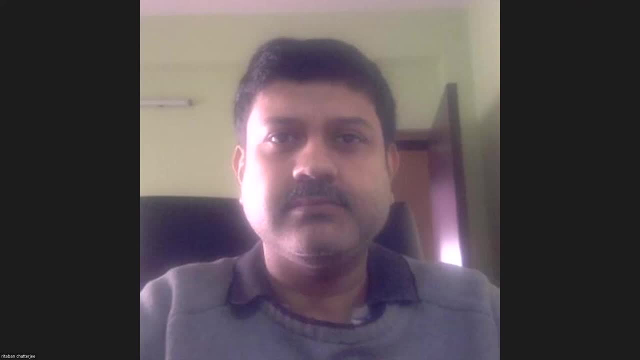 a triple agn in the ngc 77, 33, 77, 34 merging group. this talk will be through a recorded video. okay, so the volunteers will now play the video and then, uh, at the end i will give you the link to the recording of the video. so if you want to go ahead and watch the video, 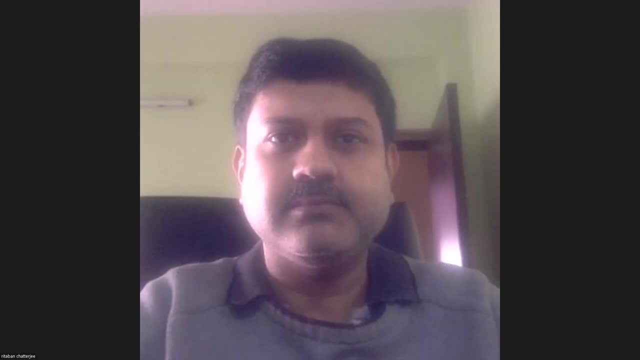 and then, uh, at the end i will give you the link to the recording of the video. so if you want to go ahead, i guess, i guess the question session will not be there because probably the speaker is not. the question session will not be there because probably the speaker is not. 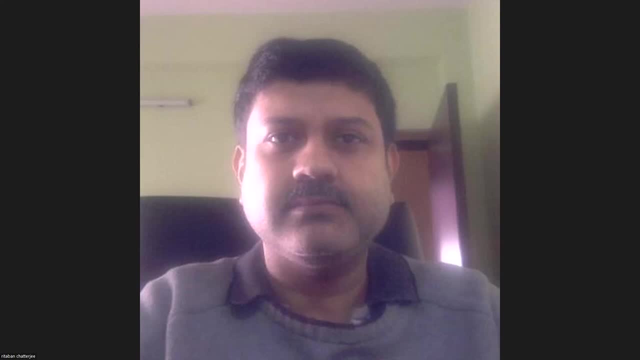 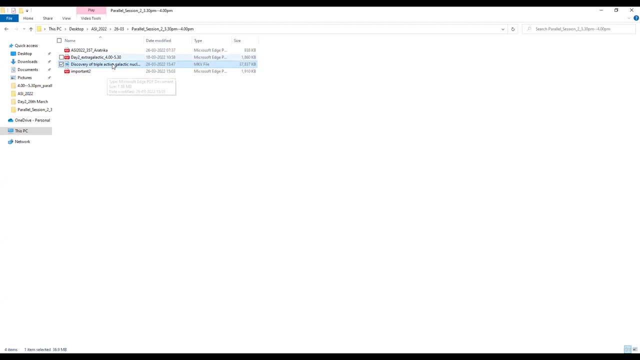 the question session will not be there because probably the speaker is not present. is that right? okay, so, please, please. i'm jyoti and first of all, i would like to thank the organizers. okay, so, please, please. i'm jyoti and first of all, i would like to thank the organizers. 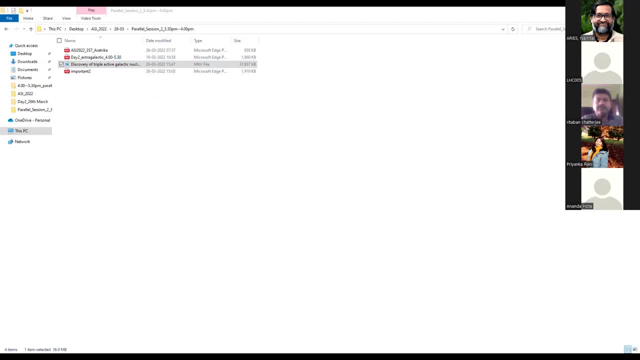 okay, so please, please. i'm jyoti and first of all i would like to thank the organizers for giving i. i cannot see the video for giving i. i cannot see the video for giving i. i cannot see the video. i can hear the voice, but i can hear the voice, but. 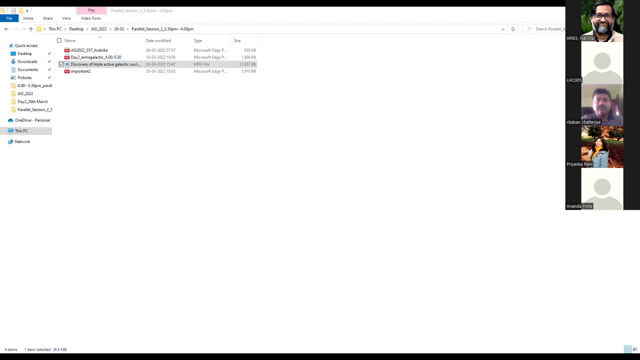 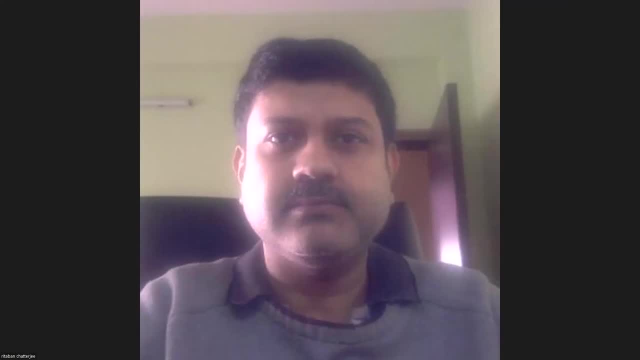 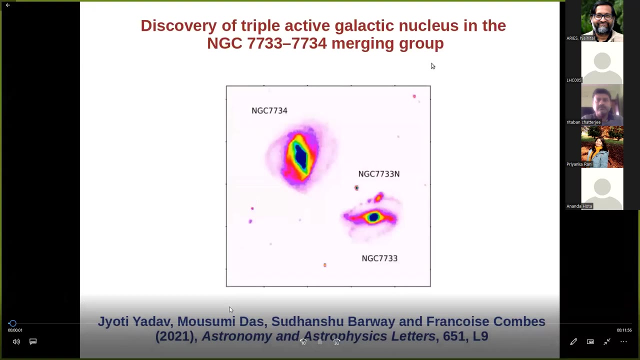 i can hear the voice, but so, yes, now i can see. yes, hello everyone. so, yes, now i can see. yes, hello everyone. so, yes, now i can see. yes, hello everyone. i am jyoti and first of all, i would like. i am jyoti and first of all i would like. 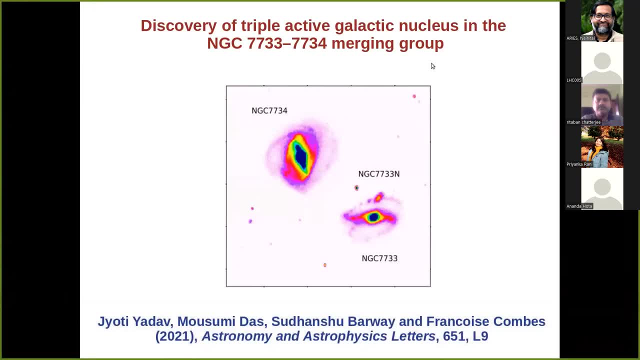 i am jyoti and first of all, i would like to thank the organizers for giving me a. to thank the organizers for giving me a. to thank the organizers for giving me a chance to present my recent work in this chance, to present my recent work in this. 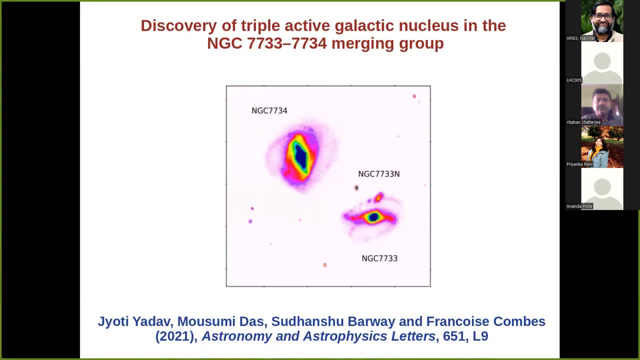 chance to present my recent work in this meeting. meeting meeting. i will discuss about my recent work on. i will discuss about my recent work on. i will discuss about my recent work on: the discovery of triple active galactic. the discovery of triple active galactic. the discovery of triple active galactic nucleus. 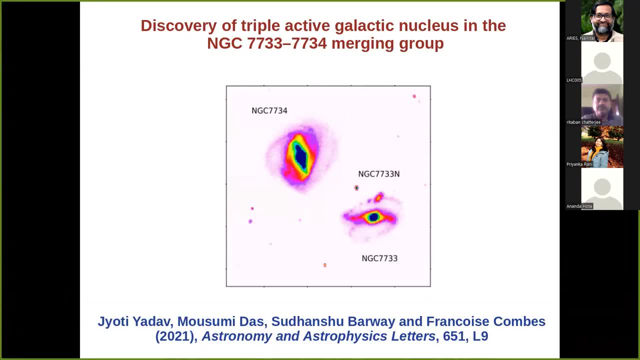 nucleus, nucleus in, and this is 7733 and 34 in, and this is 7733 and 34 in and this is 7733 and 34 merging group and i have done this work, merging group, and i have done this work, merging group, and i have done this work with marsh midas, sudhanshu barbe and 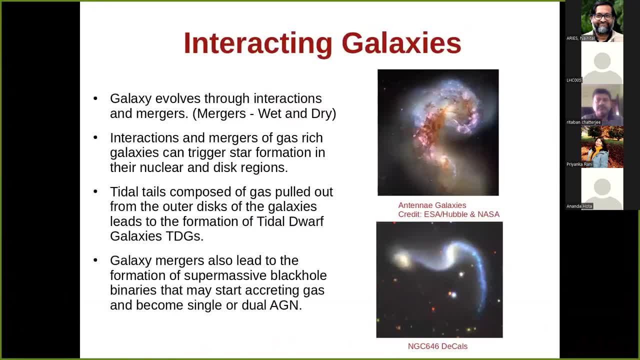 with marsh midas, sudhanshu barbe, and with marsh midas, sudhanshu barbe and french will scones. french will scones, french will scones. we know that galaxies grow through. we know that galaxies grow through. we know that galaxies grow through interactions and mergers and based on. 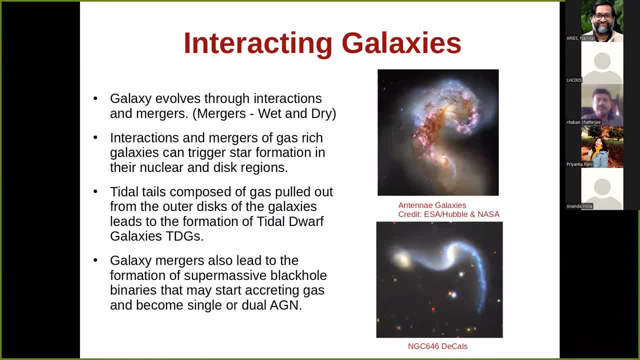 interactions and mergers. and based on interactions and mergers. and based on the gas contents in these galaxies. they the gas contents in these galaxies. they the gas contents in these galaxies. they have been classified as. have been classified as have been classified as mergers, if the galaxies are gas rich. 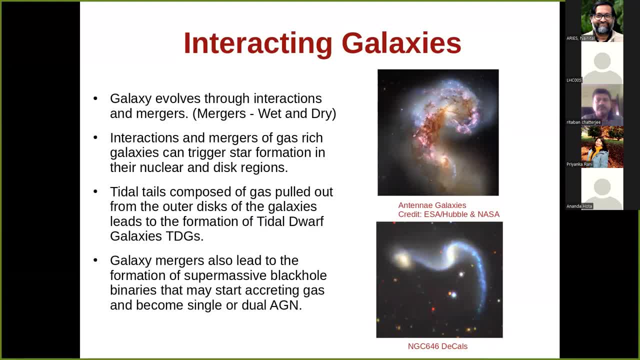 mergers. if the galaxies are gas rich mergers. if the galaxies are gas rich and dry mergers. if the galaxies are gas and dry mergers. if the galaxies are gas and dry mergers. if the galaxies are gas, poor, poor, poor. when the galaxies interact with each other. 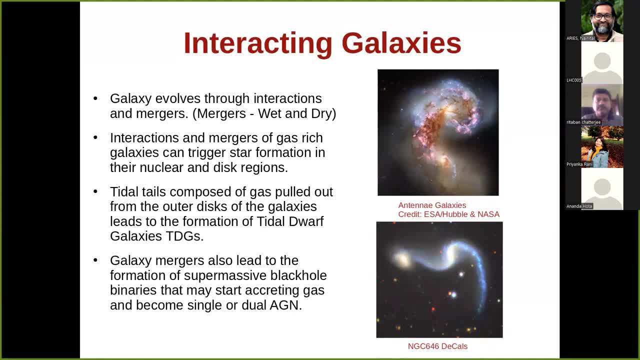 when the galaxies interact with each other. when the galaxies interact with each other, they exert tidal forces on each other. they exert tidal forces on each other. they exert tidal forces on each other, which could lead to cloud compression, which could lead to cloud compression, which could lead to cloud compression, which then triggers star formation in. 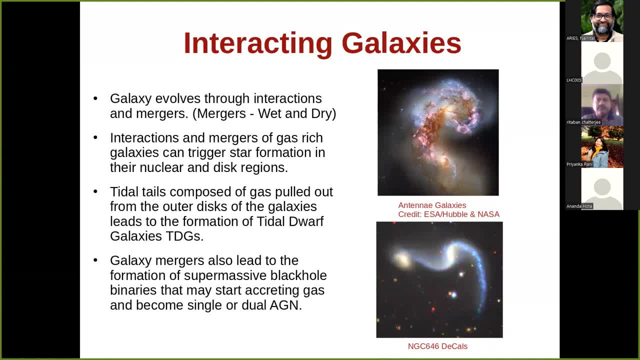 which then triggers star formation, in which then triggers star formation in their nuclear as well as in their, their nuclear as well as in their, their nuclear as well as in their experience, experience, experience during the interaction. the gas from the during the interaction, the gas from the during the interaction, the gas from the outer disk can be pulled out and it can. 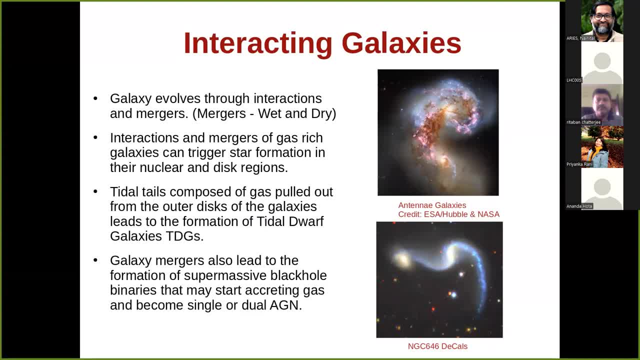 outer disk can be pulled out, and it can. outer disk can be pulled out and it can see harbors, a supermassive black hole. so see harbors, a supermassive black hole. so see harbors, a supermassive black hole. so when the galaxies come closer, the black 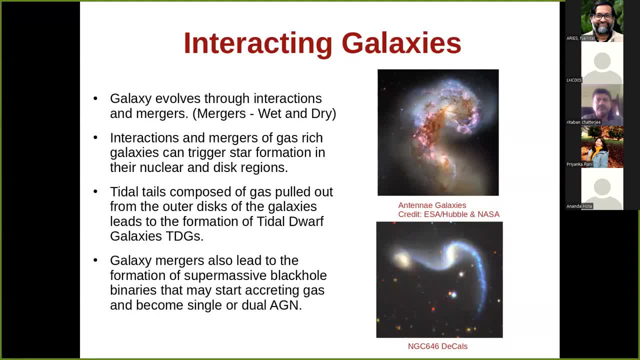 when the galaxies come closer, the black. when the galaxies come closer, the black holes also come close, which then forms holes also come close, which then forms holes also come close, which then forms supermassive black hole binaries, supermassive black hole binaries, supermassive black hole binaries. and if the black holes in these systems 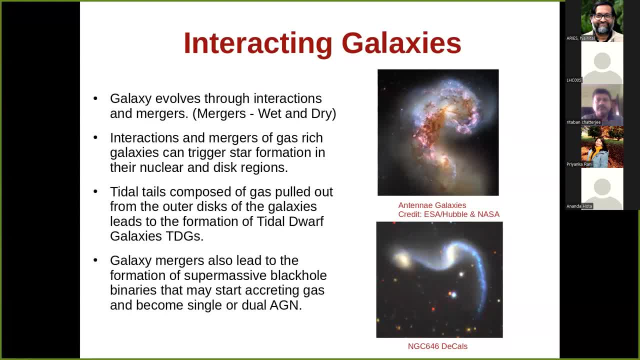 and if the black holes in these systems, and if the black holes in these systems start creating gas, they can form single start creating gas. they can form single start creating gas. they can form single agent or double agent system. agent or double agent system, agent or double agent system. so, during the merger of two galaxies, 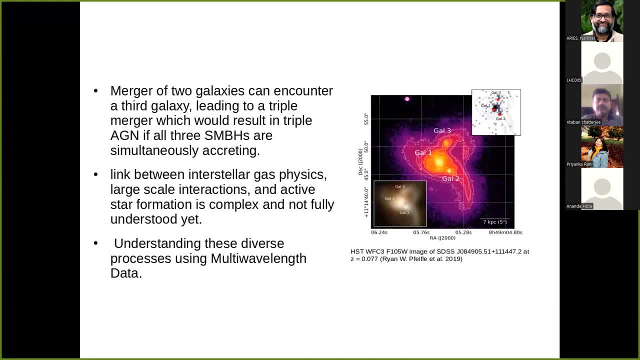 so during the merger of two galaxies. so during the merger of two galaxies, galaxies, sometimes they encounter a galaxies, sometimes they encounter a galaxies, sometimes they encounter a third galaxy. and if the black hole in third galaxy and if the black hole in third galaxy and if the black hole in that third galaxy is also aggregating, 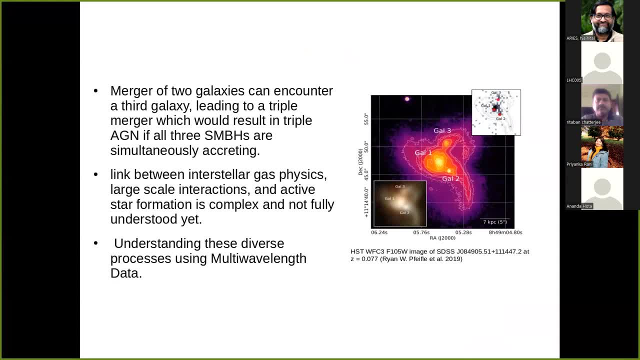 that third galaxy is also aggregating. that third galaxy is also aggregating. they form a triple agent system. they form a triple agent system. they form a triple agent system. the link between the interstellar gas, the link between the interstellar gas, the link between the interstellar gas, physics, large scale interaction and 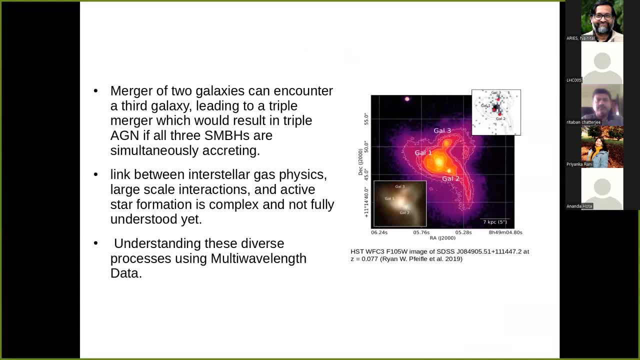 physics: large scale interaction and physics: large scale interaction and active subformation in the interacting active subformation in the interacting. active subformation in the interacting galaxies is very complex and it is not. galaxies is very complex and it is not. galaxies is very complex and it is not fully understood yet, so it is very. 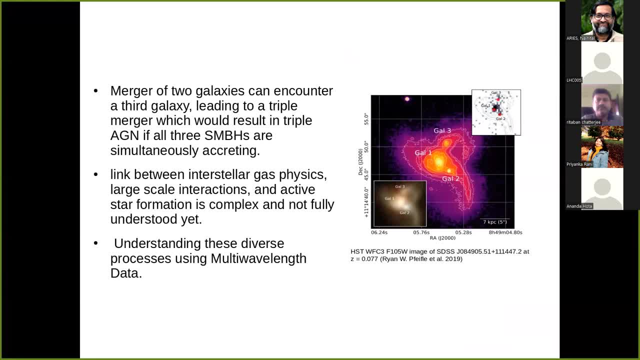 fully understood yet. so it is very fully understood yet. so it is very important to understand all these. important to understand all these, important to understand all these diverse processes using material data, diverse processes using material data, diverse processes using material data. so to do so, so to do so. 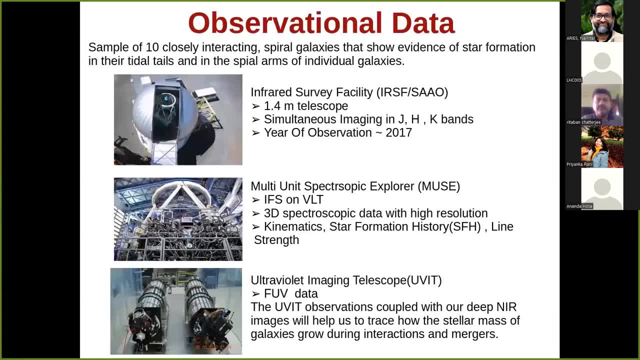 so to do so, we started a survey of 10 closely. we started a survey of 10 closely. we started a survey of 10 closely interacting southern galaxies. which interacting southern galaxies. which interacting southern galaxies. which shows evidence of star formation in. shows evidence of star formation in. 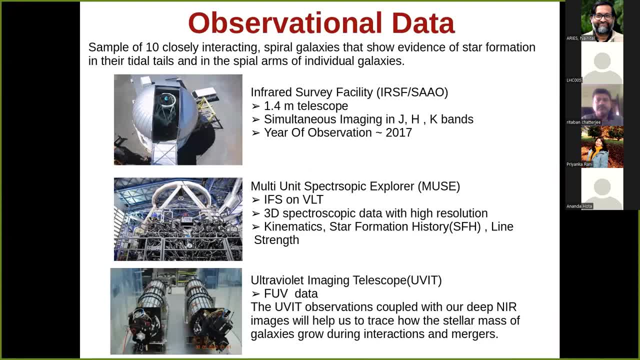 shows evidence of star formation in their tidal tips as well as the spiral, their tidal tips as well as the spiral, their tidal tips as well as the spiral arms of the individual galaxies. so we arms of the individual galaxies, so we arms of the individual galaxies. so we observe these galaxies using infrared. 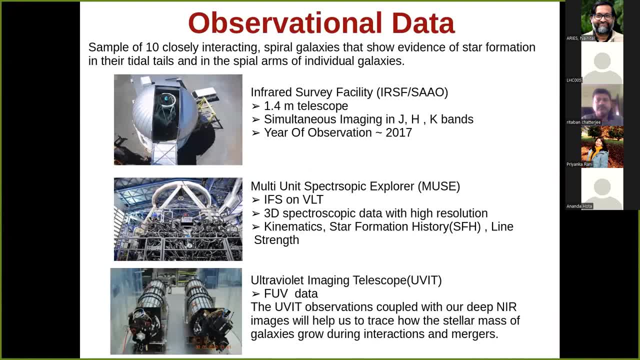 observe these galaxies using infrared. observe these galaxies using infrared survey facility telescope, which is a survey facility telescope, which is a survey facility telescope, which is a 1.4 meter telescope in south africa, 1.4 meter telescope in south africa, 1.4 meter telescope in south africa, and this telescope is capable of. 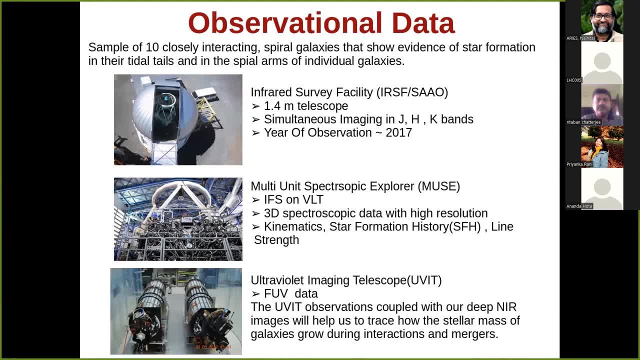 and this telescope is capable of. and this telescope is capable of simultaneous imaging in jhmk bands. simultaneous imaging in jhmk bands. simultaneous imaging in jhmk bands to study the star formation activity in. to study the star formation activity in. to study the star formation activity in these galaxies, we observed these: 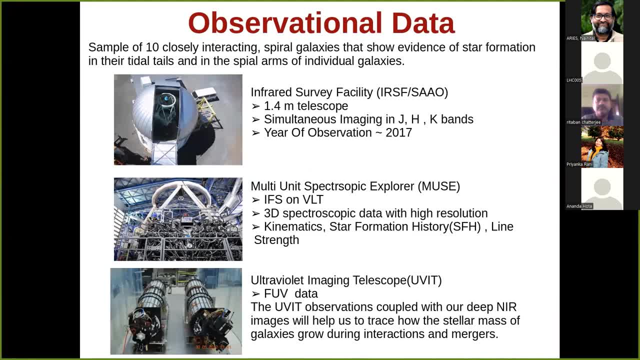 these galaxies. we observed these, these galaxies. we observed these galaxies in par ultraviolet band using galaxies in par ultraviolet band, using galaxies in par ultraviolet band using ultraviolet imaging telescope data, ultraviolet imaging telescope data, ultraviolet imaging telescope data. so the fuv data combined with our nir. 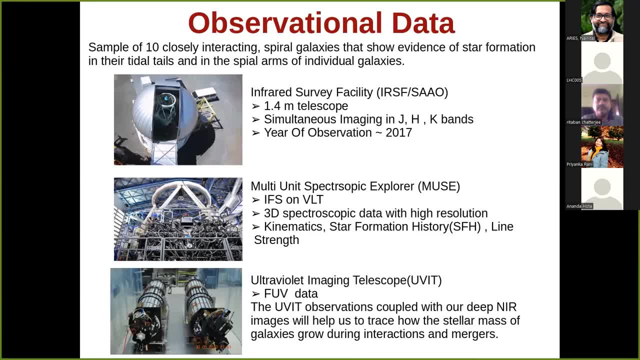 so the fuv data combined with our nir. so the fuv data combined with our nir data will help us to study how the stellar data will help us to study, how the stellar data will help us to study how the stellar masses of these galaxies grow during. 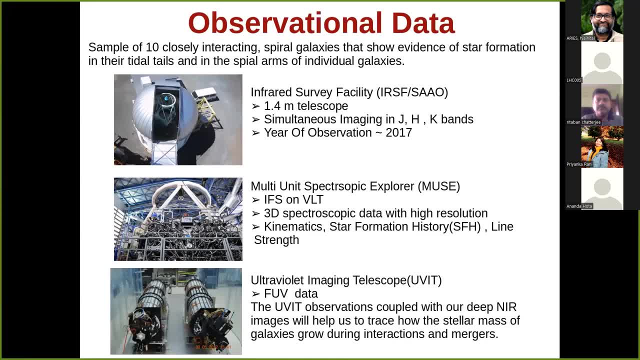 masses of these galaxies grow during. masses of these galaxies grow during interactions, and what is the effect of interactions? and what is the effect of interactions and what is the effect of interaction on the star formation? interaction on the star formation, interaction on the star formation activity in these galaxies. 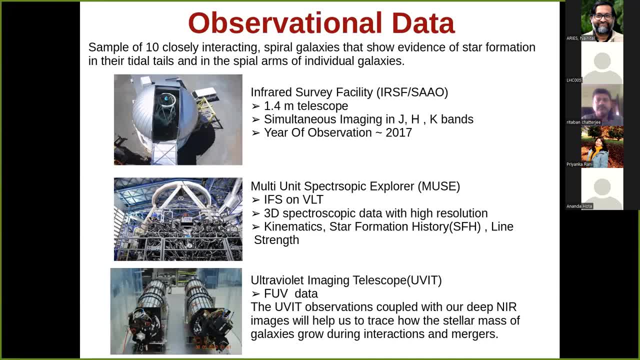 activity in these galaxies: activity in these galaxies. we also found archival news data for. we also found archival news data for we also found archival news data for these galaxies and news is an these galaxies and news is an these galaxies and news is an individual field spectrograph on very 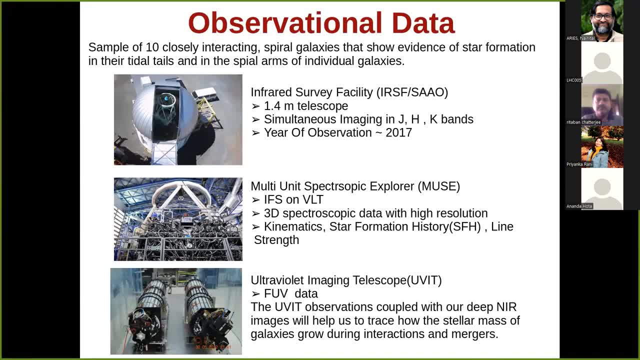 individual field spectrograph on very individual field spectrograph on very large telescope and news provides 3d large telescope and news provides 3d large telescope and news provides 3d spectroscopic data with very good spectroscopic data with very good spectroscopic data with very good resolution. so, using, using news data, we 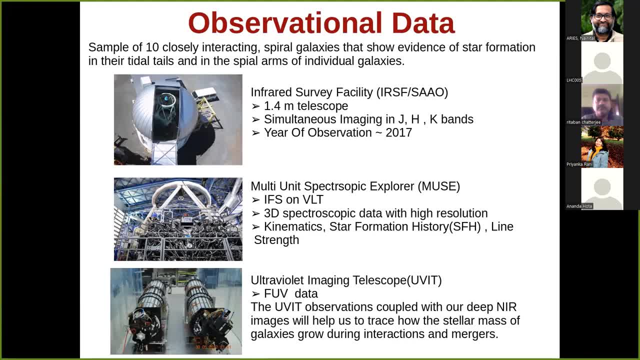 resolution. so using using news data, we resolution. so using using news data, we can get, can get, can get. gaseous kinematics, stellar kinematics, gaseous kinematics, stellar kinematics, gaseous kinematics, stellar kinematics, star formation: history line strength and star formation: history line strength and. 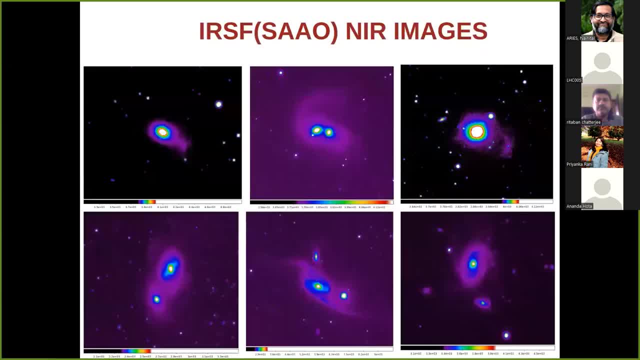 star formation, history line strength and many other properties of the galaxy, many other properties of the galaxy, many other properties of the galaxy. so these are the another images of some. so these are the another images of some. so these are the another images of some of the galaxies in our sample and from 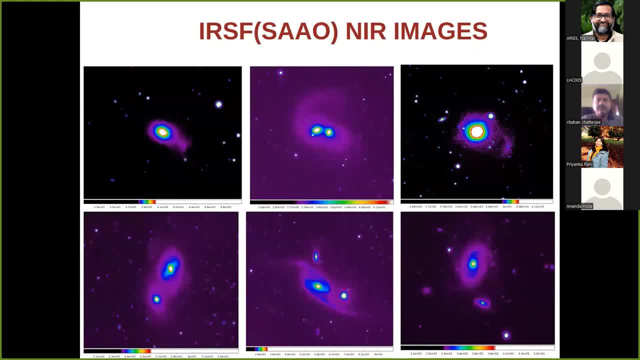 of the galaxies in our sample and from of the galaxies in our sample and from here you can see that some of the here you can see that some of the here you can see that some of the galaxies are interacting at some distance. galaxies are interacting at some distance. 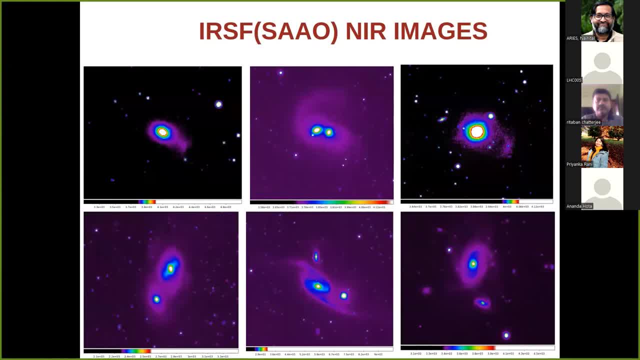 galaxies are interacting at some distance, while some of these galaxies are in the while, some of these galaxies are in the while some of these galaxies are in the advanced stage of merging. so we started advanced stage of merging. so we started advanced stage of merging, so we started with the galaxy. and this is seven, seven. 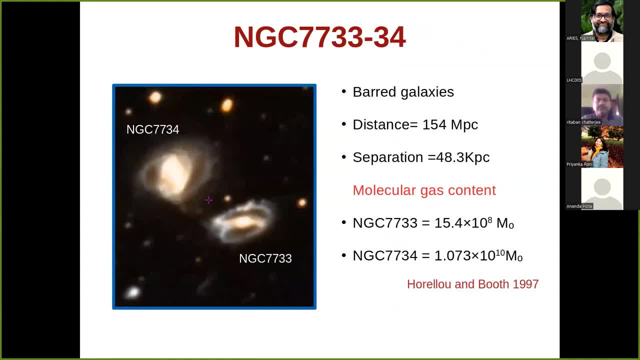 with the galaxy, and this is seven. seven with the galaxy, and this is seven, seven, three, three and three, four, and here the three, three and three, four, and here the three, three and three, four. and here the left image shows the left image shows the left image shows the interacting galaxies, and this is seven. 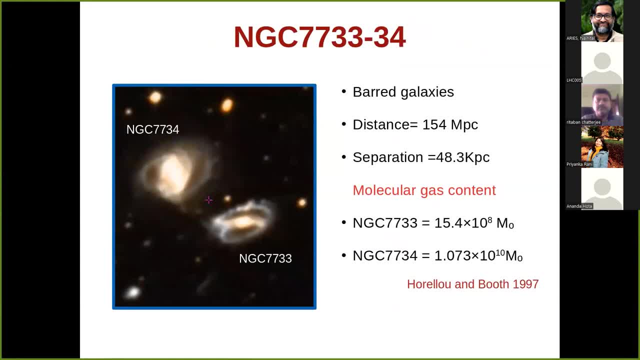 interacting galaxies and this is seven interacting galaxies and this is seven, seven three, three and three, four. so both seven three, three and three four. so both seven three, three and three four. so both the galaxies are barred and they are at a. the galaxies are barred and they are at a. 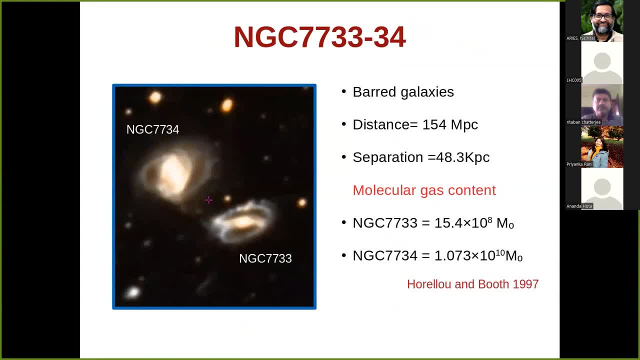 the galaxies are barred and they are at a distance of around 150 megaparsec and distance of around 150 megaparsec, and distance of around 150 megaparsec, and these galaxies are separated by a. these galaxies are separated by a. 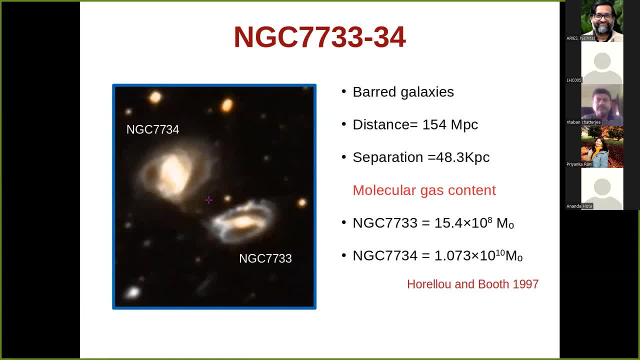 these galaxies are separated by a distance of around 48 kiloparsec, and both distance of around 48 kiloparsec and both distance of around 48 kiloparsec, and both the galaxies show molecular gas in their. the galaxies show molecular gas in their. 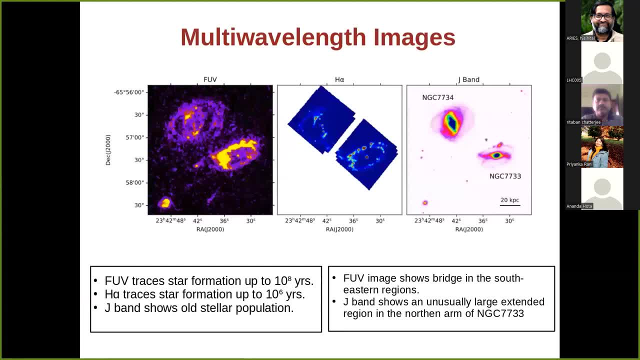 the galaxies show molecular gas in their desk. this is the middle wavelength image of this is the middle wavelength image of this is the middle wavelength image of the galaxy pair. and this is seven, seven, the galaxy pair. and this is seven, seven, the galaxy pair. and this is seven, seven, three, three and three, four. so the left. 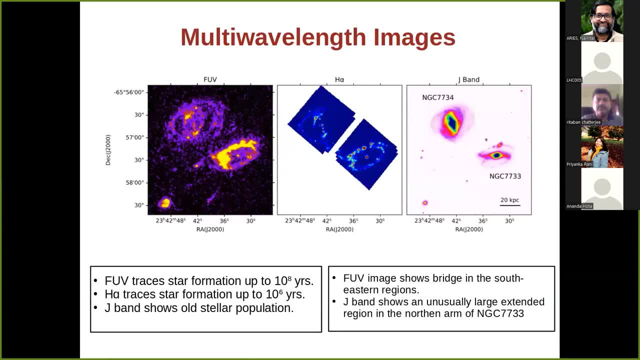 three, three and three, four. so the left: three and three, four. so the left panel shows the fubi image of the galaxy panel. shows the fubi image of the galaxy panel. shows the fubi image of the galaxy and a few will trace the star formation and a few will trace the star formation. 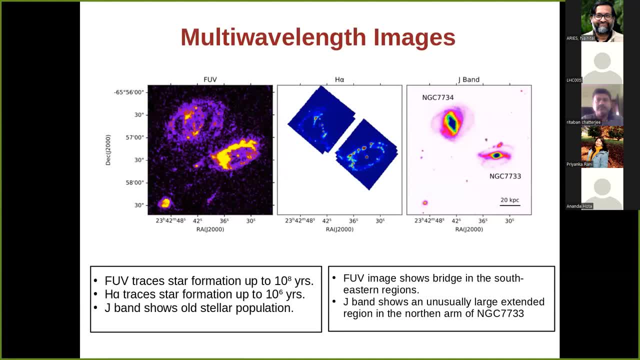 and a few will trace the star formation up to around 10 to the power eight years. up to around 10 to the power eight years. up to around 10 to the power eight years. the middle panel shows the actual image. the middle panel shows the actual image. 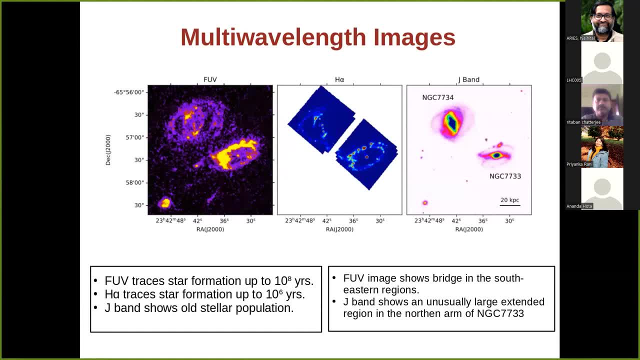 the middle panel shows the actual image of the galaxy collapsed from mu's data, of the galaxy collapsed from mu's data. of the galaxy collapsed from mu's data and it traces star formation up to 10 to. and it traces star formation up to 10 to. 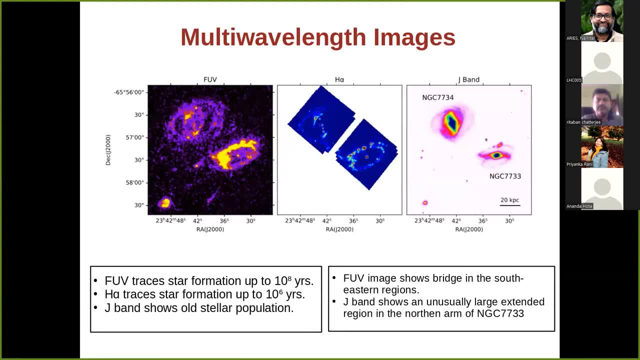 and it traces star formation up to 10 to the power. six years, so both the fuv and the power. six years, so both the fuv and the power. six years, so both the fuv and hl5 image. shows that hl5 image shows that hl5 image shows that these galaxies are going through an 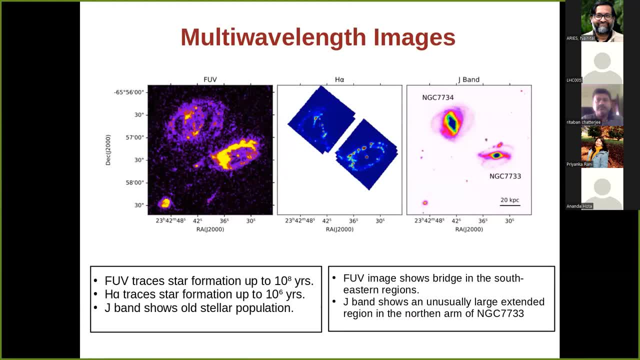 these galaxies are going through an. these galaxies are going through an ongoing recent massive star formation and ongoing recent massive star formation and ongoing recent massive star formation. and the right panel shows the j-band image. the right panel shows the j-band image. the right panel shows the j-band image of the galaxy and j-band releases the. 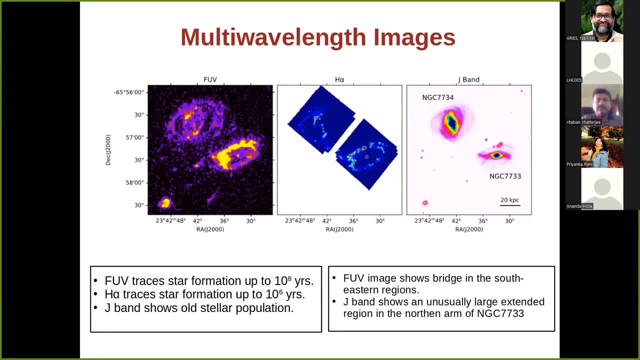 of the galaxy and j-band releases the of the galaxy and j-band releases the all-stellar population in this galaxy, all-stellar population in this galaxy, all-stellar population in this galaxy. we also notice that there is an. we also notice that there is an. 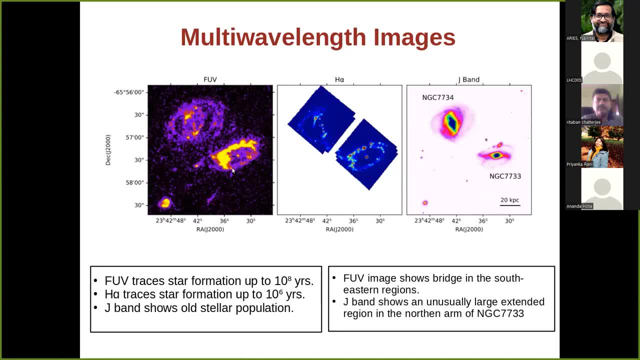 we also notice that there is an a few right clump present in the southern, a few right clump present in the southern, a few right clump present in the southern part of the galaxy. uh, and this is 7733 part of the galaxy. uh, and this is 7733. 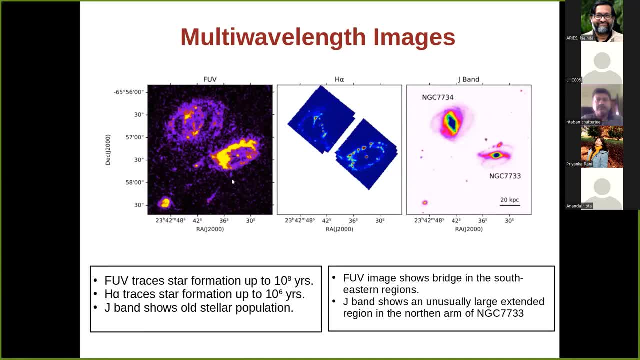 part of the galaxy. uh, and this is 7733 and it is connected to the galaxy this and it is connected to the galaxy this and it is connected to the galaxy. this is 7733 via an fub right bridge is 7733 via an fub right bridge. 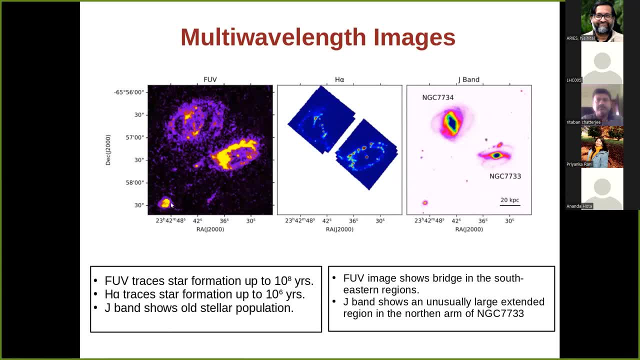 is 7733 via an fub right bridge. the redshift uh the spectroscopic data, the redshift uh the spectroscopic data, the redshift uh the spectroscopic data of this galaxy is not available. hence we of this galaxy is not available. hence, we of this galaxy is not available. hence, we could not confirm the redshift of this. 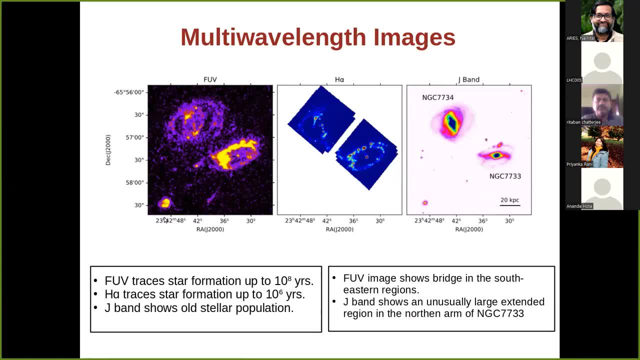 could not confirm the redshift of this, could not confirm the redshift of this source, but this could be a possible source. but this could be a possible source. but this could be a possible candidate merger with this system. candidate merger with this system, candidate merger with this system. so our aim in this study was to look at 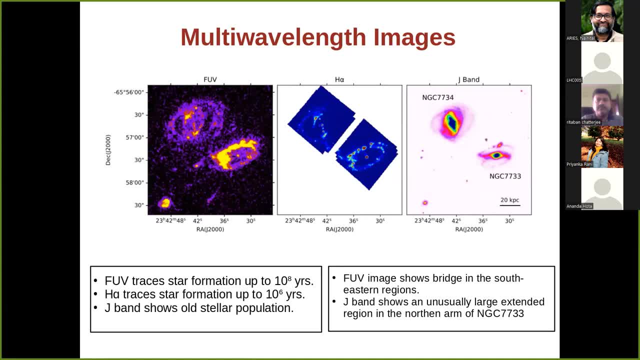 so our aim in this study was to look at. so our aim in this study was to look at the effect of interaction on the star. the effect of interaction on the star, the effect of interaction on the star, permission and agent activity in this. permission and agent activity in this. 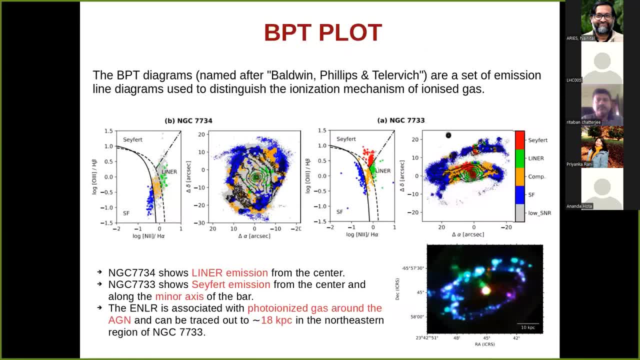 permission and agent activity in this galaxy. so to do so, galaxy. so to do so, galaxy. so to do so. we looked at the bpt diagram. so the bpt. we looked at the bpt diagram, so the bpt. we looked at the bpt diagram, so the bpt diagram was named after baldwin philip. 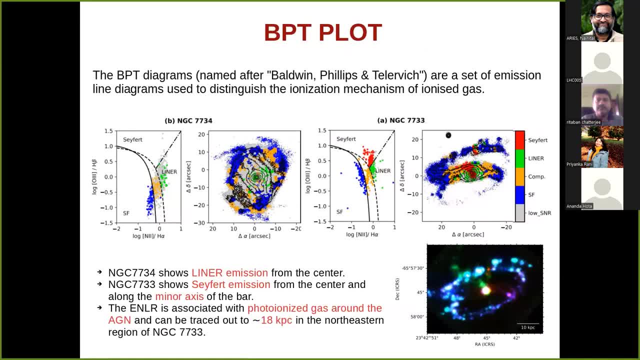 diagram was named after baldwin. philip diagram was named after baldwin, philip and talbridge and talbridge and talbridge and it is a set of emission line diagram and it is a set of emission line diagram and it is a set of emission line diagram, meaning based on the ratio of the 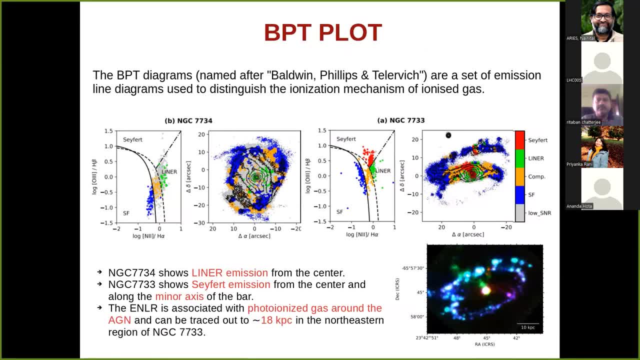 meaning, based on the ratio of the meaning, based on the ratio of the emission lines. we can tell about the emission lines, we can tell about the emission lines, we can tell about the source of ionization mechanism, of the source of ionization mechanism, of the source of ionization mechanism of the ionized gas, whether the ionized gas is. ionized gas. whether the ionized gas is ionized gas, whether the ionized gas is coming from a star forming region or coming from a star forming region, or coming from a star forming region, or whether it is coming due to a. whether it is coming due to a. 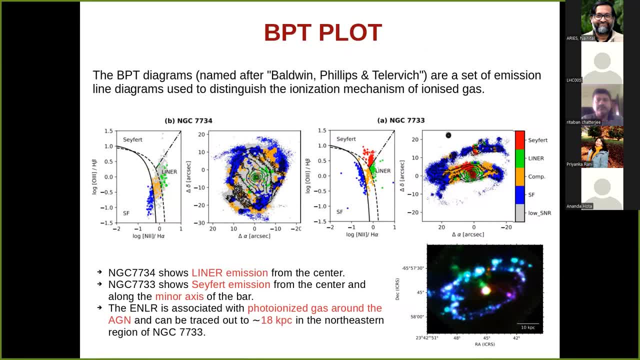 whether it is coming due to a agent. so here the left panel shows the agent. so here the left panel shows the agent. so here the left panel shows the bpt plot of the galaxy. and this is bpt plot of the galaxy. and this is bpt plot of the galaxy. and this is seven, seven, three, four. and here we see: 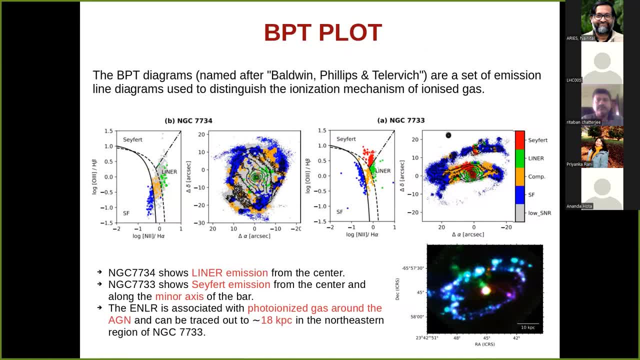 seven, seven, three, four. and here we see seven, seven, three, four. and here we see that emission from the central region, that emission from the central region, that emission from the central region, lies in the liner part of the bpt plot, lies in the liner part of the bpt plot. 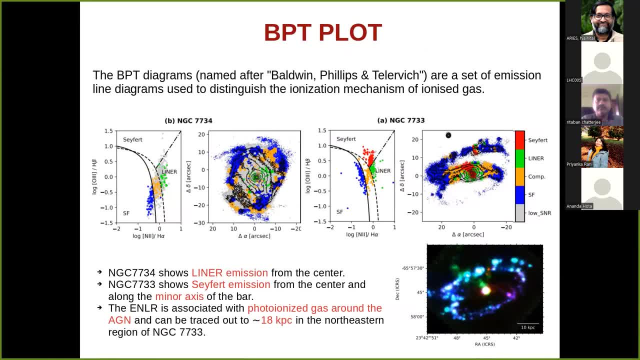 lies in the liner part of the bpt plot, which suggests that this galaxy hosts a. which suggests that this galaxy hosts a. which suggests that this galaxy hosts a liner type agent. liner type agent. liner type agent. the right panel shows the bpt plot of. the right panel shows the bpt plot of. 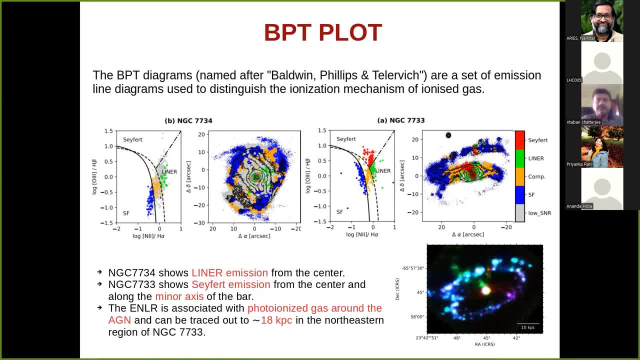 the right panel shows the bpt plot of the galaxy. and this is seven seven three the galaxy. and this is seven, seven, three the galaxy. and this is seven, seven, three, three. and here we see that the emission three and here we see that the emission three and here we see that the emission from the central region lies in the 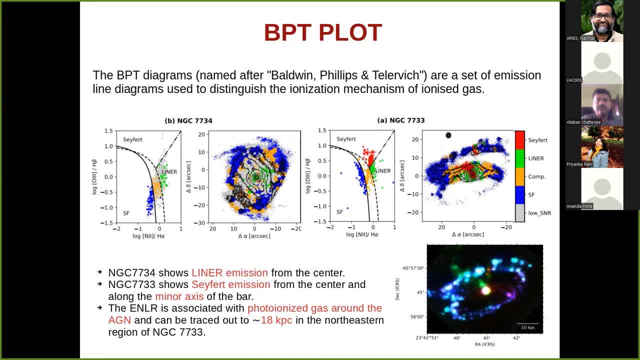 from the central region lies in the. from the central region lies in the secret region of the bpt plot. which secret region of the bpt plot. which secret region of the bpt plot which suggests that this galaxy hosts a? suggests that this galaxy hosts a. suggests that this galaxy hosts a secret type agent in the center. 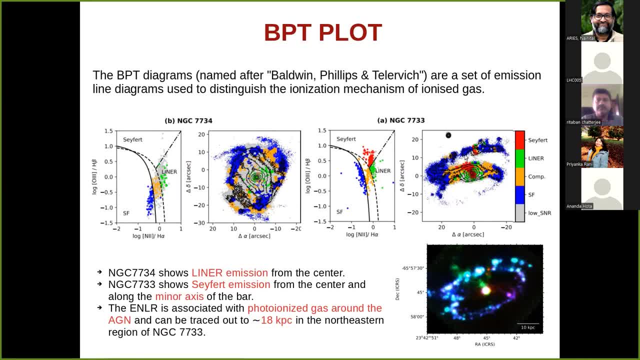 secret type agent in the center. secret type agent in the center. we also notice the secret type agent. we also notice the secret type agent. we also notice the secret type agent along the minor axis of the bar, so to along the minor axis of the bar, so to 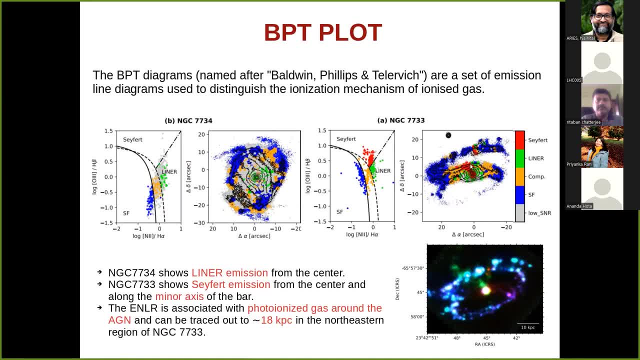 along the minor axis of the bar. so to confirm whether this safer type emission, confirm whether this safer type emission, confirm whether this safer type emission along the minor axis is actually along the minor axis is actually along the minor axis is actually associated with the agent we created a 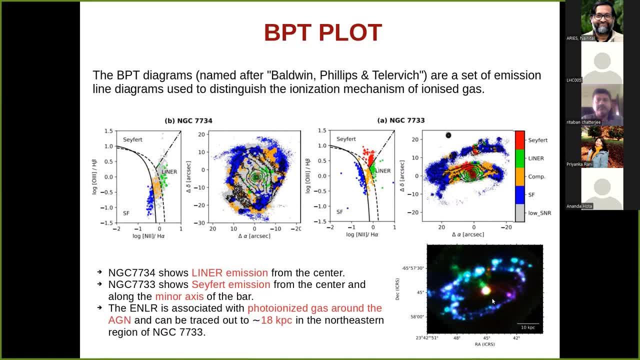 associated with the agent. we created a associated with the agent. we created a color composite image shown in the bottom color composite image shown in the bottom color composite image shown in the bottom right panel, right panel, right panel. so here the blue shows the delta image. so here the blue shows the delta image. 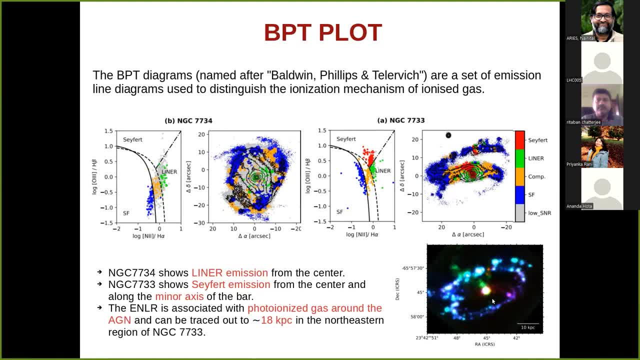 so here the blue shows the delta image and red shows the m2 and green shows the and red shows the m2 and green shows the and red shows the m2 and green shows the o3 emission. so here we see that there is o3 emission. so here we see that there is. 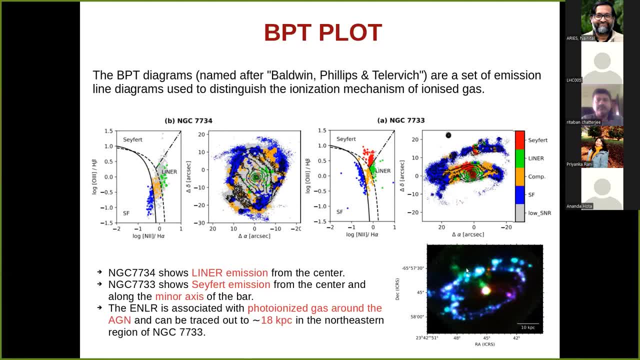 o3 emission. so here we see that there is an extended o3 emission present in the, an extended o3 emission present in the, an extended o3 emission present in the north, north, north, north eastern region of the galaxy. so north eastern region of the galaxy. so 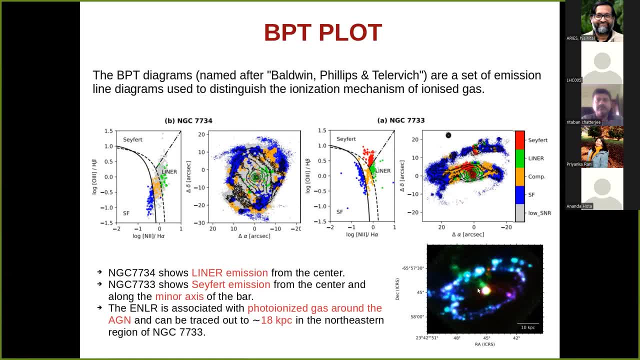 north eastern region of the galaxy. so this is, this is, this is basically an extended narrow line region, basically an extended narrow line region, basically an extended narrow line region which is associated with the photo and which is associated with the photo and which is associated with the photo and his gas around the region. and we found 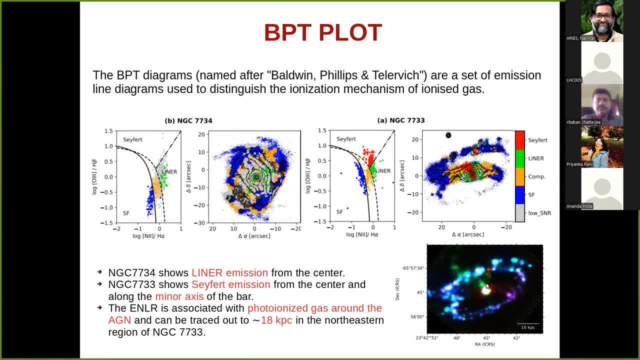 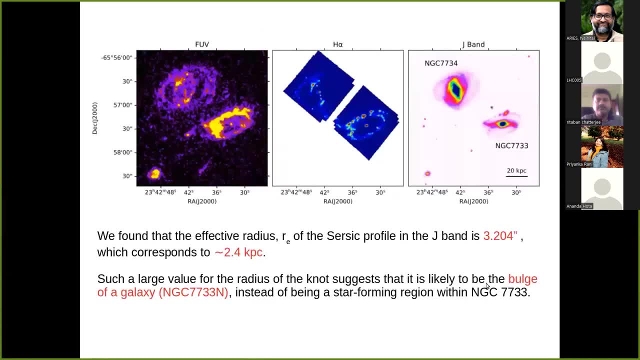 his gas around the region and we found his gas around the region and we found that the extent of this extended narrow, that the extent of this extended narrow, that the extent of this extended narrow line region is around 18 kiloparsecs, while working with this galaxy, uh, in the 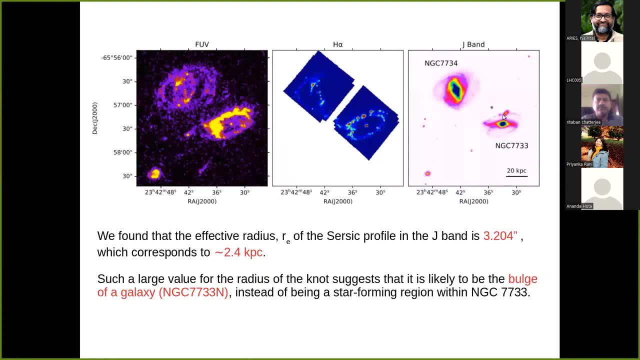 while working with this galaxy, uh, in the. while working with this galaxy, uh, in the j-band, we noticed that there is an j-band. we noticed that there is an j-band. we noticed that there is an unusually large clump present in the, unusually large clump present in the. 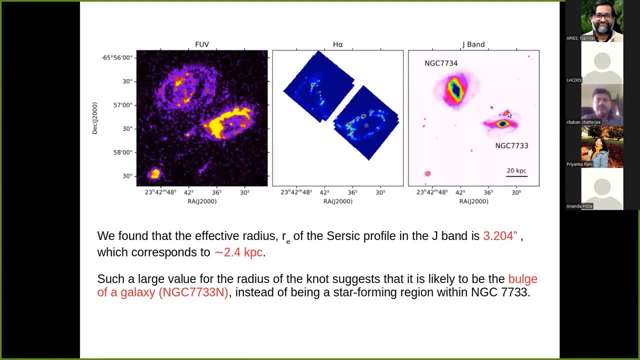 unusually large clump present in the northern arm of the galaxy and jc7733- northern arm of the galaxy and jc7733- northern arm of the galaxy and jc7733, and this clump has been identified as a. and this clump has been identified as a. 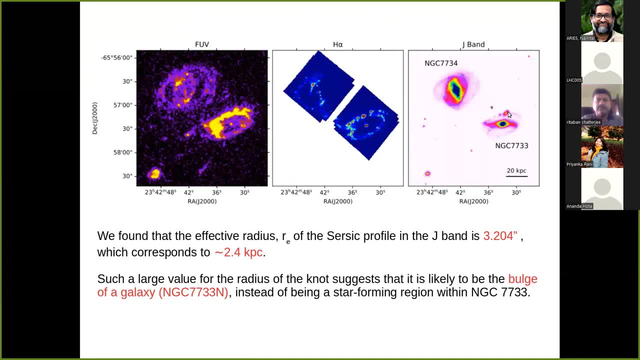 and this clump has been identified as a star forming region in the previous star forming region, in the previous star forming region, in the previous studies, studies, studies, but, and then we uh looked into this, but, and then we uh looked into this but and then we uh looked into this clump in. 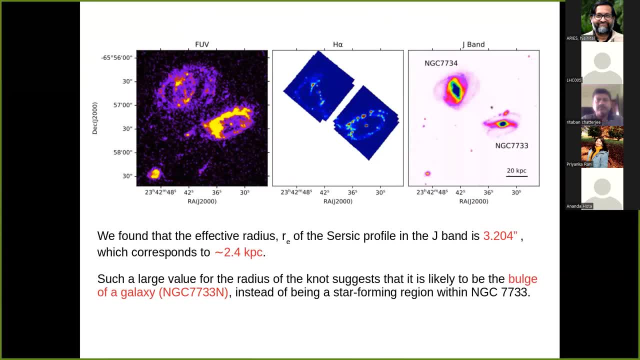 clump in clump in more details, and we did the optical more details and we did the optical more details and we did the optical decomposition of this clump and we found decomposition of this clump and we found decomposition of this clump and we found out that the effective radius of this 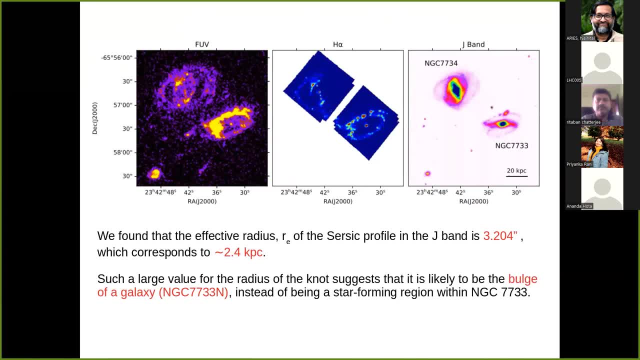 out that the effective radius of this out that the effective radius of this clump is around 3.2 arc. second, which clump is around 3.2 arc. second, which clump is around 3.2 arc. second, which corresponds to around 2.4 kiloparsec. 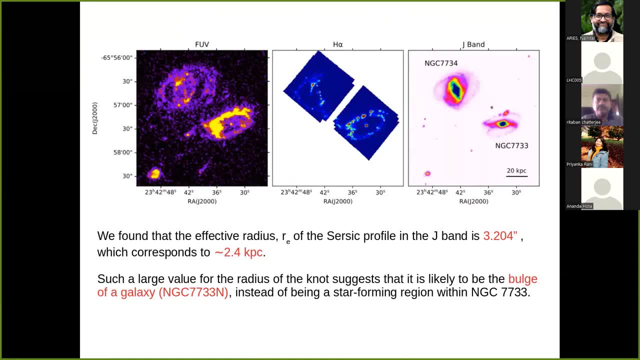 corresponds to around 2.4 kiloparsec. corresponds to around 2.4 kiloparsec. so such a large value of the radius of, so such a large value of the radius of, so such a large value of the radius of this node did not seem like. 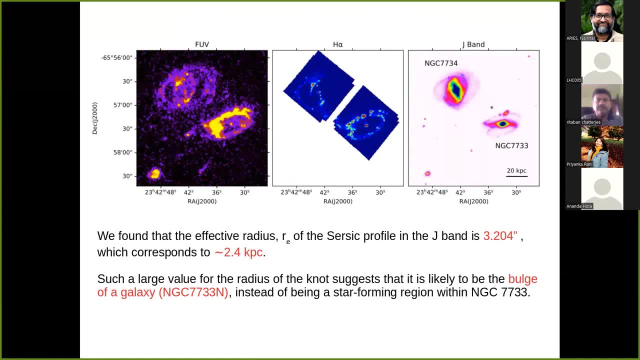 this node did not seem like this node did not seem like us to that it could be a star forming us, to that it could be a star forming us to that it could be a star forming region, but region, but region. but it suggested that it could be the bulge. 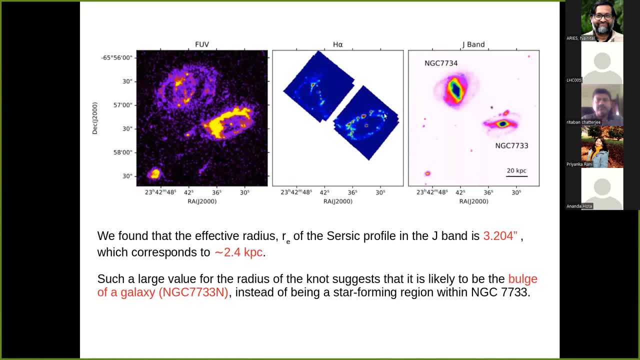 it suggested that it could be the bulge. it suggested that it could be the bulge of a galaxy, of a galaxy of a galaxy, and we also notice that there are tidal and we also notice that there are tidal and we also notice that there are tidal features associated with this. 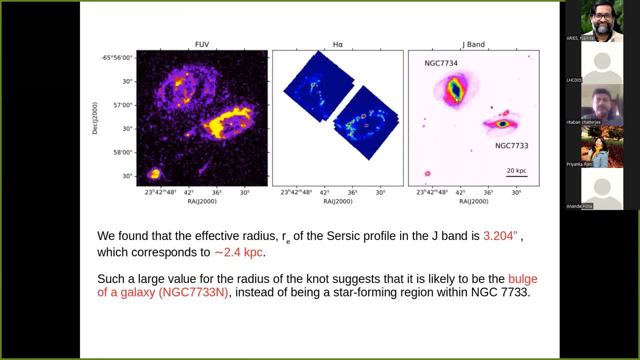 features associated with this, features associated with this club in the echelon and fuv map club in the echelon and fuv map club in the echelon and fuv map. so to confirm that, whether this clump. so to confirm that, whether this clump. 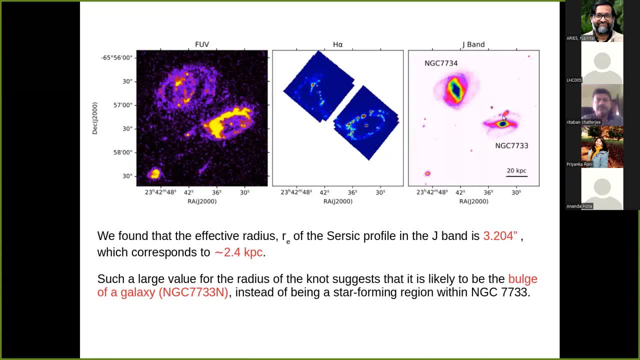 so to confirm that whether this clump is really a star forming region or it is, is really a star forming region or it is is really a star forming region or it is a separate galaxy. we looked at the, a separate galaxy. we looked at the, a separate galaxy. we looked at the velocity profile of the galaxy and jc7732. 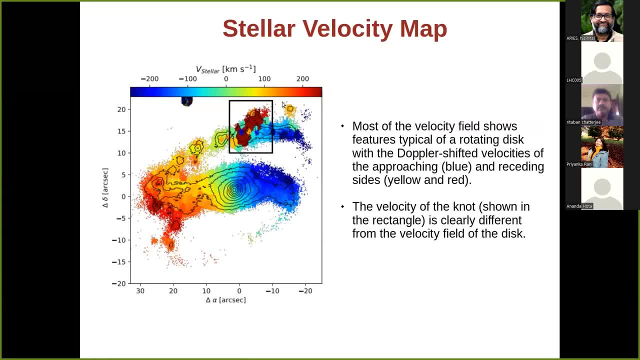 velocity profile of the galaxy and jc7732. velocity profile of the galaxy and jc7732. so here we see that most of the velocity. so here we see that most of the velocity. so here we see that most of the velocity field shows the feature of a typical 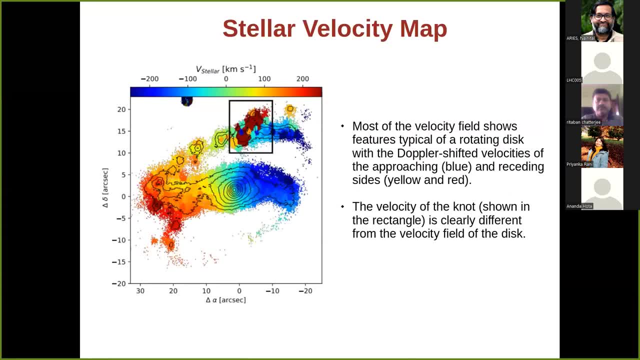 field. shows the feature of a typical field. shows the feature of a typical rotating disk with the doppler shifted rotating disk with the doppler shifted rotating disk with the doppler shifted blue and red velocities, blue and red velocities, blue and red velocities. but in the rectangle we see that the 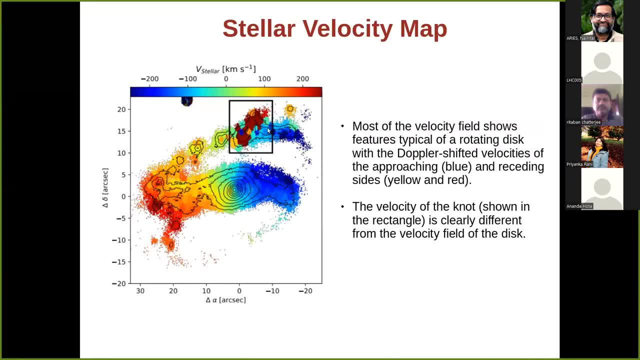 but in the rectangle we see that the but in the rectangle we see that the velocity of this knot is clearly. velocity of this knot is clearly. velocity of this knot is clearly different from the velocity field of the different from the velocity field of the different from the velocity field of the disk, which suggests that this club is not. 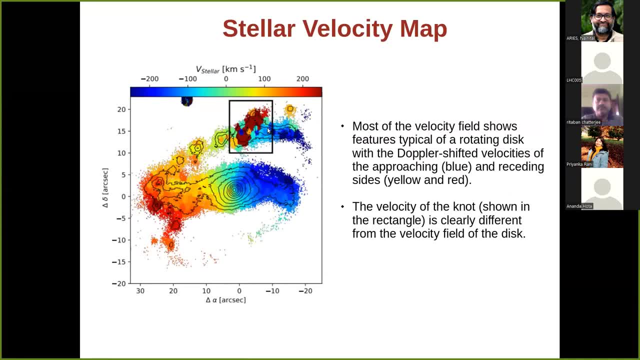 disk which suggests that this club is not. disk which suggests that this club is not a part of the galaxy, and this is 773 a part of the galaxy, and this is 773 a part of the galaxy and this is 773. rather, it is a small, separate galaxy. 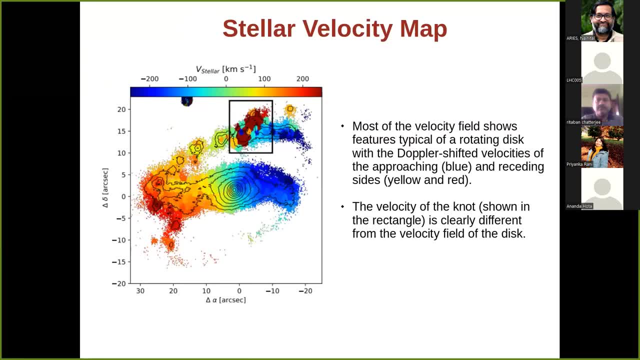 rather, it is a small separate galaxy. rather, it is a small separate galaxy which is merging with the galaxy, and this which is merging with the galaxy and this which is merging with the galaxy, and this is 733, is 733, is 733, since this object is present in the northern 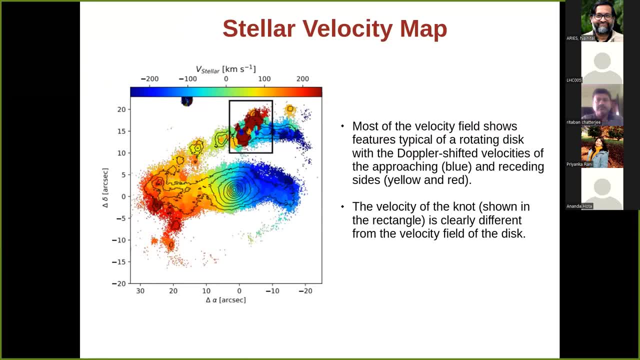 since this object is present in the northern, since this object is present in the northern arm of the galaxy, and this is 7733 we arm of the galaxy, and this is 7733 we arm of the galaxy and this is 7733- we named this object as, and this is 7733. 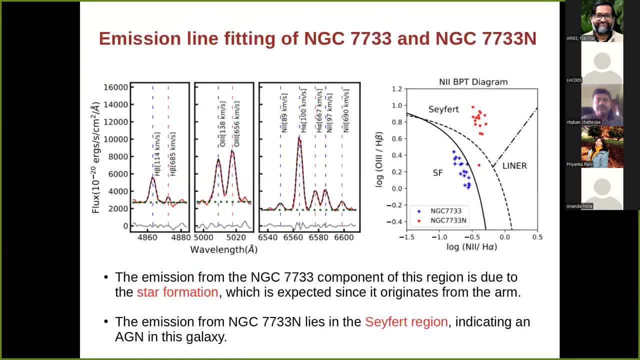 named this object as, and this is 7733. named this object as, and this is 7733 n n n. we also looked at the. we also looked at the. we also looked at the agent activity in the center of this. agent activity in the center of this. 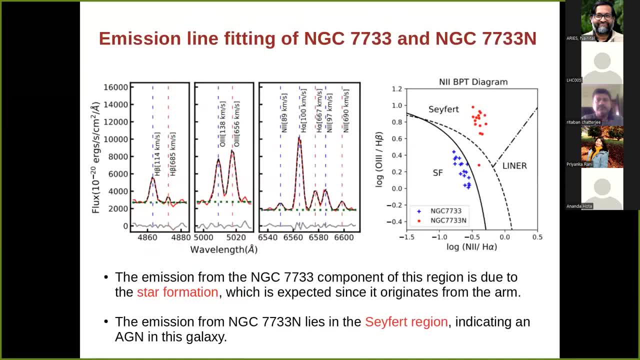 agent activity in the center of this galaxy, and this is 7733n galaxy and this is 7733n galaxy and this is 7733n. so, since this galaxy and this is 7733m, so, since this galaxy and this is 7733m. 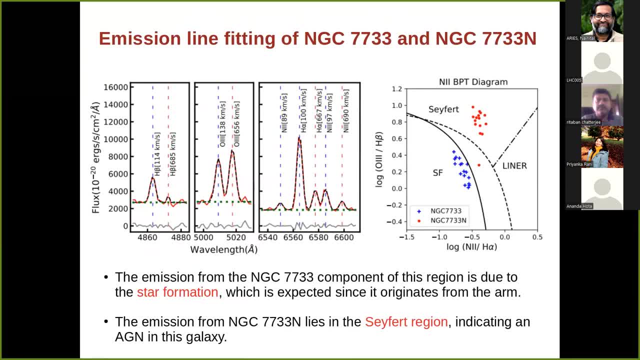 so, since this galaxy- and this is 7733m- is along the northern arm of the galaxy, is along the northern arm of the galaxy, is along the northern arm of the galaxy, and this is 7733 and this is 7733 in the emission lines we also see the 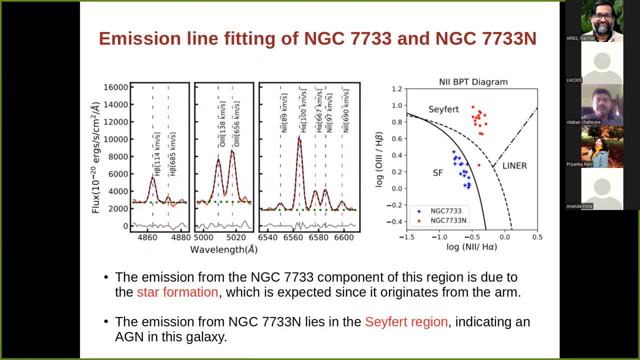 in the emission lines we also see the in the emission lines we also see the contribution from the galaxy, and this is contribution from the galaxy, and this is contribution from the galaxy, and this is 7733, 7733, 7733. so here from the figure, you can see that. 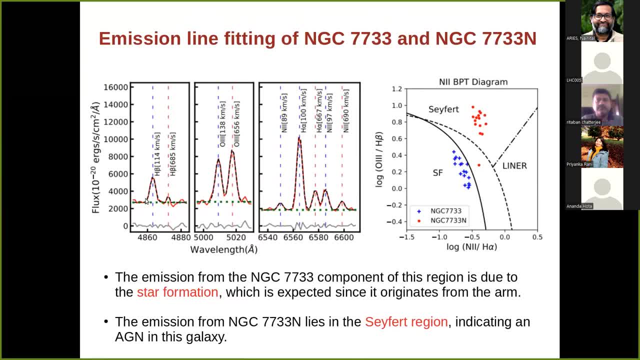 so here from the figure you can see that. so here from the figure you can see that there are two set of condition lines. so there are two set of condition lines. so there are two set of condition lines. so the blue is coming from the galaxy and the blue is coming from the galaxy and this is 7733 and the red 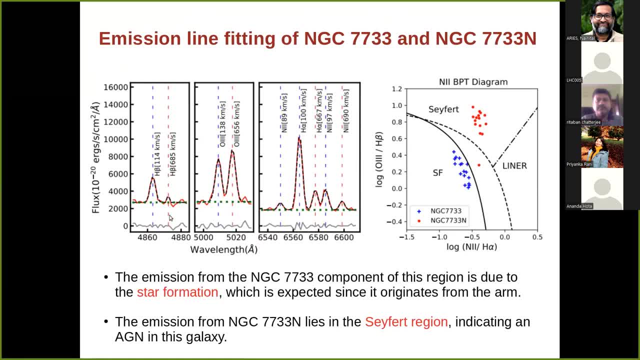 this is 7733 and the red this is 7733. and the red: uh dash line is coming from the galaxy. uh dash line is coming from the galaxy. uh dash line is coming from the galaxy and this is 7733 and this is 7733. 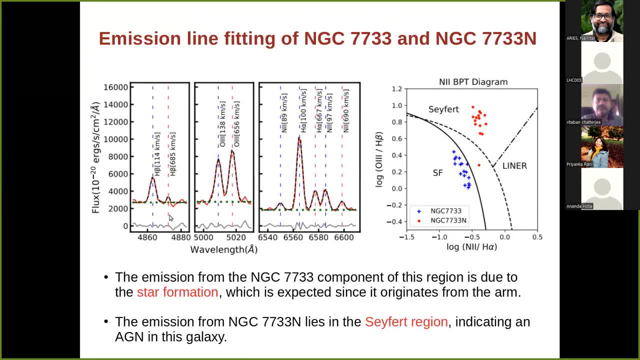 and this is 7733, and we fitted the ocean profiles in these and we fitted the ocean profiles in these and we fitted the ocean profiles in these emission lines and expected the fluxes- emission lines, and expected the fluxes, emission lines and expected the fluxes and plotted the ppt diagram. so here we. 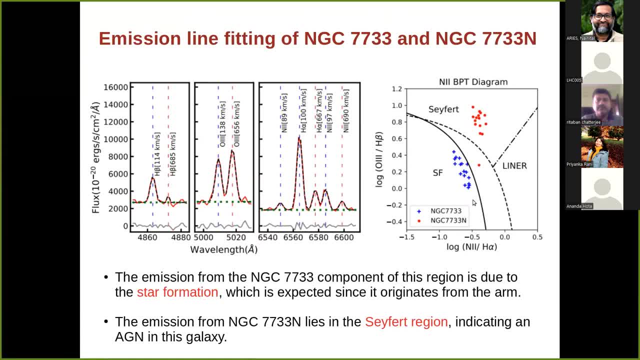 and plotted the ppt diagram. so here we. and plotted the ppt diagram. so here we. see that the contribution from the ngc, see that the contribution from the ngc, see that the contribution from the ngc: 7733 galaxy lies in the star forming. 7733 galaxy lies in the star forming. 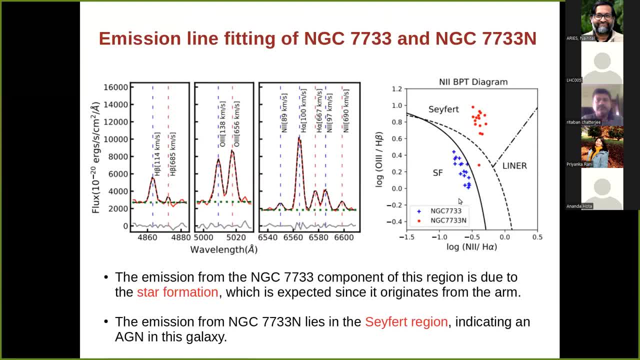 7733 galaxy lies in the star forming region, uh so which we expect because it region, uh so which we expect, because it region. uh so which we expect, because it is coming from the spiral arm and we is coming from the spiral arm, and we is coming from the spiral arm, and we expect star formation along the spiral. 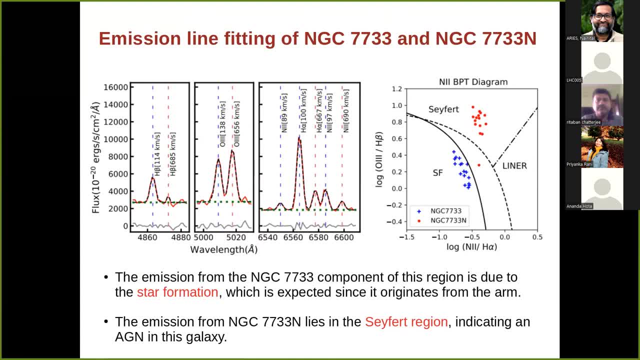 expect star formation along the spiral. expect star formation along the spiral. arm, arm, arm. well, the emission from the ngc 7733n. well, the emission from the ngc 7733n. well, the emission from the ngc 7733n lies in the 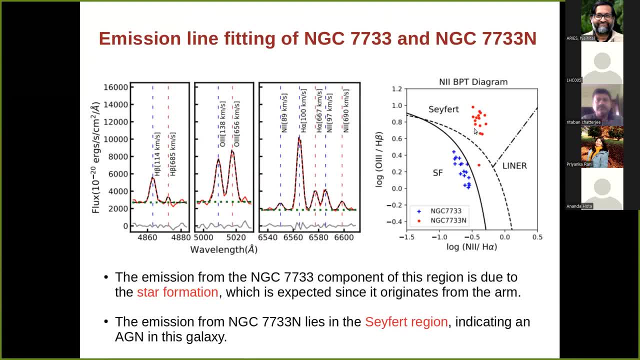 lies in the lies in the seaford region, which suggests that the seaford region, which suggests that the seaford region, which suggests that the galaxy, and this is 773 galaxy and this is 773 galaxy and this is 773 3n- also hosts an aging. hence our 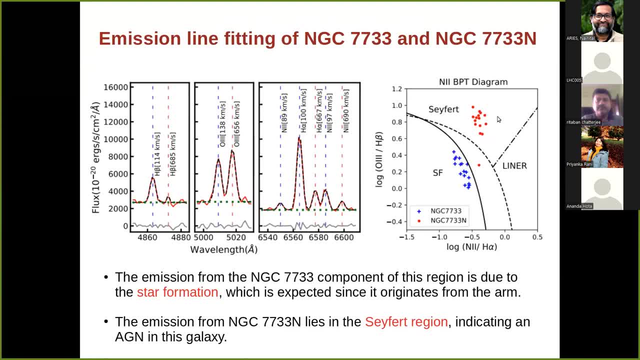 3n also hosts an aging, hence our 3n also hosts an aging. hence our triple interacting system hosts a triple interacting system, hosts a triple interacting system, hosts a triple agent, and we also looked at the triple agent and we also looked at the triple agent and we also looked at the black hole masses in this system. 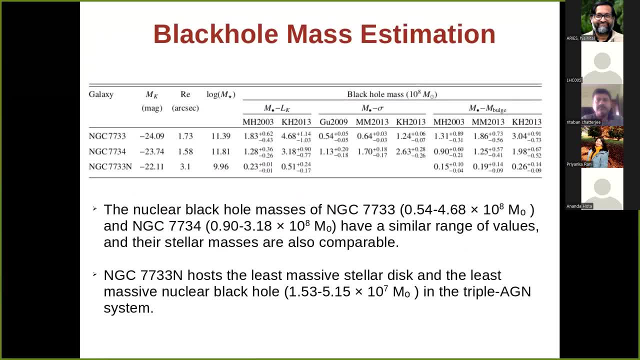 black hole masses in this system, black hole masses in this system. we found out that the black hole masses, we found out that the black hole masses, we found out that the black hole masses in the galaxies, and this is 7733, and in the galaxies, and this is 7733, and 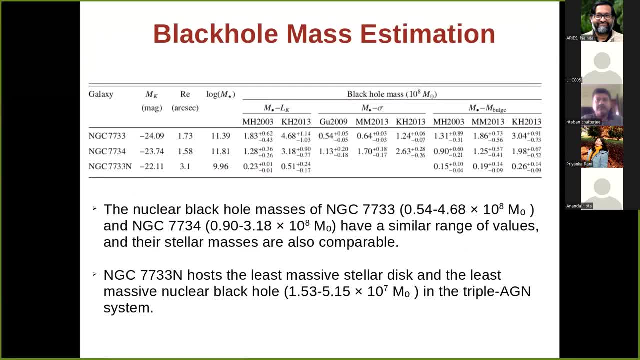 in the galaxies, and this is 7733 and 34. are have a similar range of values of 34. are have a similar range of values of 34. are have a similar range of values of around 10 to the bar eight solar mass. around 10 to the bar eight solar mass. 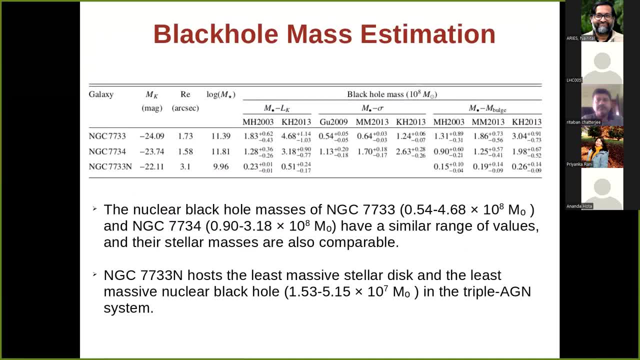 around 10 to the bar eight solar mass black hole and they also have comparable black hole and they also have comparable black hole and they also have comparable stellar masses, stellar masses, stellar masses, and this is 7733 and holds the least. and this is 7733 and holds the least. 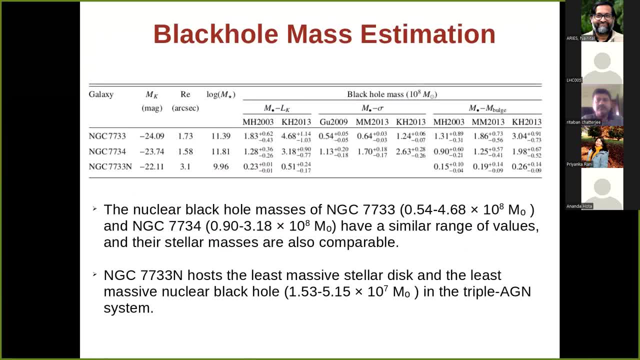 and this is 7733 and holds the least massive stellar disk and the least massive stellar disk and the least massive stellar disk and the least massive black hole, having a mass of massive black hole, having a mass of massive black hole, having a mass of around 10 to the bar seven solar mass. 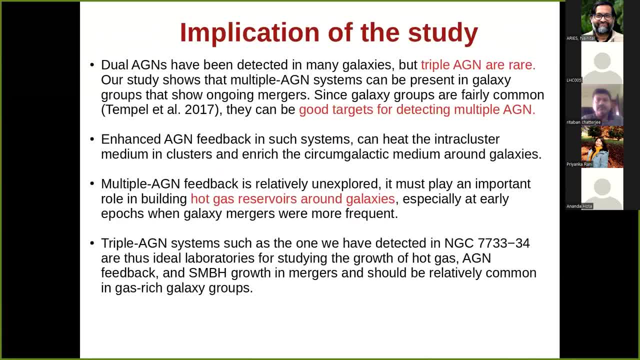 around 10 to the bar seven solar mass. around 10 to the bar seven solar mass. so these are the implications of our. so these are the implications of our. so these are the implications of our study. dual agents have been detected in study. dual agents have been detected in. 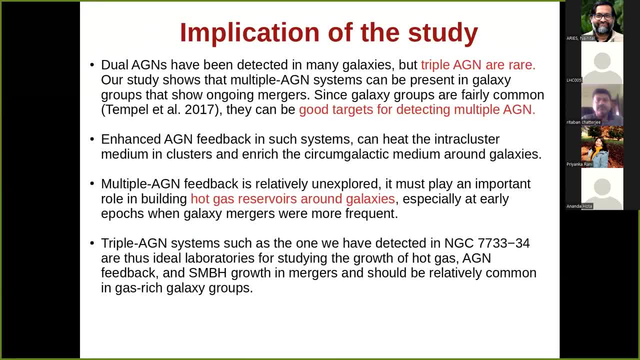 study. dual agents have been detected in many galaxies, but triple agents are rare. many galaxies, but triple agents are rare. many galaxies, but triple agents are rare and our study shows that multiple agent and our study shows that multiple agent and our study shows that multiple agent system can be present in galaxy groups. 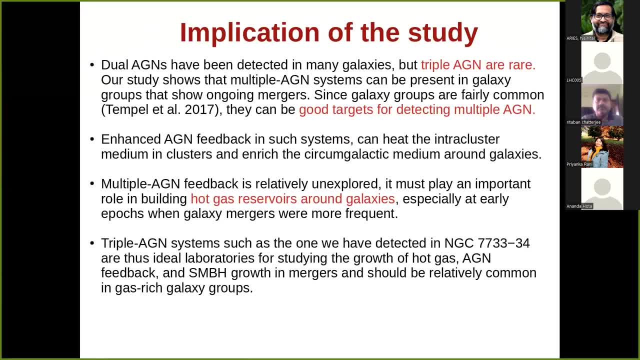 system can be present in galaxy groups. system can be present in galaxy groups that show annoying mergers and these that show annoying mergers and these that show annoying mergers. and these galaxy groups are fairly common, so they galaxy groups are fairly common. so they galaxy groups are fairly common, so they can be good targets for detecting. 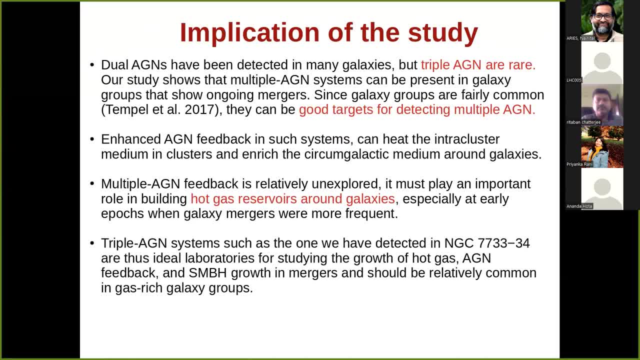 can be good targets for detecting, can be good targets for detecting multiple agents, multiple agents, multiple agents, enhanced agent feedback in galaxies- enhanced agent feedback in galaxies- enhanced agent feedback in galaxies- are relatively unexplored and it plays are relatively unexplored and it plays are relatively unexplored and it plays an important role in building both gas. 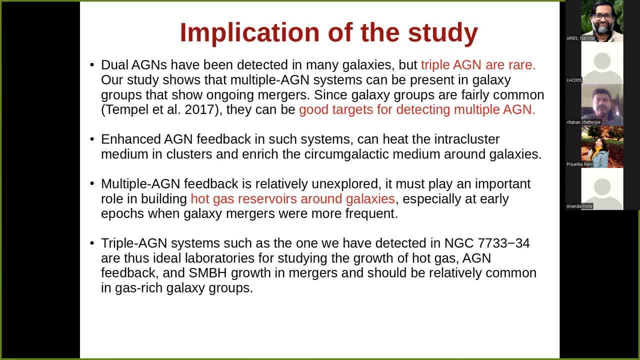 an important role in building both gas, an important role in building both gas reservoirs around galaxies, especially at reservoirs around galaxies, especially at reservoirs around galaxies, especially at early folks, when galaxy mergers were early folks, when galaxy mergers were early folks, when galaxy mergers were more frequent, and this feedback can. 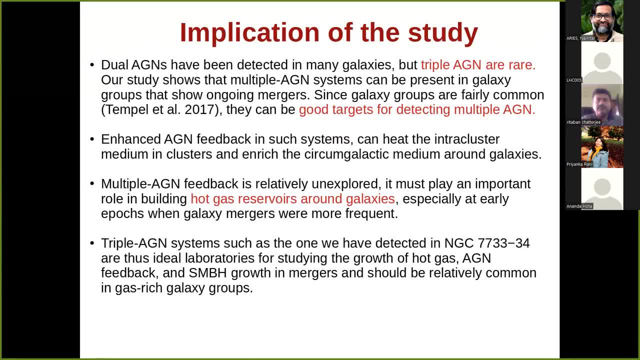 more frequent and this feedback can more frequent. and this feedback can heal the intercluster medium in clusters, heal the intercluster medium in clusters, heal the intercluster medium in clusters and can enrich the circumgalactic. and can enrich the circumgalactic and can enrich the circumgalactic medium around galaxies. 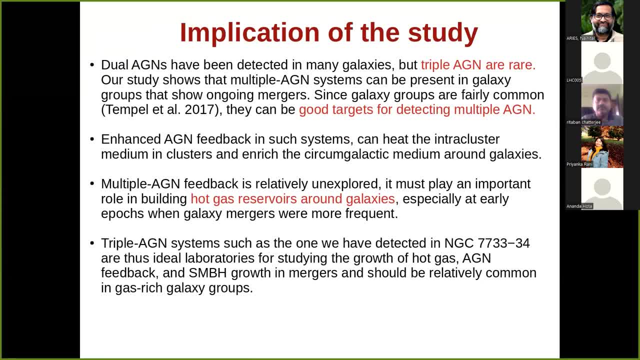 medium around galaxies. medium around galaxies, triple agent systems such as the one that triple agent systems, such as the one that triple agent systems, such as the one that we have detected in ngc7733 and 34 we have detected in ngc7733 and 34. 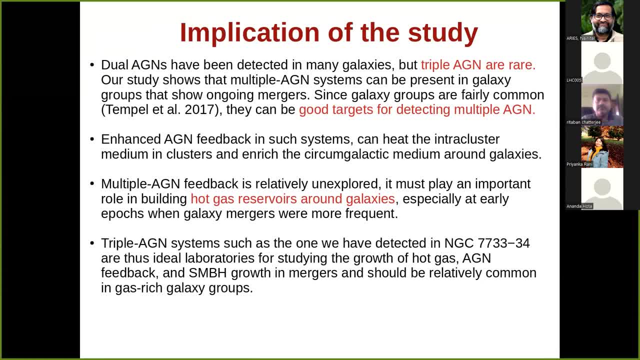 we have detected in ngc7733 and 34 are ideal laboratories for studying the are ideal laboratories for studying the are ideal laboratories for studying the growth of gas agent feedback and growth of gas agent feedback and growth of gas agent feedback and super massive black hole growth emerges. 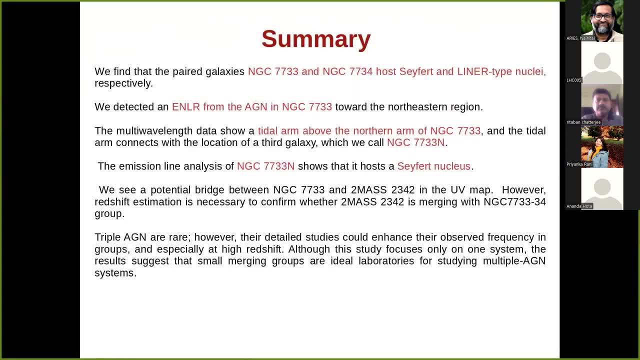 super massive black hole emerges. super massive black hole emerges and it should be relatively common in, and it should be relatively common in, and it should be relatively common in gas-rich galaxy groups. gas-rich galaxy groups. gas-rich galaxy groups. so this is the summary of our. so this is the summary of our. 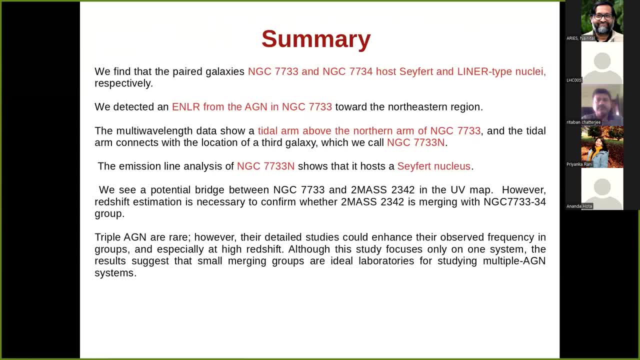 so this is the summary of our work. we found the agent activity in the work. we found the agent activity in the work. we found the agent activity in the galaxy ngc7733 and 34, galaxy ngc7733 and 34, galaxy ngc7733 and 34, and we also detected extended narrow line. 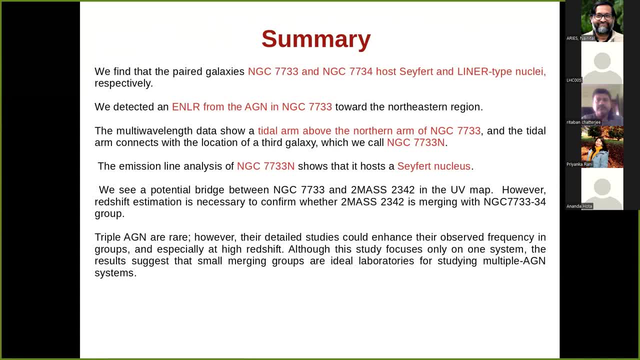 and we also detected extended narrow line. and we also detected extended narrow line region in the galaxy ngc7733 region in the galaxy ngc7733 region in the galaxy ngc7733. we also discovered a new galaxy along. we also discovered a new galaxy along. 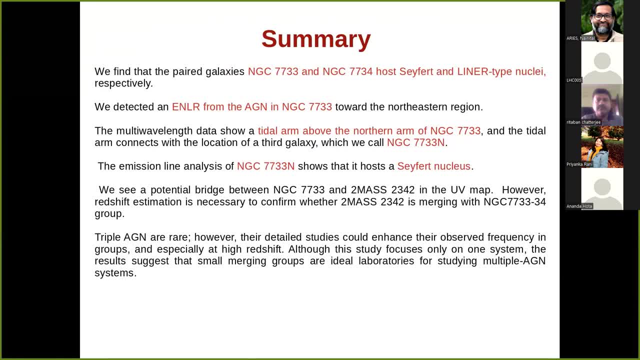 we also discovered a new galaxy along the northern arm of the galaxy and this, the northern arm of the galaxy, and this is a secret kind of is a secret kind of is a secret kind of agent. we also noticed a potential bridge agent. we also noticed a potential bridge. 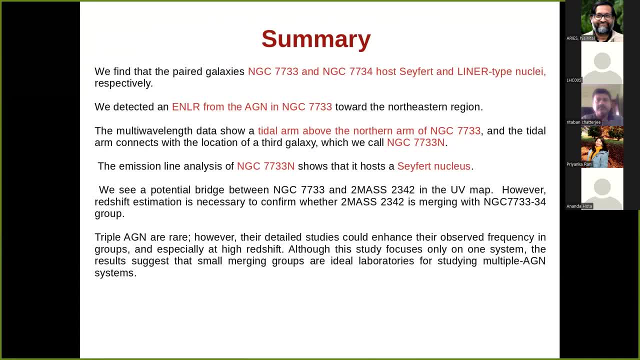 agent. we also noticed a potential bridge between the galaxy ngc7733 and two, between the galaxy ngc7733 and two, between the galaxy ngc7733 and two. marks two, three, four, two in the uv map. marks two, three, four, two in the uv map. 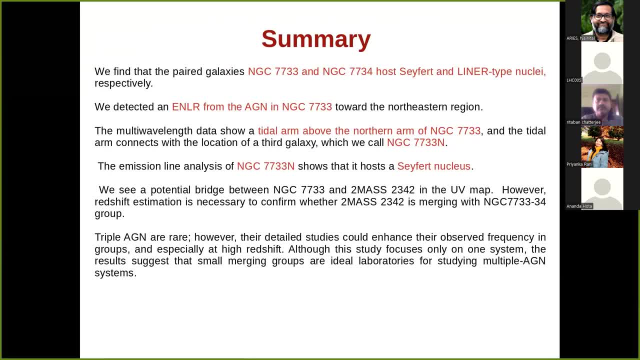 marks two, three, four, two in the uv map. however, we need rest redshift. however, we need rest redshift. however, we need rest redshift estimation to confirm whether this is estimation, to confirm, whether this is estimation, to confirm whether this is: uh, this is, this galaxy is merging with. 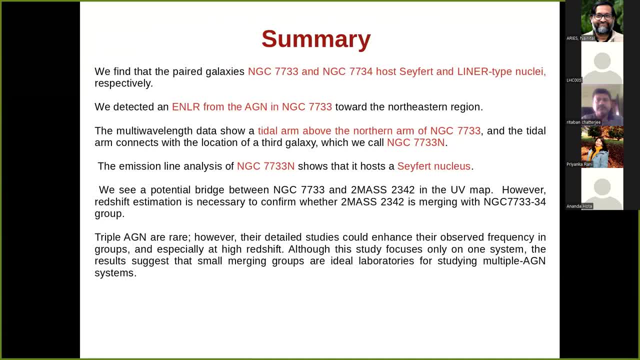 uh, this is this galaxy is merging with. uh, this is this galaxy is merging with: the galaxy ngc7733 and 34, the galaxy ngc7733 and 34, the galaxy ngc7733 and 34, and our study suggests that triple agents, and our study suggests that triple agents. 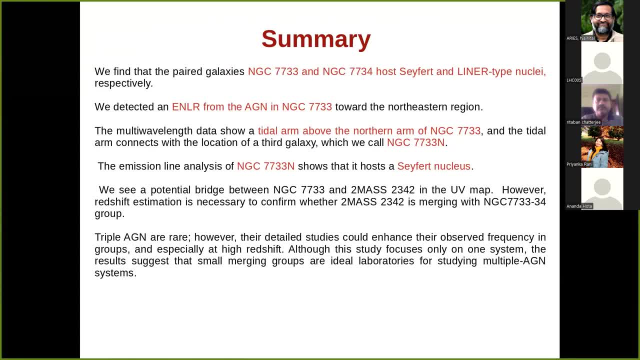 and our study suggests that triple agents are rare. however, their detailed study are rare. however, their detailed study are rare. however, their detailed study could enhance their observed frequency, could enhance their observed frequency, could enhance their observed frequency groups, and especially at higher drift groups and especially at higher drift. 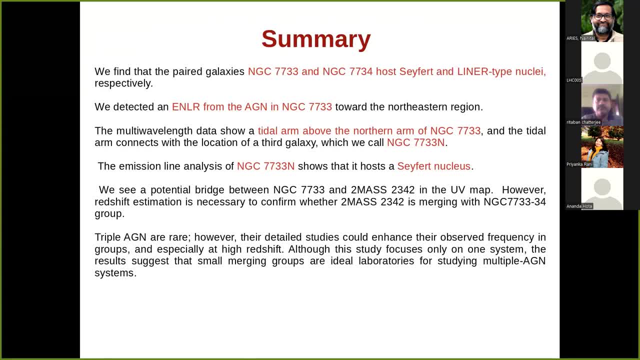 groups, and especially at higher drift. although our study focuses only on one. although our study focuses only on one, although our study focuses only on one system, the results suggest that small system. the results suggest that small system. the results suggest that small emerging groups are ideal laboratories. emerging groups are ideal laboratories. 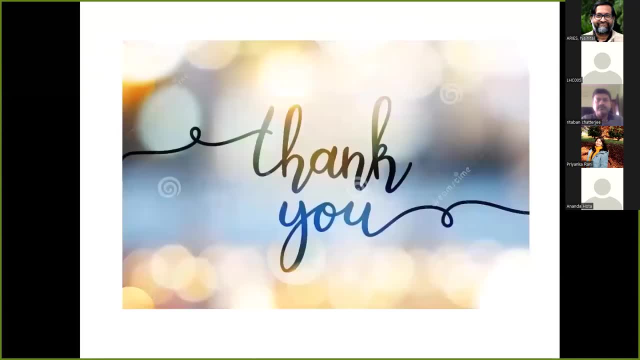 emerging groups are ideal laboratories for studying multiple agent systems. thank you, unfortunately i cannot be. thank you, unfortunately i cannot be. thank you, unfortunately i cannot be present live to answer your questions. but present live to answer your questions. but present live to answer your questions. but if you have any questions, please contact. 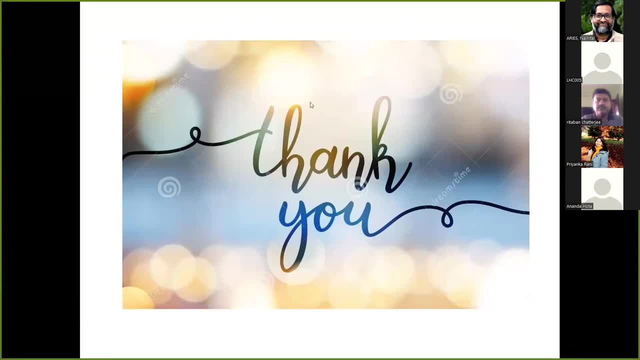 if you have any questions, please contact. if you have any questions, please contact mosh with us. mosh with us. mosh with us. or feel free to post your questions on, or feel free to post your questions on, or feel free to post your questions on slack. i will be happy to answer your. 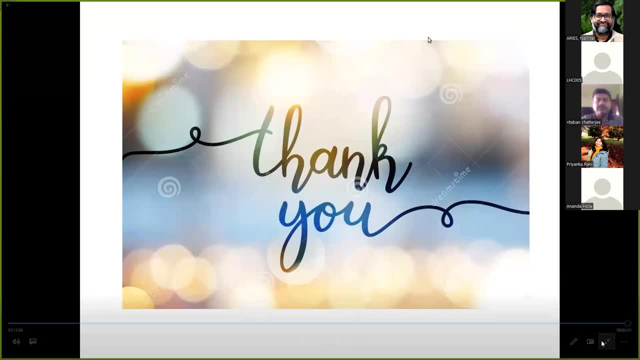 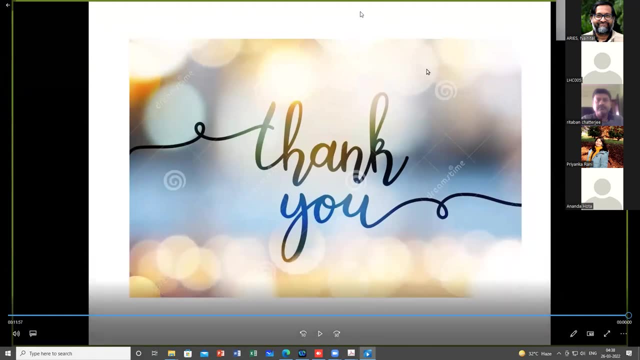 slack. i will be happy to answer your slack. i will be happy to answer your questions. okay, so, thank you, volunteers for playing. okay, so, thank you, volunteers for playing. okay, so, thank you, volunteers for playing the video. the video, the video and i think, as she explained, if you have, 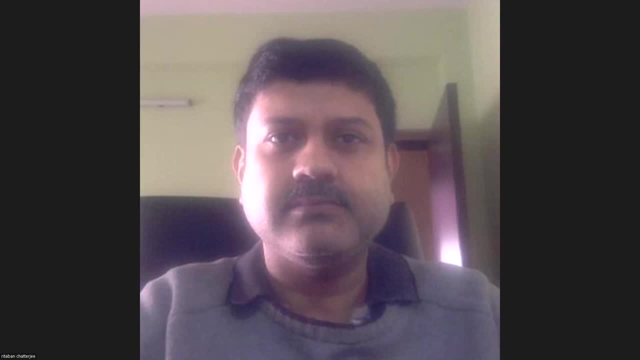 and i think, as she explained, if you have, and i think, as she explained, if you have any question, you should any question. you should any question, you should write to her in the slack channel. or if write to her in the slack channel, or if write to her in the slack channel, or if you are in the conference, you can talk. 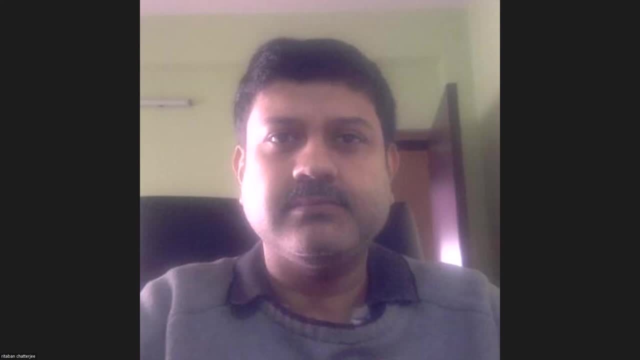 you are in the conference, you can talk. you are in the conference, you can talk to, to, to, uh her collaborator. uh professor mo, uh her collaborator, uh professor mo, uh her collaborator, uh professor mo, sumidash, sumidash, sumidash. um, okay, so let's move on to the next talk. 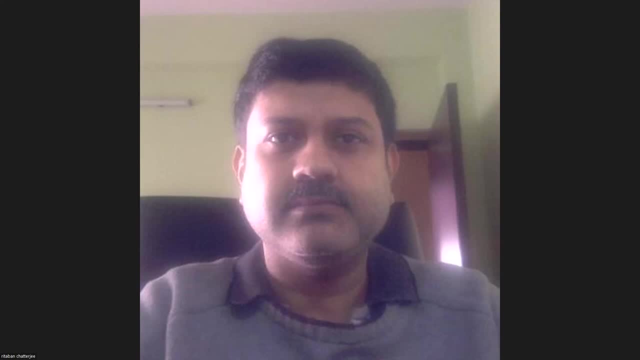 um, okay, so let's move on to the next talk. um, okay, so let's move on to the next talk, which is by krishna mahona, which is by krishna mahona, which is by krishna mahona, and the title of the talk is long-term. 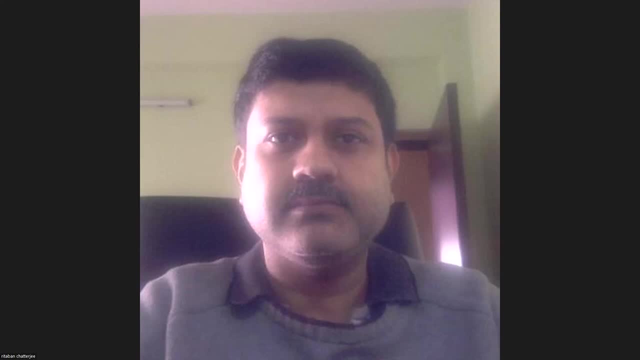 and the title of the talk is long-term. and the title of the talk is long-term- multi-band monitoring of laser. multi-band monitoring of laser. multi-band monitoring of laser- 3c66a, 3c66a, 3c66a- evidence of the two distinct states with 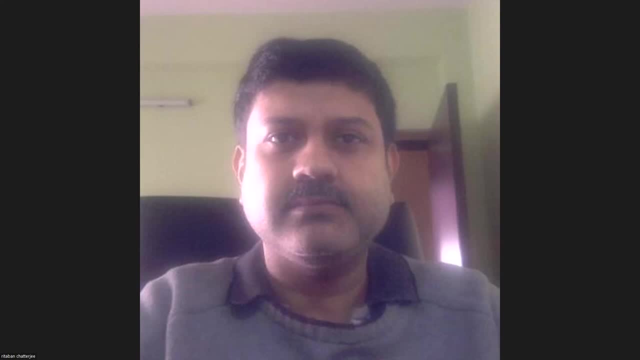 evidence of the two distinct states with evidence of the two distinct states with different baseline flux. different baseline flux, different baseline flux. so, krishna mohana, could you please uh. so, krishna mohana, could you please uh. so, krishna mohana, could you please uh, share your. can you hear me? 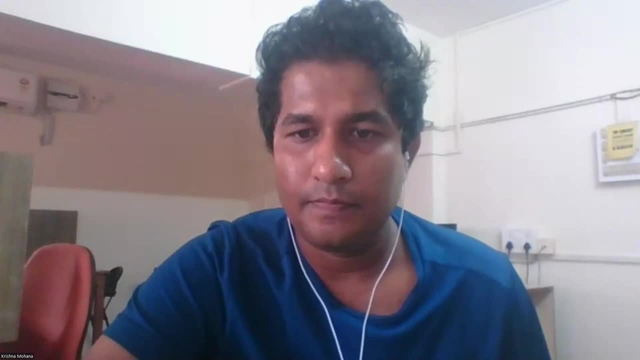 share your. can you hear me share your. can you hear me? yes, i can hear you. i will share the. yes, i can hear you. i will share the. yes, i can hear you. i will share the screen. screen screen. yes, please, yes, please, yes, please yes. we can see the screen now. 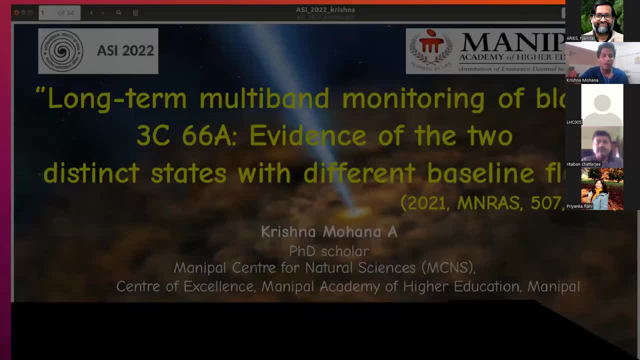 yes, we can see the screen now. yes, we can see the screen now. yes, we can see the presentation. yes, we can see the presentation. yes, we can see the presentation. okay, okay, okay, okay. good evening to all i am krishna. good evening to all i am krishna. 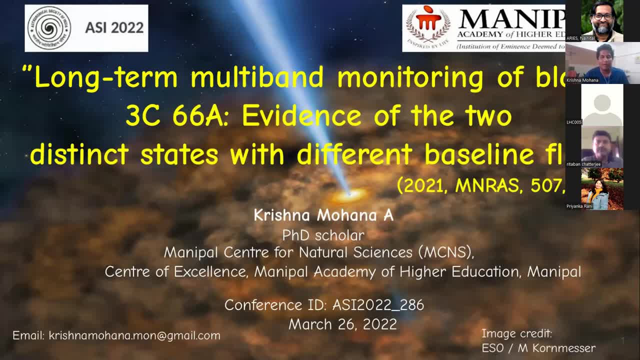 good evening to all. i am krishna mohana, mohana mohana. finally a phd student at manipal, finally a phd student at manipal, finally a phd student at manipal center for natural sciences, which is center for natural sciences, which is. 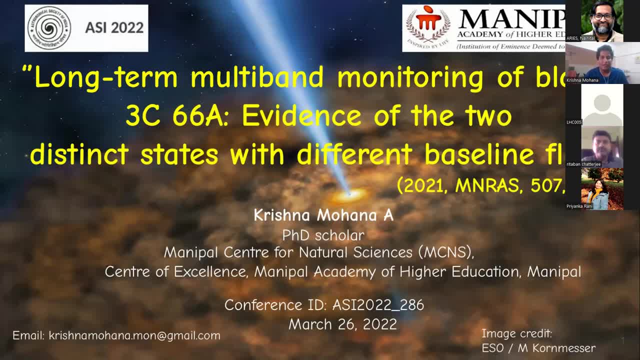 center for natural sciences, which is under manipal academy of higher, under manipal academy of higher, under manipal academy of higher education, education, education and and, and, at foremost, i thank the organizers for, at foremost, i thank the organizers for, at foremost, i thank the organizers for giving me an opportunity to 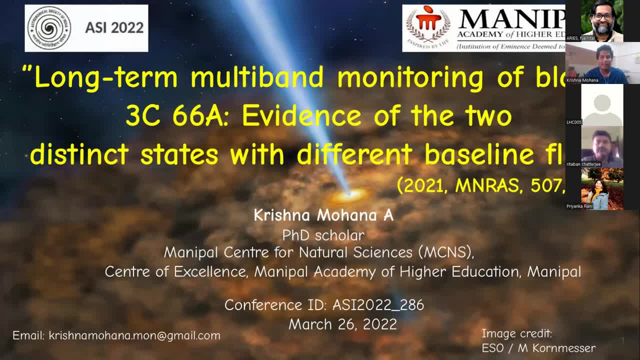 giving me an opportunity to giving me an opportunity to present our uh one of the published present, our uh one of the published present, our uh one of the published work, work work titled the long-term multiband. titled the long-term multiband. titled the long-term multiband: monitoring of the blazar- 3c66a. 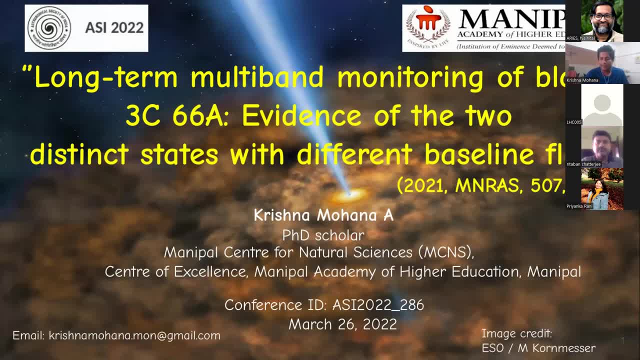 titled the long-term multiband monitoring of the blazar 3c66a. titled the long-term multiband monitoring of the blazar 3c66a. evidence of the two distinct states. evidence of the two distinct states. evidence of the two distinct states with the different baseline flux. 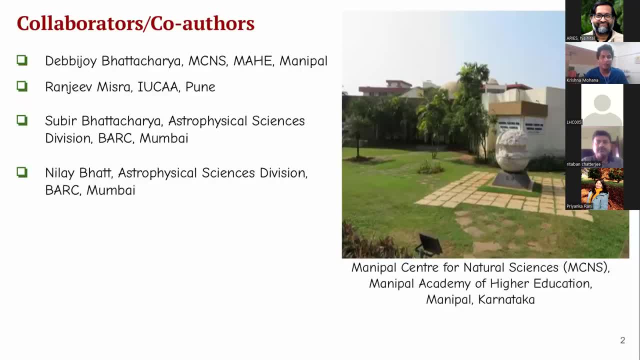 with the different baseline flux, with the different baseline flux. so i would like to also thank the. so i would like to also thank the. so i would like to also thank the co-authors of this work. uh, who is dr? co-authors of this work? uh, who is dr? 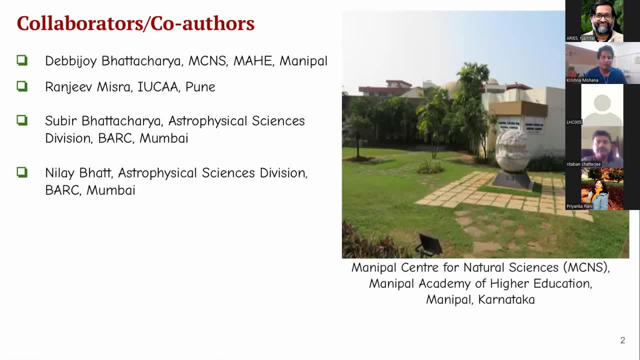 co-authors of this work: uh, who is dr devijoy batacharya, who is also my devijoy batacharya, who is also my devijoy batacharya, who is also my phd thesis supervisor, and ranjeev. 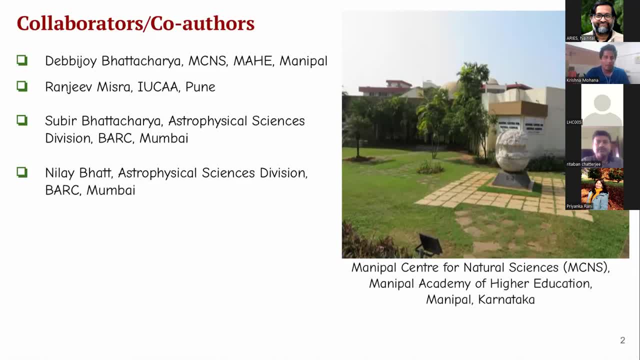 phd thesis supervisor. and ranjeev phd thesis supervisor. and ranjeev mishra, mishra mishra. subir batacharya and nilai bat. so i will subir batacharya and nilai bat. so i will subir batacharya and nilai bat. so i will give a very brief. 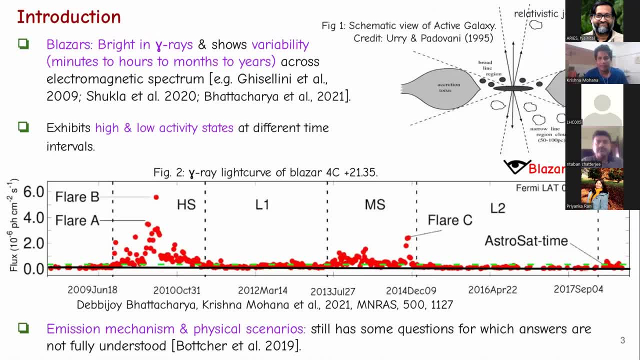 give a very brief, give a very brief introduction to the. what is uh blazar? introduction to the. what is uh blazar? introduction to the. what is uh blazar actually, if you look at the- the actually. if you look at the- the actually. if you look at the, the figure one, which is actually a schematic- 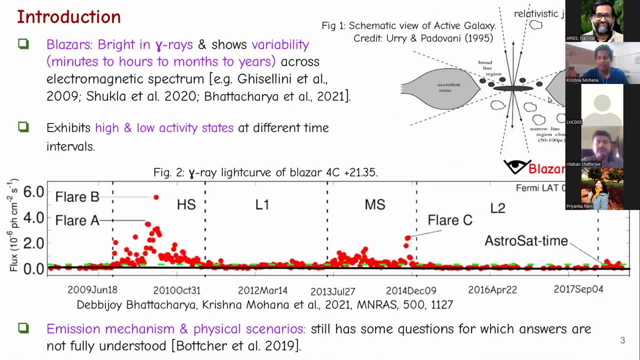 figure one which is actually a schematic figure, one which is actually a schematic representation of the representation, of the representation of the active galaxy, where you have a at the active galaxy, where you have a at the active galaxy, where you have a at the center- super massive black hole- and 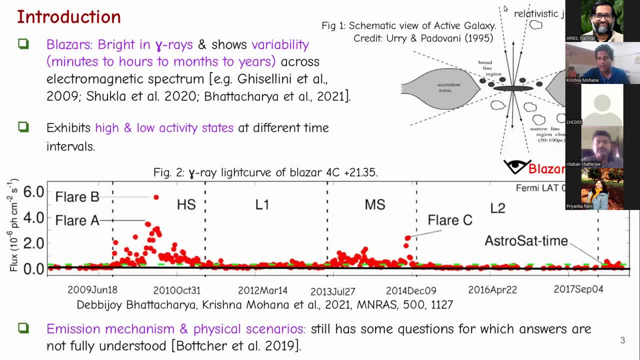 center super massive black hole and center super massive black hole and around it there is a crescent disk and around it there is a crescent disk and around it there is a crescent disk. and uh, there are relativity relativistic. uh, there are relativity relativistic. 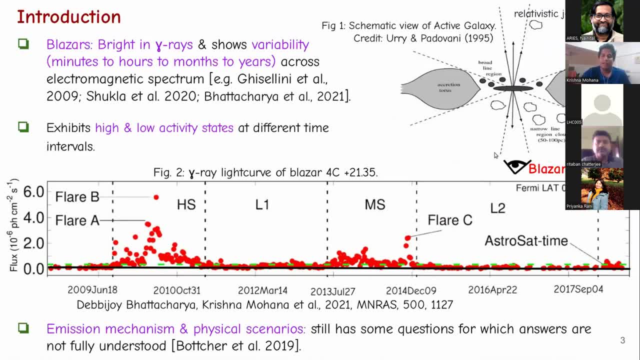 uh, there are relativity, relativistic, jet kind of structures which are emanating jet kind of structures which are emanating jet kind of structures which are emanating from this central region, from this central region, from this central region, and over the several decades different and over the several decades different. 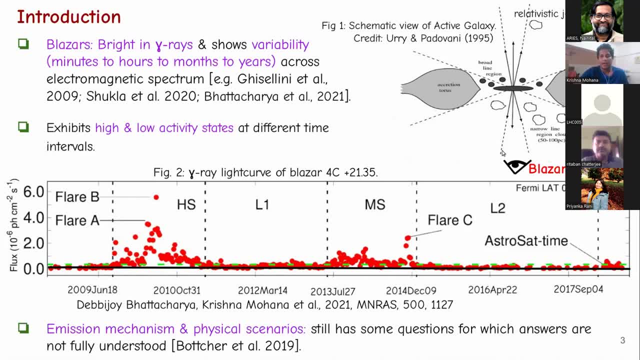 and over the several decades different kinds of active galaxies have been. kinds of active galaxies have been. kinds of active galaxies have been observed and uh under the unification observed and uh under the unification observed and uh under the unification scheme of proposed by uri and paduan. 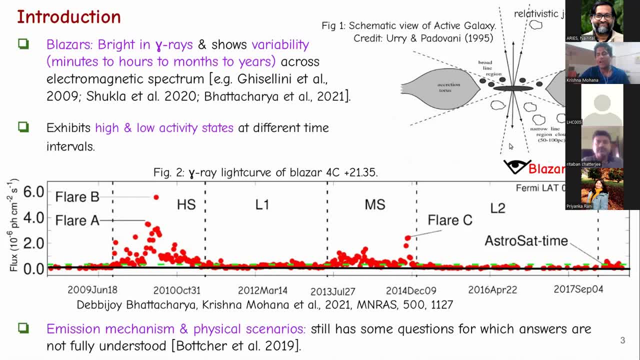 scheme of proposed by uri and paduan. scheme of proposed by uri and paduan. there's one particular class of active. there's one particular class of active. there's one particular class of active: galaxies which are very bright, galaxies which are very bright, galaxies which are very bright, and, uh, they are called as uh, blazers. 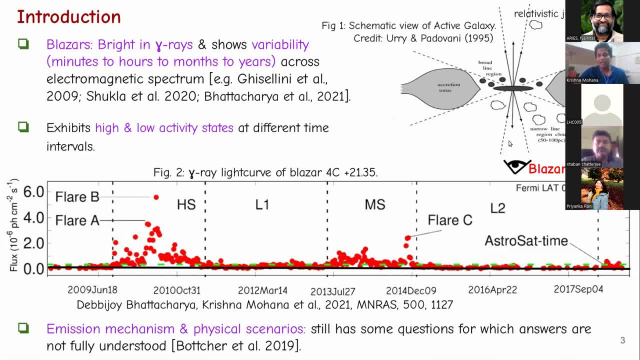 and uh they are called as uh blazers and uh they are called as uh blazers. where the relativistic jets is very, where the relativistic jets is very, where the relativistic jets is very, making a very small angle with the line, making a very small angle with the line. 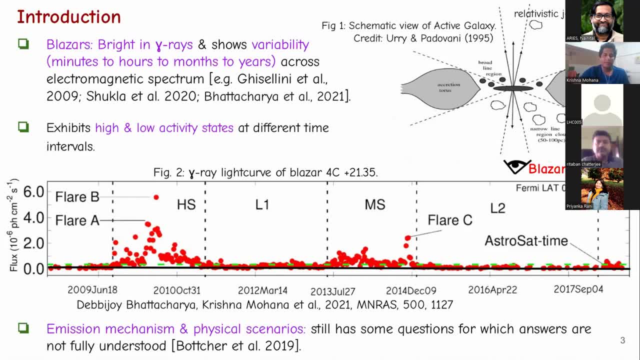 making a very small angle with the line of sight of the observer, of sight of the observer, of sight of the observer. blazers are very bright in gamma rays and it is very well bright in gamma rays and it is very well bright in gamma rays and it is very well known to show variabilities. 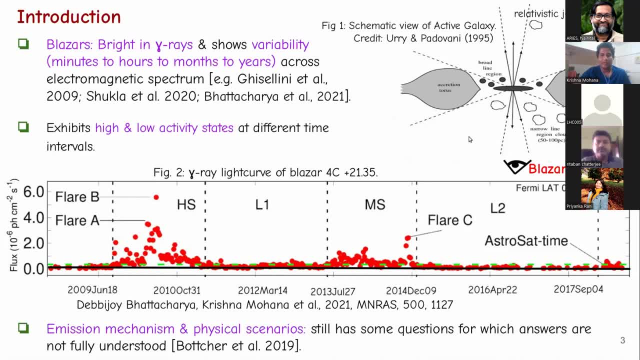 known to show variabilities. known to show variabilities: uh in gamma rays from minutes to hours. uh in gamma rays from minutes to hours. uh in gamma rays from minutes to hours, to months to, and even to months to, and even to months to and even year time scale. and uh, if you look at. 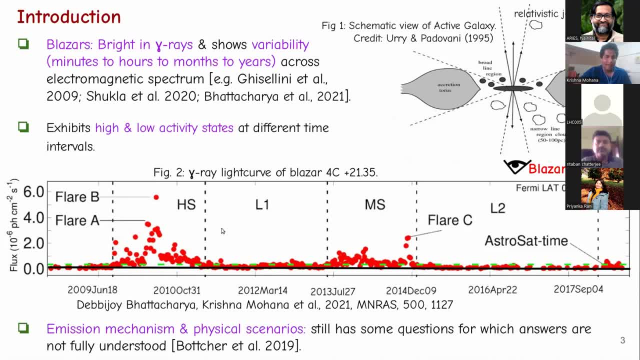 year time scale and uh, if you look at year time scale and uh, if you look at the figure two, this is a one of the the figure two. this is a one of the the figure two. this is a one of the typical gamma ray light curve of the. 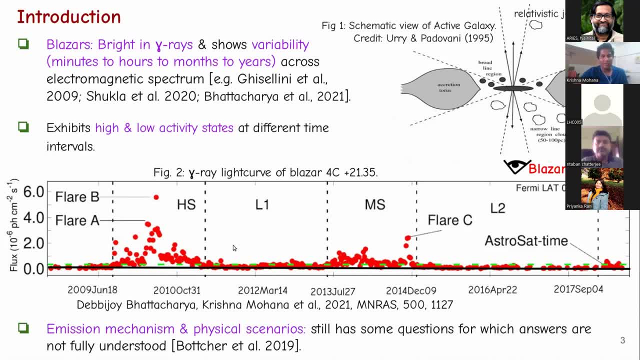 typical gamma ray light curve of the typical gamma ray light curve of the blazer 4c 21.35. blazer 4c 21.35. blazer 4c 21.35. i just wanted to emphasize on that, the uh. i just wanted to emphasize on that, the uh. 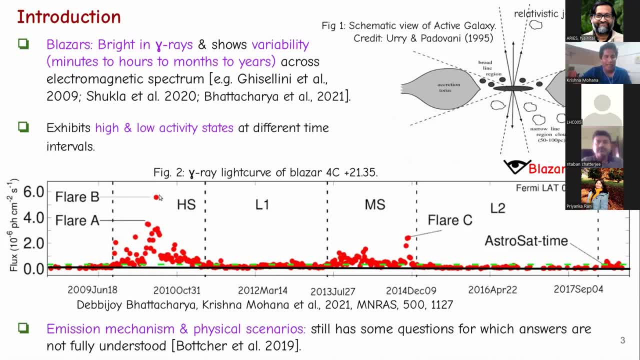 i just wanted to emphasize on that, the uh, that the. as you can see that the flux, that the, as you can see, that the flux, that the, as you can see that the flux sometimes goes very high, sometimes goes very high, sometimes goes very high, which is called flaring activities, and 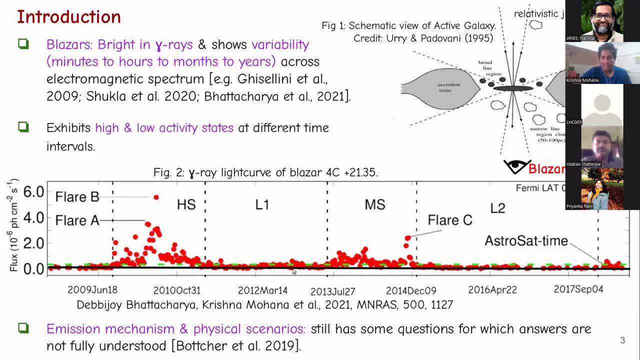 which is called flaring activities, and which is called flaring activities and then comes down and remains in the low, then comes down and remains in the low, then comes down and remains in the low activity. or the cousins for a long activity, or the cousins for a long. 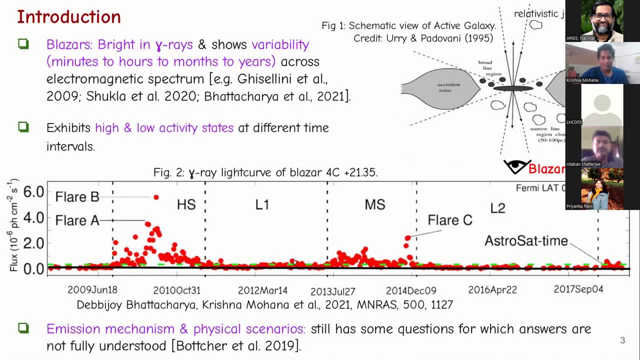 activity or the cousins, for a long period of time, period of time, period of time. so people have tried to address uh, the so people have tried to address uh, the so people have tried to address, uh the emission mechanism and possible emission mechanism and possible emission mechanism and possible physical scenarios for such activity. 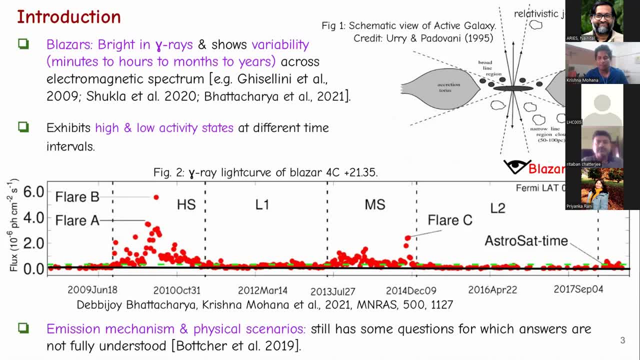 physical scenarios for such activity. physical scenarios for such activity: states, states, states over the several decades, but still there, over the several decades, but still there, over the several decades, but still there are some questions which are for which are some questions which are for which are some questions which are for which the answers are not fully understood. 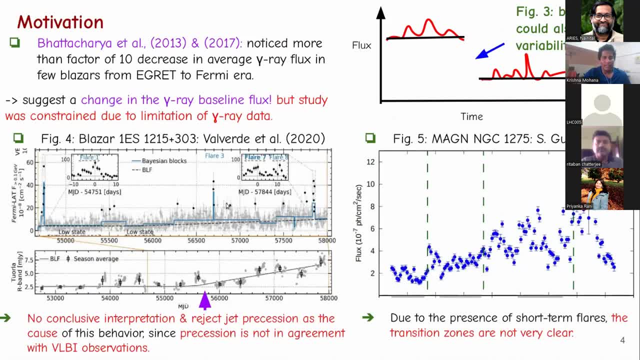 the answers are not fully understood. the answers are not fully understood based on the observation properties. based on the observation properties. based on the observation properties: uh, uh, uh. 2017. what they notice is that there is a 2017. what they notice is that there is a. 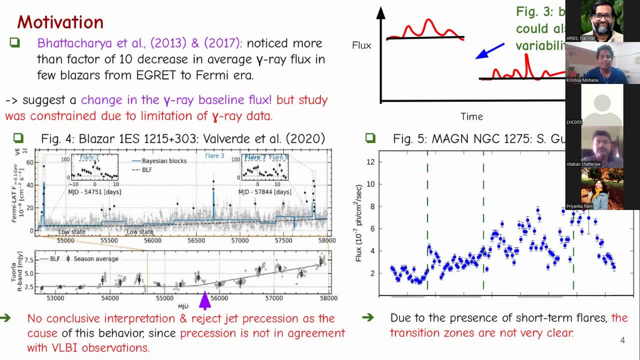 2017. what they notice is that there is a factor of more than a factor of 10. factor of more than a factor of 10. factor of more than a factor of 10. decrease in the average gamma reflux for. decrease in the average gamma reflux for. decrease in the average gamma reflux for a few of the egret egret is the earlier a few of the egret egret is the earlier a few of the egret egret is the earlier gamma emission which was 1991 to 1995. gamma emission which was 1991 to 1995. gamma emission, which was 1991 to 1995, and for me. for me was which is uh from, and for me for me was which is uh from, and for me for me was which is uh from 2008, and still it is in operational as. 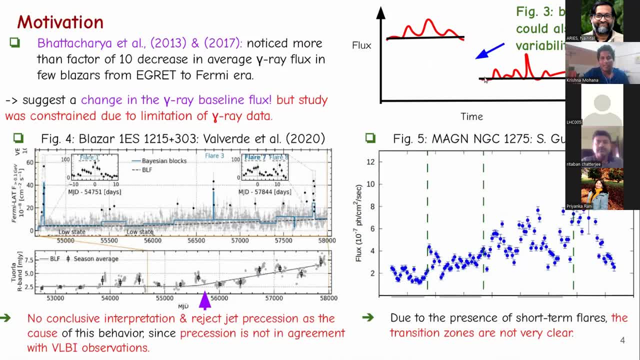 2008 and still it is in operational as 2008 and still it is in operational, as you can see in the, you can see in the. you can see in the uh figure. what we are asking is that is uh figure. what we are asking is that is. 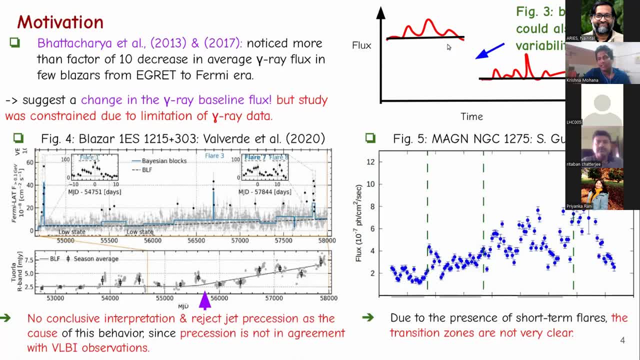 uh figure. what we are asking is that: is there any there, any there any? uh such kind of a baseline or average? uh such kind of a baseline or average? uh such kind of a baseline or average flux transition that could occur in. flux transition that could occur in. 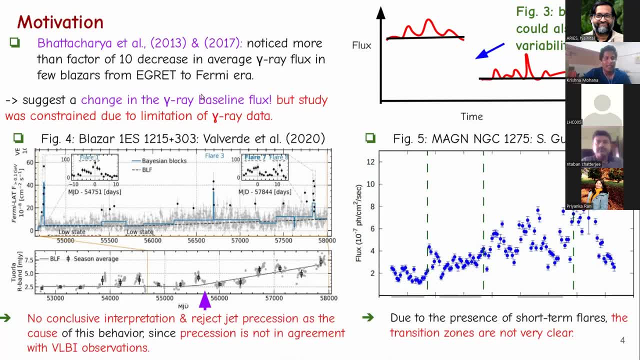 flux transition that could occur in these, uh, these, uh, these uh laser light cows. so their studies laser light cows, so their studies laser light cows, so their studies suggest some sort of a could happen. in suggest some sort of a could happen. in suggest some sort of a could happen in the sense that could occur and that 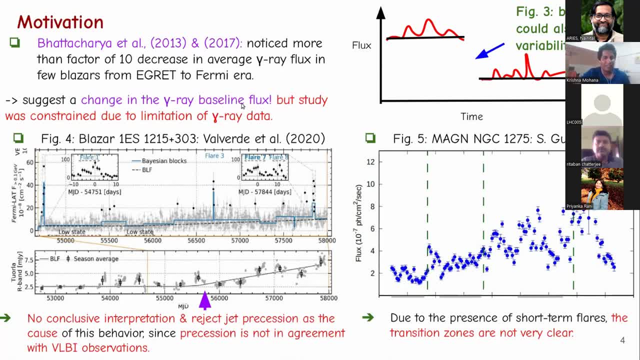 the sense that could occur and that the sense that could occur and that could lead to. the could lead to the? uh decrease in the average gamma reflux. uh decrease in the average gamma reflux. uh decrease in the average gamma reflux activity activity activity. uh in the recent times. uh with the. 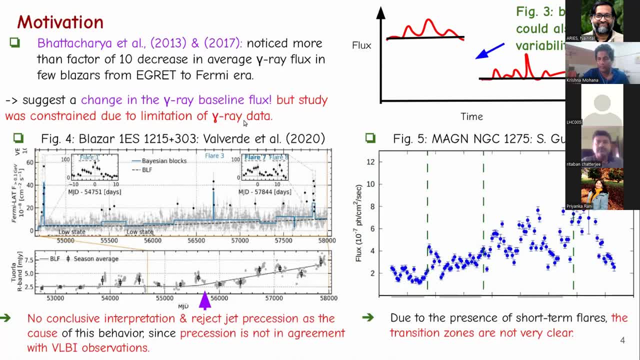 uh in the recent times, uh with the? uh in the recent times. uh with the decade-long observations, uh, decade-long observations, uh, decade-long observations. uh, one of the two few few works have been. one of the two few few works have been. one of the two few few works have been reported. one is uh. 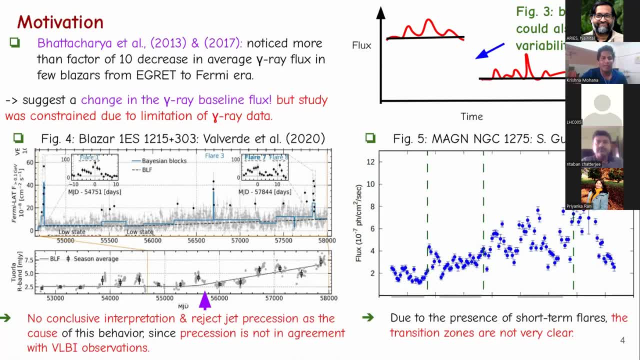 reported. one is uh reported. one is uh. in a blazar one es one, two, one, five plus. in a blazar one es one, two, one, five plus. in a blazar one es one, two, one, five plus three, zero, three by three, zero, three by three, zero, three by valverde at all 2020, as you can see in valverde at all 2020, as you can see in valverde at all 2020, as you can see in the figure four. what they see is that the figure four. what they see is that the figure four. what they see is that they see some kind of a 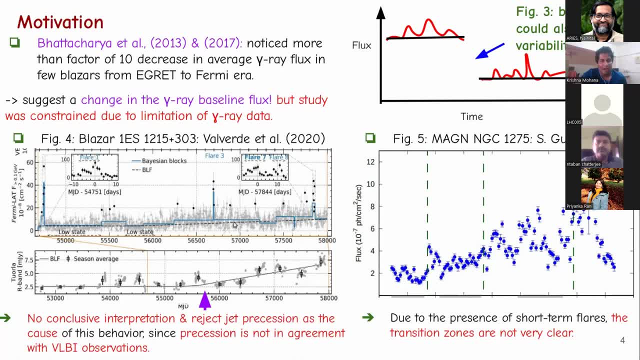 they see some kind of a. they see some kind of a gradual increase in the baseline flux, of gradual increase in the baseline flux, of gradual increase in the baseline flux of the gamma. this the gamma, this the gamma, this source in the gamma ray band, as well as. 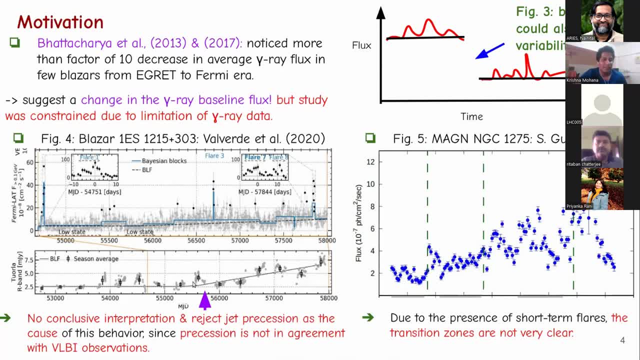 source in the gamma ray band as well as source in the gamma ray band as well as also. they see in the similar trend also. they see in the similar trend also. they see in the similar trend is also seen in the in the optical band. is also seen in the in the optical band. 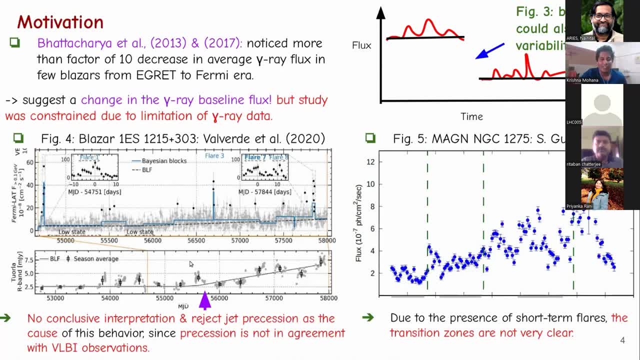 is also seen in the, in the optical band. however, uh, their study could not give. however, uh, their study could not give. however, uh, their study could not give any conclusive interpretation. why this is any conclusive interpretation? why this is such gradually it is increasing and such gradually it is increasing, and 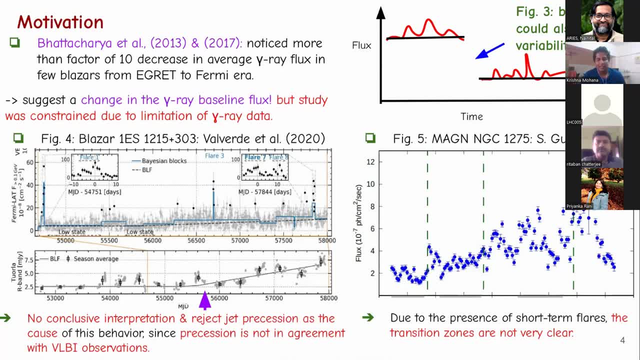 such gradually it is increasing. and they also try to look whether is there. they also try to look whether is there. they also try to look whether is there any, any, any jet precision which can cause such a jet precision, which can cause such a jet precision which can cause such a gradual increase in the 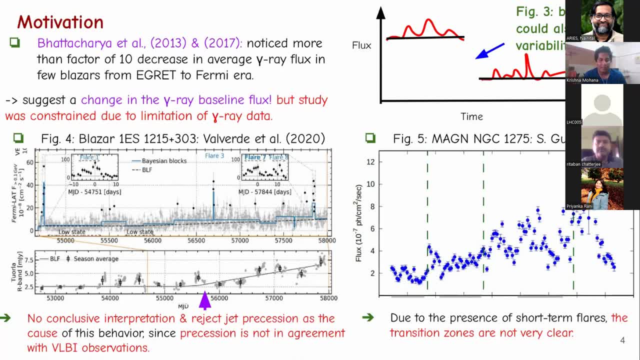 gradual increase in the gradual increase in the baseline activity uh which they reject baseline activity uh which they reject baseline activity uh which they reject this uh the hypothesis because their this uh the hypothesis, because their this uh the hypothesis, because their observations are not. observations are not observations are not. using the vlbi is not inconsistent with: 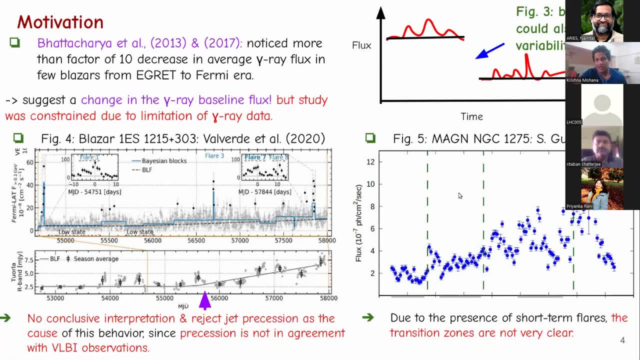 using the vlbi is not inconsistent with using the vlbi is not inconsistent with what they observe, and also there is what they observe, and also there is what they observe and also there is another study in the another class of, another study in the another class of 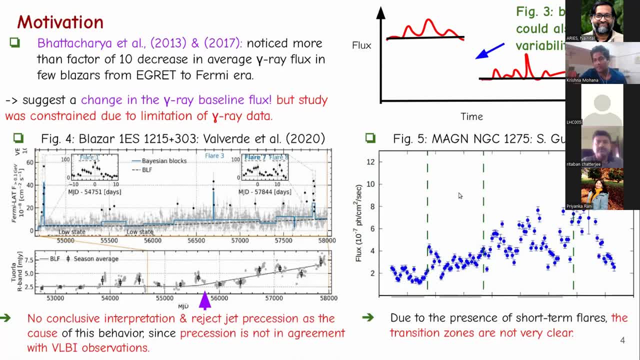 another study in the another class of activity called as mission missile and activity called as mission missile and activity called as mission missile and active galaxy, active galaxy. active galaxy: where in the ngc1275 as gulati at all, where in the ngc1275 as gulati at all. 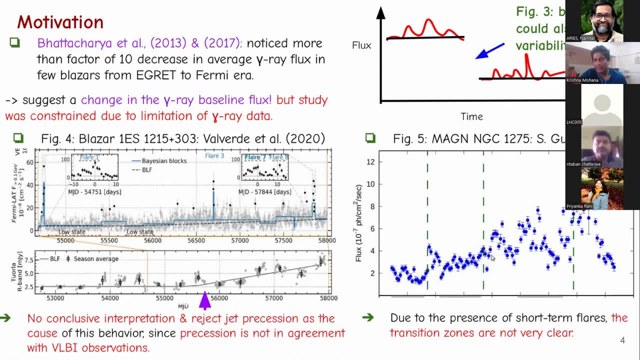 where in the ngc1275, as gulati at all, uh 2020. what they report is that there, uh 2020. what they report is that there, uh 2020. what they report is that there is also some kind of a baseline. uh, is also some kind of a baseline uh. 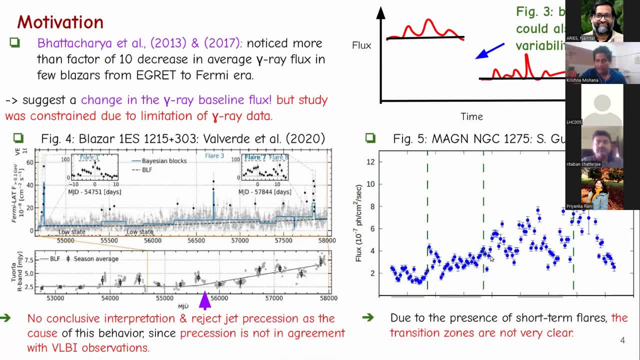 is also some kind of a baseline. uh, increase during the activity states, but increase during the activity states, but increase during the activity states, but due to the short-term fluctuation, they due to the short-term fluctuation, they due to the short-term fluctuation, they could not identify the clear transition. 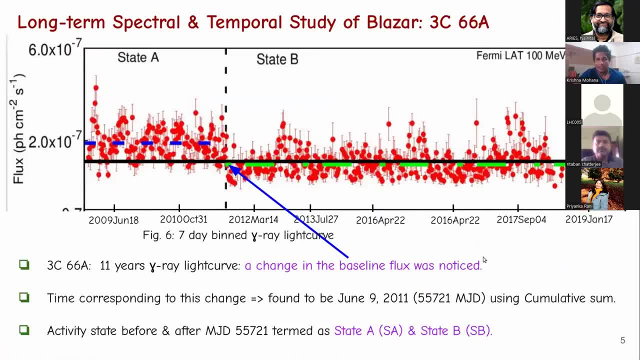 could not identify the clear transition, could not identify the clear transition zones, zones, zones in this particular source, in our uh study, in this particular source, in our uh study, in this particular source, in our uh study, which is a blazar 3c66a, which is a blazar 3c66a. 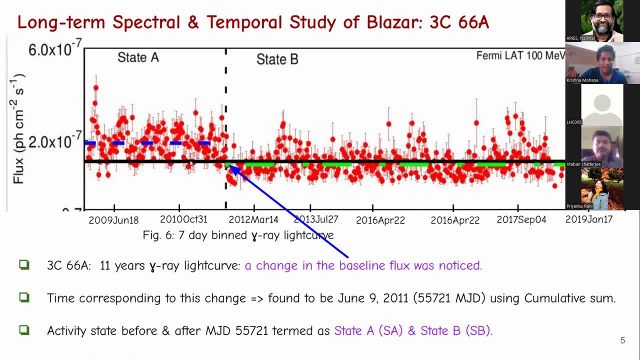 which is a blazar 3c66a. what we see is that in this figure, it is what we see is that in this figure, it is what we see is that in this figure, it is a weekly averaged gamma ray light curve. a weekly averaged gamma ray light curve. 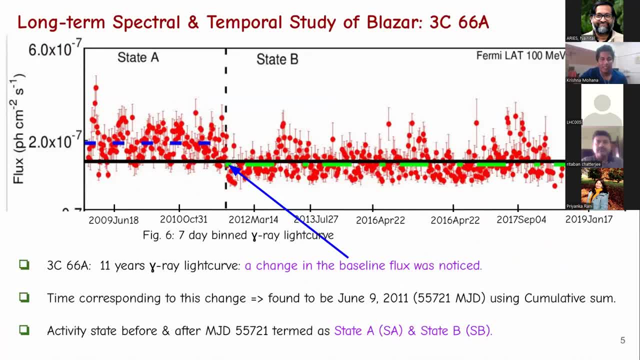 a weekly averaged gamma ray light curve. we see uh qualitatively, there is some. we see uh qualitatively, there is some we see uh qualitatively. there is some kind of a transition in the gamma ray, kind of a transition in the gamma ray, kind of a transition in the gamma ray baseline. 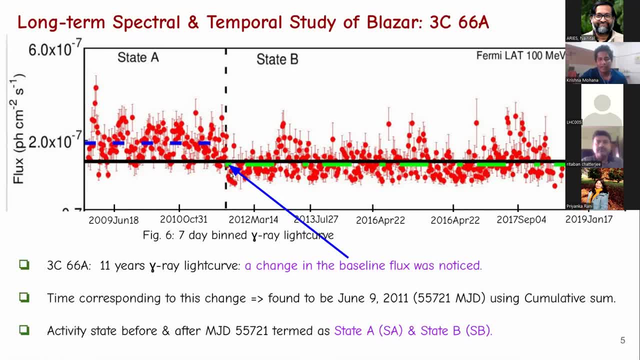 baseline- baseline which is uh happening around 2011 and which is uh happening around 2011 and which is uh happening around 2011 and june 2011. and the solid horizontal line- june 2011. and the solid horizontal line- june 2011. and the solid horizontal line is the average flux of this particular. 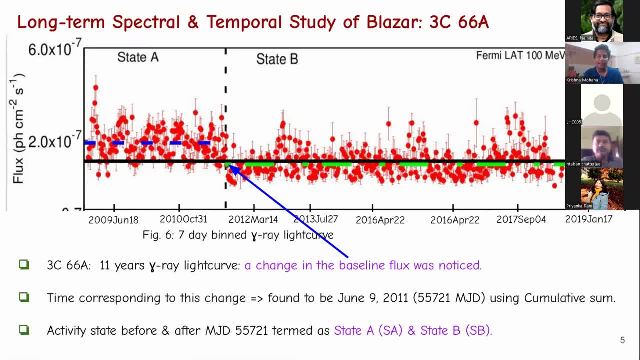 is the average flux of this particular, is the average flux of this particular source and the source and the source and the dotted dashed lines in the blue and the dotted dashed lines in the blue and the dotted dashed lines in the blue and the green are what we term it as. 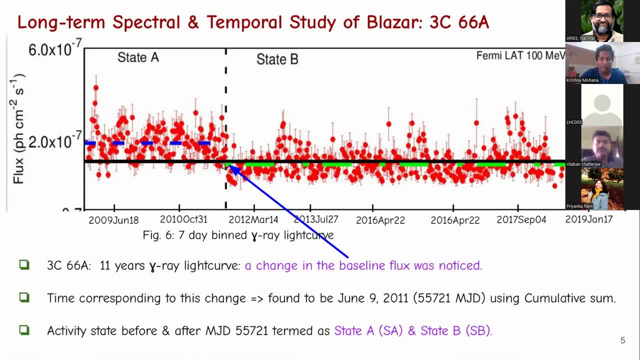 green are what we term it, as green are what we term it as the average flux for the state, which is the average flux for the state, which is the average flux for the state which is before the transition and before the transition and before the transition, and average flux for the state which is. 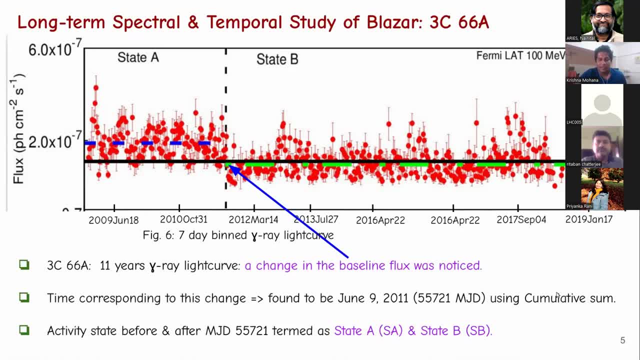 average flux for the state, which is average flux for the state which is after the transition. after the transition, we found that the transition is happening. we found that the transition is happening. we found that the transition is happening somewhere around june 9 2011, somewhere around june 9 2011. 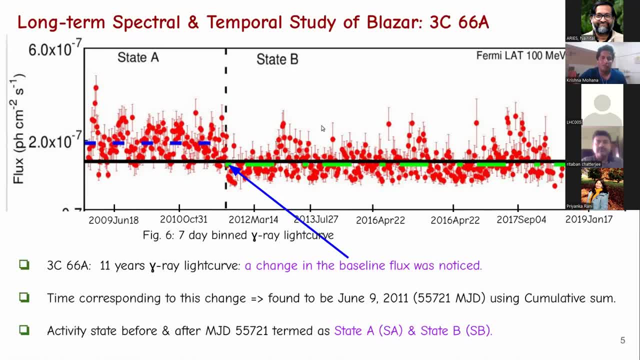 somewhere around june 9 2011, and we uh, we and we, uh, we and we uh we the state. we define the source to the state. we define the source to the state, we define the source to exhibitor- uh baseline uh transition. exhibitor- uh baseline uh transition. 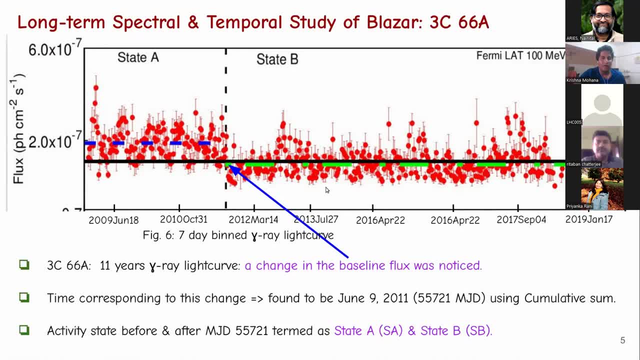 exhibitor. uh, baseline, uh, transition change, which is uh change, which is uh change, which is uh from state a to state b. now we looked from state a to state b. now we looked from state a to state b. now we looked at in the multi-band light for the. 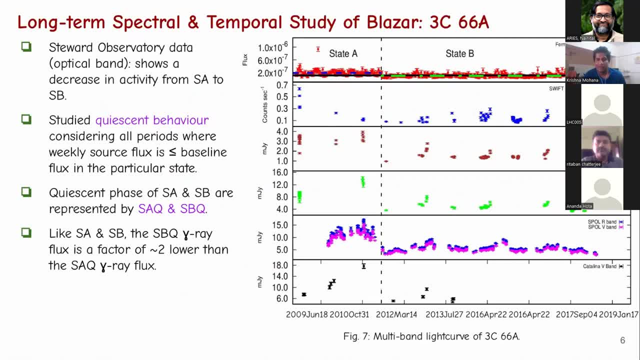 at in the multi-band light for the at in the multi-band light for the other uh energy bands, as you can see, is other uh energy bands. as you can see, is other uh energy bands. as you can see, is that the first one in this uh diagram is. 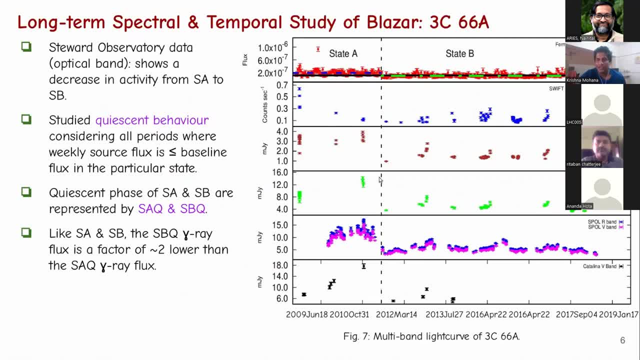 that the first one in this uh diagram is that the first one in this uh diagram is the gamma ray. like the second, is x-ray. the gamma ray, like the second, is x-ray. the gamma ray, like the second, is x-ray. third is a uv and third is a uv. and 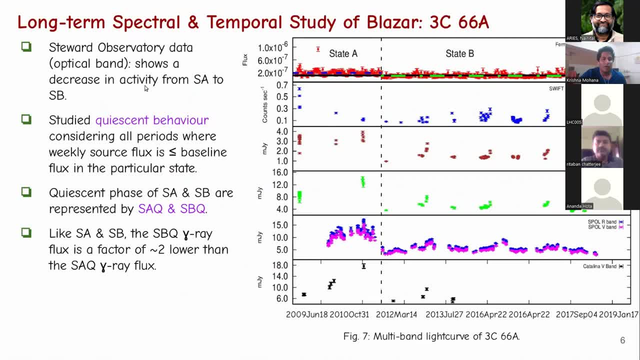 third is a uv, and fourth and fifth and sixth are in fourth, and fifth and sixth are in fourth, and fifth and sixth are in optical band. the uh optical band. the uh optical band, the uh, the optical data that is from the stewart. the optical data that is from the stewart. 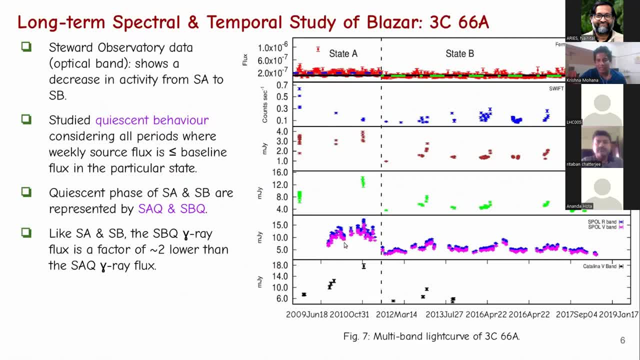 the optical data that is from the stewart observatory clearly indicates observatory. clearly indicates observatory clearly indicates that there is a some similar kind of a, that there is a some similar kind of a, that there is a some similar kind of a trend is also seen in the optical bank. 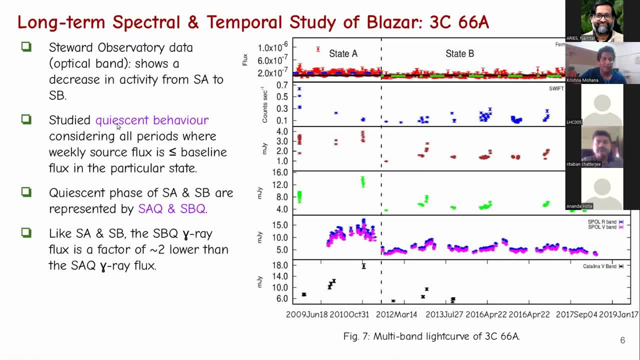 trend is also seen in the optical bank. trend is also seen in the optical bank- further we study. what we study is that further we study what we study is that further we study. what we study is that we try to address the poison behavior of. we try to address the poison behavior of. 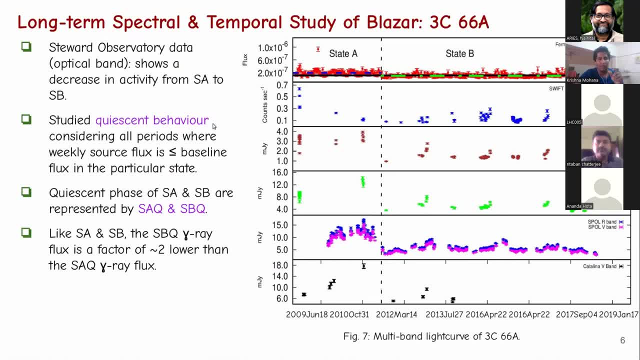 we try to address the poison behavior of this source in the gamma ray bank, where this source in the gamma ray bank, where this source in the gamma ray bank, where we consider, we consider, we consider those time periods where the flux is, those time periods where the flux is. 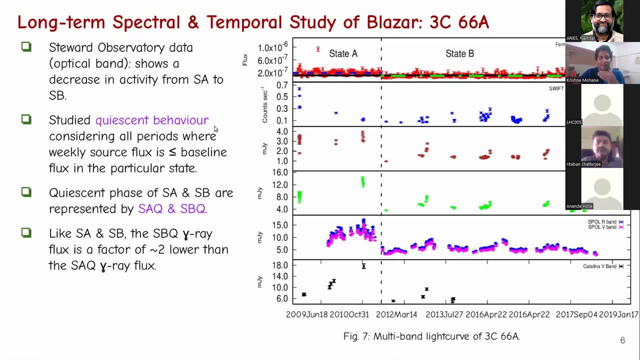 those time periods where the flux is less than or equal to the average, less than or equal to the average, less than or equal to the average flux of the during the particular state. flux of the during the particular state. flux of the during the particular state in the state a and the state b and we. 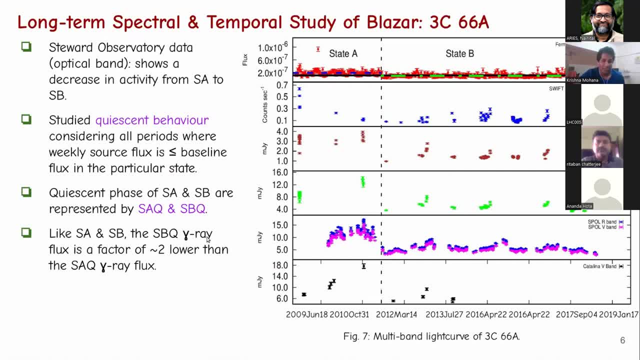 in the state a and the state b and we in the state a and the state b and we term this poison phase as saq and sbq term this poison phase as saq and sbq term this poison phase as saq and sbq- sbq. from the gamma ray analysis we find: 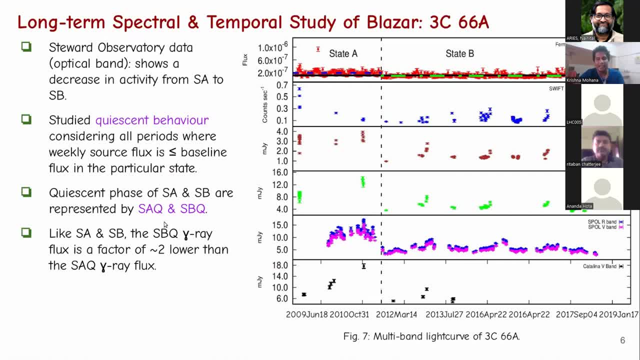 sbq from the gamma ray analysis. we find sbq. from the gamma ray analysis. we find that that that similar like that of the state a and similar like that of the state a and similar like that of the state a and state b, state b, state b- we find there is a gamma rate flux is. 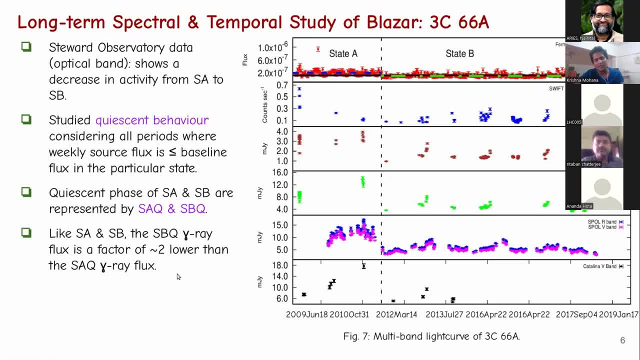 we find there is a gamma rate flux? is we find there is a gamma rate flux? is varying, decreasing by a factor of varying, decreasing by a factor of varying, decreasing by a factor of two, from state a to state b, even in the two, from state a to state b, even in the 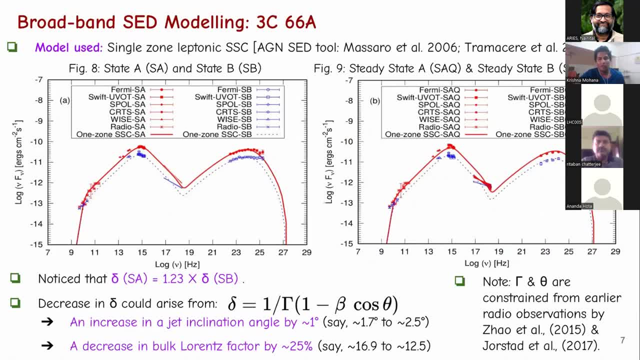 two, from state a to state b, even in the cohesion state, cohesion state, cohesion state. now we further, we investigate what could now, we further, we investigate, what could now, we further, we investigate what could be the possible reason by using, be the possible reason by using, be the possible reason by using, by constructing the broadband spectral. 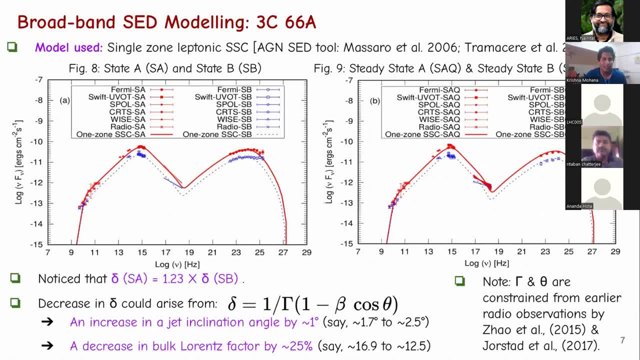 by constructing the broadband spectral, by constructing the broadband spectral energy distribution, we used a single energy distribution. we used a single energy distribution. we used a single zone, electronic zone, electronic zone, electronic self-symptom optimization model. where self-symptom optimization model, where self-symptom optimization model, where the results is shown in the figure 8 and 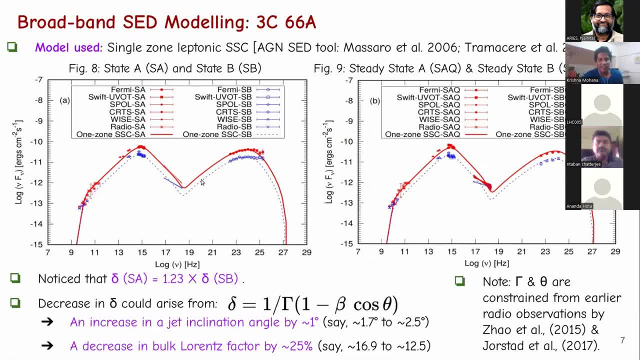 the results is shown in the figure 8. and the results is shown in the figure 8 and figure 9 for state a and cohesion states. figure 9 for state a and cohesion states. figure 9 for state a and cohesion states. what we notice that keeping the other. 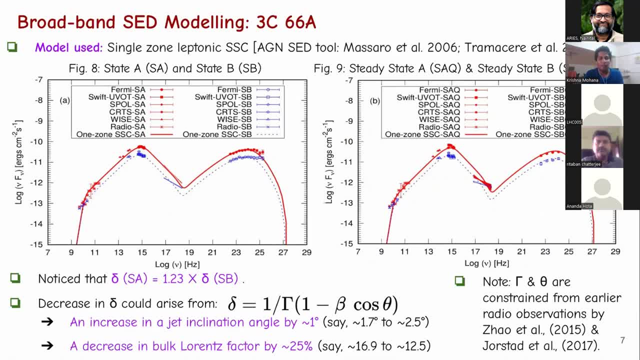 what we notice that keeping the other. what we notice that keeping the other, all the other rest of the parameters, all the other rest of the parameters, all the other rest of the parameters fixed from state a to state b, fixed from state a to state b, fixed from state a to state b, by only tweaking the change in the. 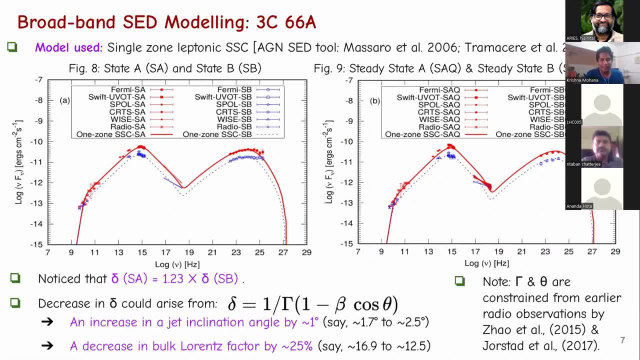 by only tweaking the change in the, by only tweaking the change in the doppler beaming factor. doppler beaming factor. doppler beaming factor. we could able to uh explain, we could able to uh explain, we could able to uh explain the, the, the, the lower, the. 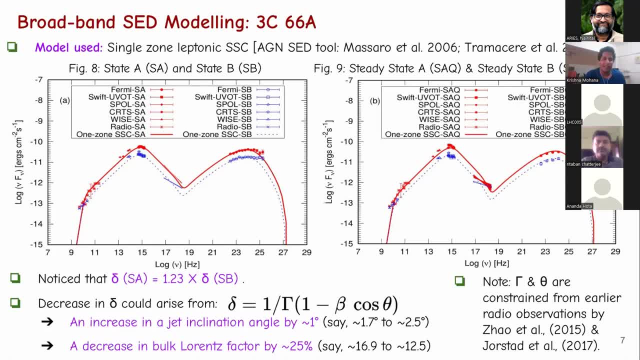 the the the lower, the the low, the the the lower, the the low activity. the baseline uh flux change activity. the baseline uh flux change activity. the baseline uh flux change from state a to state b, from state a to state b, from state a to state b. now uh doppler beaming factor could. 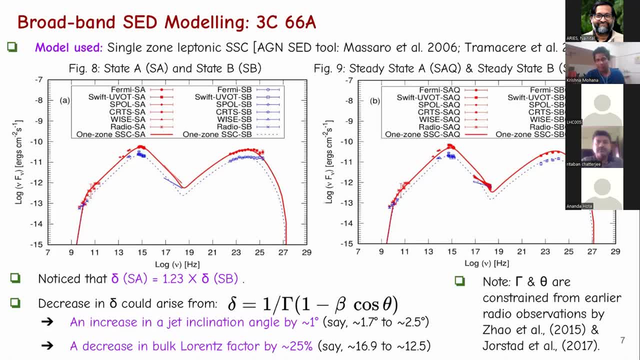 now uh doppler beaming factor, could now uh doppler beaming factor could arise, arise, arise uh. due to uh increase uh change in the uh. due to uh increase uh change in the uh. due to uh increase uh change in the doppler beam. doppler beam. 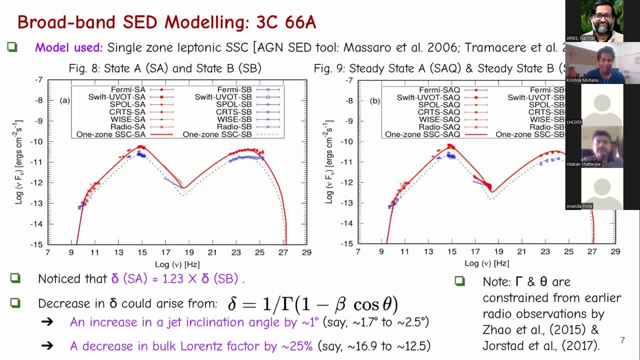 doppler beam can happen due to the increase in the jet. can happen due to the increase in the jet. can happen due to the increase in the jet inclination angle by one degree inclination angle. by one degree inclination angle by one degree, say, for example, from 1.7 to 1 to 2.5. 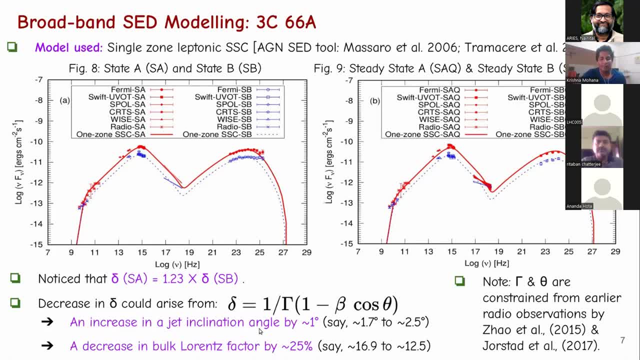 say, for example, from 1.7 to 1 to 2.5. say, for example, from 1.7 to 1 to 2.5 in this particular case, and or or else in this particular case, and or or else in this particular case, and or or else the decrease in the bulk law range. 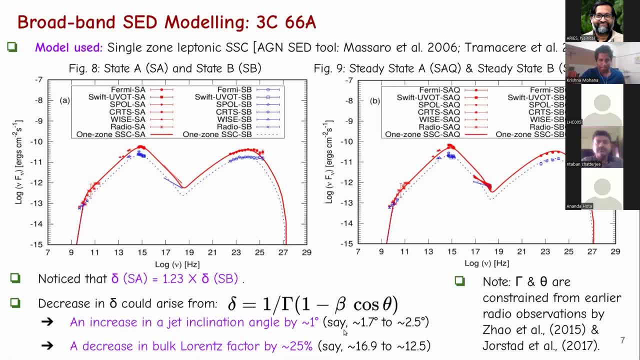 the decrease in the bulk law range. the decrease in the bulk law range factor by around 25 percent, factor by around 25 percent, factor by around 25 percent. and, uh, what we see is that is is such a, and uh, what we see is that is is such a. 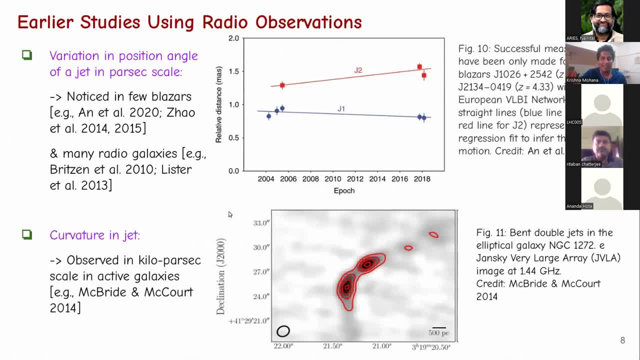 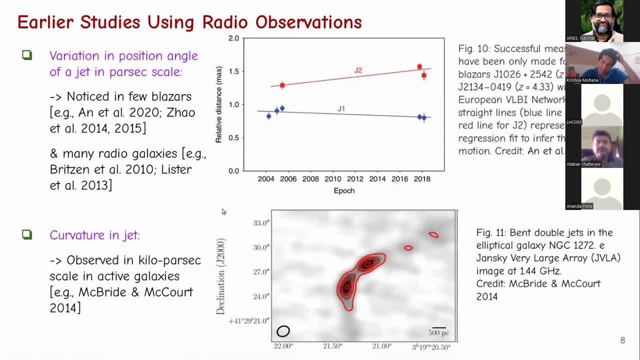 because in blazers, uh, what is how we are? we don't have a very. what is how we are? we don't have a very. what is how we are? we don't have a very. very good uh radio observations to check. very good uh radio observations to check. 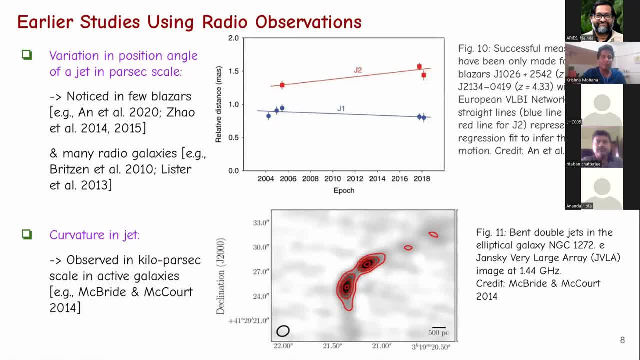 very good uh radio observations to check for the check for the, for the check for the check for the, for the check for the. the jet viewing angle. because it is a the jet viewing angle. because it is a the jet viewing angle because it is a, most of the emission is a jet dominated. 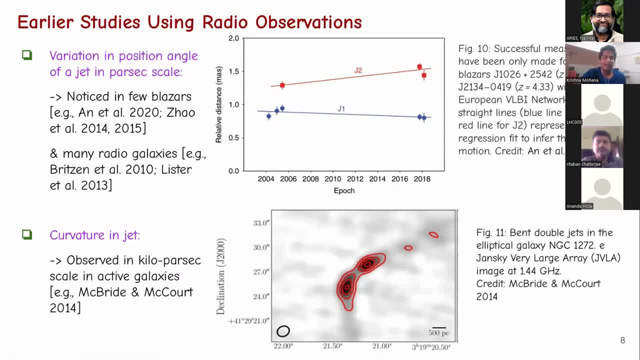 most of the emission is a jet dominated. most of the emission is a jet dominated and it is not uh highly resolved, unlike, and it is not uh highly resolved, unlike and it is not uh highly resolved, unlike the other, uh, the other, uh, the other, uh other missile and galaxies: uh, there is a. 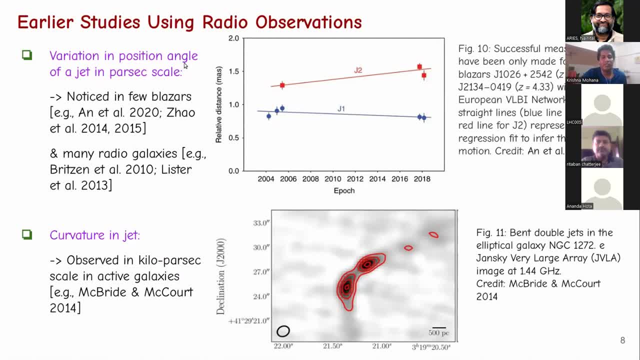 other missile and galaxies? uh, there is a other missile and galaxies. uh, there is a one particular study, one particular study, one particular study where they see that variation in the, where they see that variation in the, where they see that variation in the position angle of in the jet, in the par. 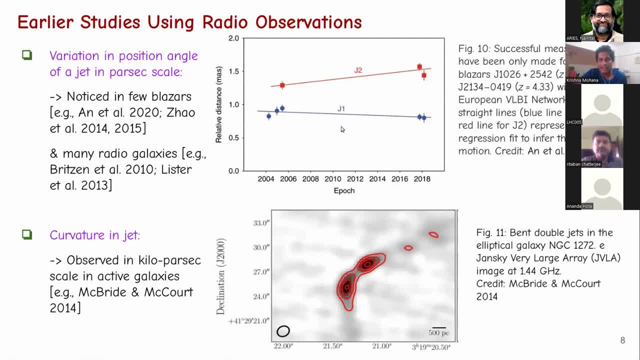 position angle of in the jet in the par position angle of in the jet in the par six scale, when, particularly in the six scale, when, particularly in the six scale, when, particularly in the blazer- uh, the figure 10 shows that it blazer. uh, the figure 10 shows that it. 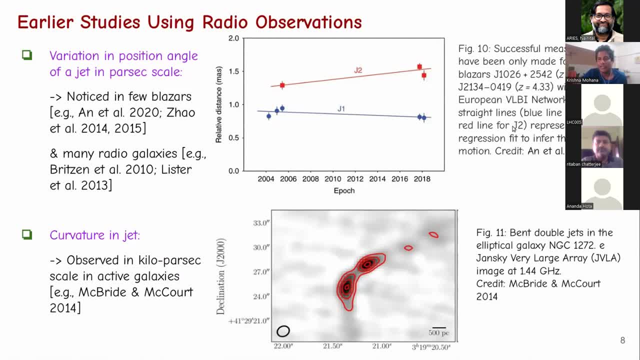 blazer: uh. the figure 10 shows that it is a more than 12 years of. uh is a more than 12 years of uh is a more than 12 years of uh. observations uh using a vlbi network. observations uh using a vlbi network. 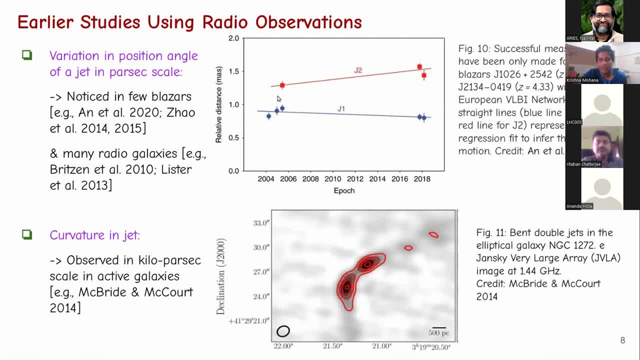 observations: uh, using a vlbi network, we open ulb network. what they see is that we open ulb network. what they see is that we open ulb network. what they see is that, for one of the blazers, so also two of. for one of the blazers, so also two of. 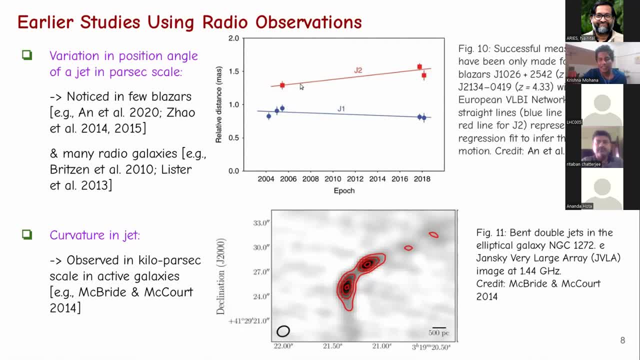 for one of the blazers, so also two of the blazers this year. the position the blazers this year. the position the blazers this year. the position angle changes almost like a around uh angle changes almost like a around uh angle changes almost like a around uh one degree. 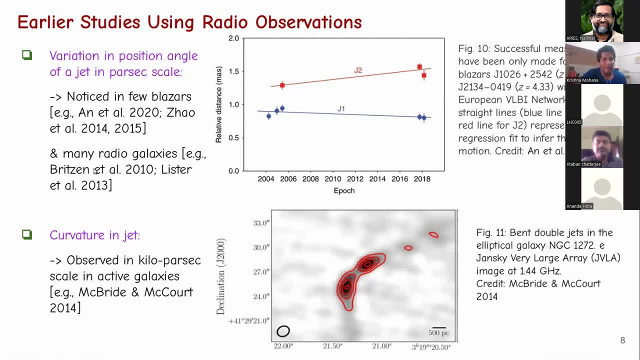 one degree, one degree and uh further also. there are stars some, and uh further also. there are stars some, and uh further also. there are stars, some of the of the of the many, many radio galaxies show such uh, many, many radio galaxies show such uh many many radio galaxies show such uh, observe such properties. 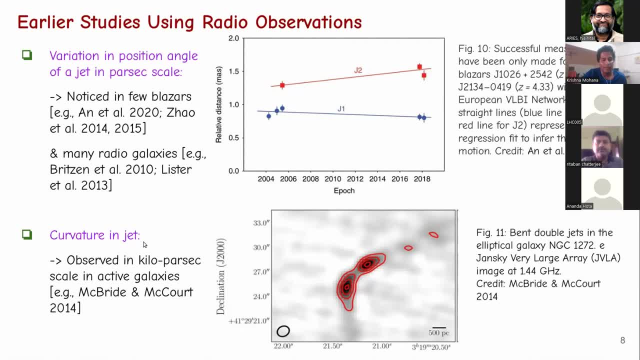 observe such properties. observe such properties, uh, and other thing is that, uh, uh, and other thing is that, uh, uh, and other thing is that uh other in the kilo parsec scales, in some other in the kilo parsec scales, in some other in the kilo parsec scales in some of the active galaxies. 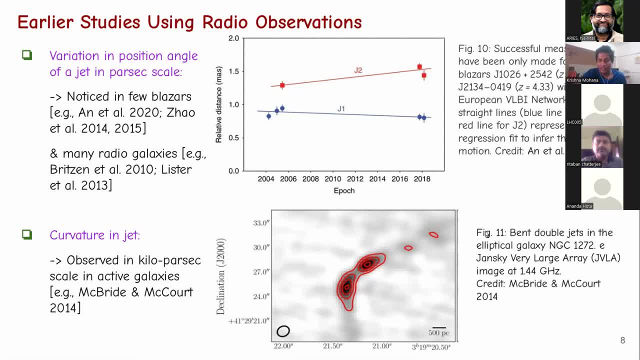 of the active galaxies, of the active galaxies, people have seen the curvature in the jet. people have seen the curvature in the jet. people have seen the curvature in the jet, which is shown in the figure 11.. which is shown in the figure 11.. which is shown in the figure 11.. have, then, what we see is that we 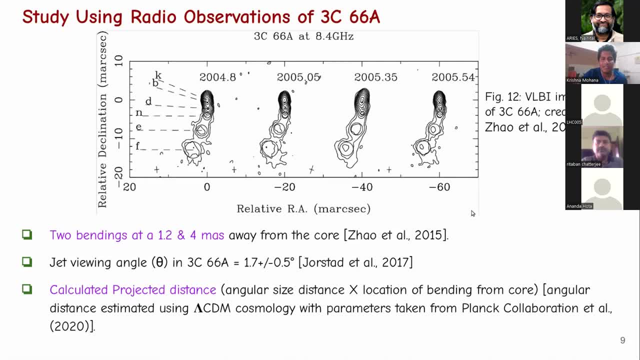 which is shown in the figure 11.. have, then, what we see is that we, which is shown in the figure 11.. have, then, what we see is that we look at the literature. did uh look at the literature, did uh look at the literature, did uh is the 3c66, our blazer, has any radio. 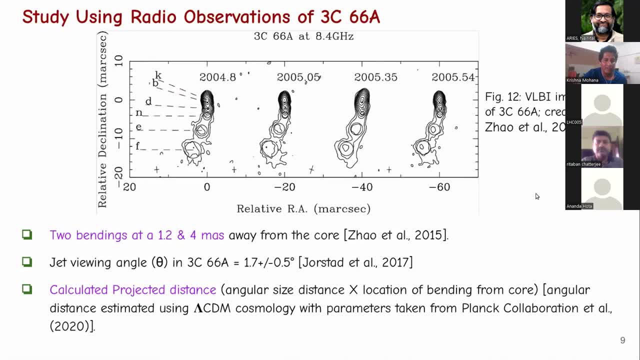 is the 3c66 our blazer has any radio? is the 3c66 our blazer has any radio observations? then we could find that observations. then we could find that observations. then we could find that from jordan 2015, what we found is from: 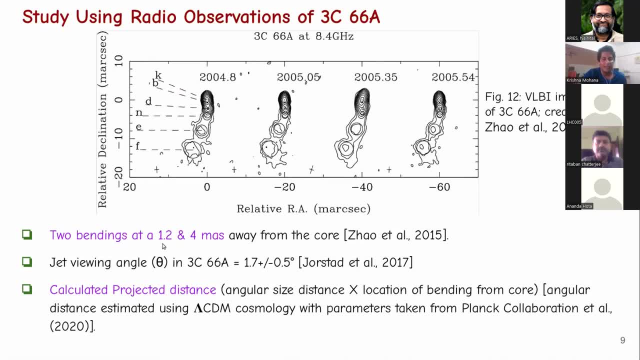 from jordan 2015. what we found is from from jordan 2015. what we found is from the vlbi radio morphology. we see that, the vlbi radio morphology. we see that the vlbi radio morphology. we see that there is a. there is a. 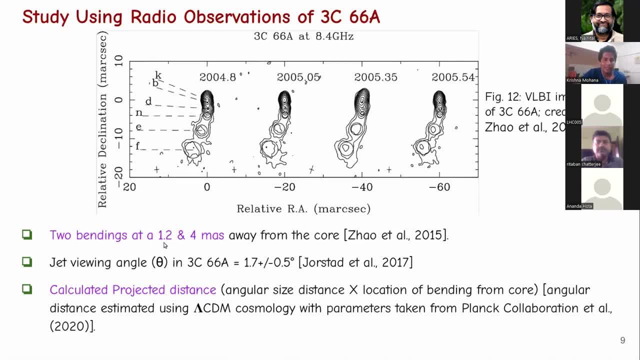 there is a bend, two banks in this particular uh jet bend, two banks in this particular uh jet bend, two banks in this particular uh jet around 1.2 mas and 4 mas from the core, around 1.2 mas and 4 mas from the core. 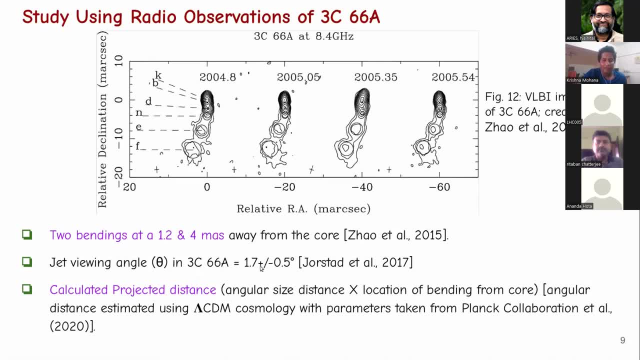 around 1.2 mas and 4 mas from the core. and uh we considered the average jet and uh we considered the average jet and uh we considered the average jet. weaving angle of 1.7, which is taken from. weaving angle of 1.7, which is taken from. 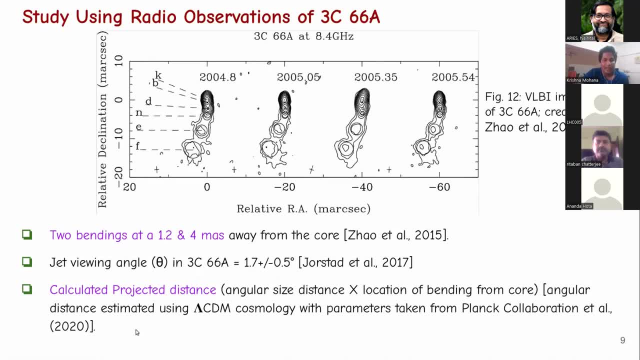 weaving angle of 1.7, which is taken from the george georgetown 2017, and we the george georgetown 2017 and we the george georgetown 2017, and we calculated the projected distance and calculated the projected distance and. 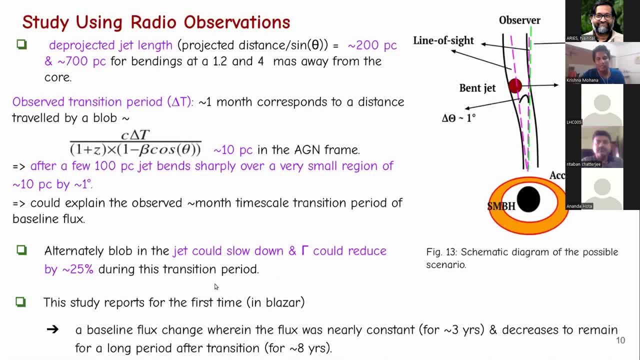 calculated the projected distance and also the, also the, also the deprojected length down the jet. where deprojected length down the jet, where deprojected length down the jet, where this bending is corresponding in the. this bending is corresponding in the. this bending is corresponding in the linear scale. it is coming around the 200. 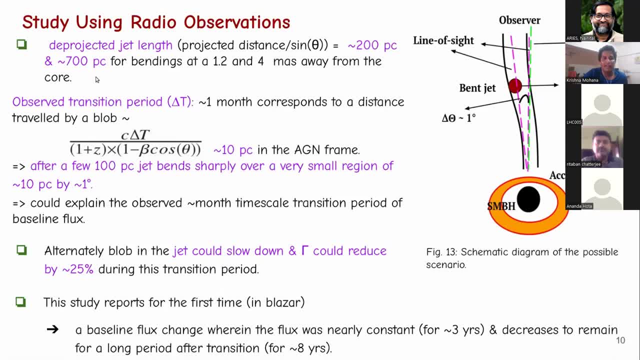 linear scale. it is coming around the 200 linear scale. it is coming around the 200 parsec for 1.2 mas and parsec for 1.2 mas and parsec for 1.2 mas and 700 parsec for the, the other core mas. 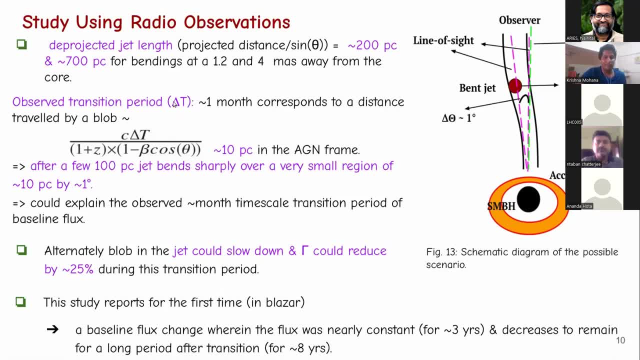 700 parsec for the- the other core, mas- 700 parsec for the- the other core, mas- value, value value and the- the transition time that period and the- the transition time that period and the- the transition time that period. what we see is that around a month time. 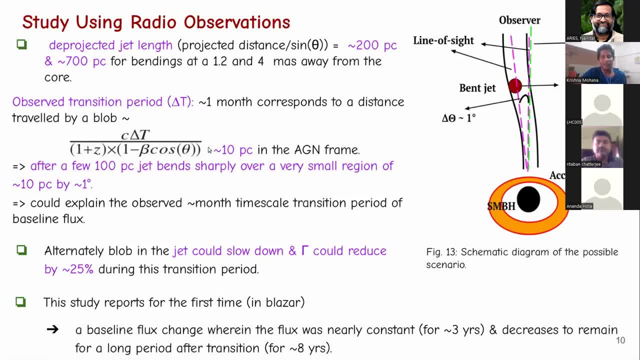 what we see is that around a month time. what we see is that around a month time scale, scale, scale. if you consider this time scale and if, if you consider this time scale and if, if you consider this time scale and if you try to calculate what is the? 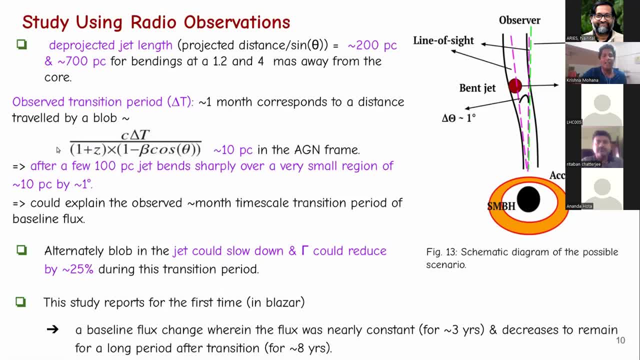 you try to calculate what is the. you try to calculate what is the. what is how far the blob has uh moved in? what is how far the blob has uh moved in? what is how far the blob has uh moved in this this, this time month? that comes around roughly 10. 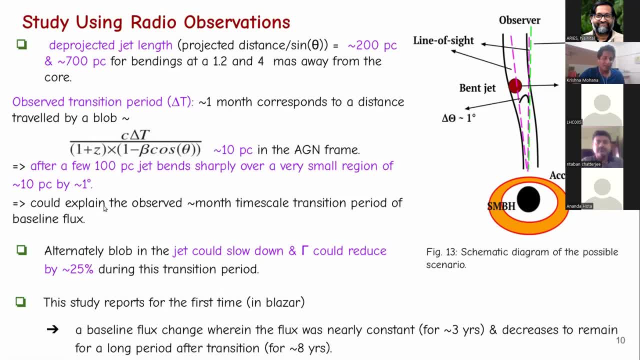 time month. that comes around roughly 10 time month. that comes around roughly 10 parsecs in the asian frame. so this parsecs in the asian frame, so this parsecs in the asian frame. so this implies that implies that implies that after a few hundreds of parsec in this, 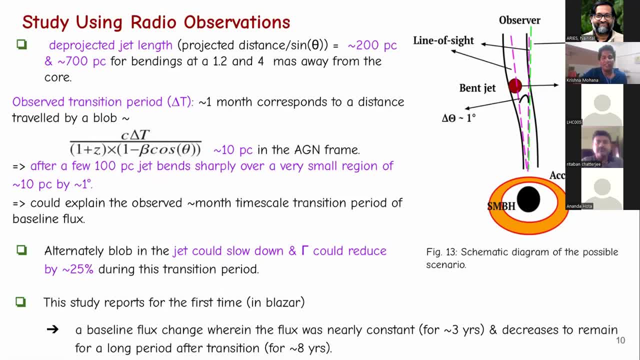 after a few hundreds of parsec in this, after a few hundreds of parsec in this 368 jet that bends sharply over a very 368 jet, that bends sharply over a very 368 jet, that bends sharply over a very small region, small region, small region, around 10 parsecs by. 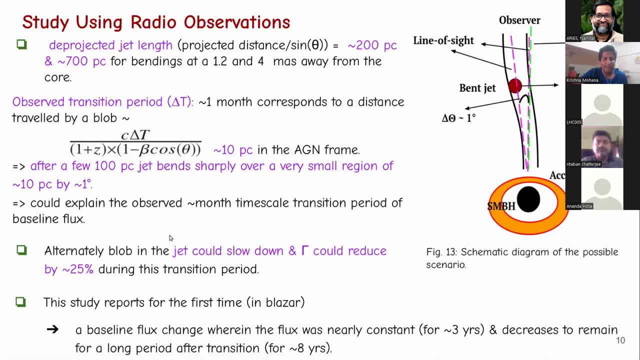 around 10 parsecs by around 10 parsecs by around one degree. uh, so this, this could around 10 parsecs by around one degree. uh, so this, this could around 10 parsecs by around one degree. uh, so this, this could explain the observed. you have two more. 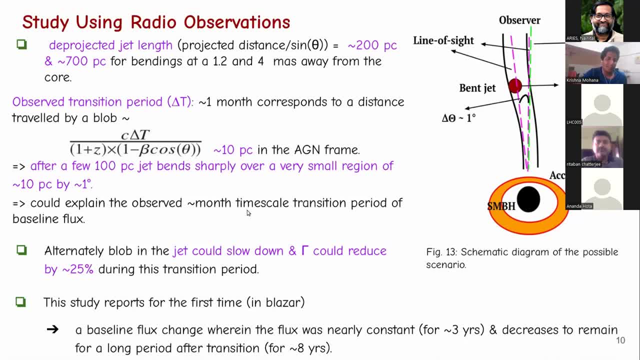 explain the observed. you have two more. explain the observed. you have two more minutes, minutes, minutes. yeah, i'm almost done, uh, uh, yeah, i'm almost done, uh, uh. yeah, i'm almost done, uh, uh. month scale time: transition period of month scale time. transition period of month scale time: transition period of the base networks. also, we are not uh. 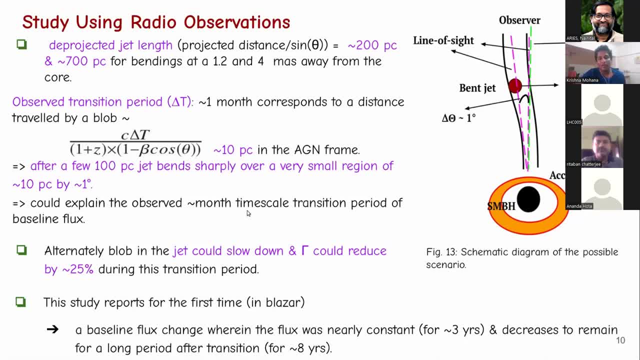 the base networks also. we are not uh, the base networks also. we are not uh, excluding. the alternative thing is that excluding the alternative thing is that excluding. the alternative thing is that the uh, the uh, the uh, blob and the jet could have slowed down, blob and the jet could have slowed down. 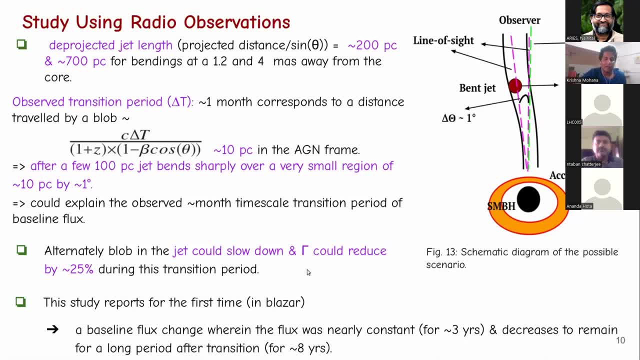 blob and the jet could have slowed down. and it is also possible that the and it is also possible that the and it is also possible that the uh reduction in the bulk orange factor, uh reduction in the bulk orange factor, uh reduction in the bulk orange factor could have happened by around 25, which. 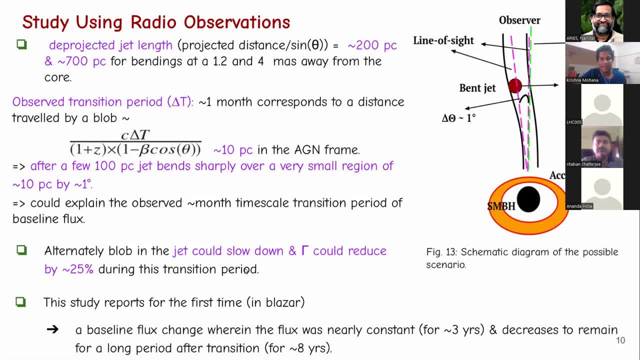 could have happened by around 25, which could have happened by around 25, which is can also explain the. is can also explain the. is can also explain the: uh, the change in the baseline uh flux. uh, the change in the baseline uh flux. uh, the change in the baseline uh flux from state a to state b. i have shown. 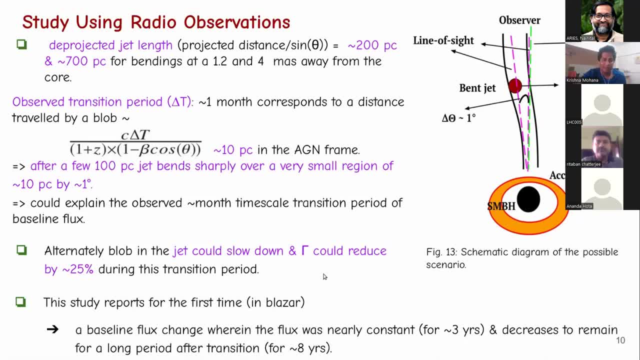 from state a to state b. i have shown from state a to state b. i have shown the year- figure 13, the schematic roughly the year. figure 13, the schematic roughly the year. figure 13, the schematic roughly, the schematic diagram: what is happening. the schematic diagram what is happening. 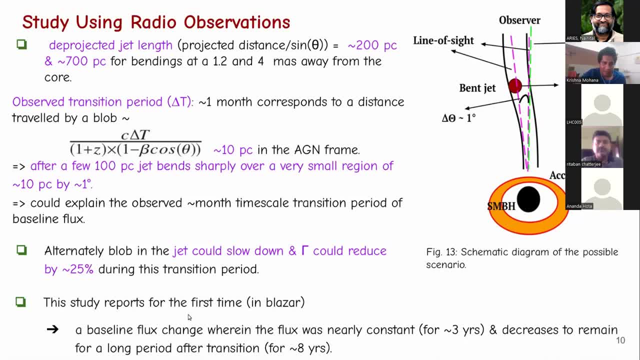 the schematic diagram. what is happening in this particular 360 stage is just in. this particular 360 stage is just in. this particular 360 stage is just. this is a first time we are reporting in this particular 360 stage is just this is a first time we are reporting in. 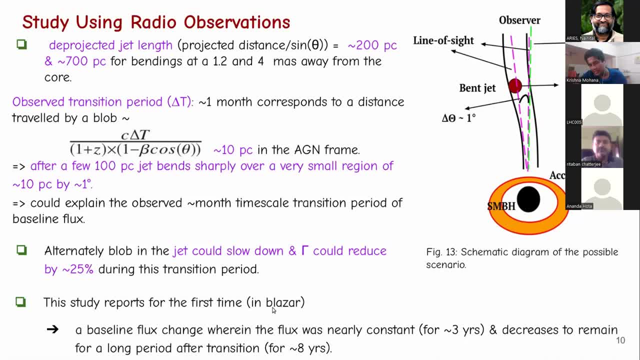 this particular 360 stage is just. this is a first time we are reporting in blazer, unlike in the worldwide blazer. unlike in the worldwide blazer, unlike in the worldwide. 2020, where they see the gradual increase. 2020, where they see the gradual increase. 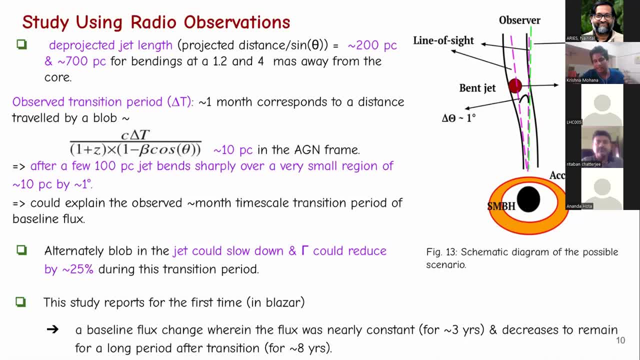 2020, where they see the gradual increase. here we see that there is a transition. here we see that there is a transition. here we see that there is a transition in the baseline flux, where the flux is in the baseline flux, where the flux is in the baseline flux, where the flux is nearly constant for roughly three years. 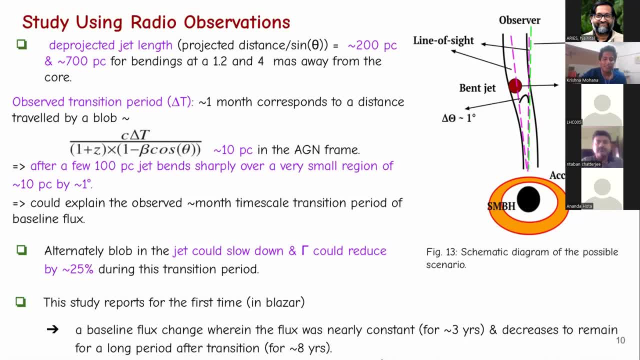 nearly constant for roughly three years. nearly constant for roughly three years, and then decreases to remain in the long, and then decreases to remain in the long, and then decreases to remain in the long period after the transition for eight period, after the transition for eight period, after the transition for eight years. so what is the future scope of? 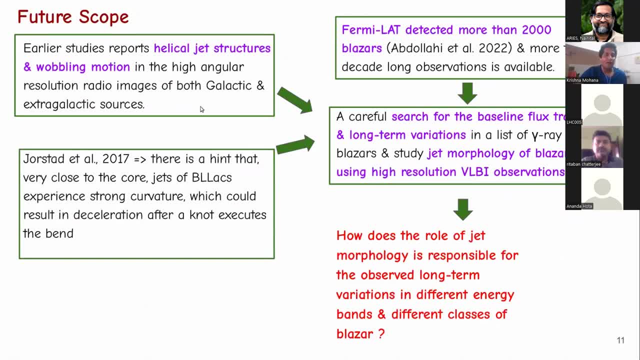 years. so what is the future scope of years? so what is the future scope of this work? of course this is done for one, this work. of course this is done for one, this work. of course this is done for one particular source, particular source, particular source we have from the literature that there. 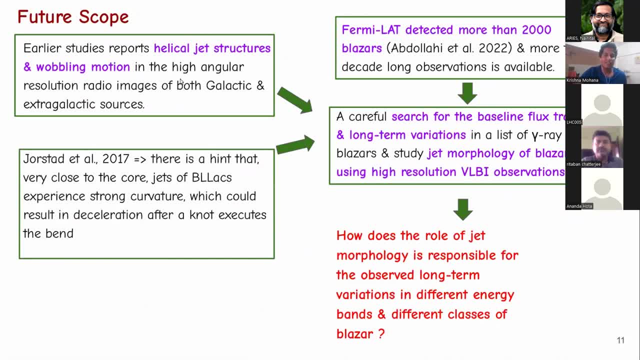 we have from the literature that there. we have from the literature that there are. people have reported helical jet. are people have reported helical jet? are people have reported helical jet structures and wobbling motions in the structures and wobbling motions in the? 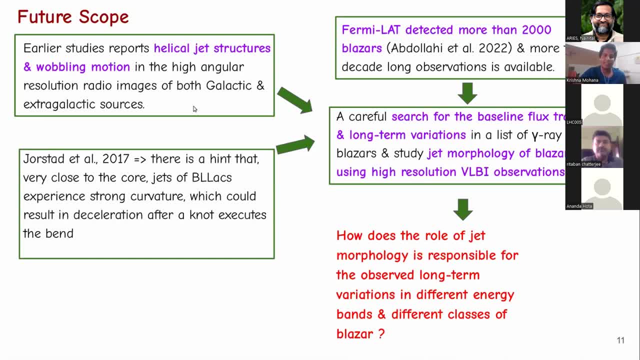 structures and wobbling motions in the, which have been seen in the high angular, which have been seen in the high angular, which have been seen in the high angular resolutions of the radio images, in the resolutions of the radio images, in the resolutions of the radio images in the galactic and extra galactic objects, and 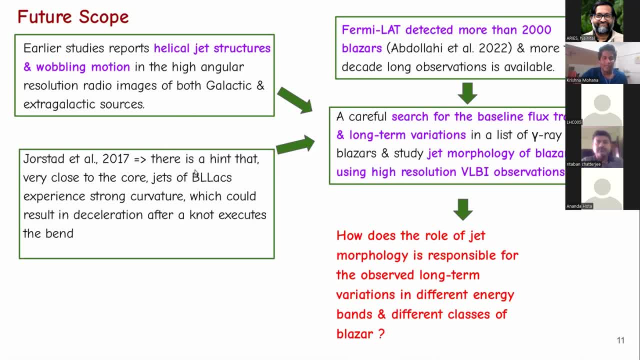 galactic and extra galactic objects, and galactic and extra galactic objects, and also also also joshua 2017. uh, they suggest that their joshua 2017. uh, they suggest that their joshua 2017. uh, they suggest that their observation suggests that there is a hint. 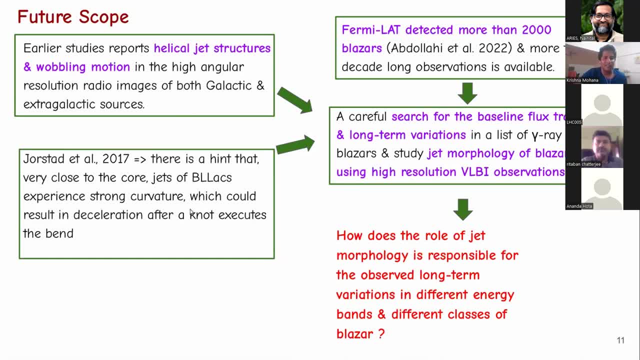 observation suggests that there is a hint. observation suggests that there is a hint that uh in the blx objects very close, that uh in the blx objects very close, that uh in the blx objects very close to the jets, they due to strong to the jets, they due to strong. 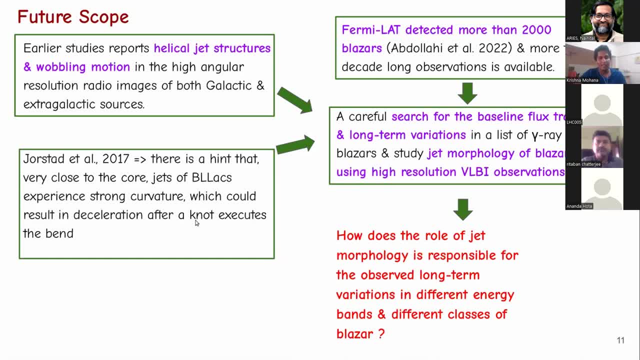 to the jets. they. due to strong curvature, which curvature, which curvature, which the. the deceleration of the blob could the. the deceleration of the blob could the. the deceleration of the blob could lead to the lead to the, lead to the, a lead to the uh. due to the bank, the. 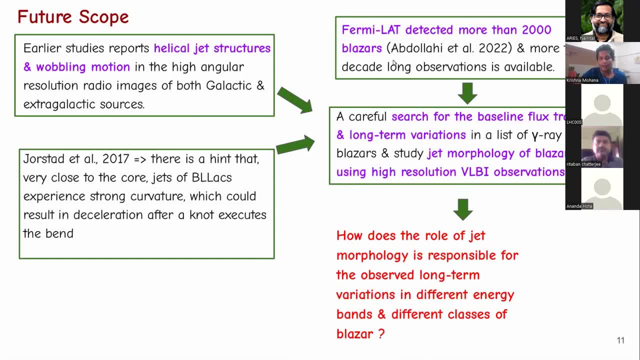 a lead to the uh due to the bank. the a lead to the uh due to the bank. the deceleration of the blob: could deceleration of the blob? could deceleration of the blob could happen and uh, we have right now happen and uh, we have right now. 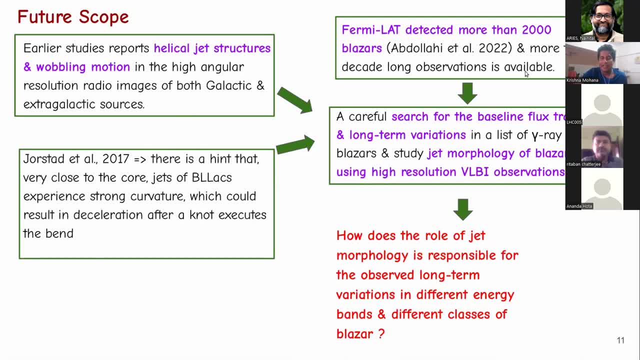 happen. and uh, we have right now formula, formula, formula with more than 2000 lasers and decade with more than 2000 lasers and decade with more than 2000 lasers and decade long observation is available. a careful long observation is available. a careful long observation is available. a careful investigation for a list of the 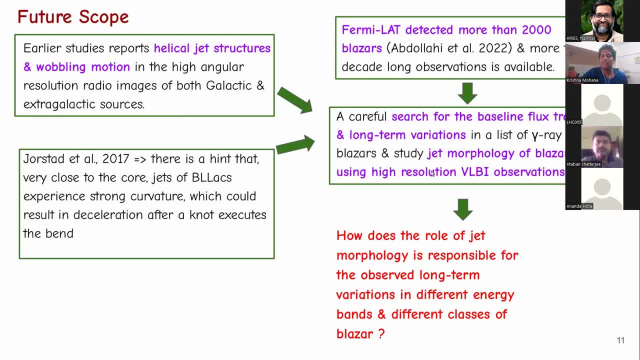 investigation. for a list of the investigation. for a list of the careful investigation in the. to look for careful investigation in the. to look for careful investigation in the. to look for the baseline flux transition for a. the baseline flux transition for a. the baseline flux transition for a list of a bright gamma ray well monitored. 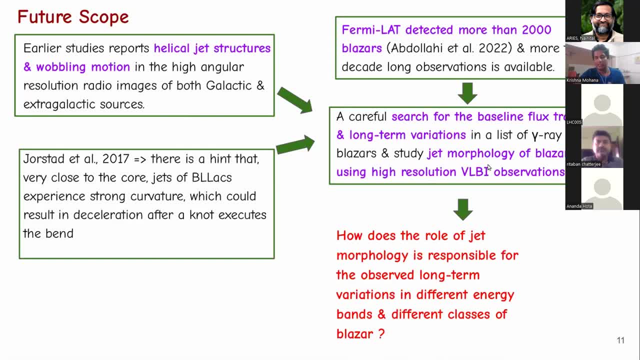 list of a bright gamma ray well monitored. list of a bright gamma ray well monitored source is required, along with the source is required, along with the source is required along with the uh, along with the the observations, uh, along with the the observations, uh. along with the the observations, we will be a high resolution. 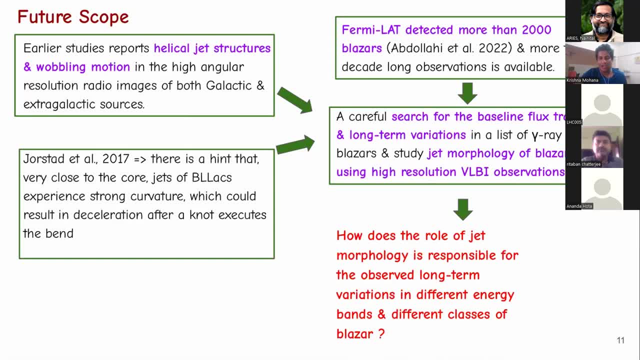 we will be a high resolution. we will be a high resolution. observations: to understand these jet observations. to understand these jet observations. to understand these jet morphologies- how they are going to play morphologies, how they are going to play morphologies, how they are going to play the. is that the baseline flux transition? 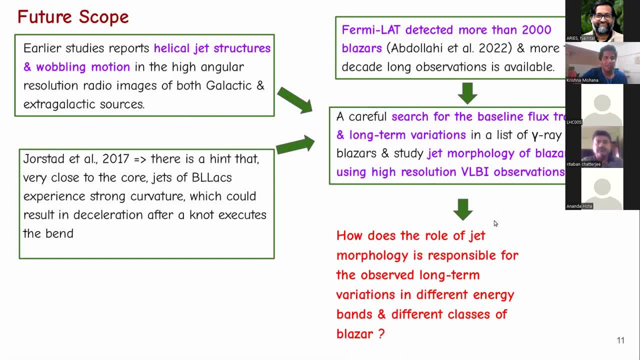 the is that the baseline flux transition, the is that the baseline flux transition, or the long-term variations in different, or the long-term variations in different, or the long-term variations in different classes of lasers. so i would like to classes of lasers, so i would like to. 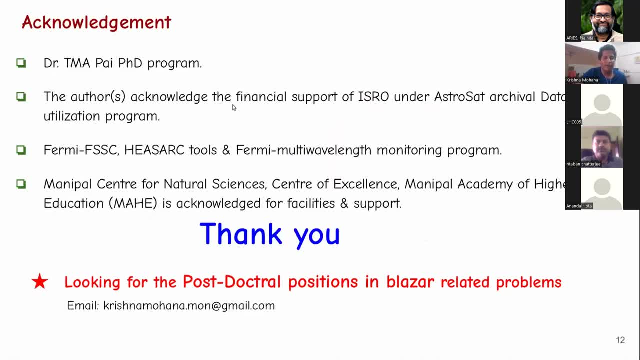 classes of lasers. so i would like to thank uh, thank uh, thank uh. dr tmfi phd program and authors are dr tmfi phd program and authors are dr tmfi phd program and authors are: acknowledged to acknowledge the financial. acknowledged to acknowledge the financial. 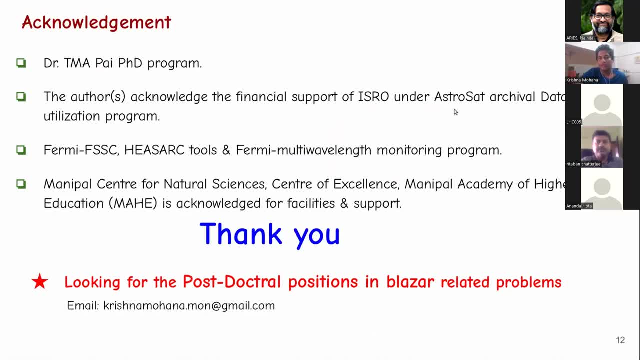 acknowledged. to acknowledge the financial support of the uh is isro and support of the uh isro. and support of the uh isro and isro. financial support from this row under isro. financial support from this row under isro. financial support from this row under the astrocyte: archival data. 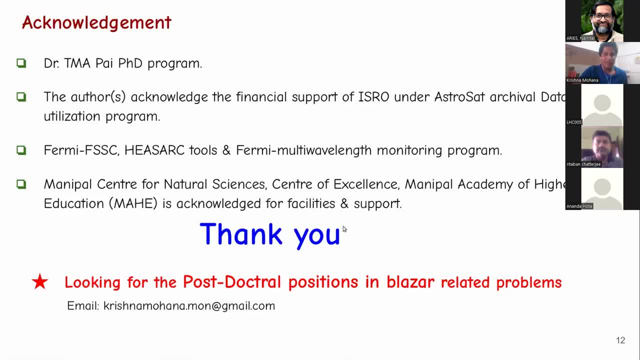 the astrocyte archival data. the astrocyte archival data utilization program also. i would like utilization program also. i would like utilization program also. i would like to mention: bring to you all people you to mention. bring to you all people you to mention. bring to you all people you want to notice is that i am about to. 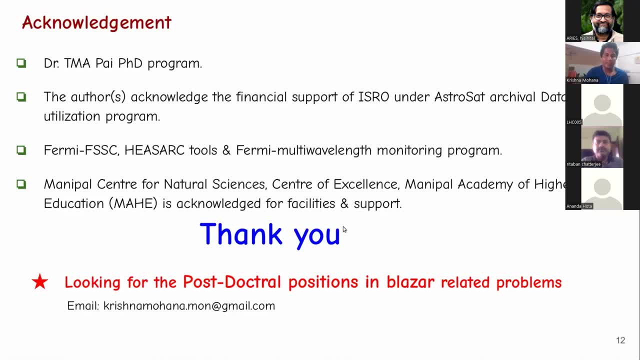 want to notice is that i am about to want to notice is that i am about to finish, finish, finish my phd- about to submit a thesis in a. my phd about to submit a thesis in a. my phd about to submit a thesis in a couple of months. and 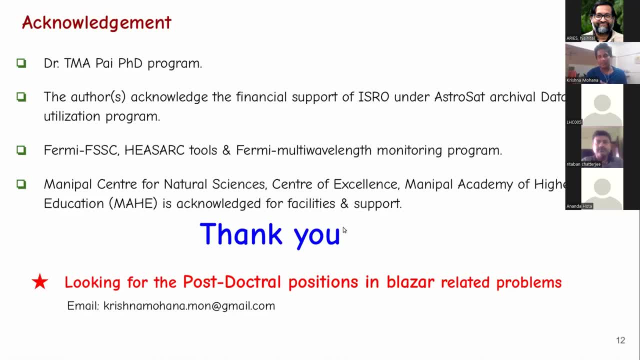 couple of months and couple of months, and right now i'm looking for the postdoctoral. right now i'm looking for the postdoctoral. right now i'm looking for the postdoctoral positions which, especially positions which, especially positions which, especially, uh, i would like to work in the blazer. 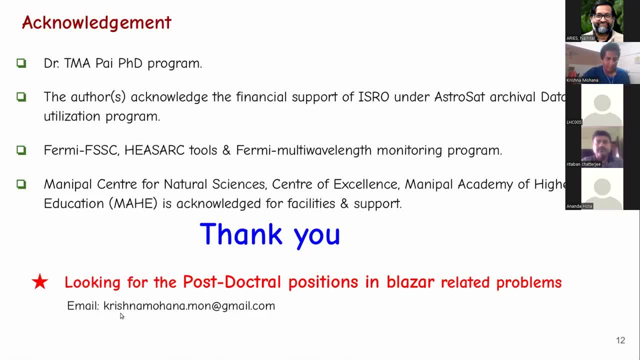 uh, i would like to work in the blazer. uh, i would like to work in the blazer. related problems, related problems. related problems. if anybody is interested, they can. if anybody is interested, they can. if anybody is interested, they can contact me, thank you. thank you for the 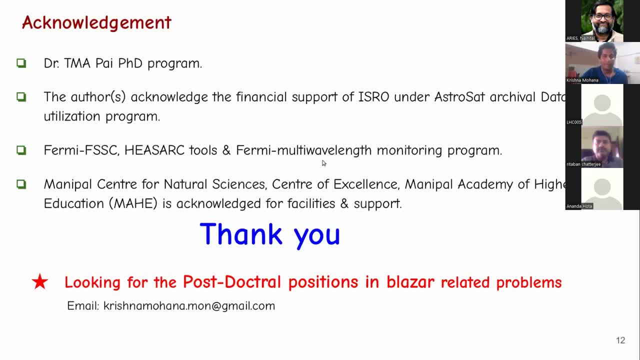 contact me. thank you, thank you for the contact me. thank you, thank you for the opportunity to share this work, opportunity to share this work, opportunity to share this work. okay, um, thank you for the talk. so is okay, um, thank you for the talk. so is okay, um, thank you for the talk. so is there any question in the? in the 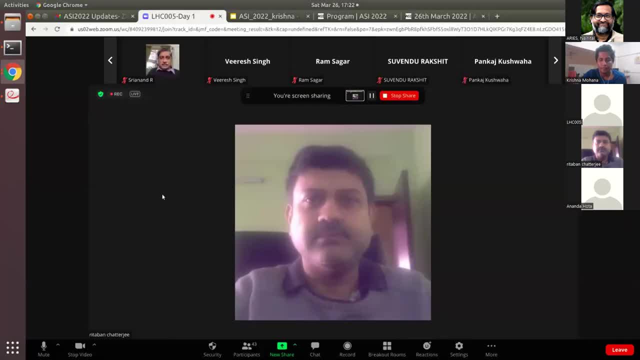 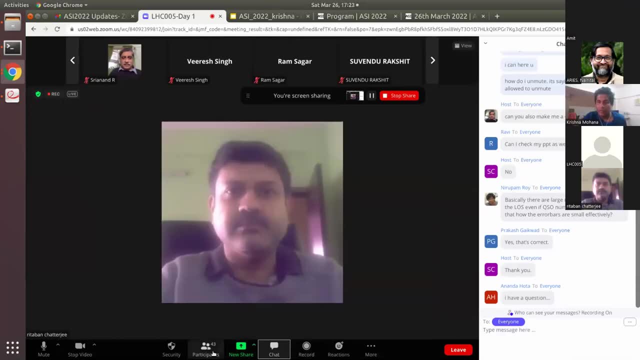 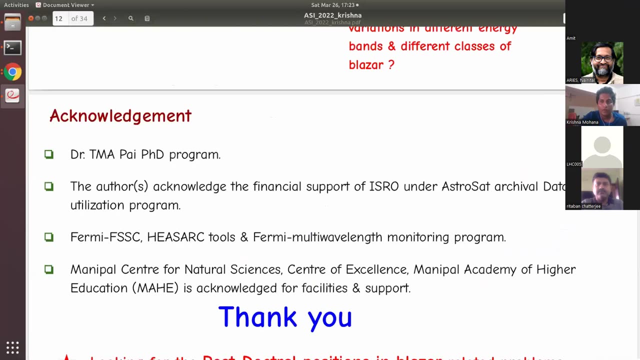 there any question in the in the there any question in the in the audience? hi uh, actually, can you switch to the hi uh, actually, can you switch to the hi uh, actually, can you switch to the slide in which you slide, in which you slide, in which you yeah, the change in the average flux. 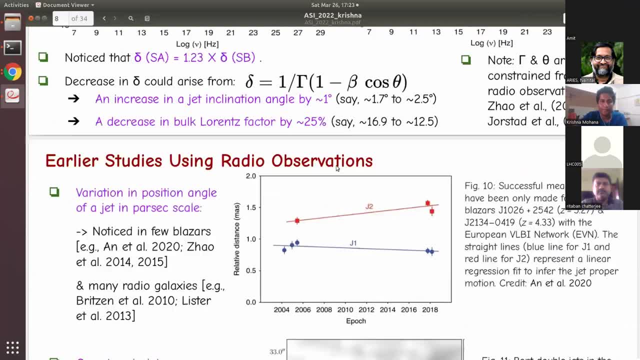 yeah, the change in the average flux, yeah, the change in the average flux, change in the average flux. this one, yeah, this one. this one, yeah this one. this one, yeah, this one. so is it an averaging effect or uh have? so, is it an averaging effect or uh have? 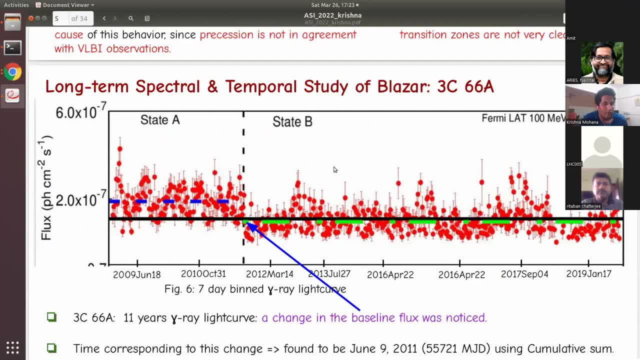 so is it an averaging effect or uh, have you looked at final? you looked at final, you looked at final? winning of the low state. i mean the winning of the low state. i mean the winning of the low state. i mean the state b, state b, state b. uh, is there a hands flux in state b? if? 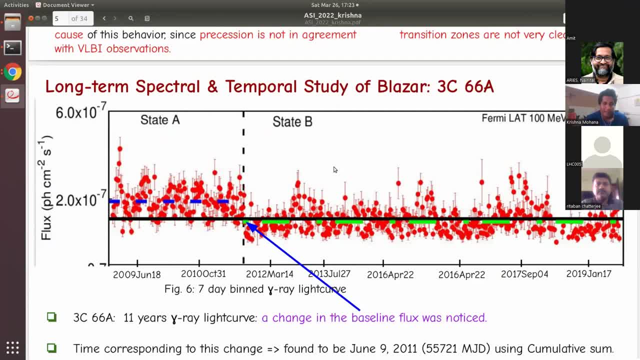 uh, is there a hands flux in state b? if uh, is there a hands flux in state b? if we do a final winning of the slide, we do a final winning of the slide. we do a final winning of the slide. yeah, this is uh. yeah, this is uh. 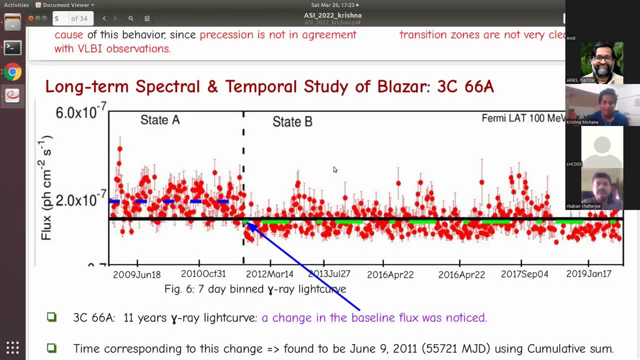 yeah, this is uh for that. is it driven by the flaring for that? is it driven by the flaring for that? is it driven by the flaring activities or the other fluctuations? what activities or the other fluctuations? what activities or the other fluctuations? what we did is we also studied the poison. 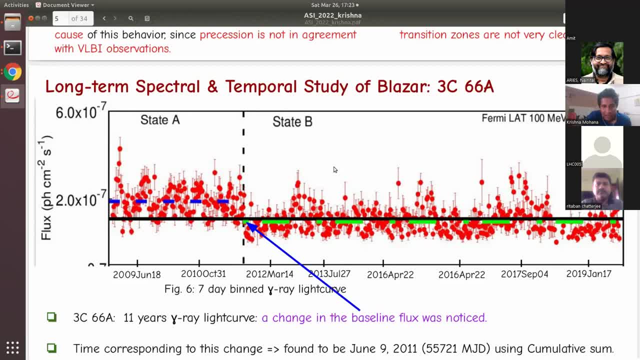 we did is we also studied the poison. we did is we also studied the poison behavior, behavior, behavior, poison behavior. what we did is that we, what we did is that we, what we did is that we need not include those fluxes, need not include those fluxes. 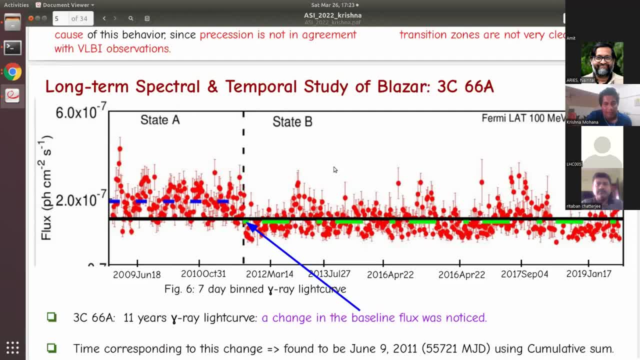 need not include those fluxes: flux, the time periods in the data flux, the time periods in the data flux, the time periods in the data and and and where the flux is where the flux is, where the flux is greater than the average flux. we only greater than the average flux, we only. 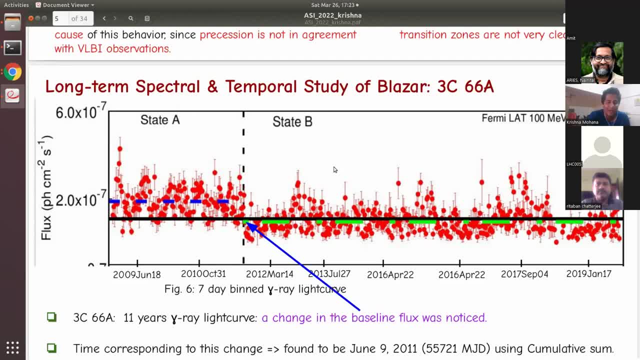 greater than the average flux. we only considered it. either it is a lesser than considered it, either it is a lesser than considered it, either it is a lesser than the average flux in the particular state, the average flux in the particular state, the average flux in the particular state, or lesser than. 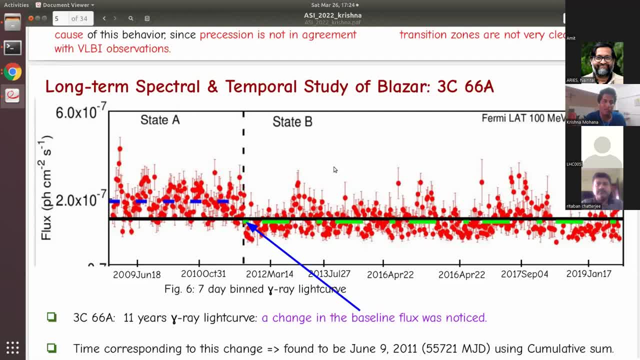 or lesser than or lesser than, equal or lesser than that. that means equal or lesser than that. that means equal or lesser than that. that means that automatically it removes the all that. automatically, it removes the all that. automatically, it removes the all those flaring activities. so from the 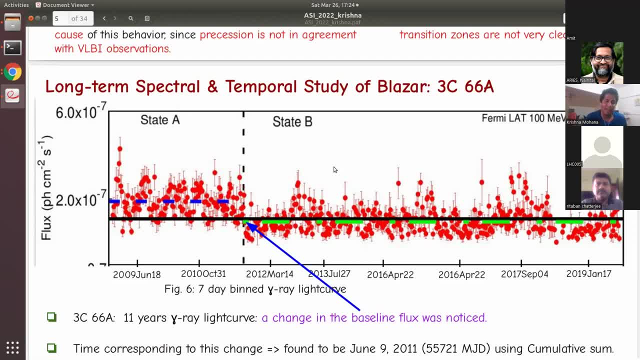 those flaring activities. so from the those flaring activities, so from the gamma analysis, we gamma analysis, we gamma analysis, we find a similar uh flux variation. so the find a similar uh flux variation, so the find a similar uh flux variation. so the average flux variation is changing. the. 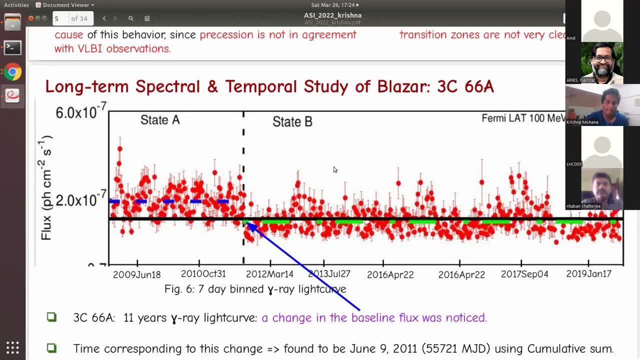 average flux variation is changing. the average flux variation is changing. the cosine in state b: you have excluded all those in state b. you have excluded all those in state b. you have excluded all those points when the flux is exceeding the points when the flux is exceeding the. 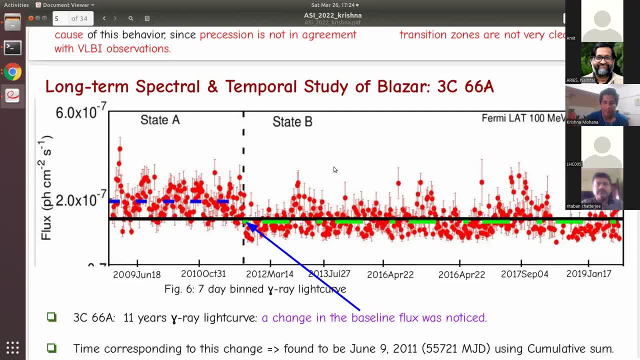 points when the flux is exceeding the average flux. average flux, average flux. yes, you have to find the average flux. yes, you have to find the average flux. yes, you have to find the average flux with the green line, with the green line, with the green line, yes, okay, so, uh, it is a discontinuous. 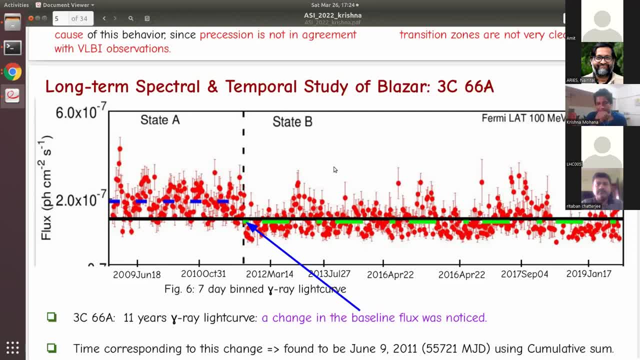 yes, okay, so, uh, it is a discontinuous- yes, okay, so, uh, it is a discontinuous data, data, data, and you have developed this, yeah this, and you have developed this, yeah this, and you have developed this, yeah, this. continuous data in the sense all these continuous data in the sense all these. 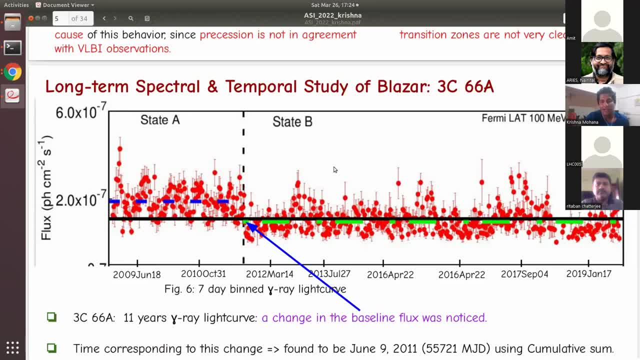 continuous data in the sense, all these red color data points: they are detected. red color data points: they are detected. red color data points: they are detected. points, these are points, these are points. these are three sigma detected weekly detected: three sigma detected weekly detected. three sigma detected weekly detected point: these are detection points. 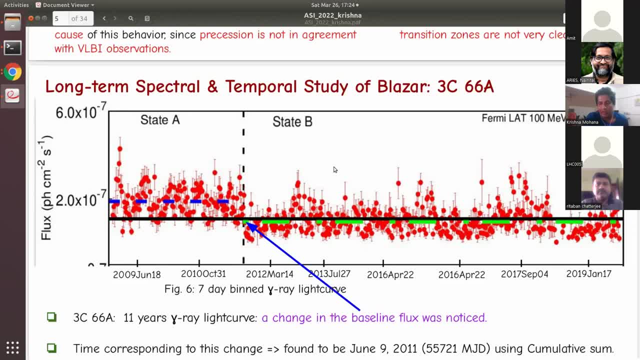 point. these are detection points. point. these are detection points. in between: there are upper limits. those in between: there are upper limits, those in between there are upper limits, those upper limit data points. i have not upper limit data points. i have not upper limit data points. i have not included. 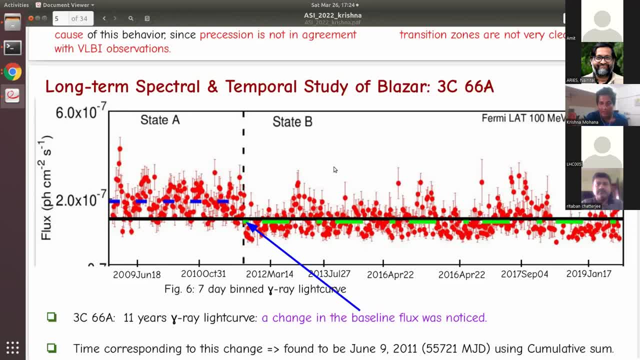 included, included. so what happens is that there is one. so what happens is that there is one. so what happens is that there is one particular, particular, particular technique in the fermi lat. it is called technique in the fermi lat. it is called technique in the fermi lat. it is called some likelihood analysis. 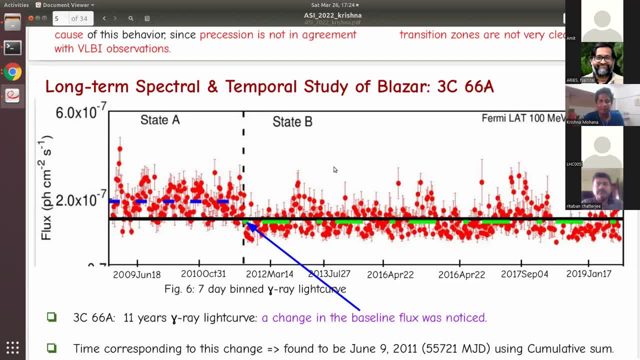 some likelihood analysis, some likelihood analysis: where, where, where you can at a different time interval, if you can at a different time interval, if you can at a different time interval, if the data, the data, the data, is in a different time ranges, you can is in a different time ranges, you can. 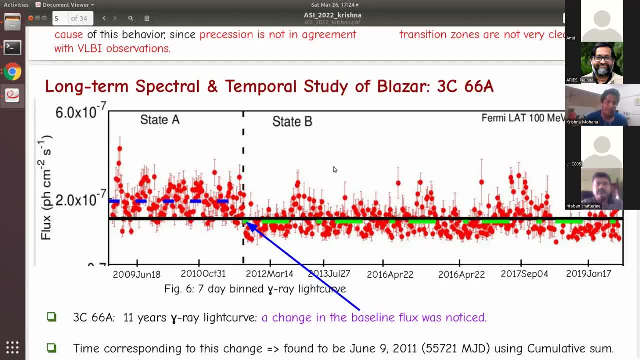 is in a different time ranges, you can choose those time intervals and do the choose those time intervals and do the choose those time intervals and do the analysis, analysis, analysis. so that is what, okay, and i also want to. so that is what, okay, and i also want to. 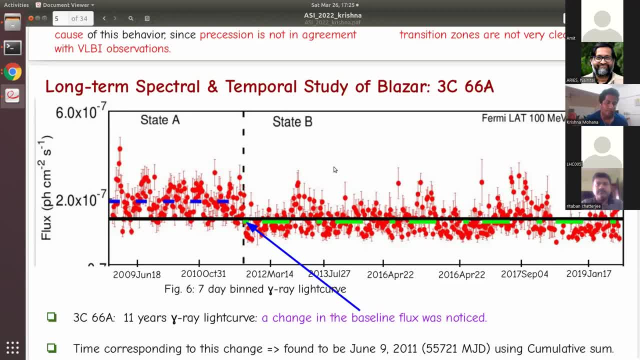 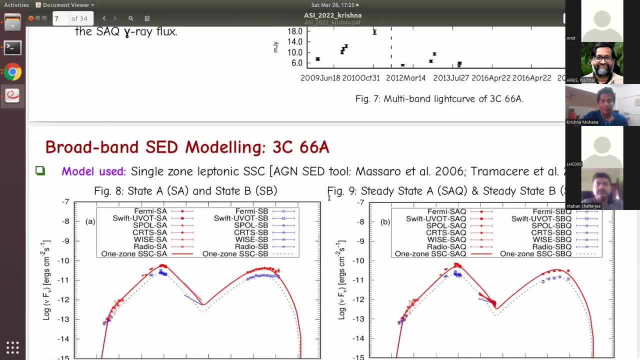 so that is what? okay, and i also want to know that: how have you know that? how have you know that? how have you changed the state a and state b? uh, changed the state a and state b. uh, changed the state a and state b. uh, exactly similar. 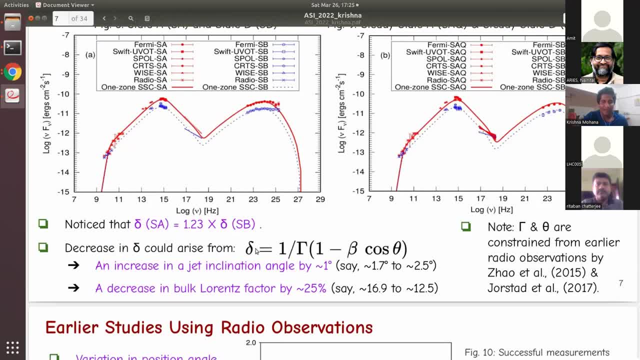 exactly similar, exactly similar. and we have. we change the tweak to only. and we have. we change the tweak to only. and we have. we change the tweak to only: the doppler beaming factor, the doppler beaming factor, the doppler beaming factor and this doppler that could change the 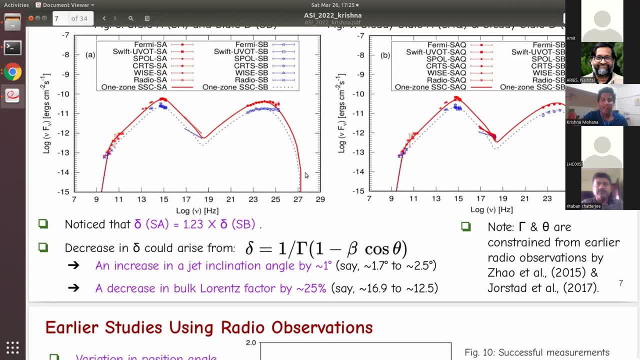 and this doppler that could change the and this doppler that could change the doppler beaming factor itself. doppler beaming factor itself, doppler beaming factor itself, could explain the state a to state b and could explain the state a to state b. and. 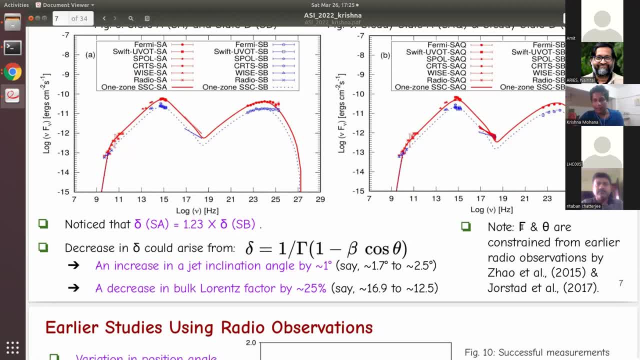 could explain the state a to state b and i will also. i will also. i will also bring your notice that the people could bring your notice, that the people could bring your notice, that the people could can ask how about the can ask how about the can ask how about the. if you change this automatically, your. 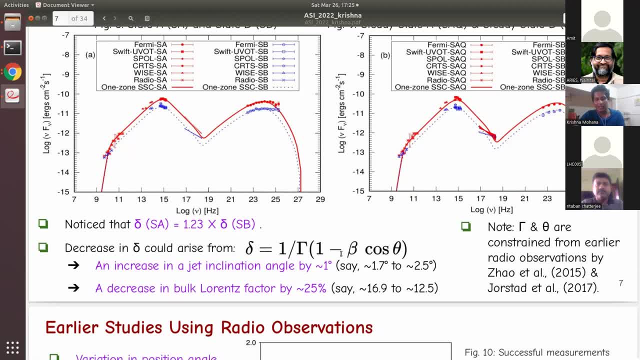 if you change this automatically, your- if you change this automatically, your delta will change. then we looked for delta will change. then we looked for delta will change. then we looked for this delta has the two factors. one is a. this delta has the two factors. one is a. 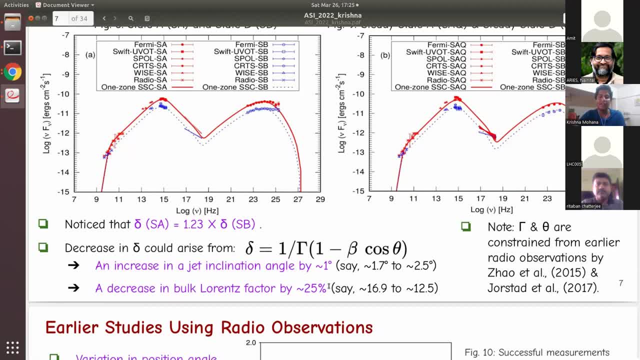 this delta has the two factors: one is a doppler beaming for this bulk florence doppler beaming for this bulk florence doppler beaming for this bulk florence factor. and theta this can factor and theta this can factor and theta this can. this variation is very consistent with 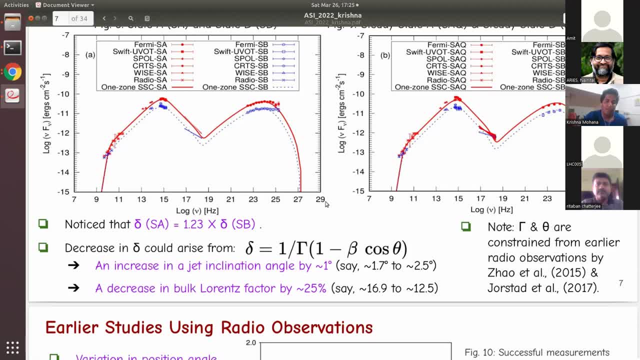 this variation is very consistent with. this variation is very consistent with the what is observed in the radio radio, the what is observed in the radio radio, the what is observed in the radio radio. observations, observations, observations. okay, so i think we have to move on now. okay, so i think we have to move on now. 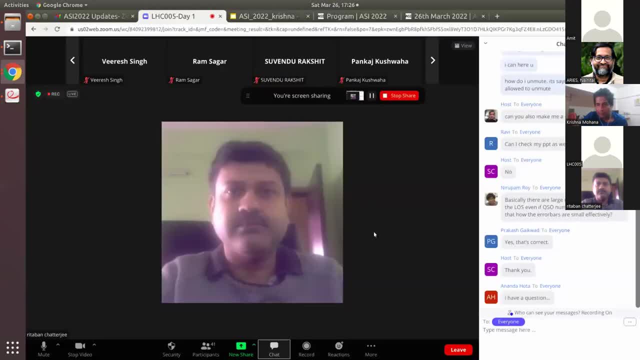 okay, so i think we have to move on now. um, so we'll have one question from the um. so we'll have one question from the um. so we'll have one question from the zoom session. so amit has a question, zoom session. so amit has a question. 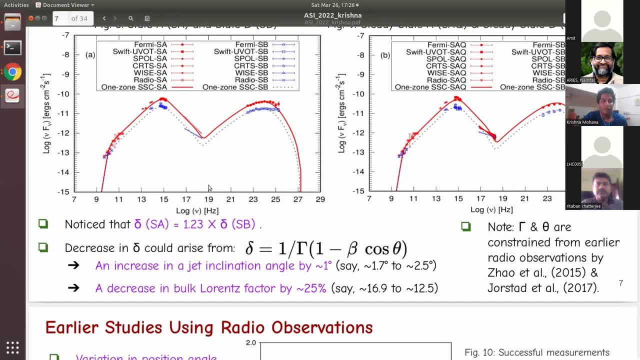 zoom session. so amit has a question. could you please just ask one question? could you please just ask one question? could you please just ask one question? and and uh krishna, could you please? and and uh krishna, could you please? and and uh krishna, could you please keep the answer to the point. 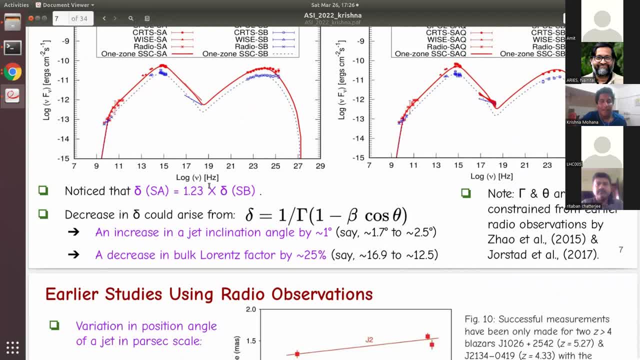 keep the answer to the point. keep the answer to the point. yes, yes, sure, yeah, hi krishna, very yes, yes, sure, yeah, hi krishna, very yes, yes, sure, yeah, hi krishna. very impressed in work, impressed in work, impressed in work. i have one thing to which i am quite. 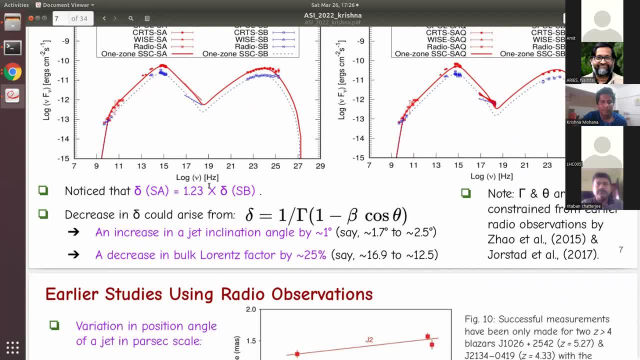 i have one thing to which i am quite. i have one thing to which i am quite interested: that you showed that, uh, your interested that you showed that, uh, your interested. that you showed that, uh, your blob or the jet is getting bended around. blob or the jet is getting bended around. 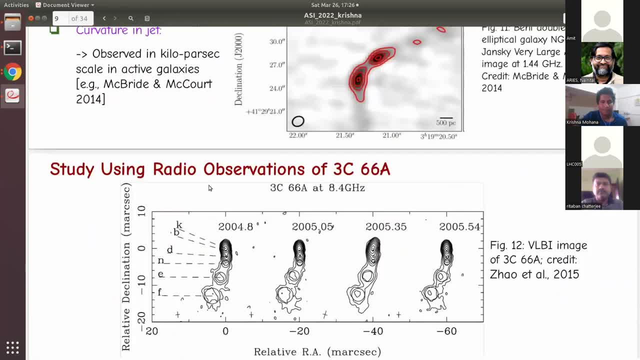 blob or the jet is getting bended around: 700 parsecs, right. 700 parsecs right- 700 parsecs, right, yes, yeah. so if you take you and you are yes, yeah. so if you take you and you are, yes, yeah. so if you take you and you are trying to explain your acp through, 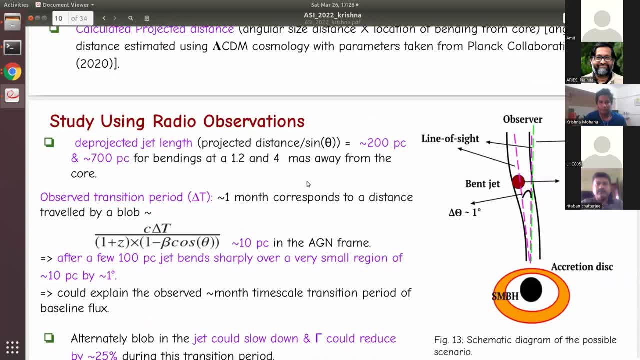 trying to explain your acp through, trying to explain your acp through synchrotron self-prompting emission. so synchrotron self-prompting emission, so synchrotron self-prompting emission. so let's say, if you start with some, 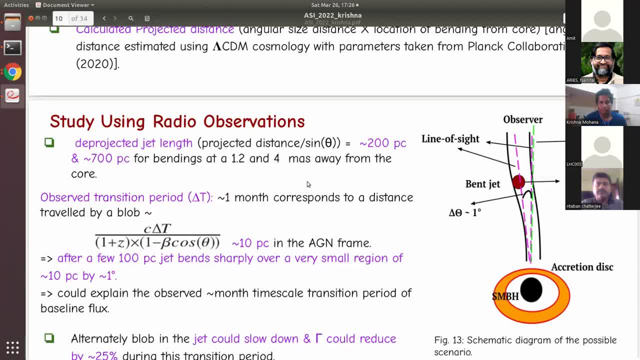 let's say, if you start with some, let's say if you start with some particles, if they travel that much particles, if they travel that much particles, if they travel that much distance, they will lose their energy distance. they will lose their energy distance, they will lose their energy. and probably you need 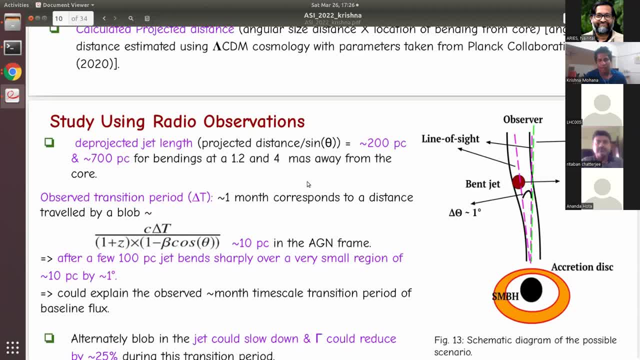 and probably you need, and probably you need to have the magnetic field as well as to have the magnetic field, as well as to have the magnetic field as well as your particles to be accelerated, your, your particles to be accelerated, your, your particles to be accelerated. your blob should not expand, so magnetic will. 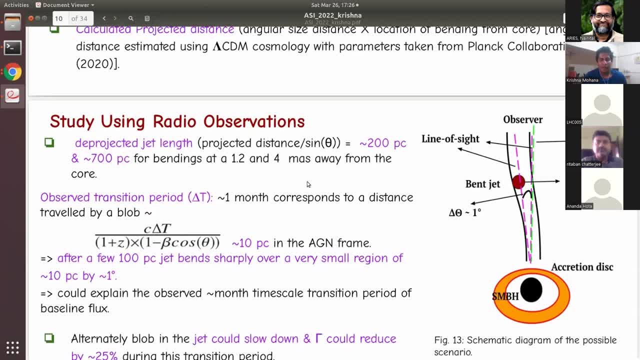 blob should not expand, so magnetic will. blob should not expand, so magnetic will get diluted. so how you are managing get diluted, so how you are managing get diluted, so how you are managing this in your model, this in your model, this in your model. you know, you know. 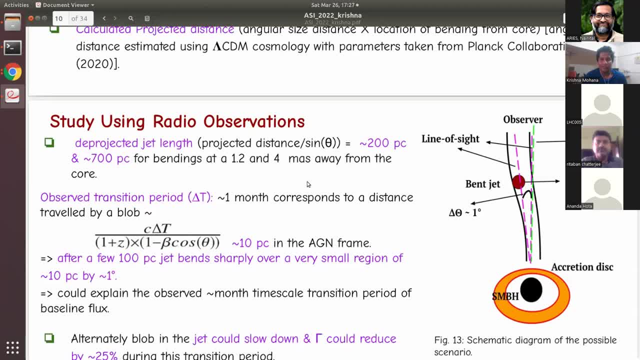 you know, this is actually, this is not a temporal. this is actually this is not a temporal. this is actually this is not a temporal model. actually, this is a static model model. actually, this is a static model and, uh, what we did is that we are not, and, uh, what we did is that we are not. 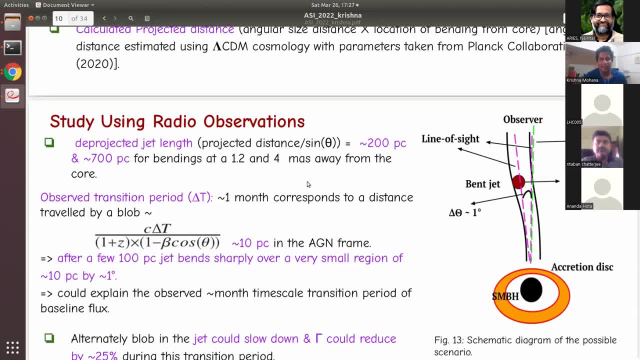 and uh. what we did is that we are not claiming that it is claiming that. it is claiming that it is. uh, the blob is bending at uh 700. uh, the uh, the blob is bending at uh 700. uh, the uh, the blob is bending at uh 700. uh, the blob is moving at 700 parsecs. 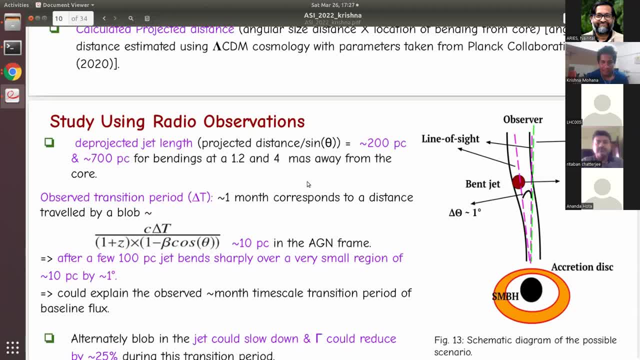 blob is moving at 700 parsecs. blob is moving at 700 parsecs. we are saying that it could either go. we are saying that it could either go. we are saying that it could either go through any of this, uh, through any of this, uh, through any of this, uh, hundred of a parsec. it is just roughly. 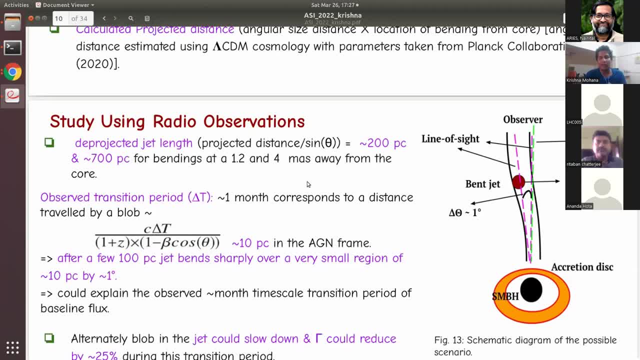 hundred of a parsec, it is just roughly. hundred of a parsec, it is just roughly. it is not a strong claim. i know that it is not a strong claim. i know that it is not a strong claim. i know that after a certain parsecs, these uh. 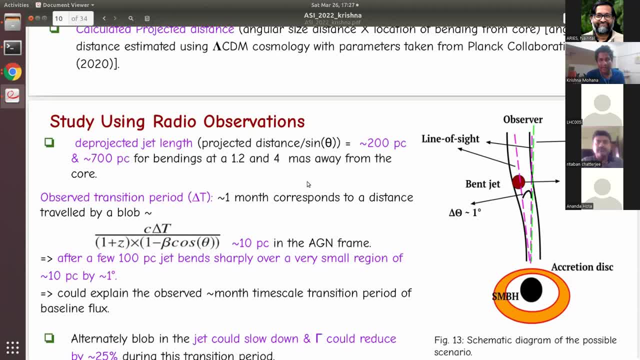 after a certain parsecs, these uh. after a certain parsecs, these uh the blob. can uh the blob, can uh the blob, can uh lose the energy. so that is what we are: lose the energy. so that is what we are, lose the energy. so that is what we are also saying, that. 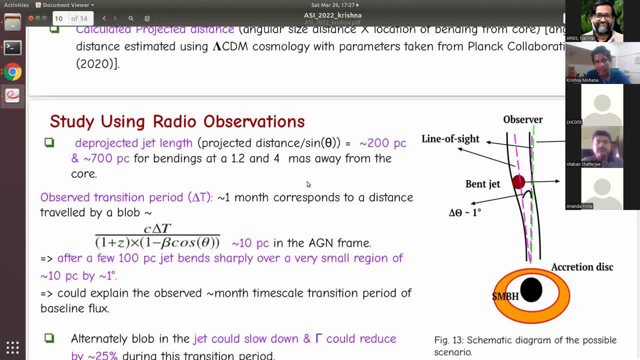 also saying that, also saying that the change in the bulk chlorine factor, the change in the bulk chlorine factor, the change in the bulk chlorine factor itself, could itself, could itself, could itself, can explain this one. i understand itself, can explain this one. i understand itself, can explain this one. i understand the your question, but, uh, we are not. 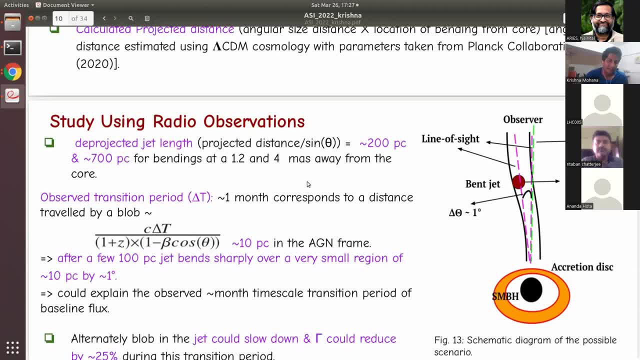 the your question. but uh, we are not the your question. but uh, we are not strongly claiming on the strongly claiming on the strongly claiming on the. what is this the the jet? what is this the the jet? what is this the the jet is one of the scenario we are saying. is one of the scenario we are saying is one of the scenario. we are saying that it could be the one of the, that it could be the one of the, that it could be the one of the possible is one of the scenario. possible is one of the scenario. 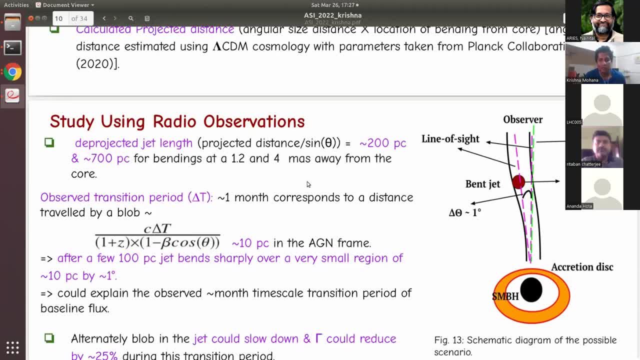 possible is one of the scenario. so we have to further look for many. so we have to further look for many. so we have to further look for many other blazer quarters, other blazer quarters, other blazer quarters. okay, so i i think we have to move on to. 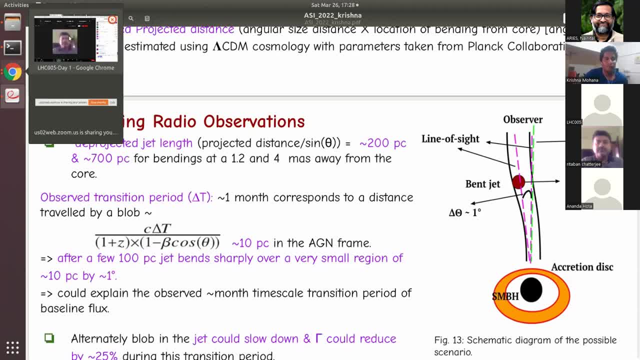 okay, so i i think we have to move on to. okay, so i i think we have to move on to the. to the final talk now, the. to the final talk now, the. to the final talk now. and uh, so, if you have, if there are other. and uh, so, if you have, if there are other. 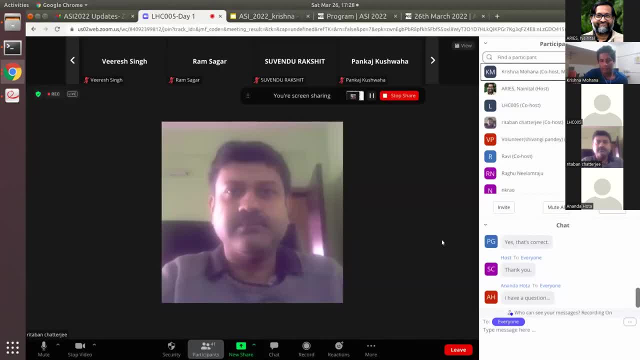 and uh. so, if you have, if there are other questions, please contact the speaker questions. please contact the speaker questions. please contact the speaker. after the session. um, and we'll move on after the session. um, and we'll move on after the session. um, and we'll move on to the final talk of the session. 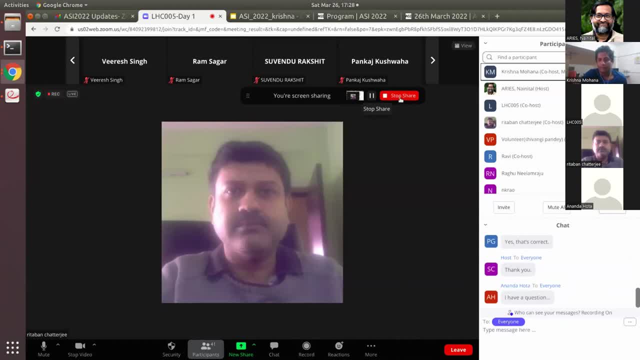 to the final talk of the session. to the final talk of the session by ravi joshi. the title of the talk is by ravi joshi. the title of the talk is by ravi joshi. the title of the talk is x-shaped radio galaxies. 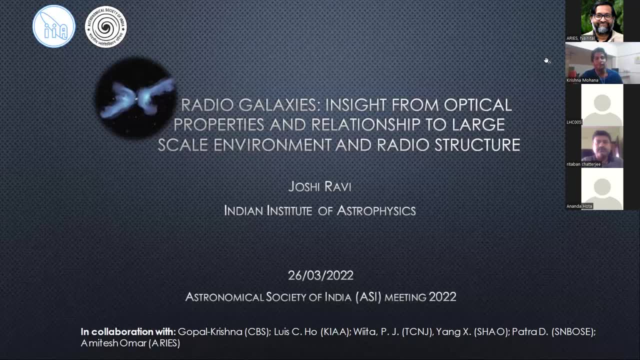 x-shaped radio galaxies. x-shaped radio galaxies: inside from optical host properties. inside from optical host properties. inside from optical host properties. environment and radio structure. environment and radio structure. environment and radio structure. so ravi, yes, so i can uh, we can see. so ravi, yes, so i can uh, we can see. 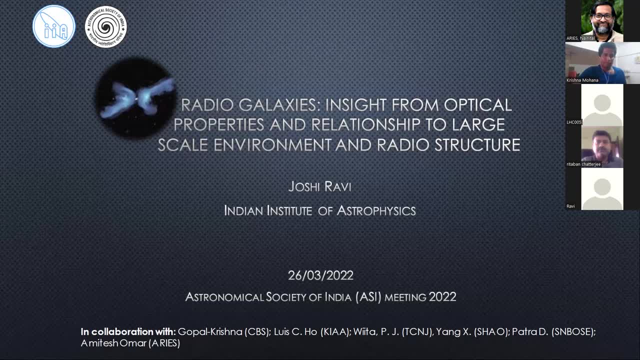 so ravi, yes, so i can uh, we can see your uh, your uh, your uh. thank you. yeah, so thanks uh. so thank you. yeah, so thanks uh, so thank you. yeah, so thanks uh. so first of all, i would like to thanks the first of all i would like to thanks the. 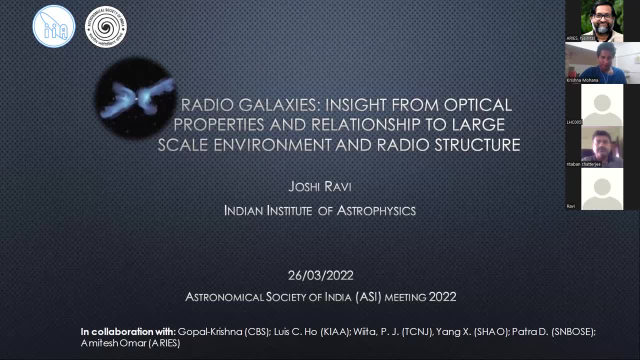 first of all, i would like to thanks the organizers for giving this opportunity. organizers for giving this opportunity. organizers for giving this opportunity. so i'll be discussing about our. so i'll be discussing about our. so i'll be discussing about our recent effort to understand the recent effort to understand the. 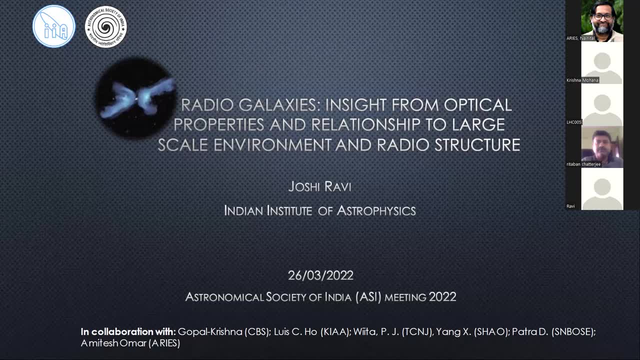 recent effort to understand the x-shaped radio galaxies. that will be x-shaped radio galaxies that will be x-shaped radio galaxies that will be primarily from the, primarily from the, primarily from the optical host galaxy perspective. optical host galaxy perspective. optical host galaxy perspective. and the collaborators are listed here. 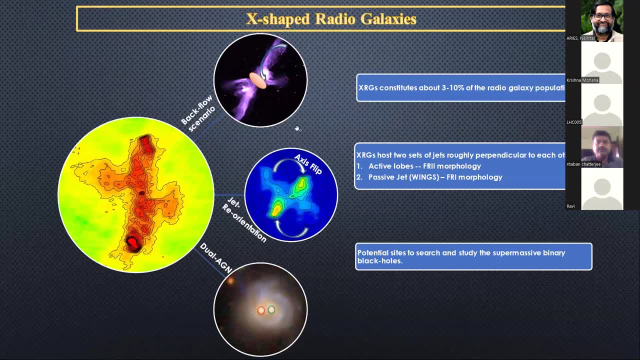 and the collaborators are listed here, and the collaborators are listed here. so what are the x-shaped radio galaxies? so what are the x-shaped radio galaxies? the kiloparsec to the megaparsec scales. However, there is roughly 3 to 10 percent of radio galaxies. 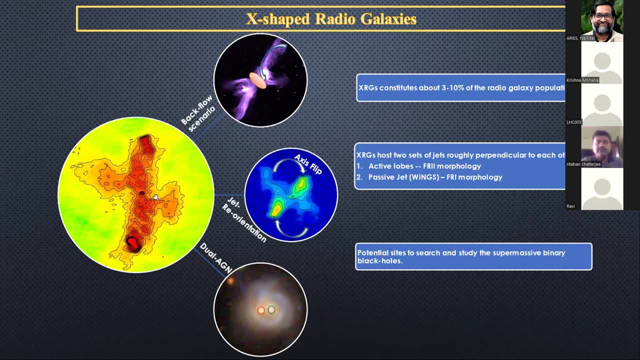 which shows a peculiar kind of morphology which you can see here. So what you see here is that you see a jet showing the hotspots- This is like conventional FR2 kind of radio morphology, which I will call like primary or the active jet- And then, other than this, you see a diffuse radio. 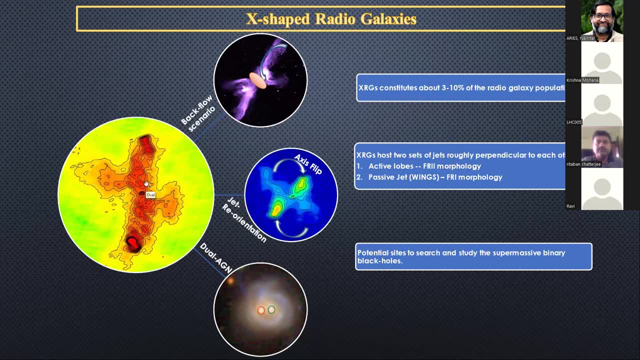 emission roughly at an angle of 90 degree with respect to the primary jet. These are typically of like a formal kind of morphology and overall it makes a shape of X. So these class of radio galaxies are called X-shaped radio galaxies. So what we know about them or how do they form? So 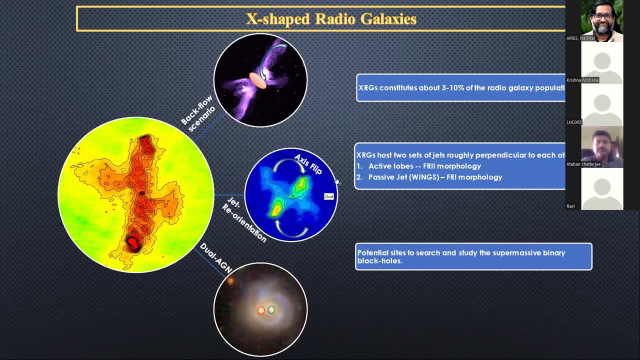 there are many scenarios that have been performed and few like. most discussed scenarios are, for instance, the backflow scenario, Where you can believe that plasma from the hotspots will flow back to the host and then it moves along the low pressure gradient direction, forming an X kind of structure. 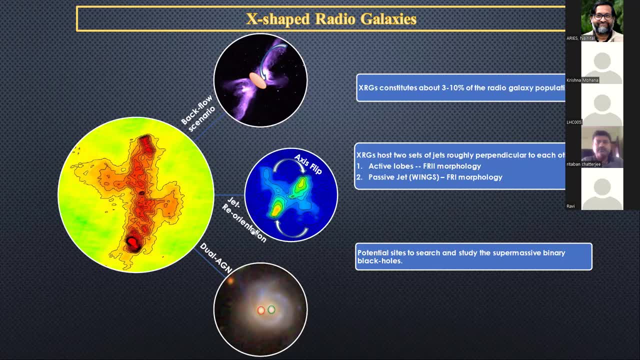 The other discussed model is jet reorientation model, where you can think that the diffuse structure, what you see here, this is nothing but the relic emission of previous jet activity And because of the merger probably the jet has been reoriented and now you see the active jet in. 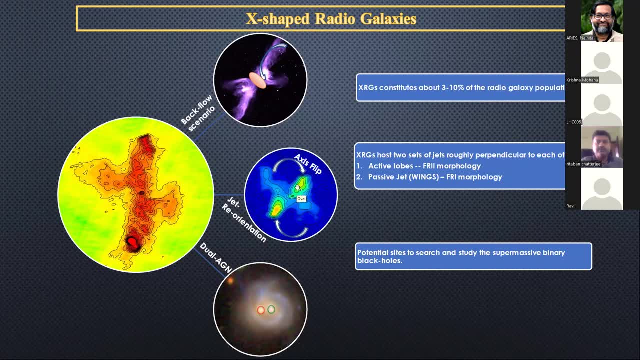 the middle of the host and then in the middle of the host it is reorienting, So this causes the formation of X-shaped structure. The third discussed scenario is probably the dual agent scenario, where we know that the mergers are prevalent, So it's possible that a galaxy hosting dual 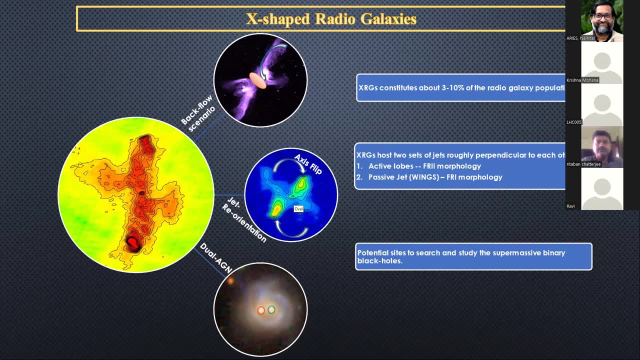 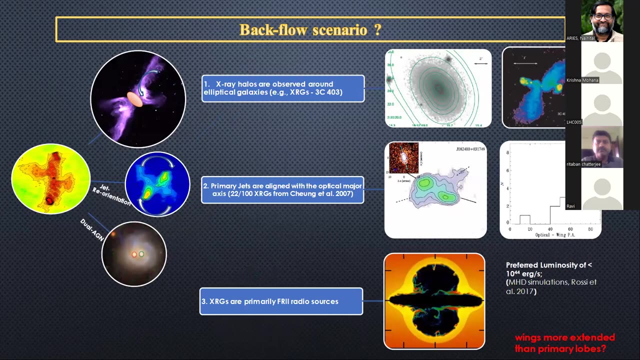 ATNs may be launching their own jets in two different directions, which will lead to the X kind of structure. So, however, there is no consensus so far. The reason being is that there are evidences in support and against in all the proposed models. For instance, if you, if you, look at the backflow scenario, then it's been found these in in most. 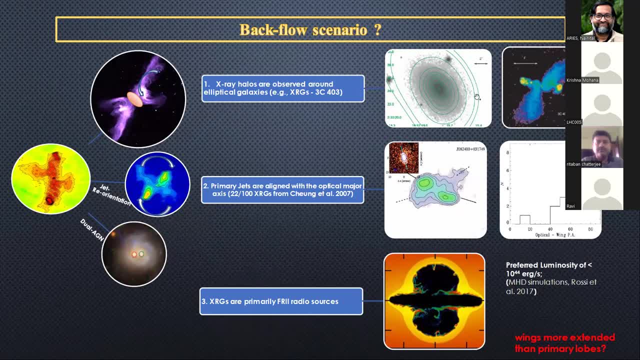 of. in several elliptical galaxies the gaseous halos has been found which extends like, sometimes even even larger distances than the optical of optical counterpart. So this kind of halos may lead to the diversion of the backflow plasma in a certain direction. The other evidence comes from a tight correlation. 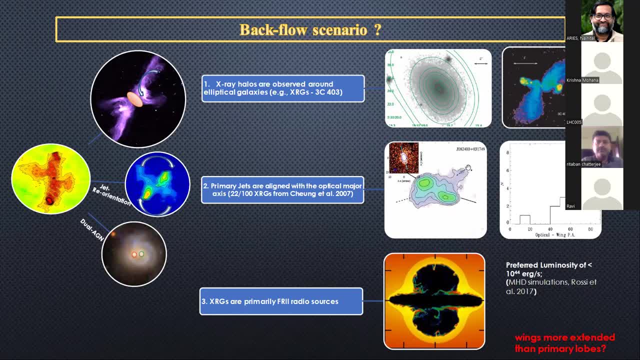 observed between the position angle of the wings, which are mostly, almost always- found to be always found to be aligned with respect to minor axis of the radio galaxies. So this again supports the backflow model. The third scenario comes from the morphology of the X-shaped radio galaxies which are preferentially found to be hosting FR2 kind of radio morphology. 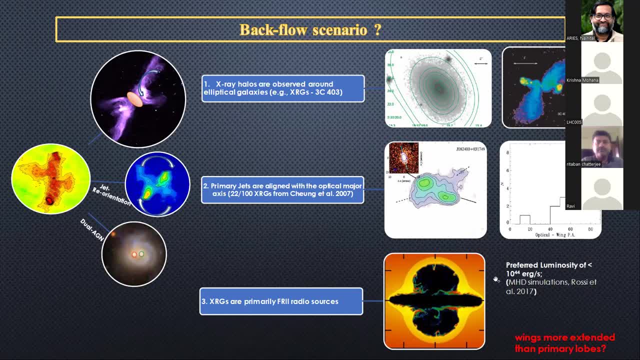 where you expect to see the hot spots, and even in the civilized simulations, also energy simulations also using it, It's been found that there is what is FR2 kind of radiomorphologies if you have a preferred luminosity less than 10 to 44.. 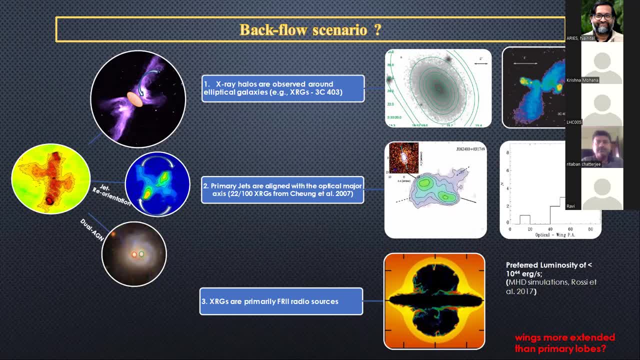 So then, this will lead to the X kind of structure. However, for some of the X-shaped radio galaxies, the wings are found to be even more extended than the primary jet. So so this backflow scenario model is not able to explain that why, in some 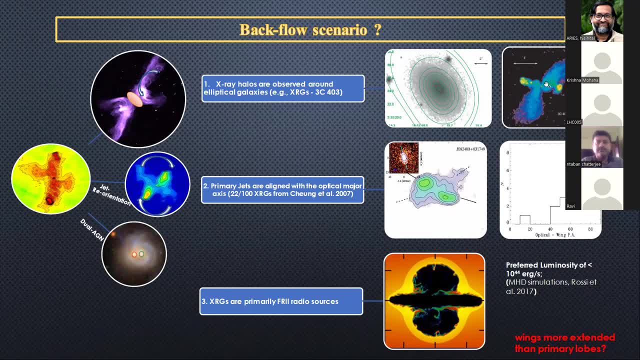 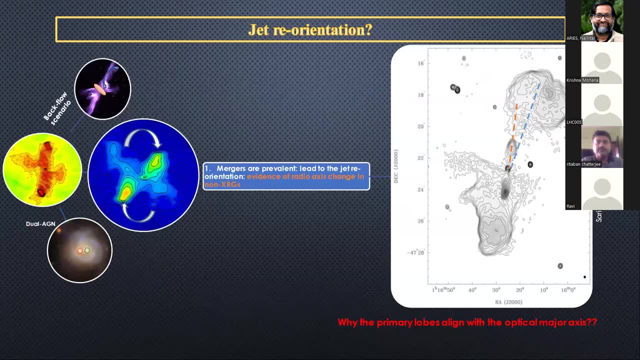 some of the cases is the plasma which is flowing with the supersonic speed. how can it go like even further than the active jet? So this phase here, The another possible scenario is the jet reorientation model. So it has been seen in observations that for some cases 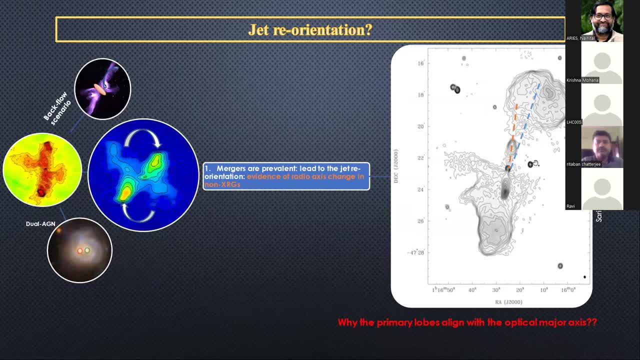 jet has been seen to be reoriented, For example. here is one of the examples. This is a double leader galaxy and if you look at the primary jet of this galaxy and the newly launched jet, there is a difference in the angle between two and if this angle is larger than certain. 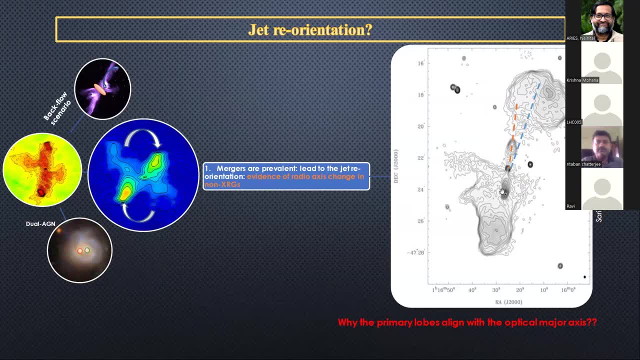 number, this will appear like an X kind of structure. However, this model does not explain that, why, for this galaxy, the primary jet should align with the major axis of the optical host. The third possible scenario is the dual or the binary agent scenario. So this is the 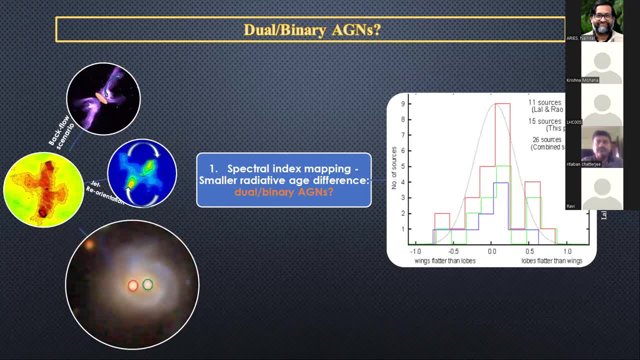 first example, So in this. so, for example, if you believe that the diffuse radio emission, what we see here, this is a relic of the previous jet activity, and if you do the spectral index mapping, then now you should. one should expect that the wings will have the steeper spectral. 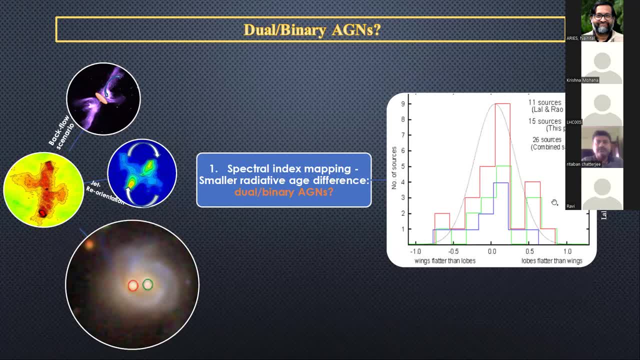 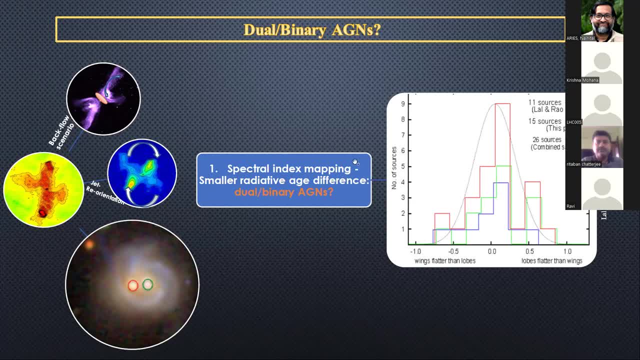 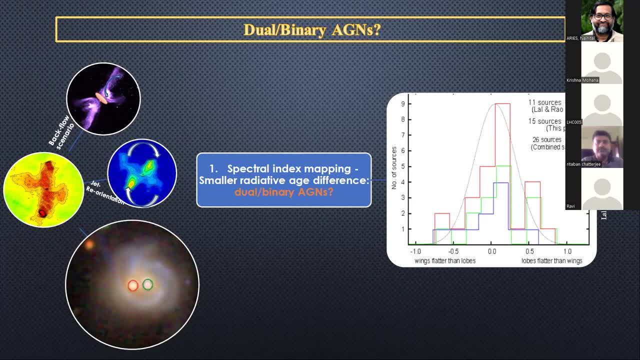 So what they found surprisingly is that sometimes the wings are relatively flatter than the. The reason being is that until recently, only about 100 X-shaped radio galaxies were discovered. So to understand like this formation of the X-shaped phenomena we have recently tried to 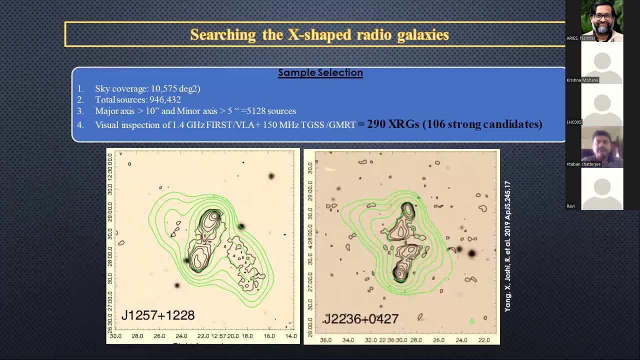 search for more such candidates. So for this we have searched these systems at 1.4 gigahertz, first VLA survey, This supplemented with the 150 megahertz TGSS GMRD survey. we have discovered about 290 X-shaped radio galaxies, And among them we have classified about 106 systems as strong. 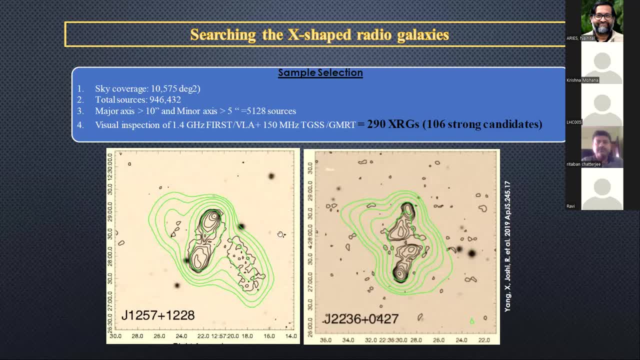 X-shaped radio galaxy candidates. So here are the two examples you can see for the strong X-shaped radio galaxy candidate: If you look at the black contour, these are the first 1.4 gigahertz images And a low X-shaped radio galaxy candidate is the first 1.4 gigahertz image And a low X-shaped radio galaxy candidate is the first 1.4 gigahertz image And a low. 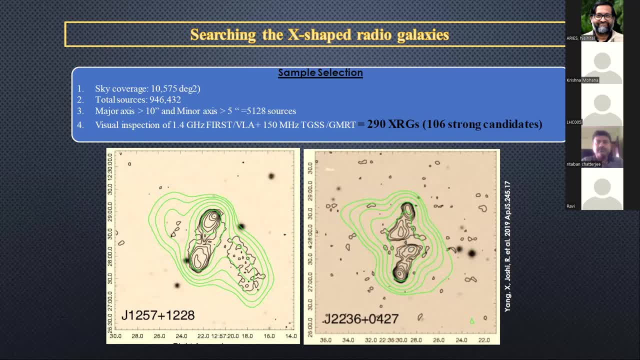 X-shaped radio galaxy candidate is the first 1.4 gigahertz symbol. This symbol means when looking at the first images, it's difficult to say that they are having actual structure. However, if you overlay the PGS's images, the actual structure nicely comes out. So using this, 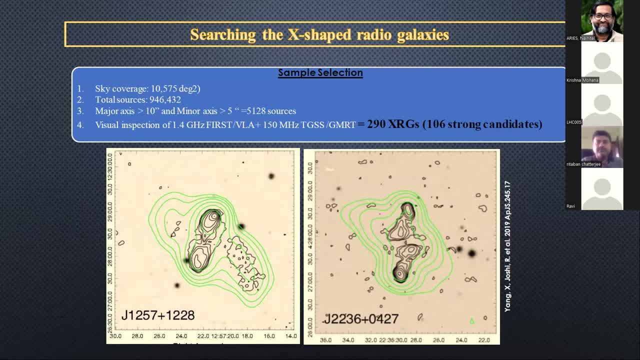 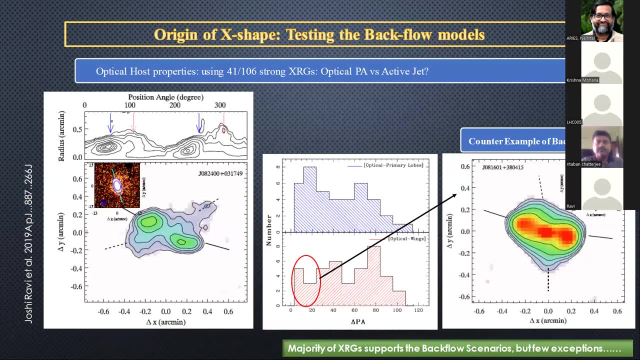 sample of 106 strong X-shaped radio galaxies. we tried to look for various correlations based on the optical host property. So first of all we questioned the backward scenario model. So for the optical host property, we have used about 41 X-shaped radio galaxies for which the optical images were adequate to 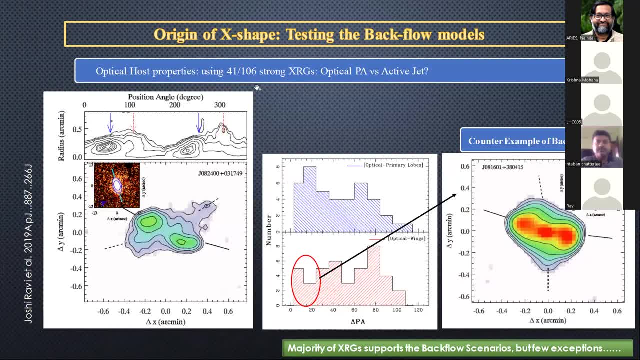 calculate the major axis of the galaxy. So what you see here is that this is the optical host and this is the major axis of the optical host if we plot it. And similarly, the position, angles of the waves and as well as the active jet have been determined. So if you just compare the 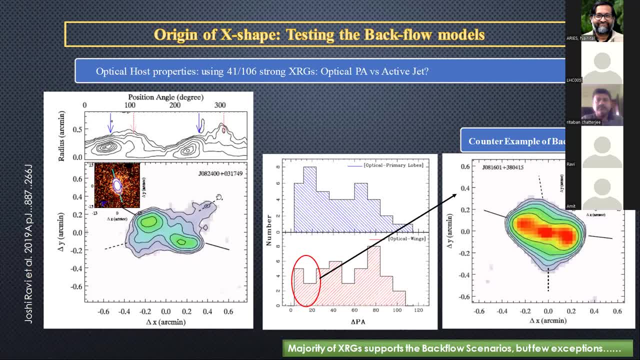 difference between the optical major axis with the wings position angle. that is being plotted here in the Brents diagram. So what you see here, apparently, is that the difference between the major axis of the optical host and the wings is mostly larger than 60 degree or say 40 degree, However. so this essentially, like again supports the backward. 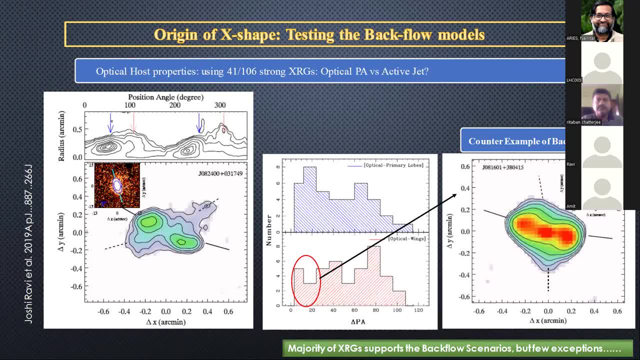 scenario model, But we have found a few exceptional cases also. These are the counter examples, where we found that the optical major axis is more or less aligned along the wings of these, along the wings of the radio structure. So this becomes basically so: one set of the systems supports the backwards scenario. but there are counter examples also. 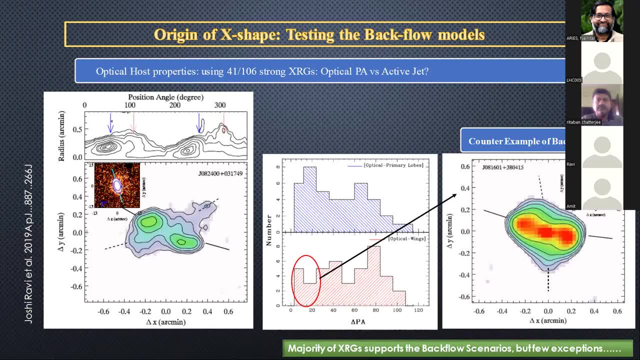 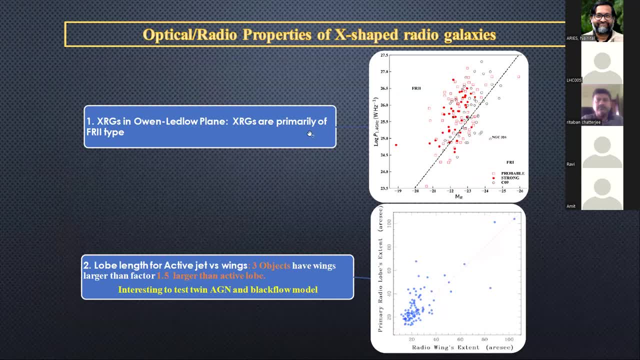 So this becomes essential to like test this scenario. The other thing, of course: one can plot the various observed quantity. For example, if you put all these galaxies in the overlapping plane, which is nothing but the radio luminosity as a function of absolute magnitude, then you can see that all of them lie in the locus between the. 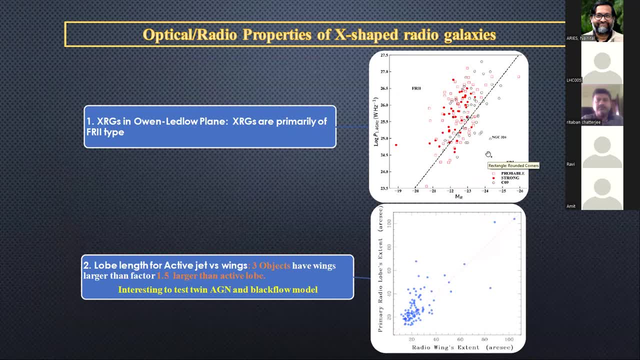 FR2 and FR1 kind of radio galaxies. This hints that probably these systems are transiting from one phase to other, But this needs more investigation If you compare, for example, the low length of the active jet and the wings in these systems. So for three of the systems. 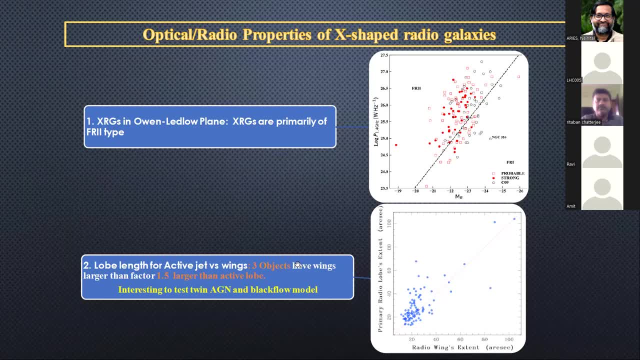 we found that the wings are almost like factor two larger than the active jet. So this is interesting and this may be like the. this kind of examples will be the best to test the various scenarios, For example, the twin AGM scenario or the backflow model. 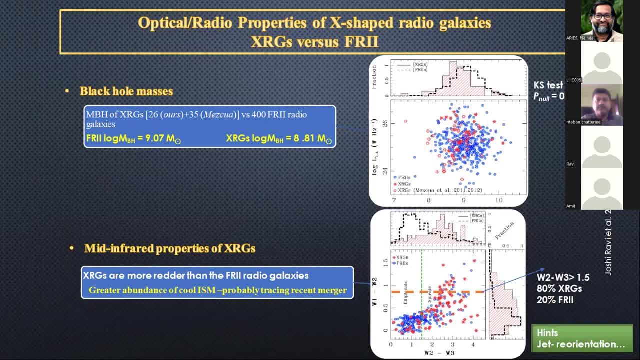 Well, further we look for. see, as I said, like this, X-shaped radio galaxies are primarily hosted in the FR2 kind of radio galaxies. So it's interesting to compare how these X-shaped radio galaxies correlates with their classical FR2 kind of system. So for this, first of all, we compare the black hole masses and for this we have 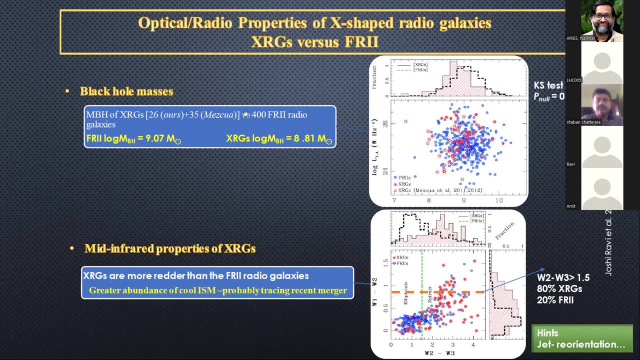 compiled about 61 systems from the Sloan survey and compared with the control sample of about 400 FR2 galaxies, almost at the same redshift. and this has been plotted here. So what? the red stars? what you see, they are the. they represent the X-shaped radio galaxies and the blue stars. 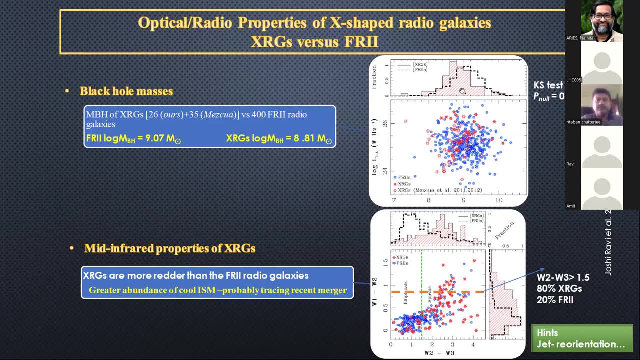 represents the classical FR2 system. The same has been drawn here in the histogram. So the red hatched systems are: belongs to the X-shaped radio galaxies. So if you compare the masses, so for the so we found that these X-shaped radio galaxies are systematically lower. 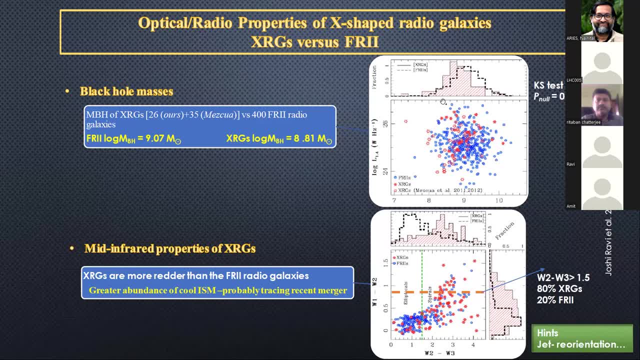 You have two more minutes. Okay, they are systematically lower than the FR2 kind of systems. They think that even even even in a minor measure will lead to the jet orientation in this kind of systems. If you compare the medium private properties of these systems, again, the convention is: 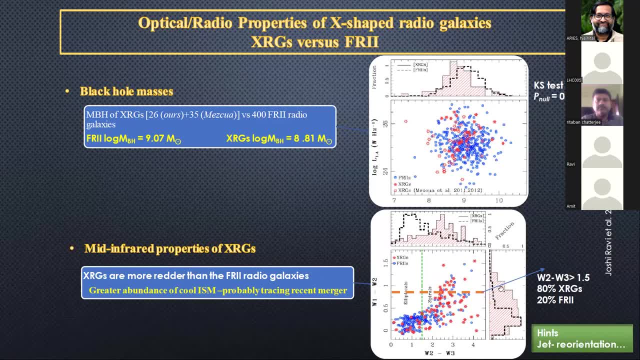 saying the red stars are the X-shaped radio galaxies, Then we found that almost 80 percent of these systems are having white color more than 1.5, whereas only 20 percent of FR2 galaxies shows the redder behavior. So, given they are dead and 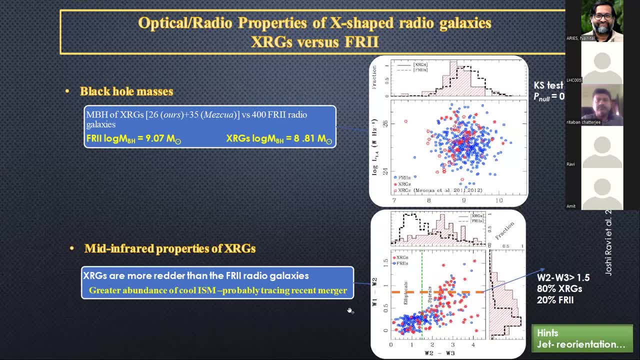 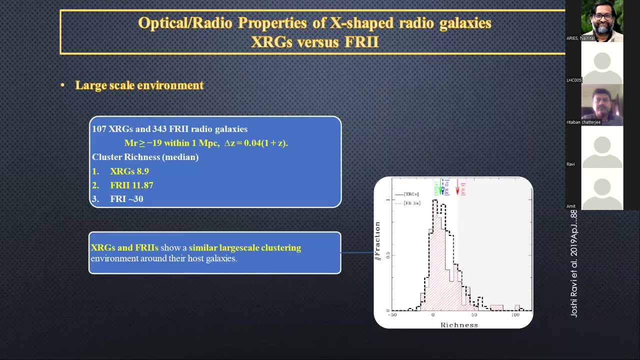 probably they are evident with the cool ISM and probably tracing the recent merger. So these two evidences support the jet reorientation scenario. Well, one can look for the large scale environment as well, given that the large scale environment will will drive the shape of the jets We try to. 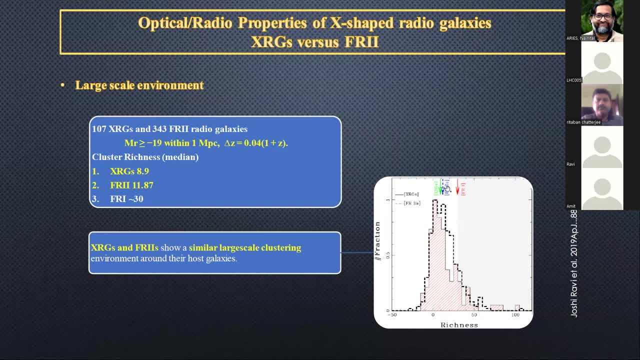 compare it for the X-shaped radio galaxies along with the FR2 systems and FR1 systems, which is being plotted here, And you can see that for both the FR1 and for both, for both the X-shaped radio galaxies and FR2 systems, they they live in relatively poor environment with a richness of about 10.. Whereas the FR1. 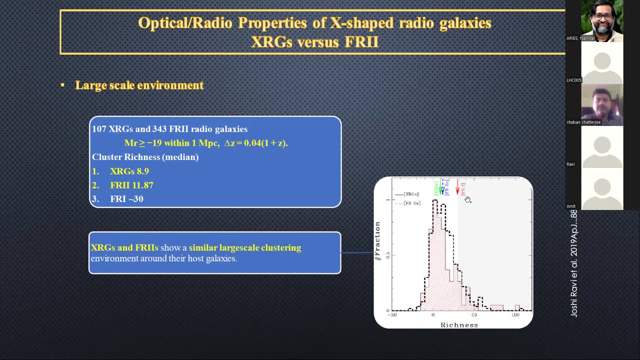 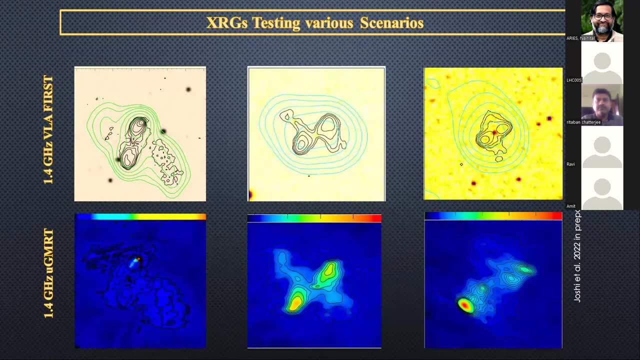 kind of systems. they live in the high density environment. So there is some similarity between the X-shaped radio galaxies and FR2 systems in terms of the large scale environment. However, to understand like more about these systems, we are following them with the various telescopes, like with the VLBA and UGM-RD. So here are a few examples I have shown. So what? 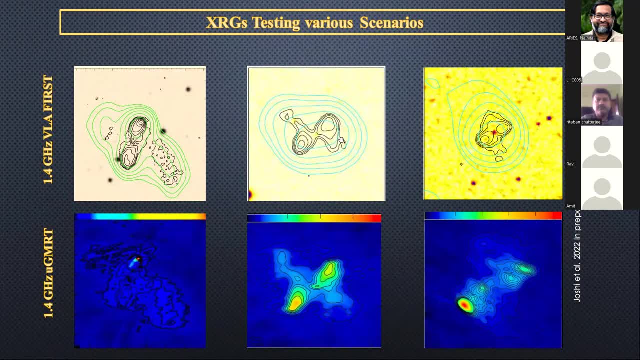 you see in the top panel, these are the 1.4 gigahertz first images and overlaid with the TGSS maps. And the bottom panel shows our recent 1.4 gigahertz UGM-RD survey images. So now we are trying to get data. 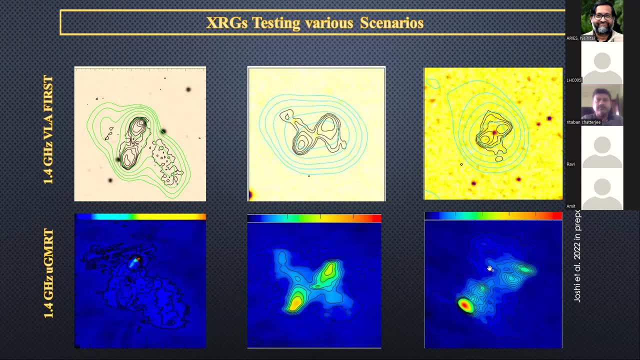 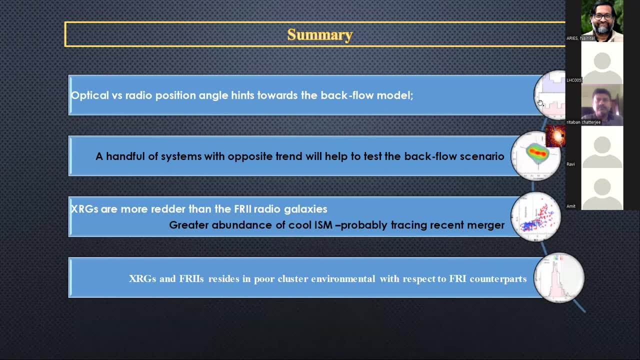 like different frequencies, to map the spectrum index and try to constrain various scenarios. So in conclusion, I will just say that what we have seen so far is that we have seen that the optical and radio position angle alignment actually hints that the backflow scenario may be. 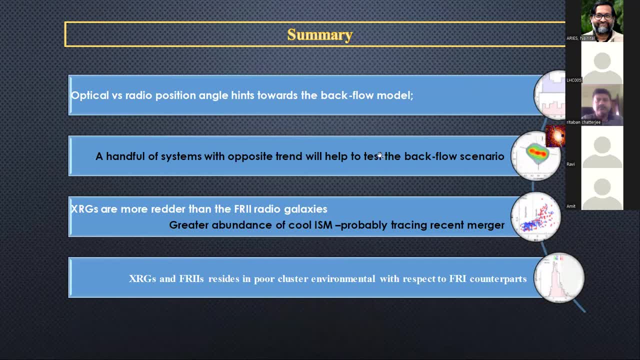 that backflow scenario may be in the act But, however, the handful of the systems also show the opposite trends. So it will be better to investigate these systems to test the backflow scenario. In terms of the rattling of the actual video galaxies, they hint that probably rattling as well as the masses of 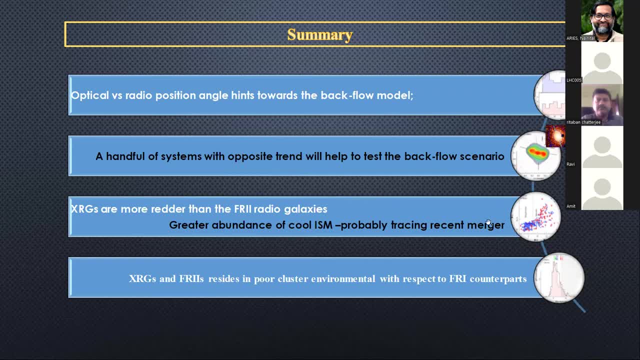 these systems hints that probably they are. we are tracing the recent merging and probably this is led by the trajectory orientation scenario And, of course, the large-scale environment of the FR2 and actual video galaxy is going to be similar. So we are following this and 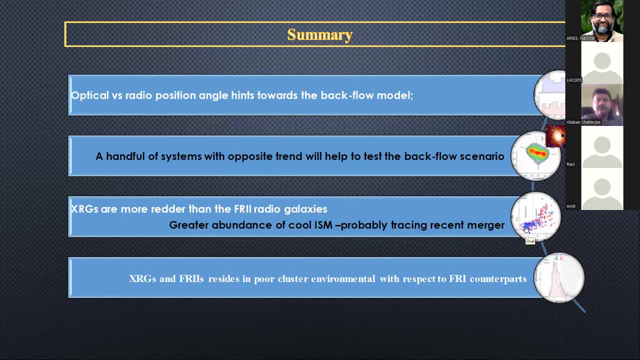 to. we are following this with various telescopes to understand the various possible scenarios. Thank you, Okay, thank you, Ravi. So is there any question in the in in the hall? Hi, thanks for that nice talk, Ravi. So my question is: you said that that you you have about 250. 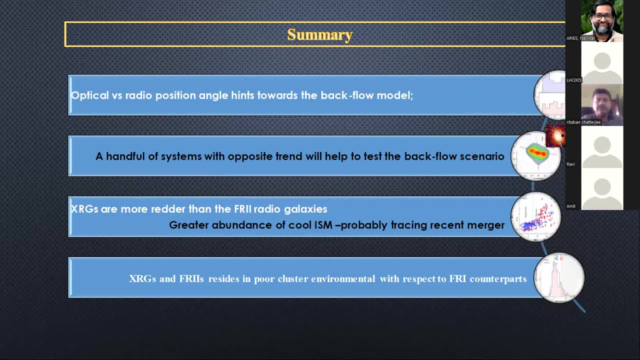 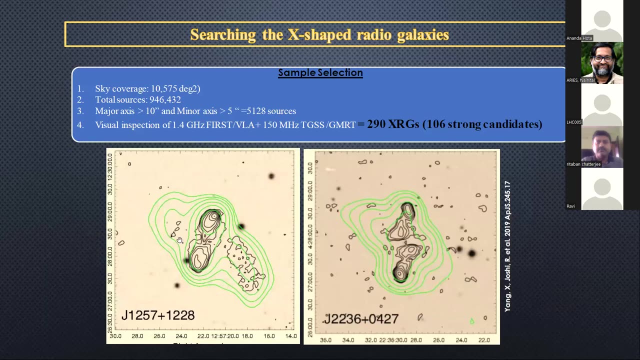 candidates and you have 106 strong egg-shaped radio galaxies, right? So about six or seven more than the previously Recorded about 100.. So what is the criteria you use to classify as uh, x-shaped versus some low axial ratio galaxy? Yeah, so so basically for the, for the x-shaped thing, we demand that, uh, given the first resolution, 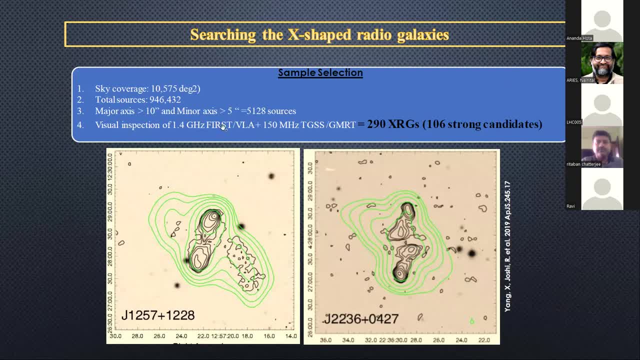 because these are, uh, these have been basically selected based on the first survey and and supplemented with the 150 megahertz pvc survey. So we demand that, uh, the the axis ratio, like the major axis should be more than 10 up second and the minor axis should be more than five up second. That is the resolution. 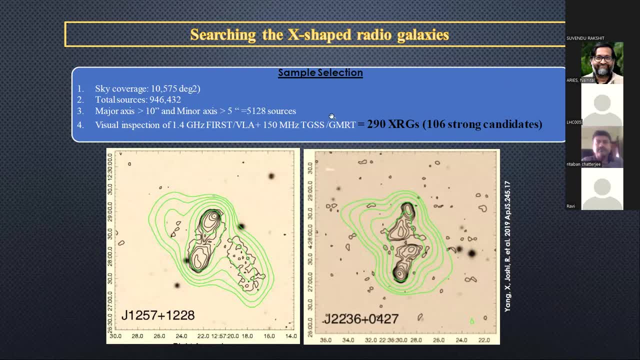 of the VLA And, yeah, and for as far as like the strong and the problem candidate systems. So we know that, like when we go over the visual, that is like highly subjective classification. So we basically with three of our, our authors, have independently checked. 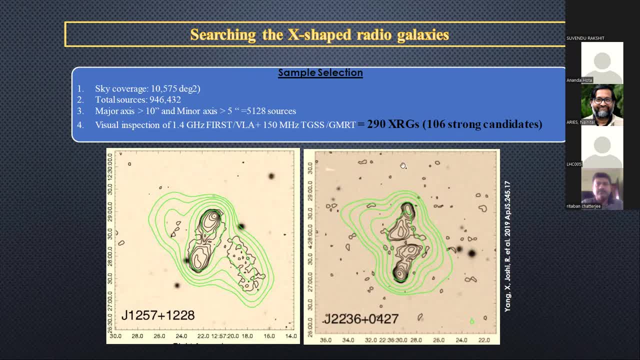 those systems and, based on those flags, we have go for the strong end of the problems. Okay, so is there any other question offline? Yes, sir, there is a question also. Yes, please, please, go ahead, Hi Rabhi. so, uh, this slide number eight, where you showed, like, uh, your except galaxies. 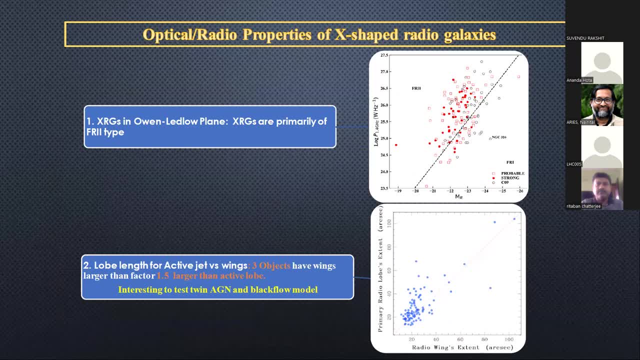 as well as fr1, fr2 and they all are overlapping. So just for the clarification that you said that maybe it is the somewhere in transition phase from fr1 or fr2.. Am I correct? Yeah, yeah, So what? how? uh, yeah, so my uh. so that's why I'm getting confused that. 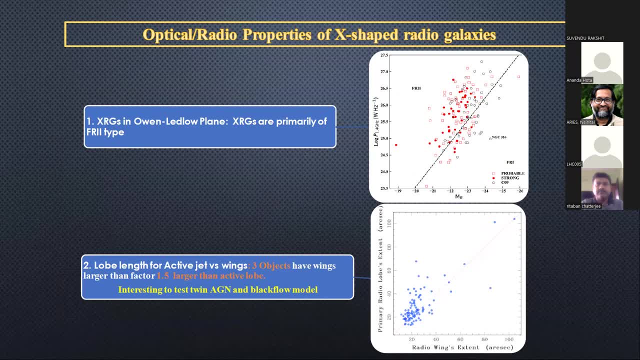 with what scenario process. but thinking that manner, that if it is transitioning from one to another, Yeah, so if you look at basically this, uh overnight domain, uh radial velocity versus the absolute magnitude, So this line basically divides the two, uh two systems. And if you look at the like, 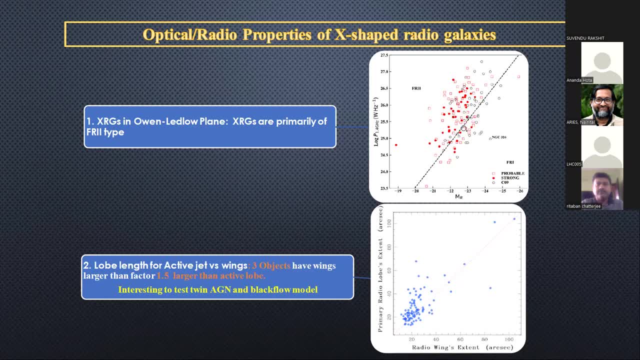 average power of the hypothesis. uh, the x-shaped radio galaxies, uh, they lie basically in between these two, So, uh, so. so that's why I said, probably it's the hint that we have to just carefully check whether, if they are transiting from one to other, Yeah, So what are, uh, what are the physical? 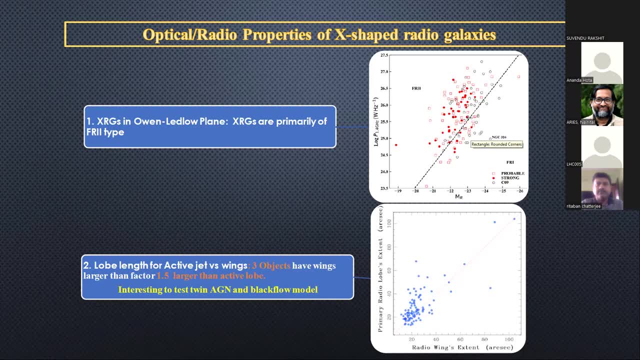 processes can be involved, like when you're saying transition. So I mean. So by the transitions I mean is essentially the aging of the, the electrons only. So yeah, but the time scales we do know, Okay. So, um, Anand Hota has a question online. So, Anand, could you please ask a question? 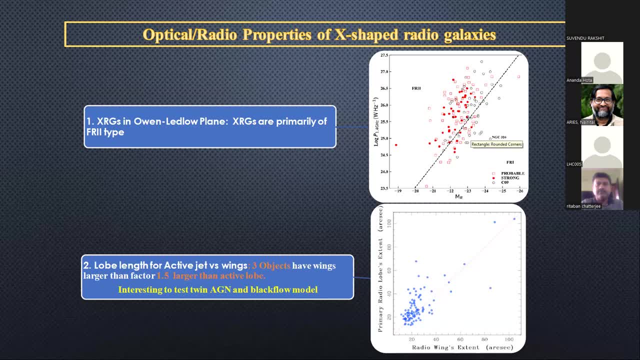 Hi, Can you hear me? Yes, I guess, yeah. Um, I have been thinking about this thing. One question: I would like to say that people connect the wing direction with minor axis of the optical host. Yes, And it doesn't explain everything. 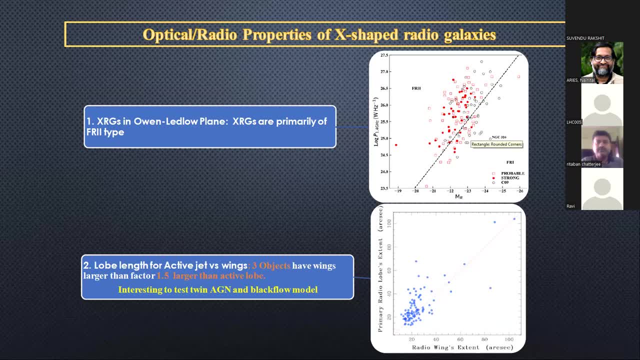 And the backflow model people are also supporting now because of this new uh meerkat image. Yes, Very impressive image. Yes, What I find people are missing is the uh Gopal cited one of my paper on NGC 3801.. The rotation axis of the gas people are not looking at very carefully. Yes, Because 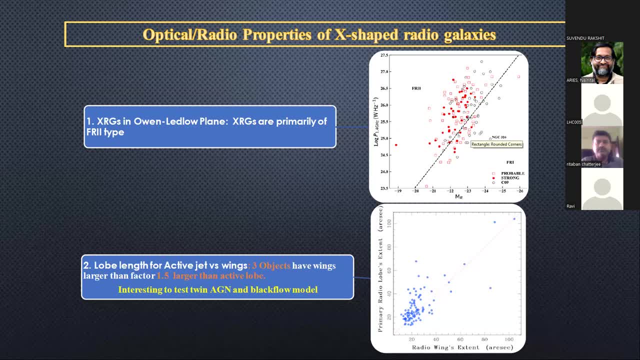 the 3801 is a kinematically decoupled core. The active lobe may be responding to the central part, but the outer region could be saved by the outer region's gas dynamics. So people should look at the rotation of the gas in these systems. 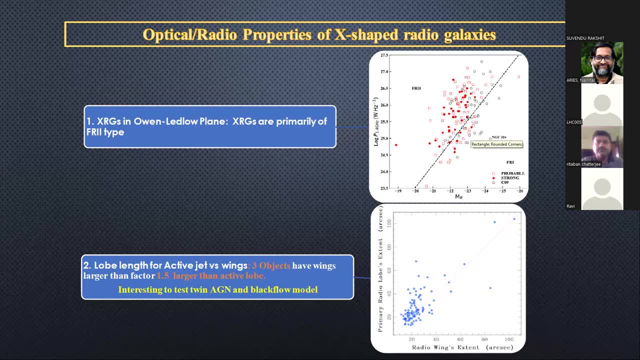 Yeah, I agree actually. So so, regarding this, we have basically- so that is basically a situation- the kind of shell model, right, and you can have. so we, we look like all these uh 290 systems for the deep optical images. uh, that is from the decal survey and, unfortunately, 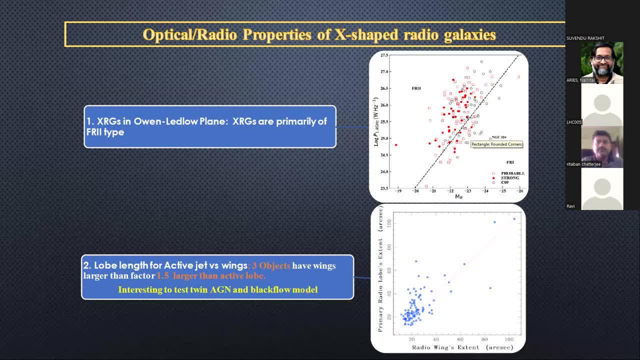 none of them. uh, host the shell, given the probably the redshift, the relatively high redshift of these. so, yeah, no, no, no, no, no, no. I'm not talking about stellar cells, what I'm talking about the gas dynamics there, so that at least there is a long slit spectroscopy done for the center. 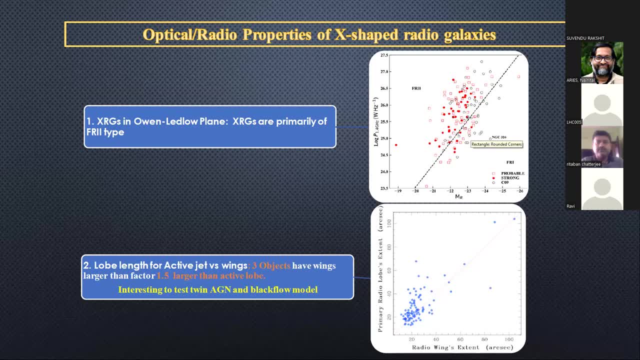 what is the rotation direction of the gas in the system more stronger than the gas and stars, plasma and the stars in the system? yes, yeah, yeah, so okay, thank you. thank you, we will talk later about sure, okay, so, uh, there's a question. yeah, hi, Ravi, so nice talk. so I'm wondering, uh, do you have any IFU observations? 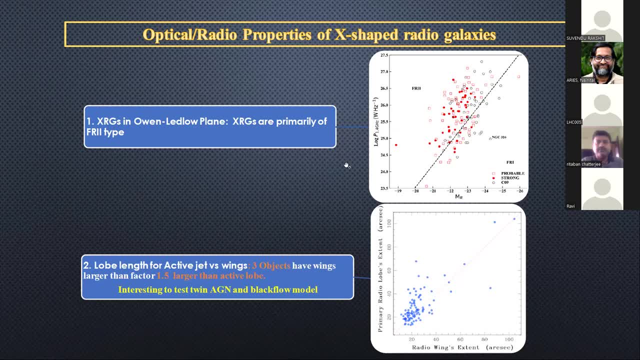 on these sources? uh, not really. uh, I have not checked the literature for that, but uh, I'm not very sure we need to check, okay, or any, uh, like a long slit spectroscopy along the direction of the exit, like both direction. uh, in the cross, like, like, as Anand said, like this can be like one of the things. 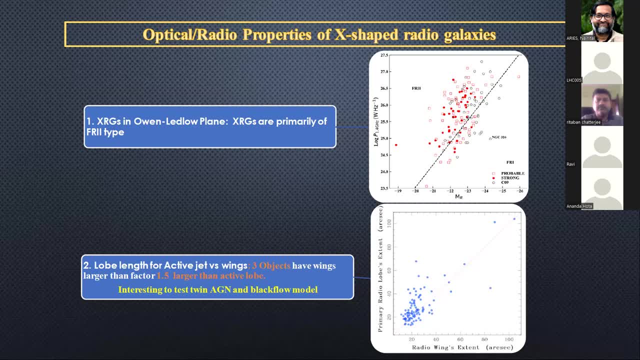 that is necessary for the follow-up, but, uh, no, because what we are relying mostly on the archival data right now. okay, and the masses that you mentioned, black hole masses- they are calculated by m sigma or how? yeah, these? these basically come from the stellar velocity question measurement. 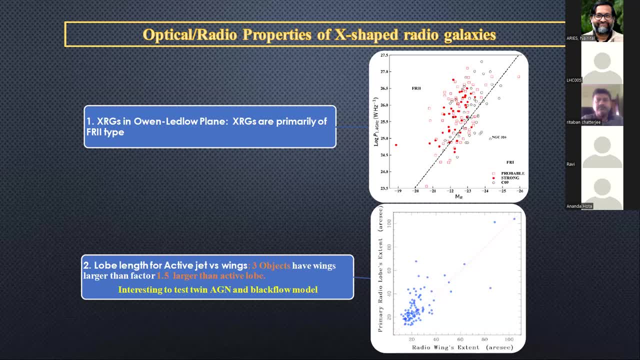 okay, yeah, okay, thanks, yeah, okay. so, um, I think I will uh. so that would be uh. if there are further questions, please uh contact the speaker after the session. i would like to mention that uh, pankaj kushwa made a comment to krishna mahana on the chat.